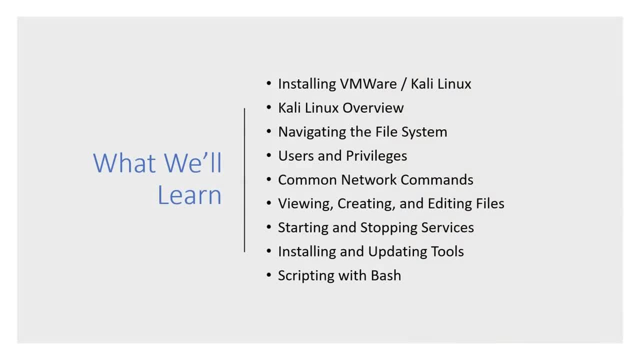 what we'll learn in this course. So this course is going to be all hands on. Besides this little introduction here, you're not going to see a lot of PowerPoint besides quick overview of what the course or the video that you're about to see has coming. So 95% hands on. course I will not kill. 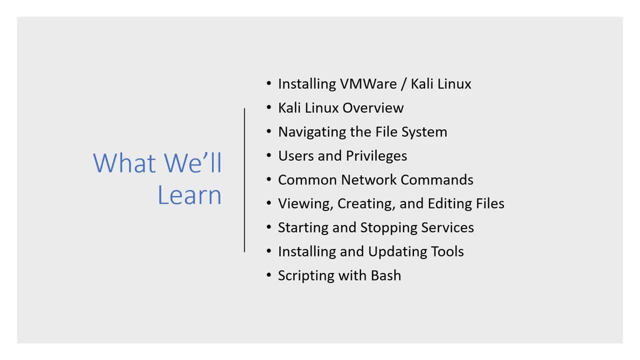 you with PowerPoint. That's not my goal. We're going to be focusing on Kali Linux, which is a deep dive into the terminal. So what that means is we're going to be hands on learning Kali Linux this entire course and really learning Linux, and learning Linux for the purpose of becoming ethical. 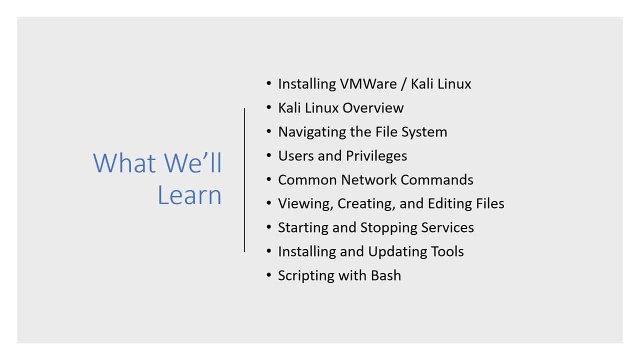 hackers. So we're going to install VMware, which is a virtualized software, virtualization software- And then we're going to run Kali Linux inside of VMware. After that, I'm going to give you a overview of Kali Linux, show you some of the common tools, what it can do, why it's awesome And. 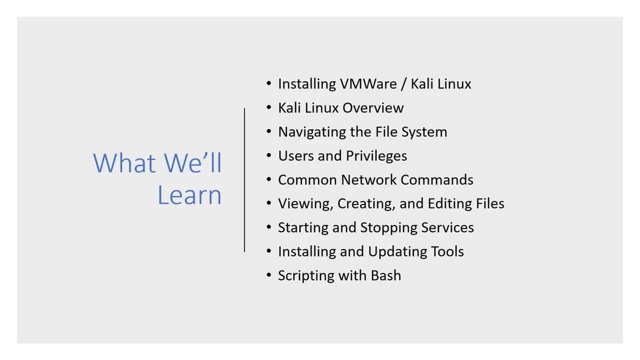 then we're going to do a deep dive into the terminal. So what that means is we're going to be hands on doing commands and learning Linux. So we'll be running, navigating the file system, So how to get around in the file system. from the terminal. we'll learn about users and privileges. 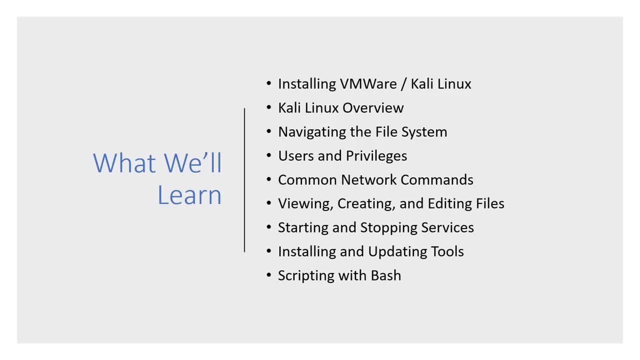 how to add users, how to. what kind of privileges and permissions are there? what important files exist regarding those? we're going to talk about common network commands. So if you want to be a pen tester, ethical hacker, you need to know networking, at least at a basic minimum. So we'll 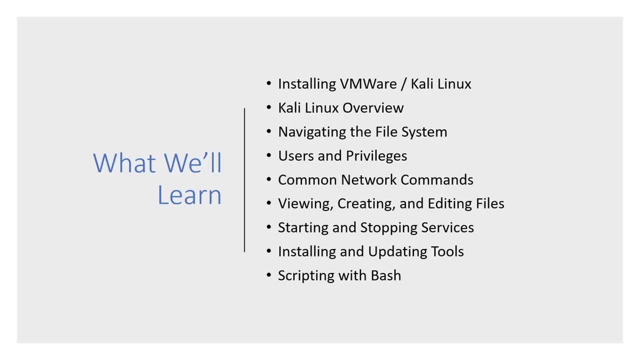 talk about those common network commands that you should know how to run them, what they do. We'll talk about viewing, creating and editing files. That's obviously important If you want to create a quick file or edit a file from the command line- how you can do that. We'll talk about starting and 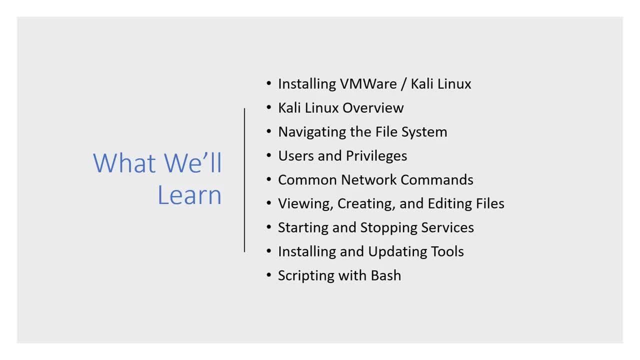 stopping services such as a web server, SSH, SQL database, etc. We're going to talk about how to install updates, how to install tools and how to update those tools, And then, lastly, we're going to put everything we learned together and do some scripting. 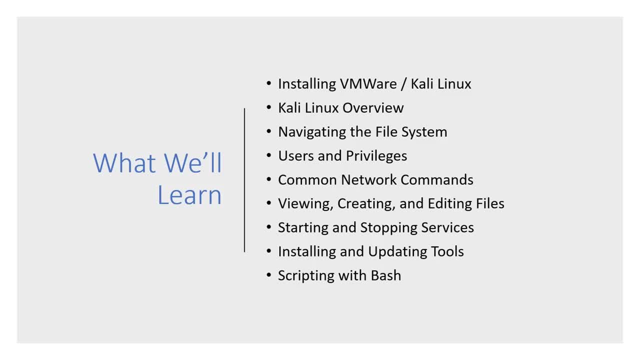 So we're going to write a basic bash script and then we'll improve upon it, And then I'll show you some for loops, some other logical scripting ideas, And then we'll kind of put that together and hopefully come to a nice completion when it's all said and done. So, with all this being said, 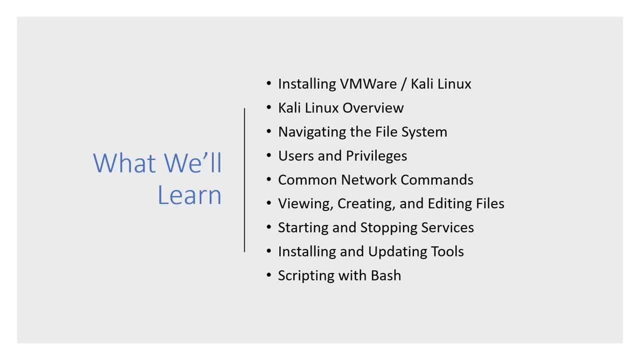 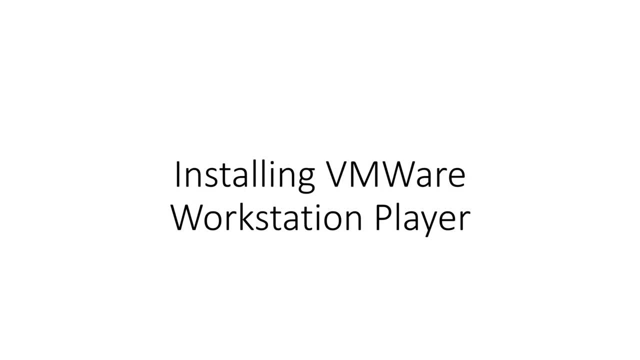 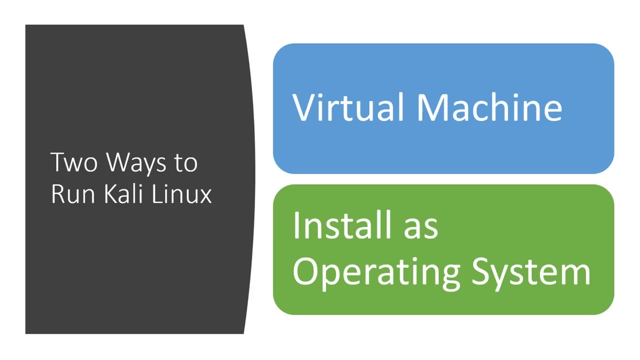 I'm excited to have you in the course with me. I look forward to teaching you, and let's go ahead and start with installing VMware. All right, the first thing we're going to do is we're going to install software called VMware Workstation Player. Now we have two ways to run Kali Linux. We can 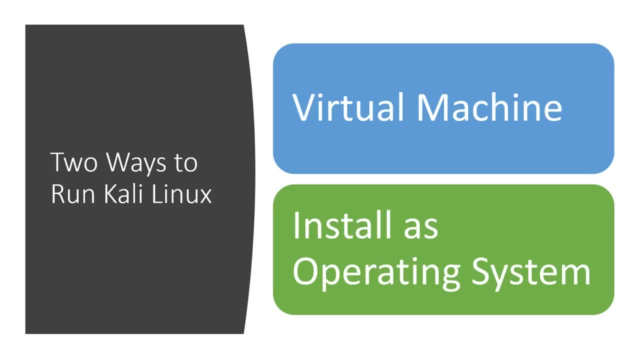 either run Kali Linux through a virtual machine or we can install it as an operating system on a hard drive. For this course and this lesson, we're going to be using a virtual machine And, preferably, we're going to be using VMware Workstation Player. I'm going to show you how to. 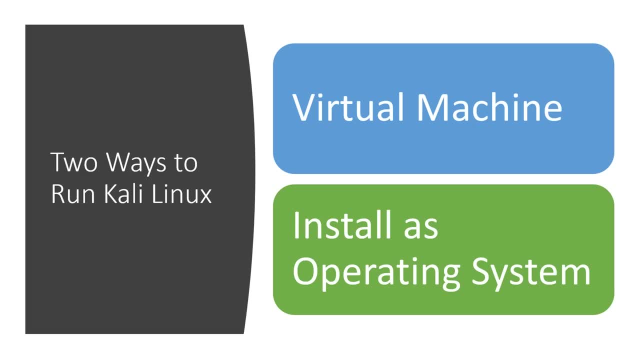 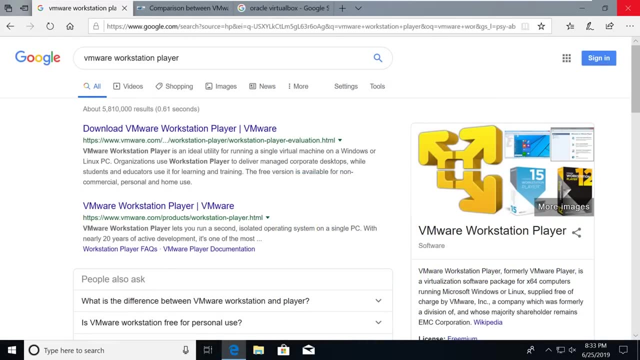 run VMware Workstation Player And I'll show you some of the alternatives to it as well. So let's go ahead and dive right in. Okay, so if you go out to the interweb and you go to Google and you type, 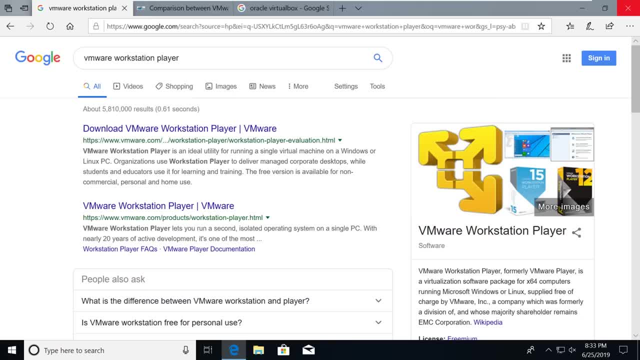 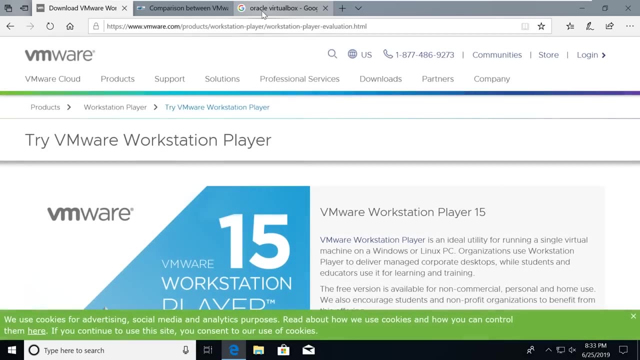 in VMware Workstation Player. the first thing that'll come up for you is this: download VMware Workstation Player link. you're going to go ahead and just click on this, And now I also want to show you the installation that's going on. So there is a another software platform called. 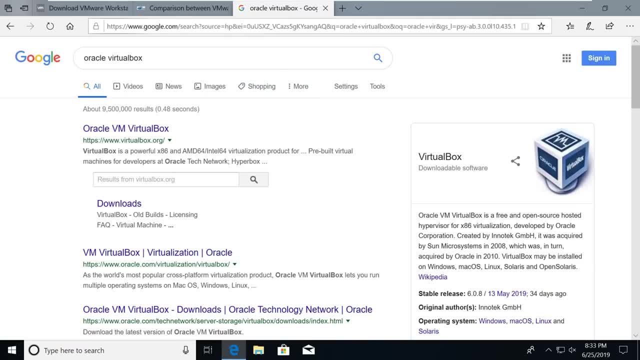 Oracle VirtualBox And you will be able to install either my preference and the course that's going to be taught. the rest of the way through is going to be in VMware Workstation Pro, But we will use Player for the install. you'll be able to follow along with Player. You'll also be able to follow. 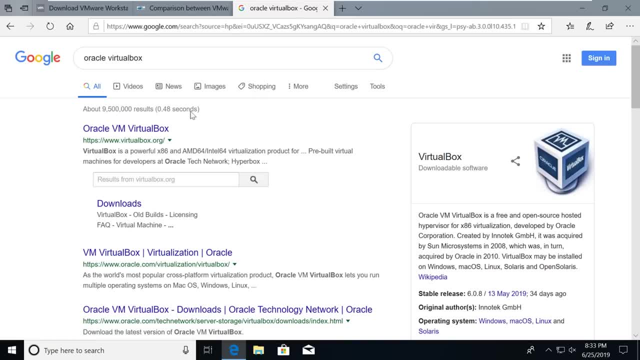 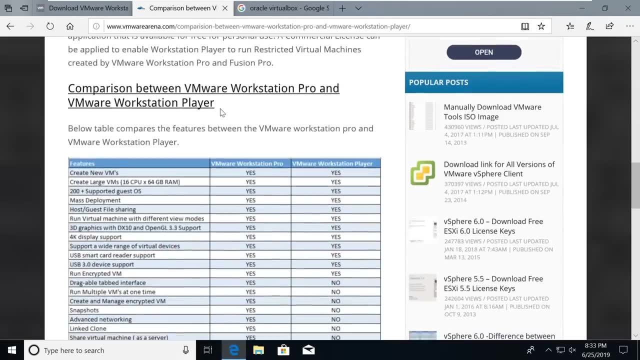 along with Oracle VirtualBox if you so choose, but we will not be showing that installation. Ryan Harklessillas 1.0 Kali Linux- 1.0 Kali Linux 100% page here and I will be using VMware Workstation Pro. There's a nice little checklist here that. 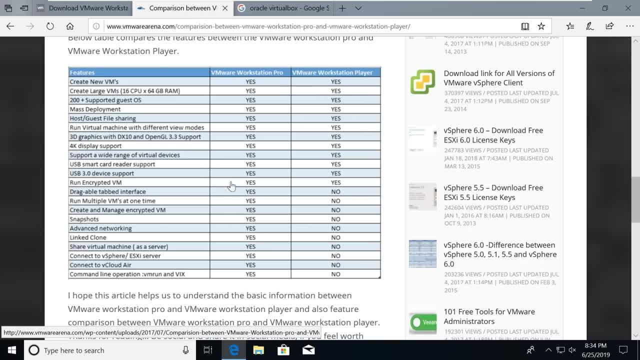 shows what pro can do versus player. It has a lot of the same features here. Some of the nice things is running multiple VMs at once. You can technically do that with VMware Workstation Player- There's workarounds for it- But to have it in a single tabbed interface it's very. 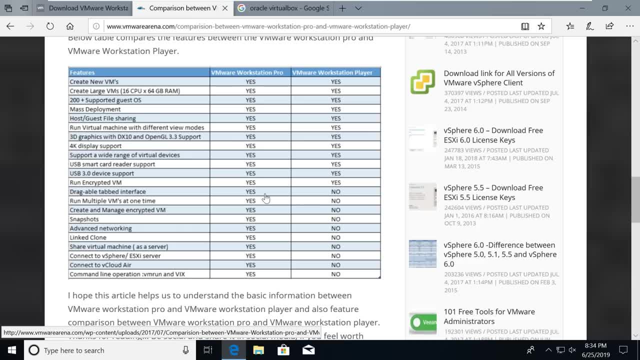 very nice. You see here the draggable tabbed interface. That's another feature: Snapshots, So basically making a backup of your machine, all included in Workstation Pro. So if you have some money to shell out and this is something that you're interested in doing, 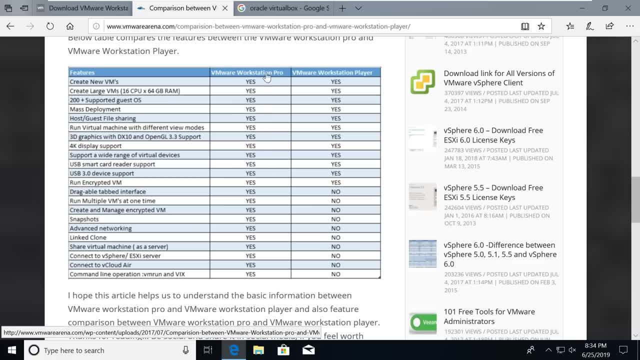 long term it may be worth looking into a Workstation Pro license, But by all means you can get away with a Workstation Player installation, And that's exactly what we're going to do. So let's go back to the first tab here And you can see it says: try VMware. 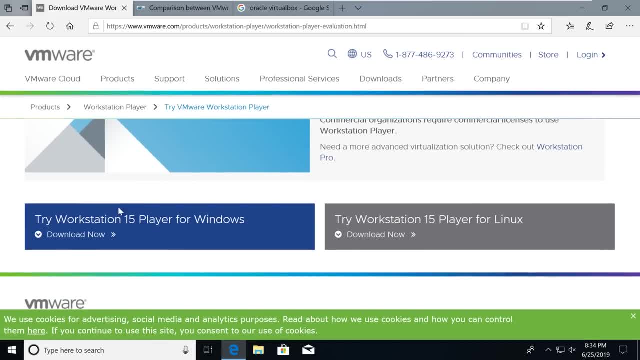 Workstation player. We're just going to scroll down and this install and everything is going to be running on top of Windows for me. If you're installing for Linux, that's fine as well. Just follow your instructions for your respective OS. Go ahead and select download. now I'm going to save the file. 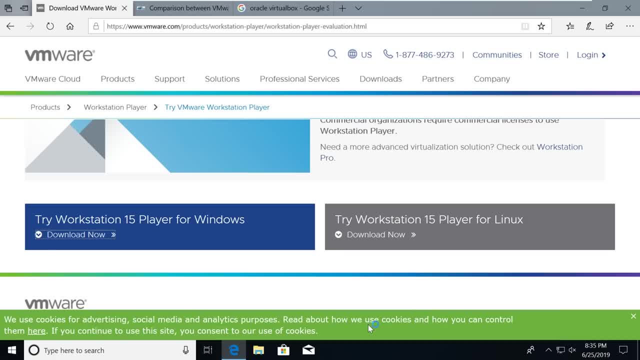 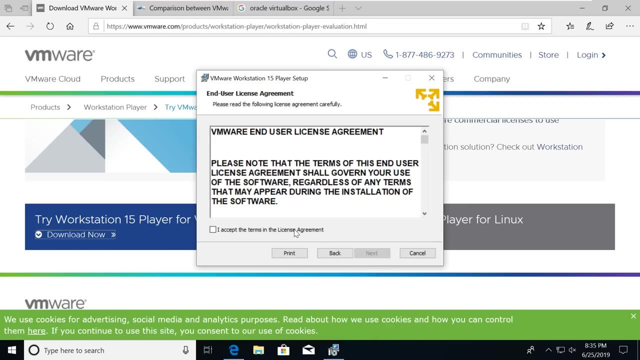 Okay, it downloaded. I'm going to hit run. It's going to ask if we want to accept the changes. Yes, Okay, now we're going to hit. next. We'll accept the license agreement and possibly give away our first born. I'm going to go ahead and check. yes, for the enhanced keyboard driver. 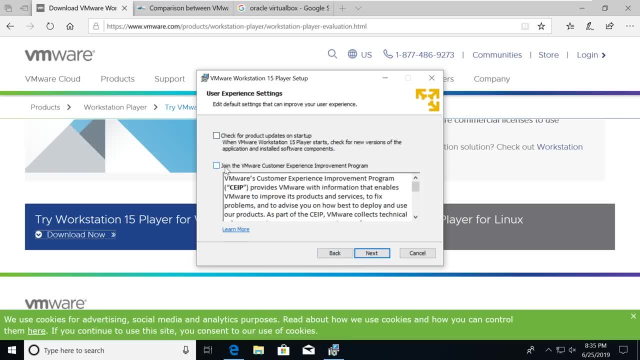 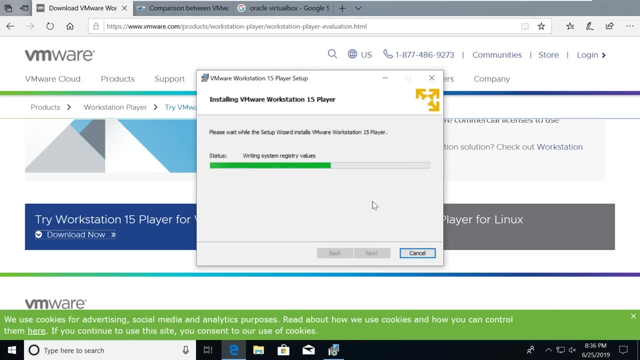 We don't need to check for a product update. We don't need to join the VMware customer experience improvement. We'll hit next on that. You can leave both of these checked or check to your preference, And then hit install. And while this is installing, I can actually show you what VMware Pro looks like. This is a pro. 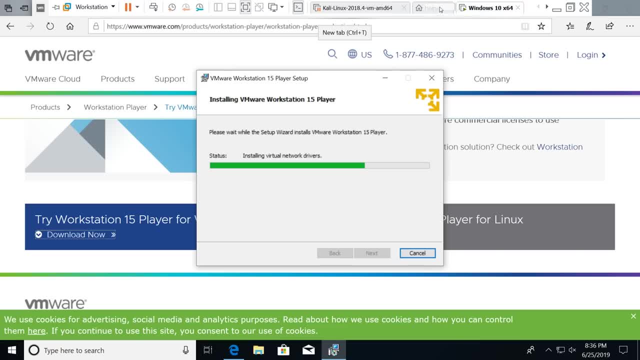 instance running here. You can see that I have the tabs and they're draggable, as it was notated in that, that differential spreadsheet that you saw, And I've got a Kali instance running. That's actually my main Kali machine. I've got Windows 10 running here And this is all actually sitting. 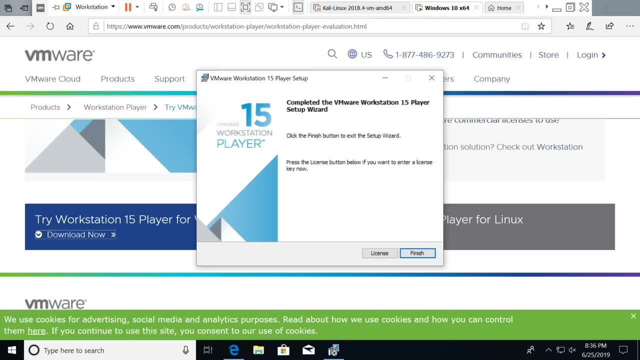 on top of a real Windows 10 machine. So I'm going to hit install And while this is installing, I'm going to run this workstation player. So we're just installing workstation player. I'm going to run it- a VM inside of a VM. So it's going to be a little bit of VM exception here, And then we're. 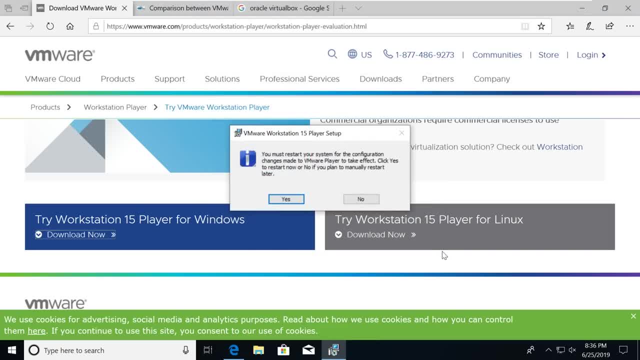 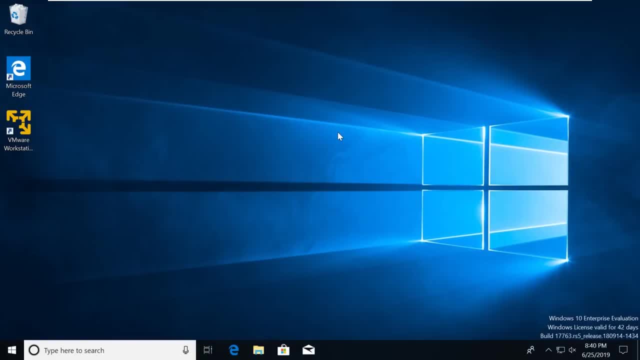 just going to hit finish And then we are going to restart this machine, as it needs a reboot real quick. Okay, now we are restarted And we're back to our desktop. here You can see that VMware workstation player has been added to the desktop. Let's just go ahead and double click that to 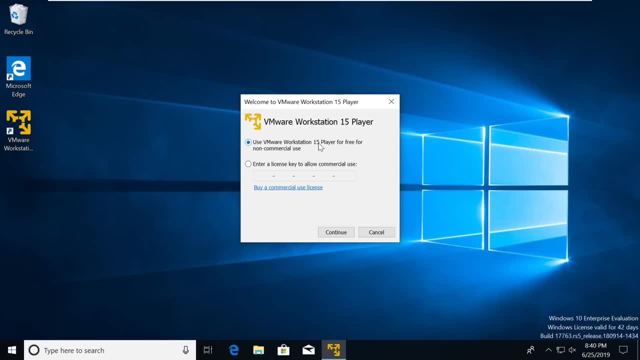 run And we're going to hit finish And then we're going to hit finish And then we're going to hit open it And we're going to choose to use VMware workstation 15 player for free for non commercial use. If we wanted the pro edition, we would enter in our access key here, our license key, and 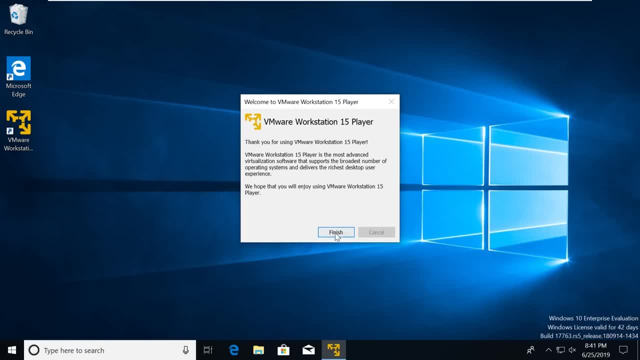 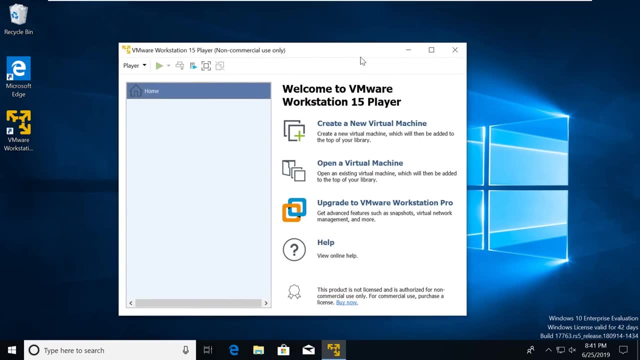 continue on with the pro edition, And now we will use the finish button here and we will be brought to our VMware workstation 15 player. So you can see here that it's a much, much different view. It's very, very basic. 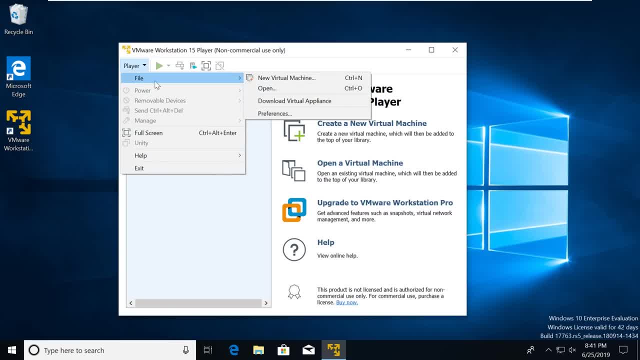 We have the option to open a VM here and we'll have the one VM stored in this tab that we can open up, And that'll be it. There are ways around running multiple VMs at the same time, But if you're looking to build a fluid lab out and have multiple VMs running, similar to what I have here, 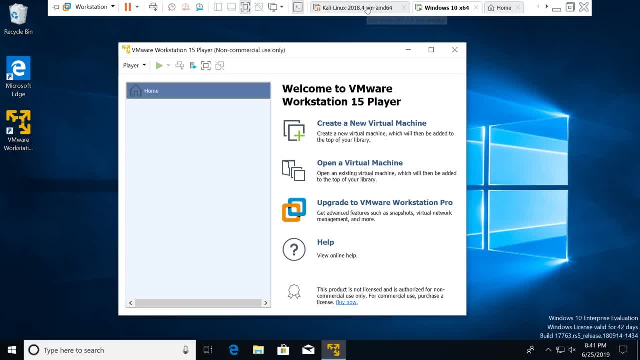 having the VMware pro again. it does have its benefits here. So you can see, this is a much, much different look. This is very generic, as we, we can see here. So from here, what we're going to do is we're going to go ahead and stop in the 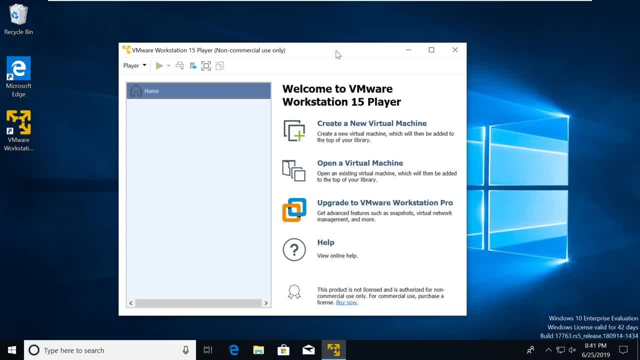 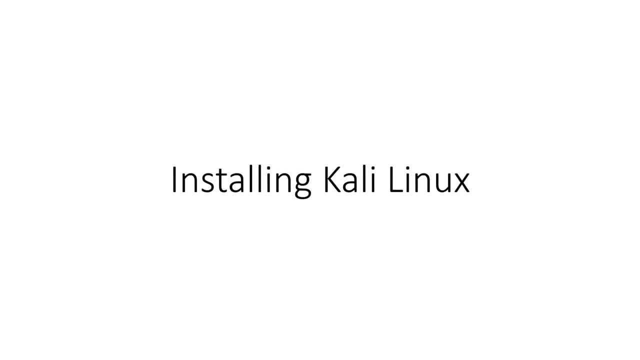 next video we are going to focus on downloading Kali Linux, And we'll talk about what Kali Linux is and some of its features as well. So I'll catch you over in the next video. All right, now let's move on to installing Kali Linux in our VMware software. Okay, 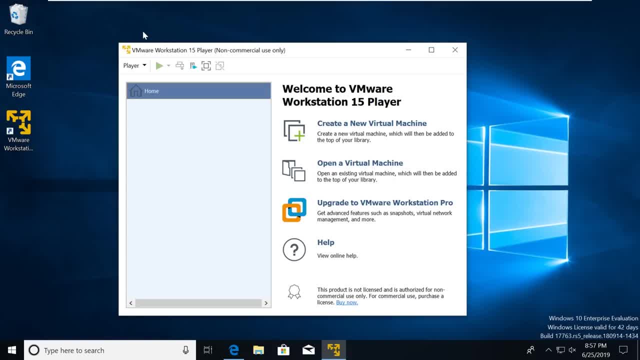 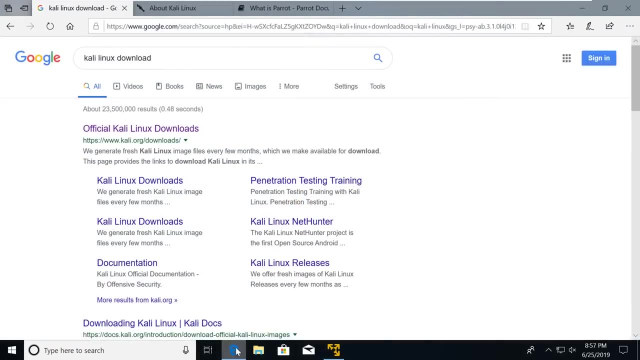 so, picking up where we left off, we had just installed VMware Workstation 15 player, And now we need a VM to actually be able to play with it. So this whole course is going to be based on Kali Linux. If we open up a internet browser here, I've got a few tabs already opened. So what I want you? 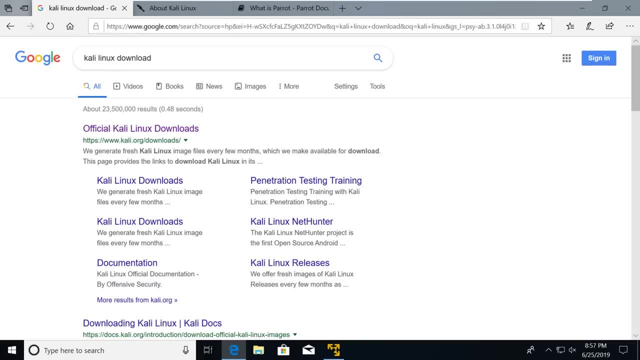 to do is go ahead and go out to Google and just type in Kali K-A-L-I Linux download and leave it here. What we're going to do as well is: I want to talk just a quick second about what Kali Linux. 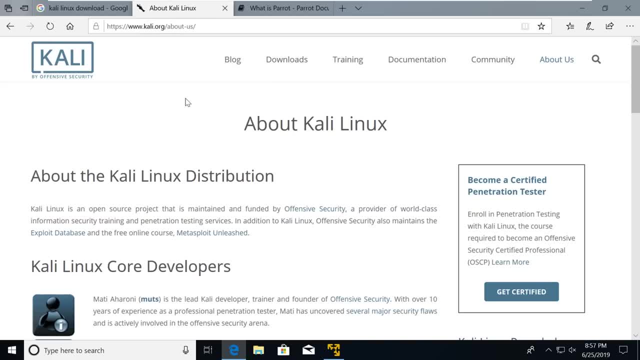 is So. Kali Linux is a Debian based Linux OS, So it's based on pen testing tools and it's made for pen testers. So what it does is it comes preloaded with a bunch of penetration testing tools- a toolkit, if you'll call it- And it is just made for. 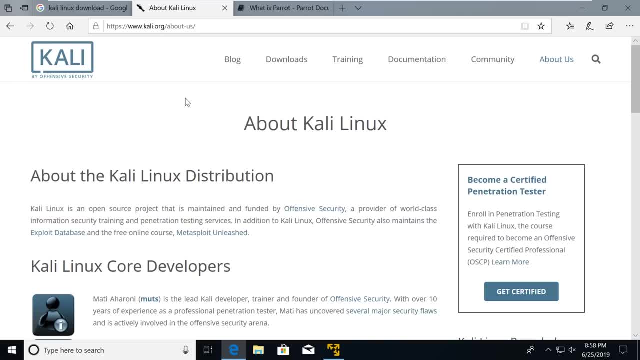 people who are looking to do pen testing. So this is provided by offensive security. If you come to kaliorg and you look at the about us, it provides a little bit of information about who the core developers were and some of the moderators, But basically what it is. is it followed up a tool? 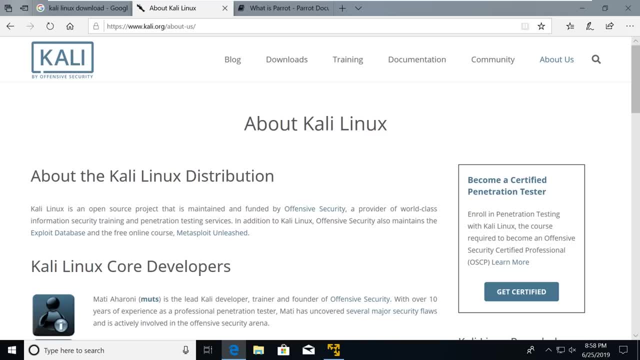 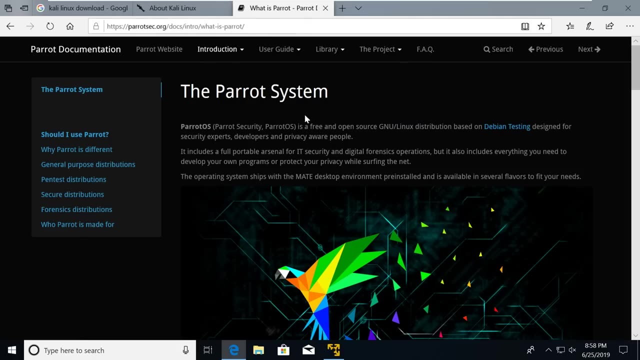 called or distribution called, backtrack. So the new, the new tool is Kali Linux. Now there are alternatives out there. One of the alternatives right now is called parrot. So if you go to parrot secorg and you look into what is parrot, you can see that they have different distributions And they talk about why. 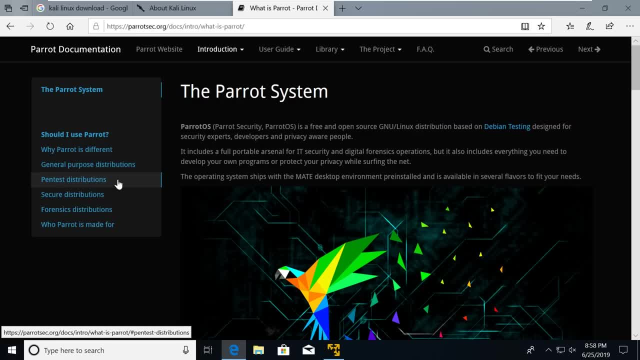 parrots different, but they do have a pen test distribution here. So for this course we're going to be using Kali Linux, but I always do like to introduce the alternatives. Kali Linux is probably more popular at this point. parrot OS is kind of on the way. 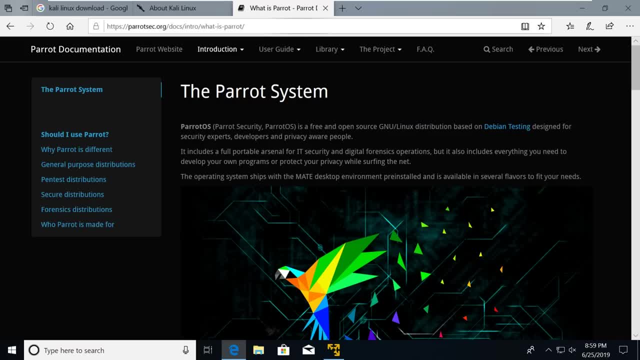 newer side. some people are starting to get behind it and liking it, But I would say Kali still dominates. The third option is that you set up your own distribution, So you have an OS that you like and then you install the tools on the OS that you like and you have your own custom build. 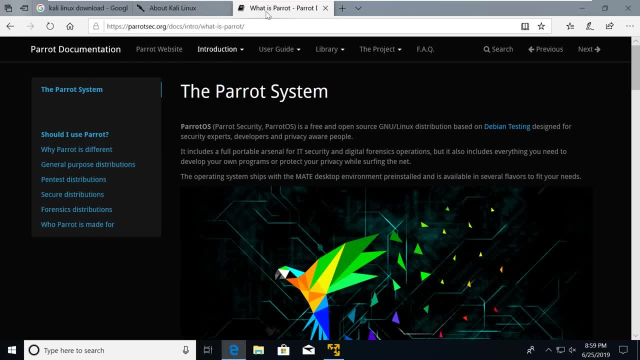 So some people feel like you know Kali or even Parrot, they come with a bunch of tools that they'll never need, So their systems bloated and they really just have a set amount of tools that they like And if there's a tool that they want to add into the system, then they'll download that. 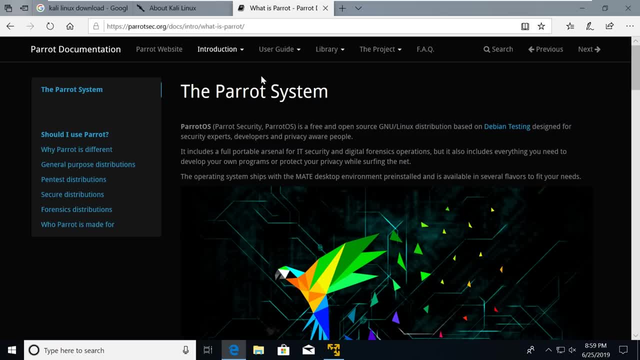 on their own. They don't want to have a ton of bloatware coming with their system. But with my experience in the industry, mostly everybody that I've worked with is using Kali Linux. Some people are doing their own builds, especially on, like the web app, pen testing side, And then now Parrot is 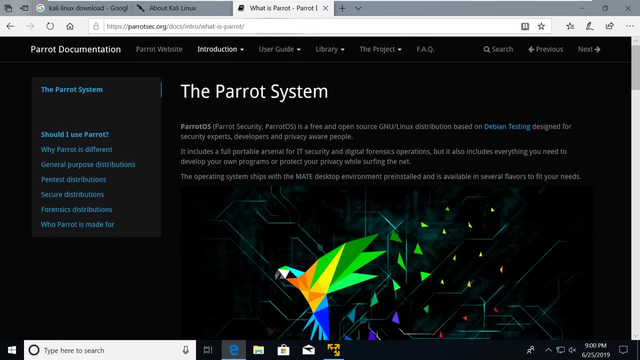 kind of that up and coming OS that some people are transitioning to, but it is predominantly Kali Linux. So that is why we're doing this course in Kali Linux, And I feel like it's the best option for us to learn some- just some- basic Linux skills and learn it in the OS that is the most dominant in the industry. 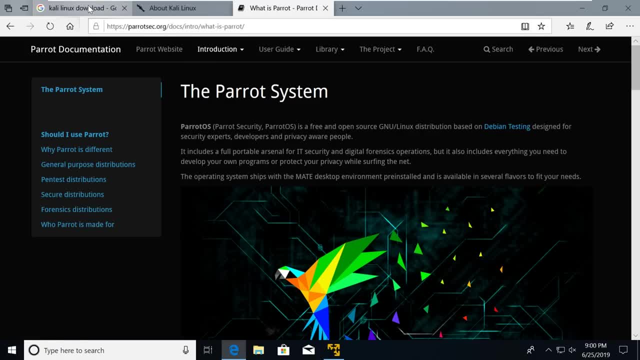 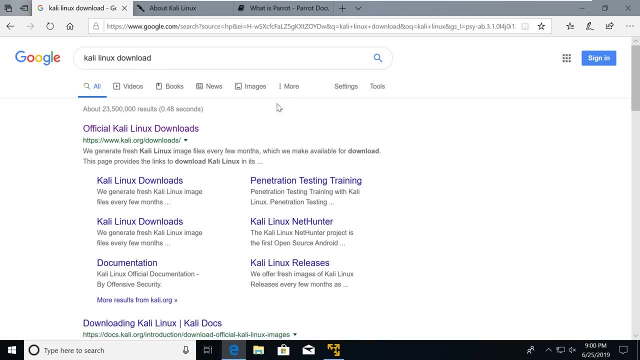 right now. So let's go ahead and go back to that Kali Linux download. And while this link has been clicked on, do not let it fool you. we're actually not clicking on the official Kali Linux downloads page. we're going to scroll down a little bit. I want to go to the Kali Linux custom. 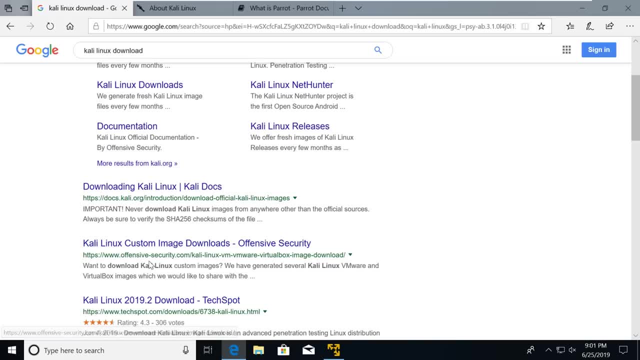 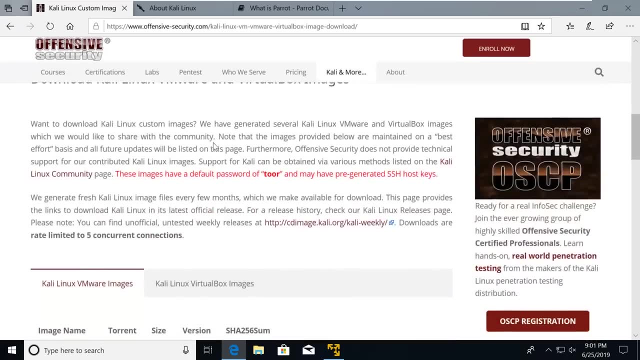 image downloads page And I'll show you why here. So this is that offensive dash securitycom- Make sure that's the one you're following along with- And if you scroll down just a bit, you see that they're providing us VMware images and VirtualBox images. So remember when I told you that VirtualBox 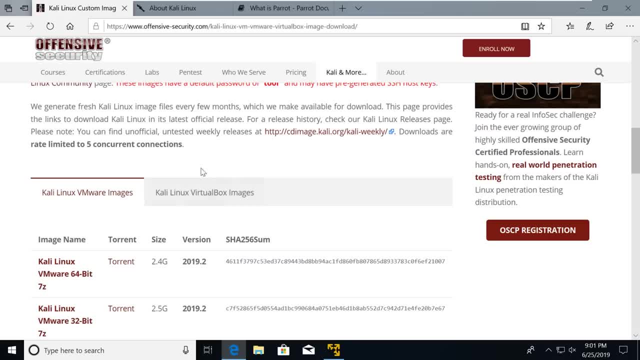 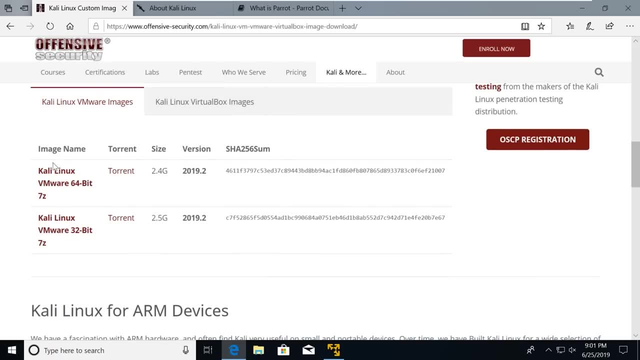 was an option. If you chose that option, here you go right here, you'll click on this tab and you will download the VirtualBox image. Now what we're going to be doing is we're going to be running a bit And we're going to download this seven zip right here. you also have the option to download a. 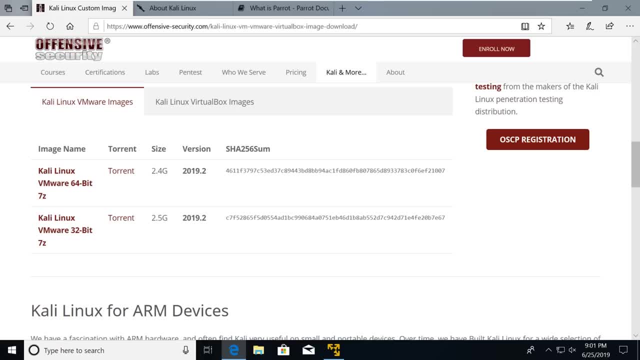 torrent if you'd like. the file size is going to be 2.4 gigs So it might take you a minute, depending on your your speed of your internet, And they also provide a shot to 56. Some, if you want to. 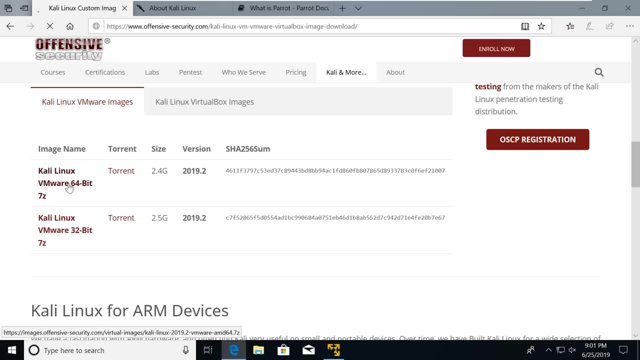 check the file when you download it. So I'm going to go ahead and just hit download on this And I'm going to save it And I will come back as soon as this file is finished downloading. Okay, so my file has finished downloading. 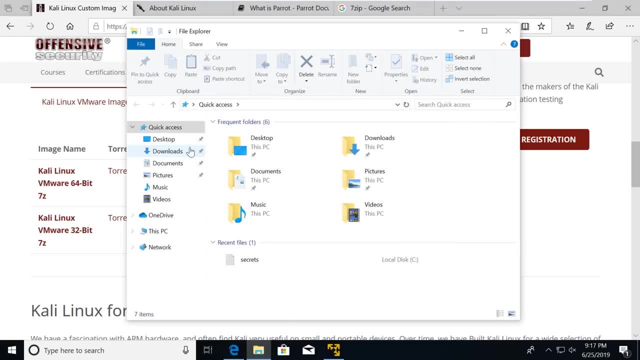 I'm going to navigate to the folder where it has downloaded to, which is the downloads folder, And you can see here that it is a seven zip file. So my installation by default does not have seven zip. If you do not have seven zip either, we can go ahead and download that together. 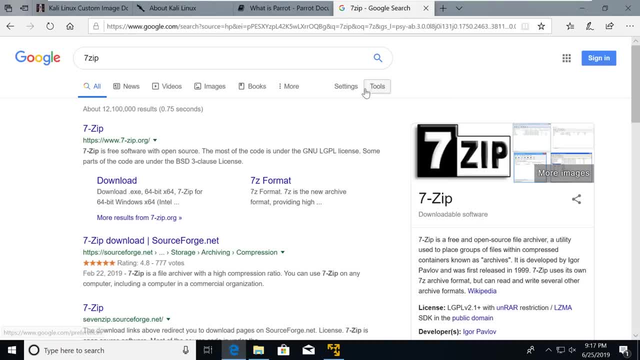 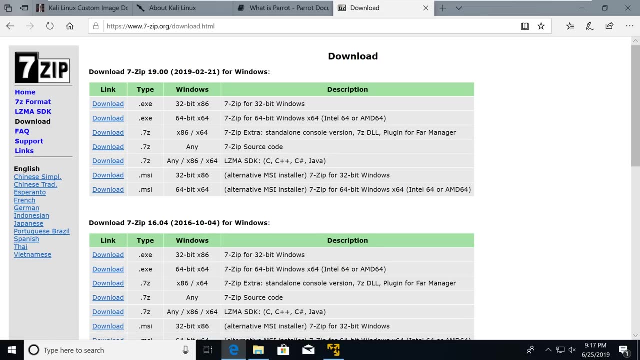 So if you go out to Google and you just type in seven zip, the first thing that comes up is seven dash zip dot org. you'll see a download tab here. just go ahead and click on that link And go ahead and download the executable for your respective operating system. So for me, i'm going to 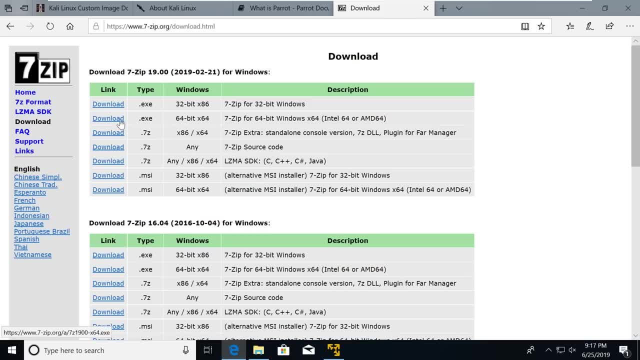 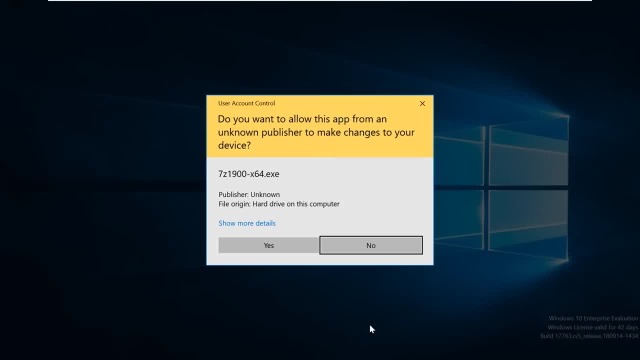 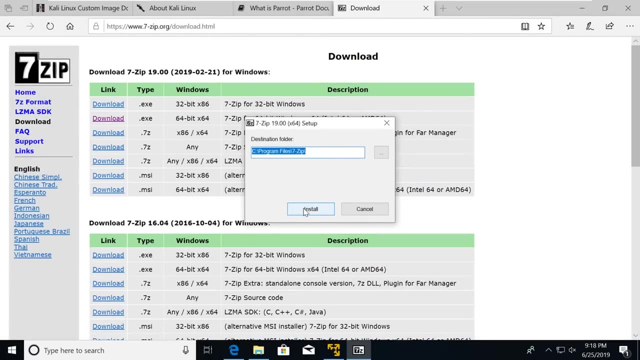 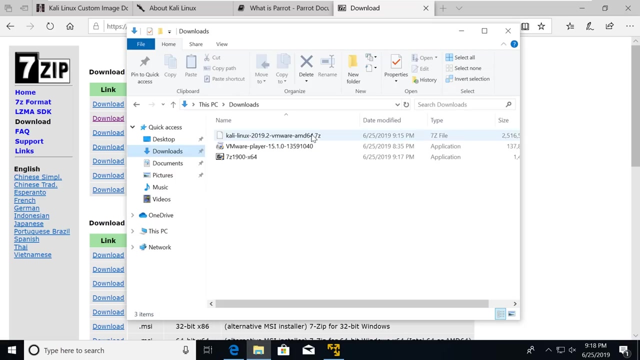 be downloading the 64 bit Windows version here And I'm going to hit save, I'm going to hit run, Say yes, I'm. I'm going to go ahead and install to the default directory. Okay, now that's installed, let's go back to our folder. 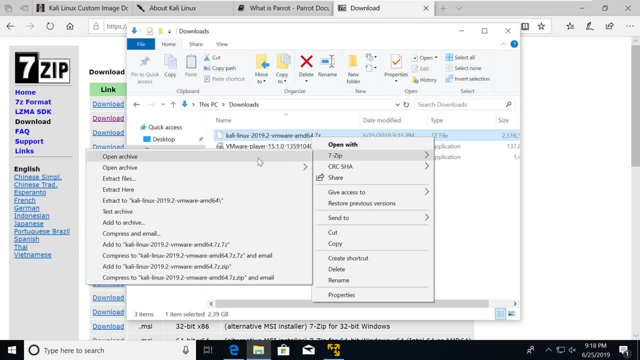 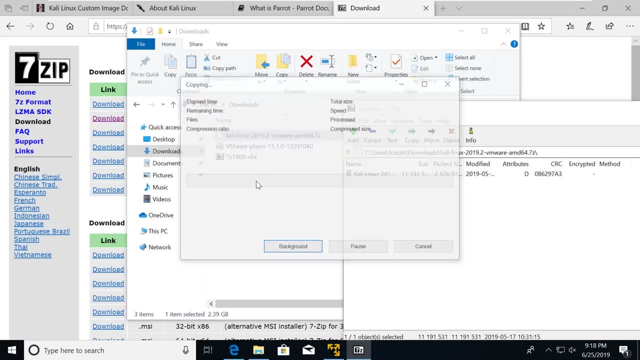 And let's select that we open with seven zip here. Okay, now let's see if we can drag and drop. We can, so all I'm doing is dragging and dropping. I'm putting it in the downloads folder. You don't have to do that. 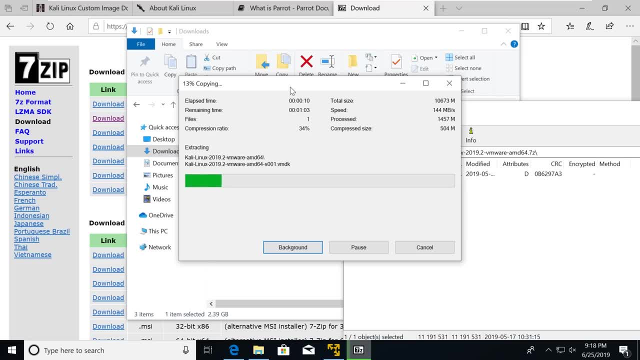 You can drag it and put it in a location that you would prefer. This is going to extract, I believe, at a larger file size than just the 2.5 gigs- that we downloaded the 2.4 gigs, So make sure that you have file space where you're going to put this. 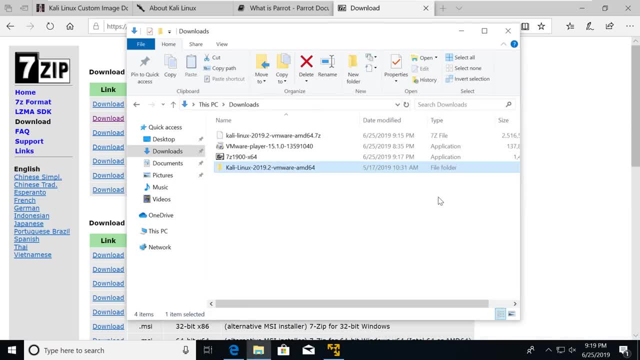 So I'm gonna go ahead and let this finish and then I will be right back. Okay, so I successfully unzipped this file And, just for the record, if we hover over it, you can see that it actually extracted to be 10.4 gigabytes. 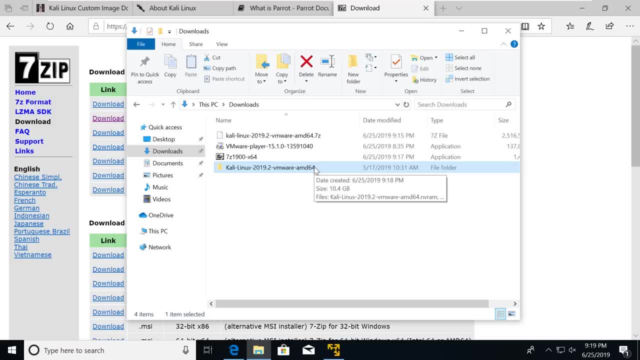 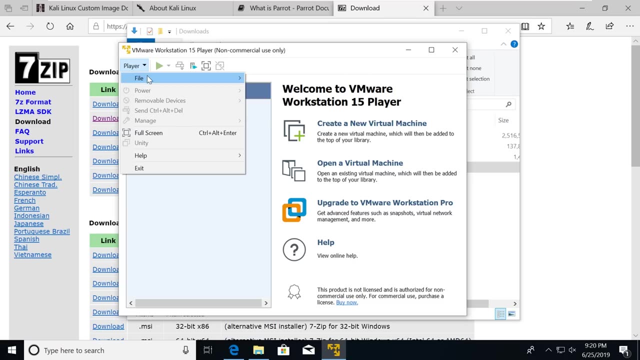 So let's make sure that, wherever you extract it to, you have the 10.4 gigabytes in order to successfully complete the extraction. So, from here, let's go ahead and open up our VMware player, And we're going to go to player up in the left hand corner, we're going to select file. 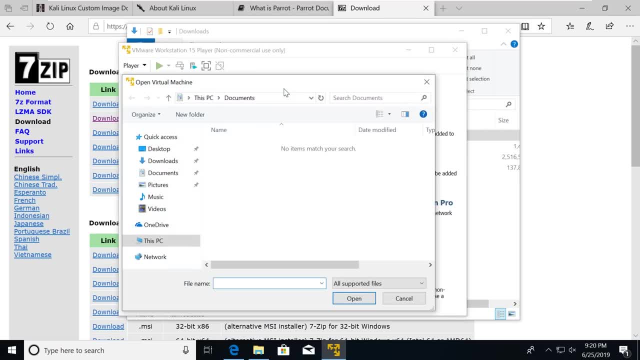 And then we're going to select open And then we're going to go to downloads And we're going to go into our Kali Linux folder here And You put it, if you didn't put it in the downloads folder, and then just select the one item. 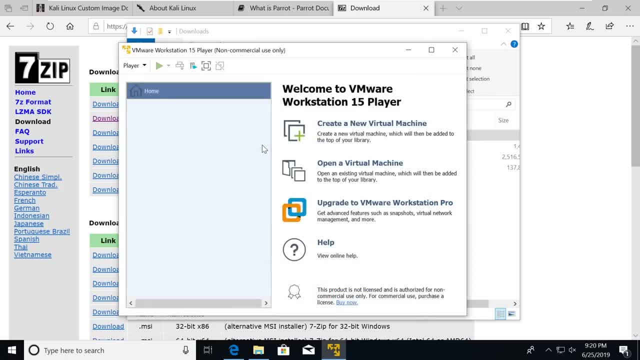 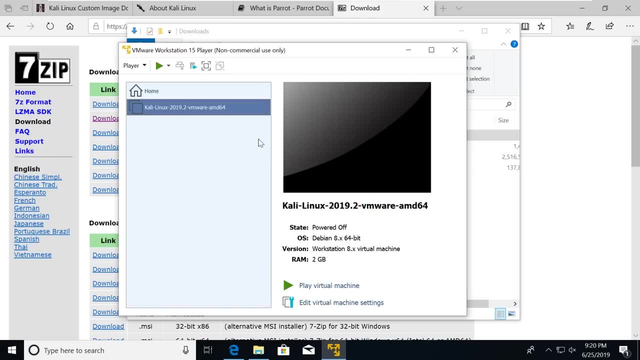 that should be here. It's a little four kilobyte file, And what this does for us is it automatically has a build that's just ready to go. So this is really awesome. We don't have to download the image itself and then install it and then pick all the 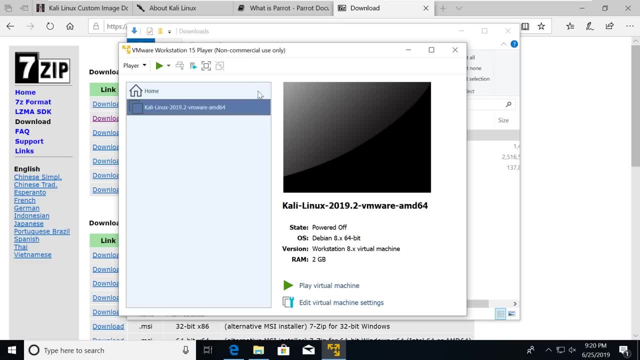 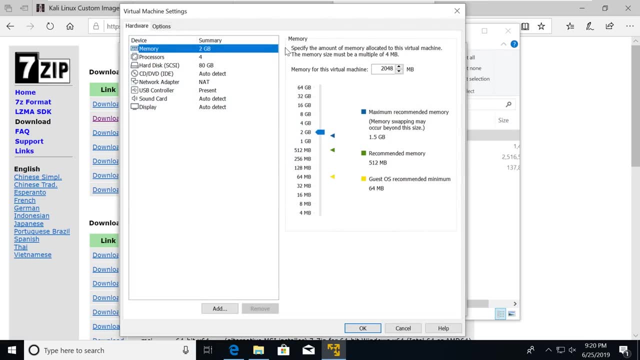 features. No, this is just ready to go for us, So we can also come down here and select, edit virtual machine settings And there are a couple features here, So depending on the amount of memory that you have on your machine. so right now, this: 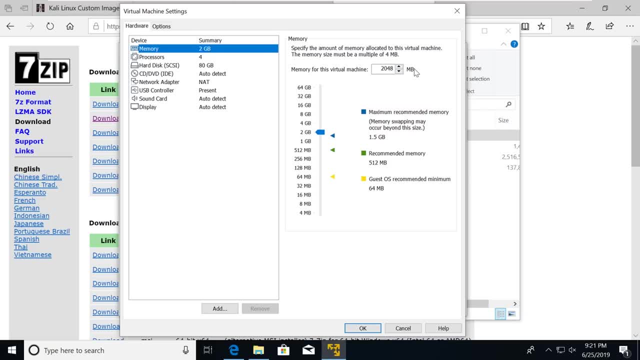 is sitting at two gigs of RAM. that's fine. If you want it to run faster, I recommend going somewhere between four and eight. Obviously, the more RAM you give it, the better it's going to perform, But if you're running on eight gigs of RAM for your machine really not going to do well. 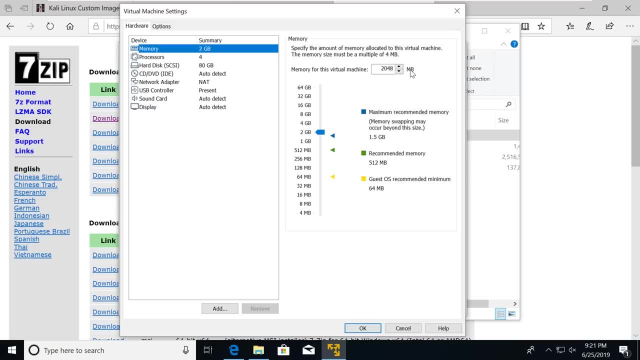 for you. Okay, So the configuration is no more than a fourth. So if you're running on 16, then maybe give this four. you could really try pushing it up to eight, But I am running on 32 right now, So I could crank this up to eight by my role here. 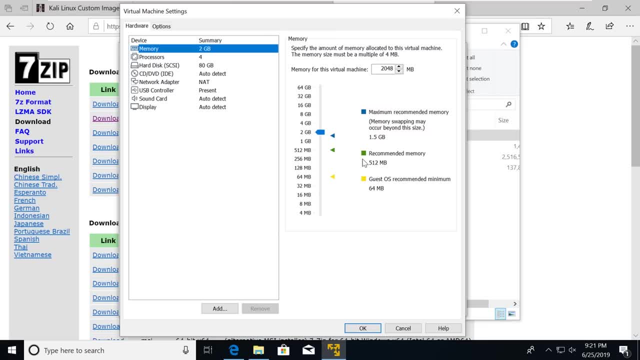 But just for working with you and following along, I'm going to set this to two, and then we're going to perform into that way that we are working at the same speeds across the board. Another thing that we need to know is the network adapter. 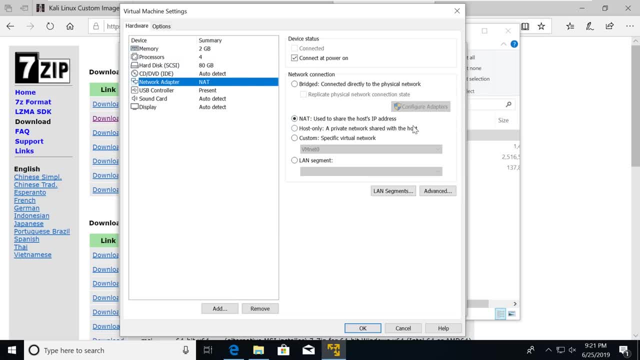 By default It's set to NAT. We're going to go ahead and just leave it at NAT here. Yours may come set to bridge. if for some reason it's set to bridge, You can try that, But my default preference is NAT. 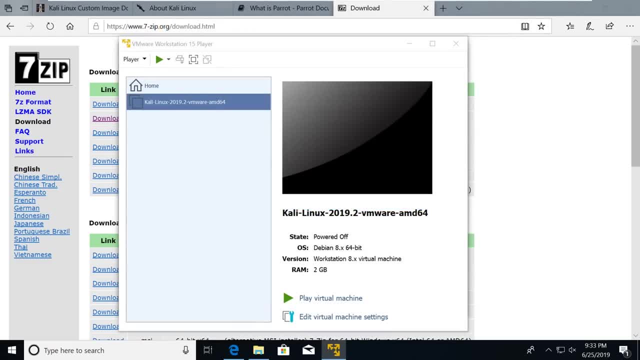 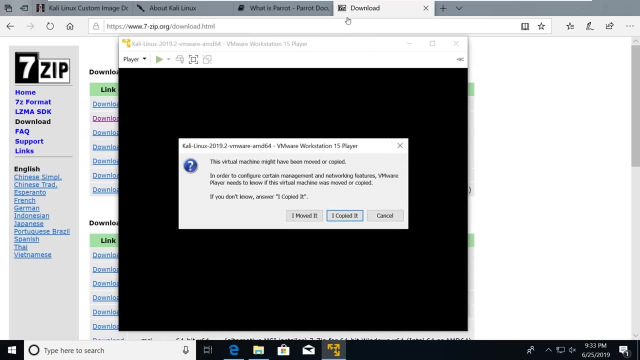 So let's go ahead and just hit okay, Okay, and now we're just going to hit play virtual machine. And a little side note: I am actually now on my OS. I'm running on my, my Windows OS, as opposed to just running inside the VM. if I was running a VM inside of the VM, I would 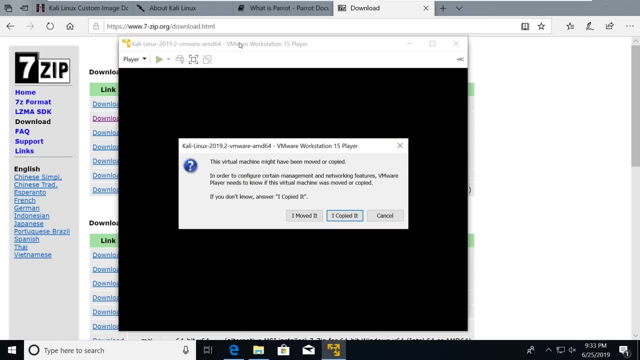 have a lot of issues: degradation, etc. So now I've actually moved out of the VM and have this running in player on my Windows OS. Okay, and then when we get this pop up here, go ahead and just say I copied it. 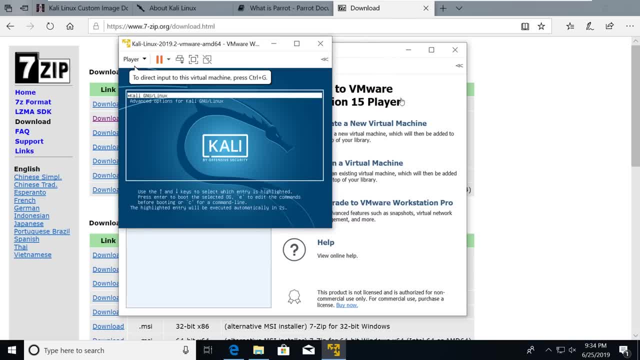 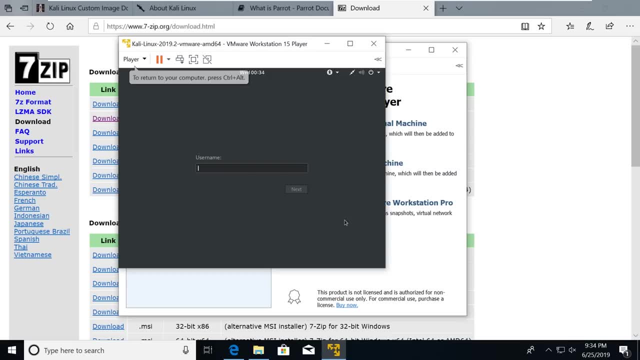 And this will start the machine And you can see the other VMware player back here. it's going to go ahead and directly just start loading up here and we get to this screen, So we click in And if we try to just update it, 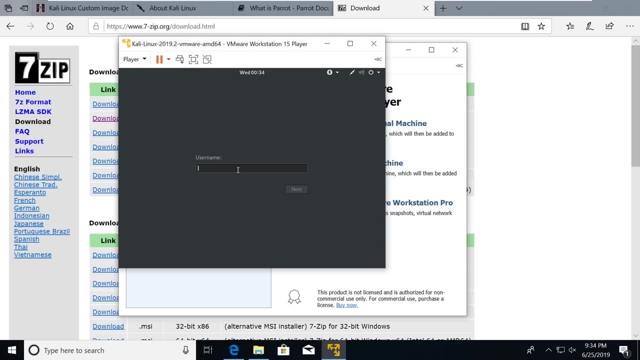 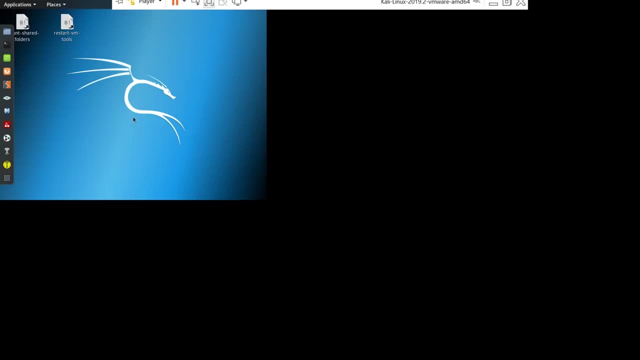 Okay, Just enter in our username and password. Our username, by default, is going to be root. Our password is going to be root backwards. So t o o r, and then hit enter. Now we can make this full screen over here by clicking this button. 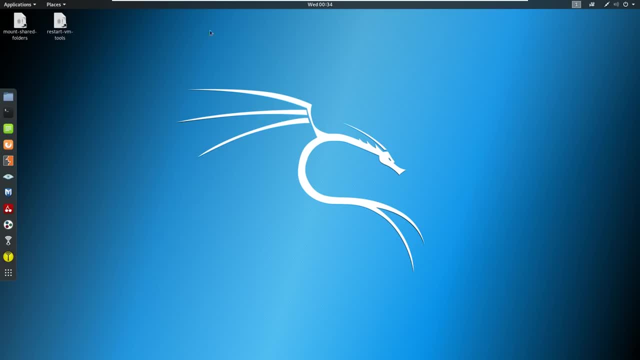 And we'll enter into full screen mode. We are now successfully logged into our Kali Linux machine, We've installed this successfully and now we are ready to start learning. So that's it for this video. In the next video, what we're going to be doing is we're going to cover some of the 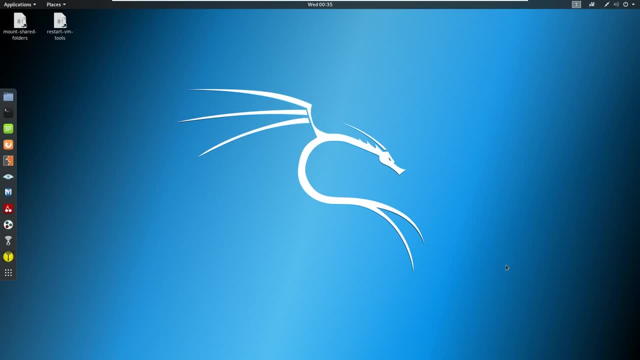 tools and features of Kali Linux And we'll start talking about what it's capable of. And then we'll dive right into the terminal after that and start learning some- So command line and some useful tools with Linux. So I will catch you guys in the next video. 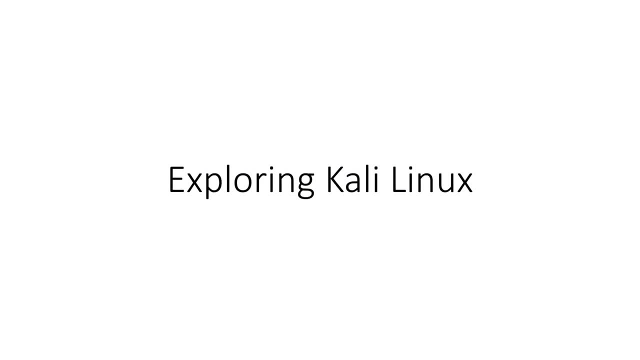 All right, now let's take a look around Kali Linux and just see what it has to offer us In terms of tools, design, etc. So let's dive right in. Okay, so we're at our desktop here inside of Kali Linux. 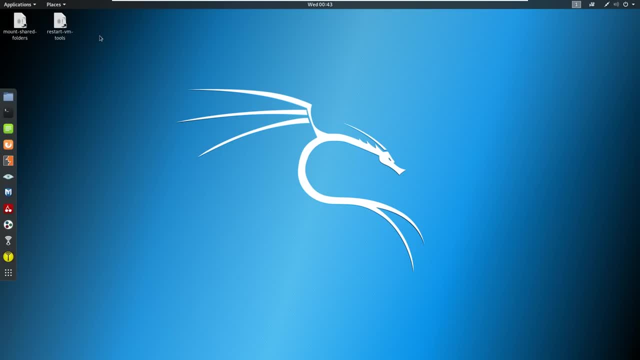 Now you see the Kali Linux logo. you see there's a couple of things on the desktop. you don't have to worry about these. These are just from VMware themselves put on your desktop. If you install this as an actual OS, this will not be here. 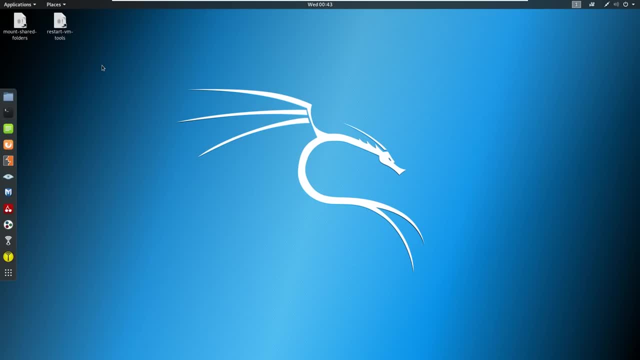 So when we talk about navigating around Kali Linux, There's a couple of things, There's a couple of places that we can look. If we look right away, you can see on the left hand side over here we've got a favorites. 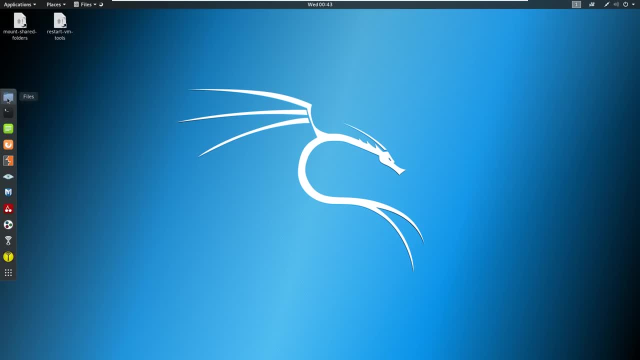 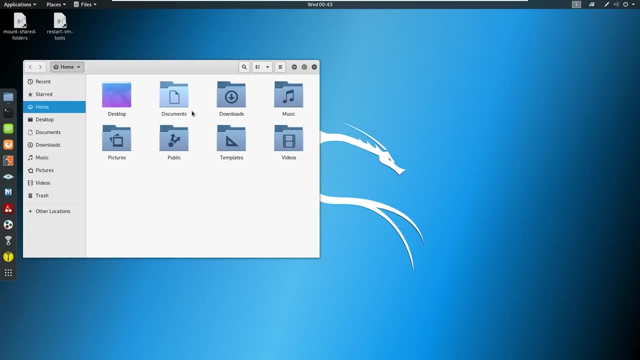 bar. So we've got our folders. So if we click on the folders or our files, we can navigate around. this feels like any other machine. right, We have our documents, downloads, music, pictures. if you're a Windows user or Mac user, whatever, 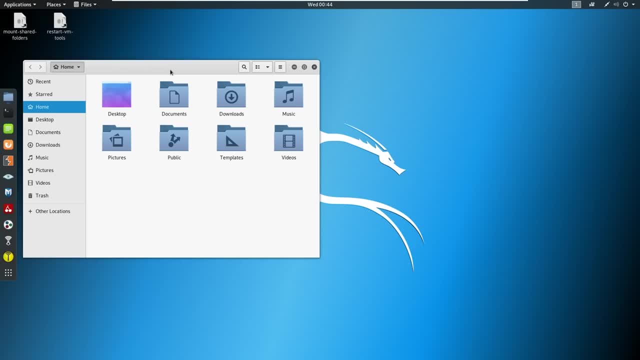 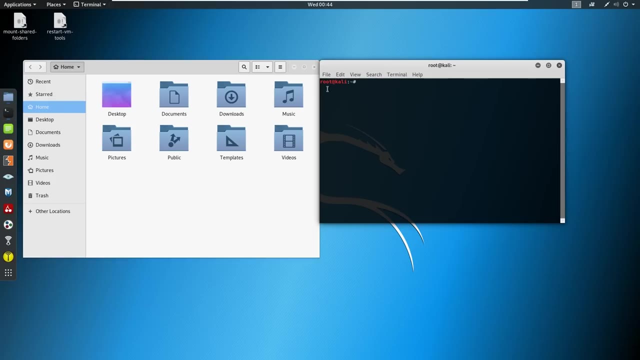 this feels pretty common. So this is a GUI or graphical user interface way of interacting With the folders. as you move on and we move on in this course, we're going to be living in the terminal, So the terminal is right here. If you click on the terminal, this is something similar to your command line. 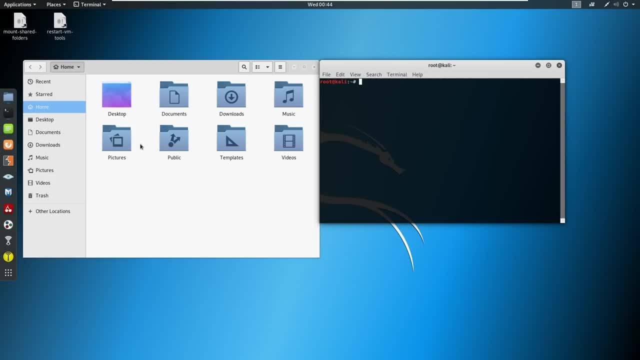 So from here we can actually navigate to all these folders here and we can put files in there, take files out. anything that we can do in a graphic point of view we can also do from this command line point of view as well. 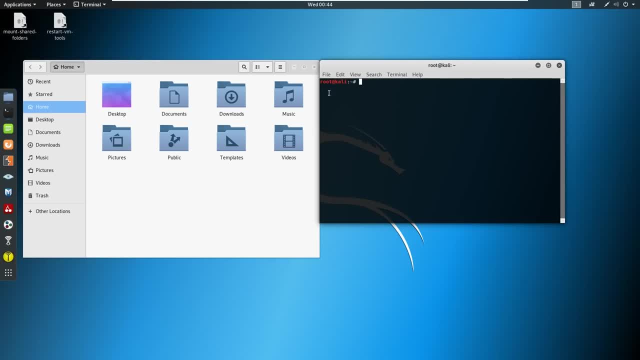 So, as we learn, We're going to get a little less relying on the graphical interface and more on the terminal side of things. However, do know that there are ways to do a lot of things from a graphical side if you still need that, that interaction with the machine, and you don't want to be completely 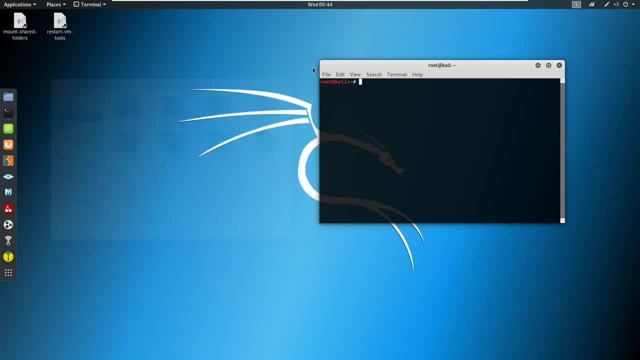 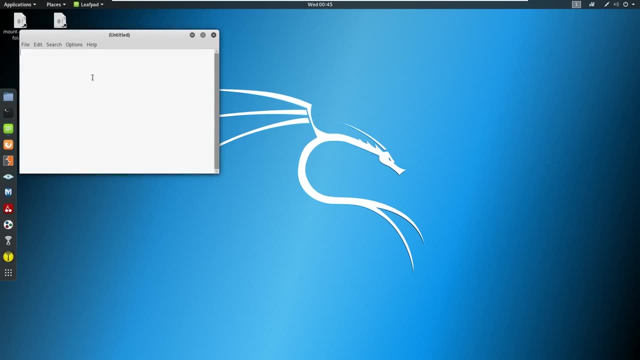 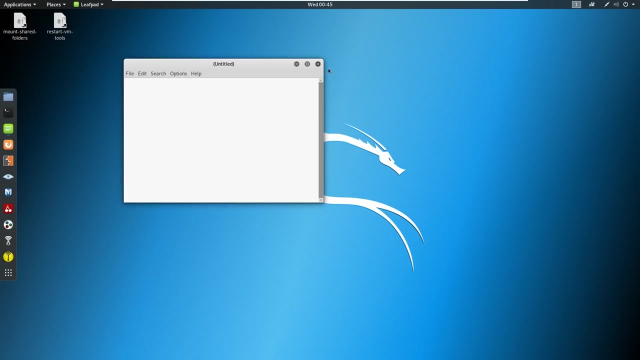 keyboard oriented. There are also tools on the side over here. If we look, we've got a leaf pad. So leaf pad is just like a notepad, right, Or, you know, a keyboard. So just your notebook. here you can take some quick notes, save it out, should be pretty. 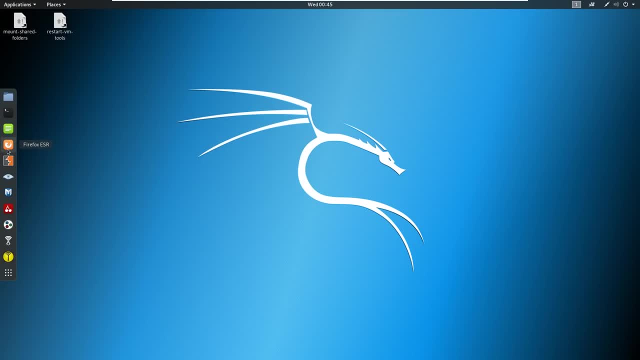 familiar for you as well. So they've got Firefox. it used to be called ice weasel, And that's just your web browser. Down here are some of the tools that you may use Now. burp suite is a very popular tool for web application penetration testing. 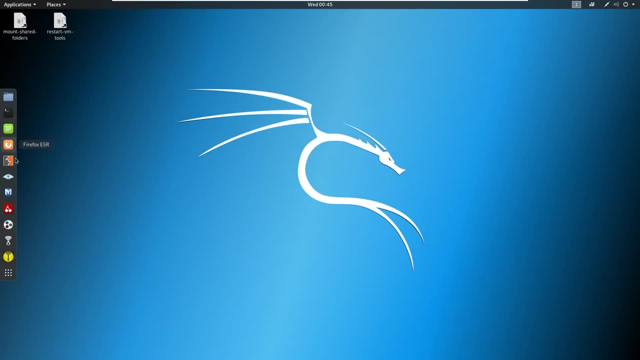 We're not gonna be getting into any of these tools at the moment, But I will cover what a couple of them do. So again, burp suite: It's a web application penetration testing tool. If you ever get into web app, or if you even get into some basic pen testing, chances are. 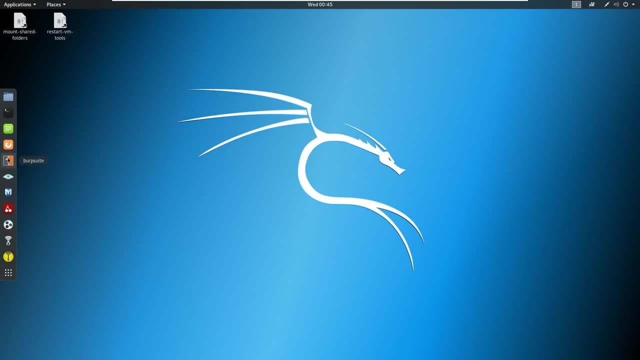 you're going to start using burp suite on a pretty regular basis. Over here is Zen map. Now this is the graphical version of a tool called n map, And you will be using n map pretty religiously when you're doing pen testing. 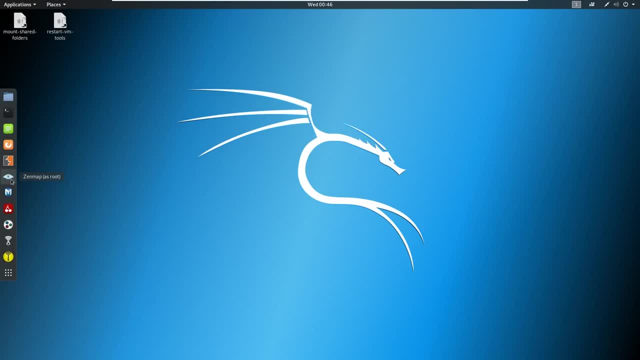 So if you like a visual view of doing scanning, so n map is a network mapper. It allows you to scan machines for open ports and for vulnerabilities. So if you want that in a more of a visual type of view, a graphical interface type view, 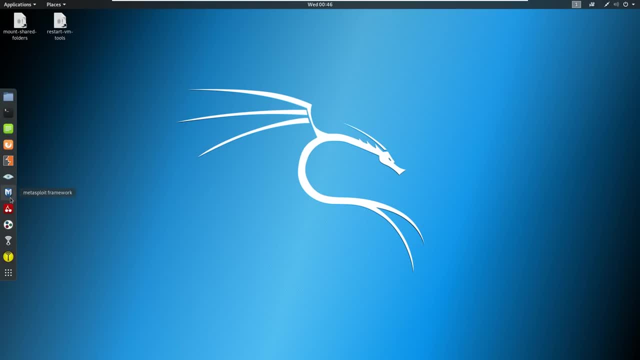 then you have Zen map as a feature. This little guy down here is Metasploit. Now, Metasploit is a tool that can be taught. all these are tools that can be taught in deep, deep lessons all by themselves, not to make that intimidating for you at all. 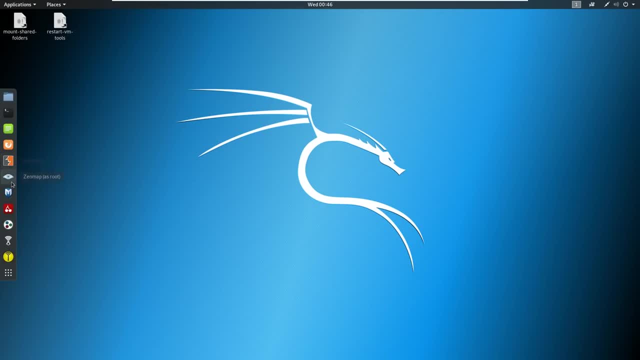 It's how robust this is. we're looking at three tools right here And they're all very, very powerful, And this isn't even the half of it, or the quarter of what Kali Linux has to offer. So Metasploit- you may have heard of it. 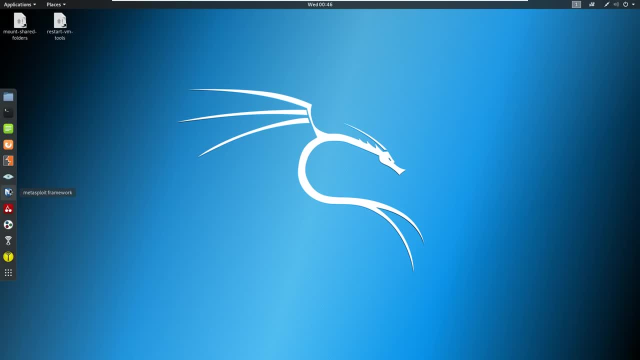 If you've heard of anything in pen testing, it is a framework that does just a little bit of everything, So a lot of pen testers live and die by this. It's a fantastic tool, in my opinion, And you're going to get very, very intimate with it very, very quick. 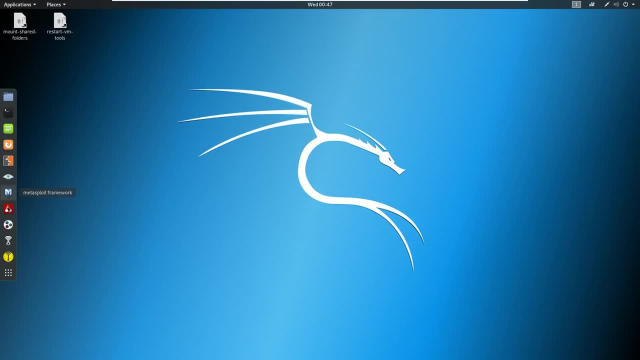 If you do move into pen testing. Down here is a tool called cherry tree, And that's pretty much where I'm going to stop. We've got Maltego in Kismet. These are just. this is wireless base And this one here is is information gallery base, but cherry trees another useful one. 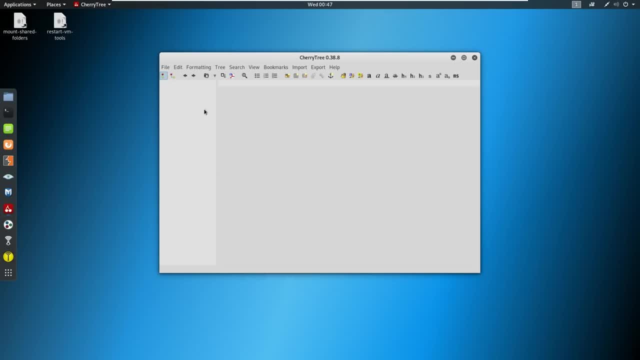 If we open that up, this is actually another note keeping tool, like I showed you. leaf pad- leaf pads just for quick little one offs Cherry tree is more of Note keeping as a whole. So you've got nodes that you can add. so you can add a node here and just say: say you're. 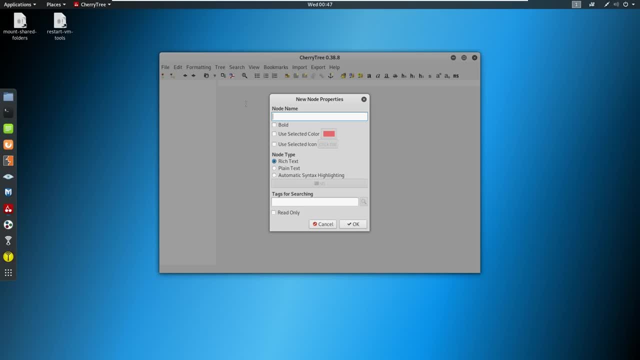 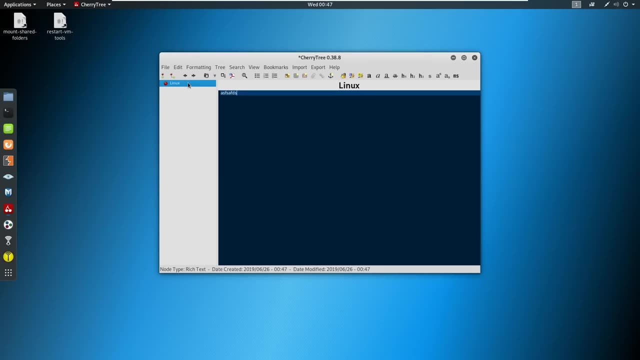 following along and you want to add notes. You can say Linux, you know, and then you have a node. You can add all of your notes in here And then you can actually add children nodes as well. So maybe there's a command that you want to add in. 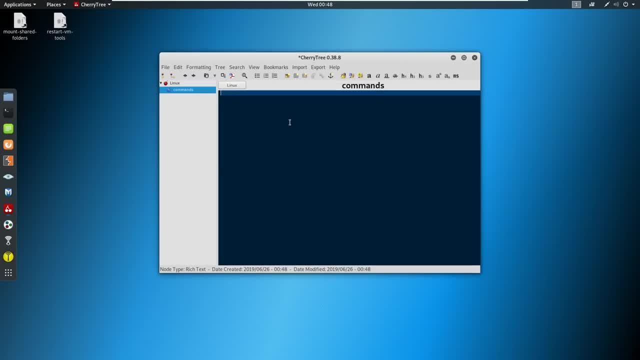 So say, we're covering commands and you want to write all the commands in about Linux down here. You can do that as well And then save this out. Nice thing too is that you can take screenshots and put them in here and exports- really nice. 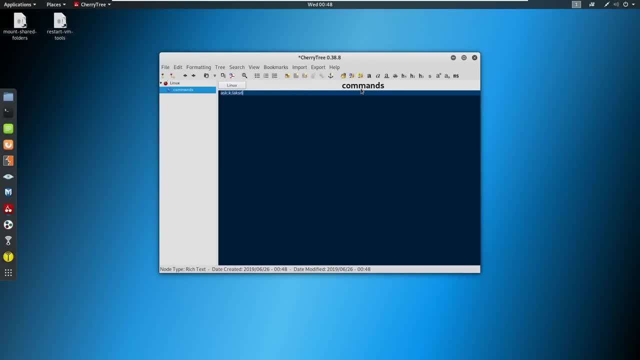 And this is going to be very, very useful for anything in your career. But when it comes to pen testing, there are so many tools, so many commands that I think it is incredibly important to be able to take notes, and cherry tree is built in already. 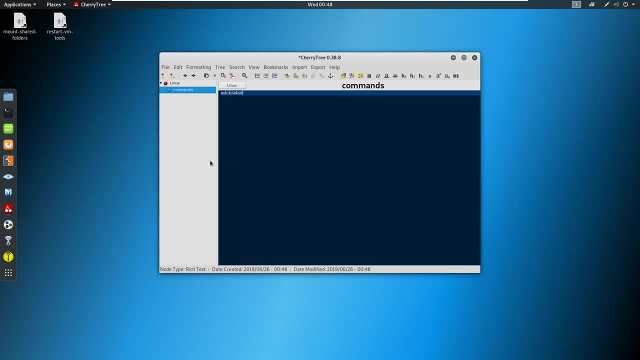 Personally, I use what used to be in Kali Linux, which is a tool called Keep note, but cherry tree is a great alternative as well, So either of them would work, and I is highly recommended by me that you use some sort of. 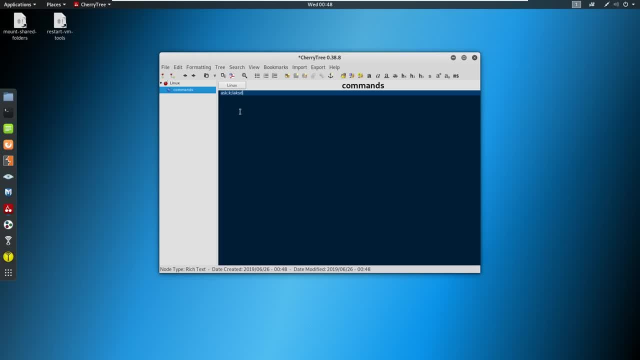 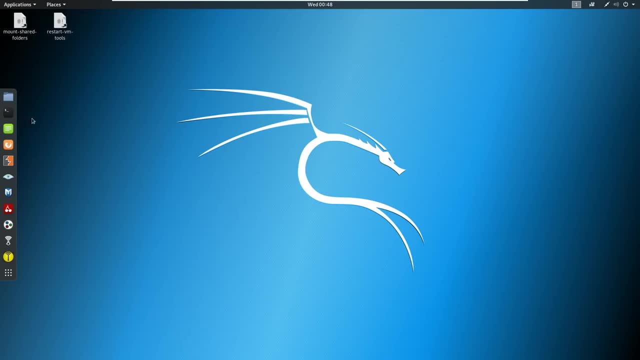 note keeping tool as you go through your courses and get better as a pen tester. So I'm going to close out of this here And I want to show you a couple more things. you have a feature here where you can show all of your applications. 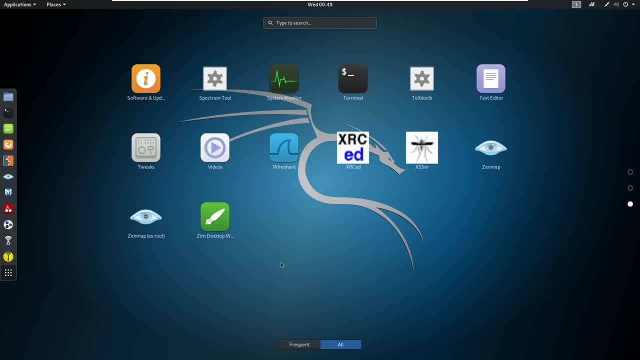 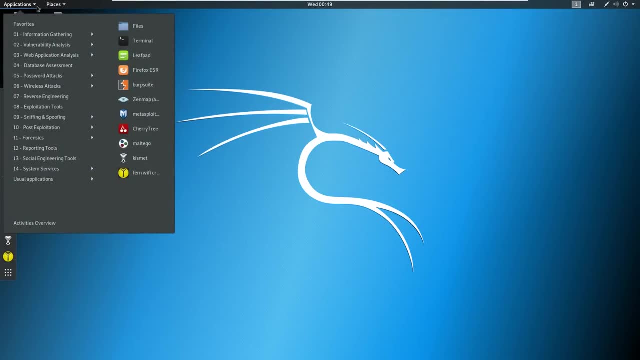 So if you click on that, it'll bring up all the applications, including the ones that are grouped down here. Another way to do this is if we come up into applications at the top, you can see that everything is grouped. really nice for you. 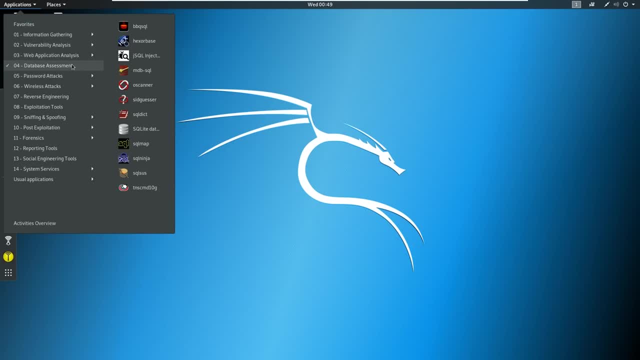 So it goes through the steps of penetration testing And let's say that like, hey, I'm gathering information on a client, Okay, well, here are some of the built in tools for information gathering right here, Say, you want to do a wireless assessment and you want to do that? those sorts of attacks. 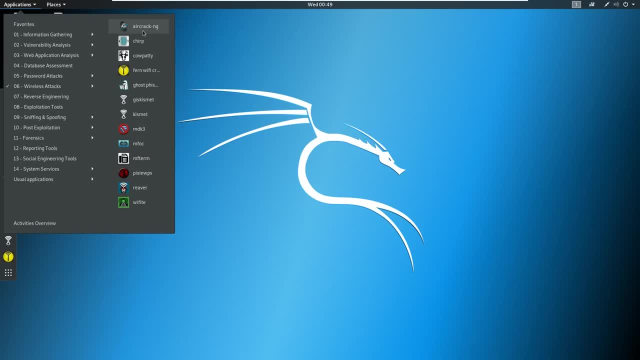 you've got all these wireless tools in for you right here. Now. chances are you're going to be running these tools from the command line. So again, you know you don't want to get too hung up on the graphical side of things. 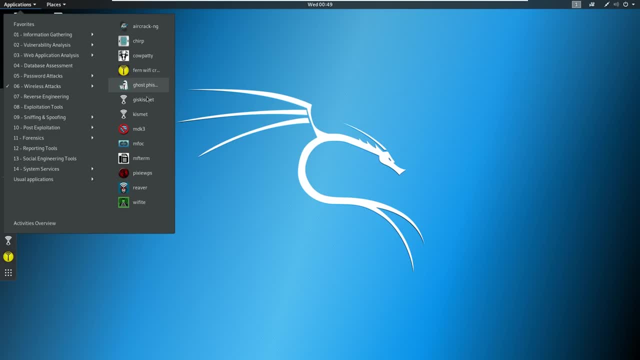 As you may not always have access to that either, But it's important to know what tools that you have in front of you, And there are even tools like Wireshark in here, So that very, very useful. pretty much a little bit of everything that you can imagine. 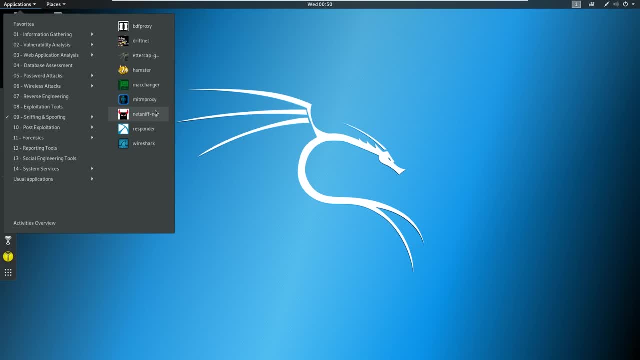 So, just you know, take some time and go through the tools And if you're becoming a pen tester, you're working on it. you know, just just you know. look at a tool and do some research on it. 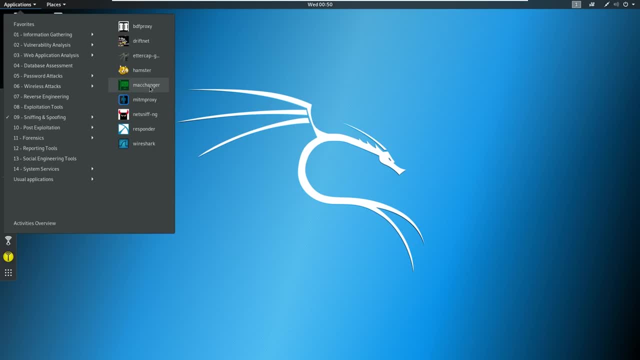 Say you want to know what this Mac changer is. it might be obvious. it might not be obvious, right? So maybe you go Google what Mac changer does, how to use it, what the syntax is, and then you play around with that. 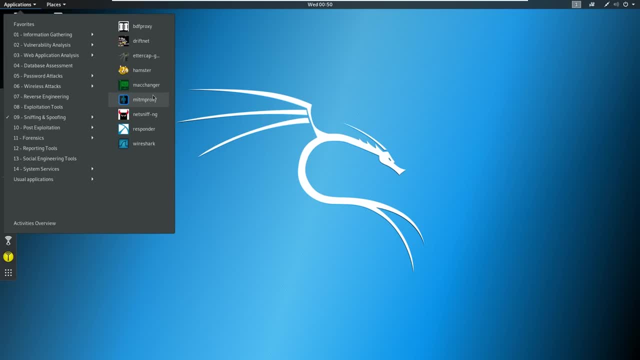 Pick a new tool every day, figure out something that you can do with it, how to use it, what it does. But so Kali Linux is a distribution full of useful tools And it- it, you know, for a base OS. it's fantastic. 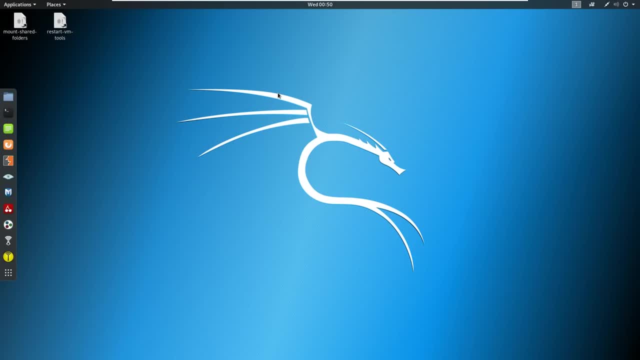 And this is why so many people in the industry just download this, install it and they're ready to go. You know we talked about in a previous video how there are other OS's or there are people out there that like to just do their their base install. 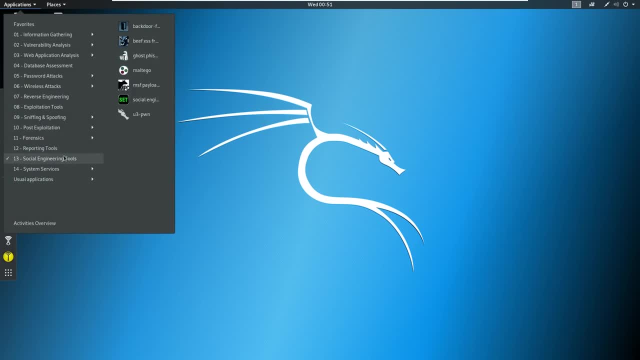 And you can see that there's bloatware here, if you want to call it that- right, like there's forensic tools and maybe you'll never do any forensics in your life and you don't need all this installed in your system. 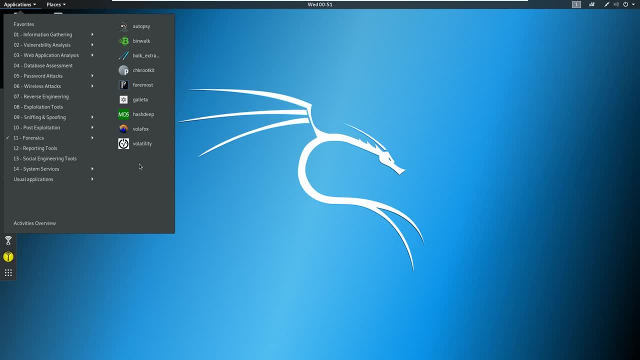 So if you're a type of person that is, you know it doesn't want this extra stuff, this extra software on your system, okay then maybe you do start moving towards that custom build eventually in your career you say, Hey, I want, I want to learn all these things. 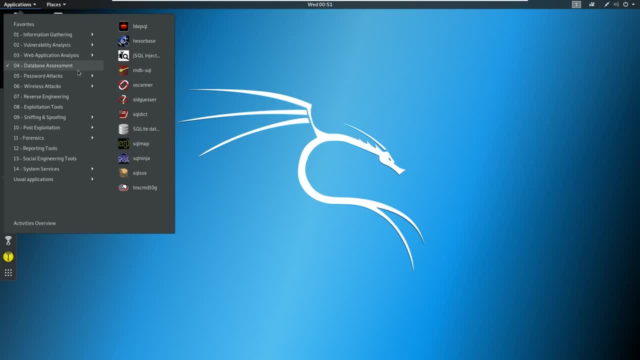 first And then, once I learned what tools I really like, then maybe you move to your own distribution that you create yourself And you spin that up every time, instead of having all these tools built in, But as a base OS, as something that you can learn from and start with. this is why I've 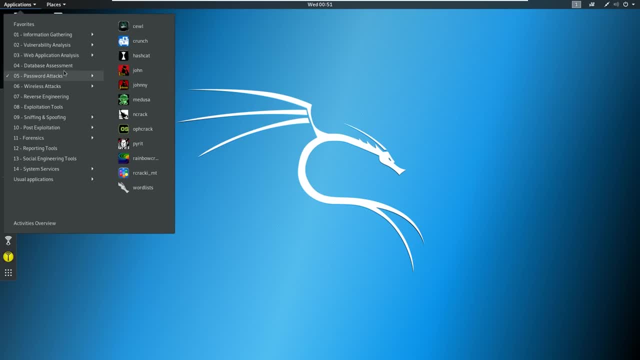 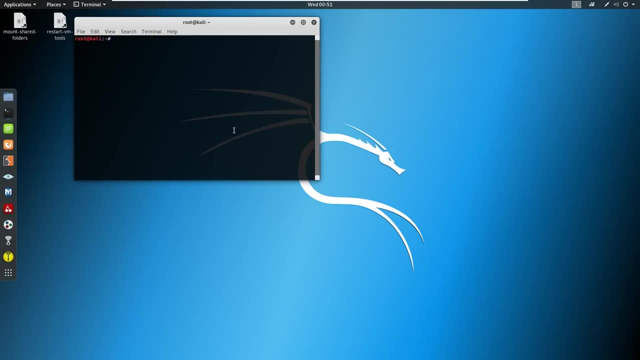 chosen Kali, And this is why we're going to learn it today. So let's go ahead From here. what we're going to do is we're going to dive right into the terminal. So let's just open this terminal And then we're going to full screen it and move on to the next video. 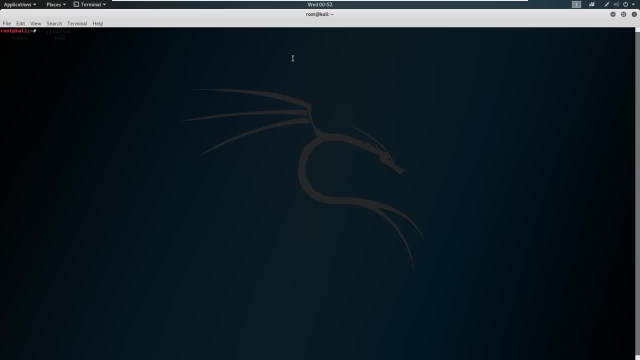 So, from here on out, what we're going to be doing is we're going to be living in this terminal. Um, we're going to back away from the graphical side of things and really just uh, get your your hands dirty in the terminal. make you feel comfortable. 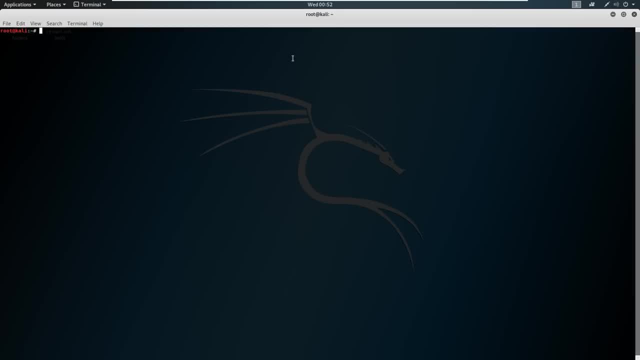 If you've never used Linux before, this is perfect for you. So I'm going to give you the the pen tester perspective on why we're doing a lot of these things. Uh, some of these commands are going to be the same commands regardless. if it's uh. 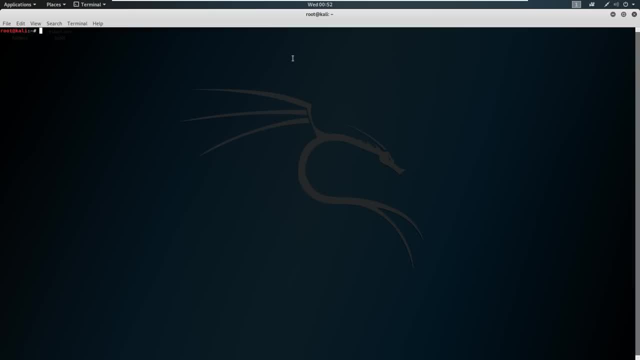 on a Kali Linux machine or if it's on a another distribution of Linux. So you'll be able to take a lot of these commands And just use Linux and another system as well. So if you're interested in pen testing, if you're interested in Linux, this is where. 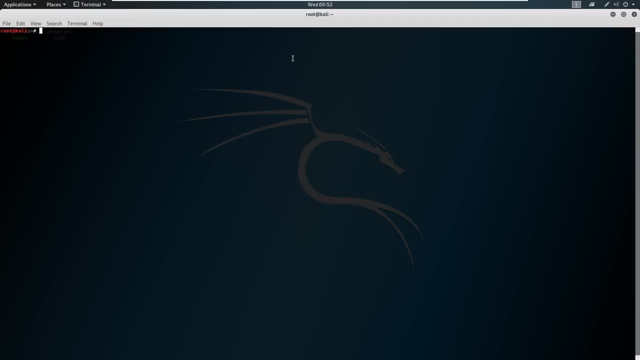 we really get into the meat of the course and it should get interesting for you. So I will catch you over the next video when we're going to start talking about how to navigate the file system and get comfortable with that. All right on to navigating the file system. 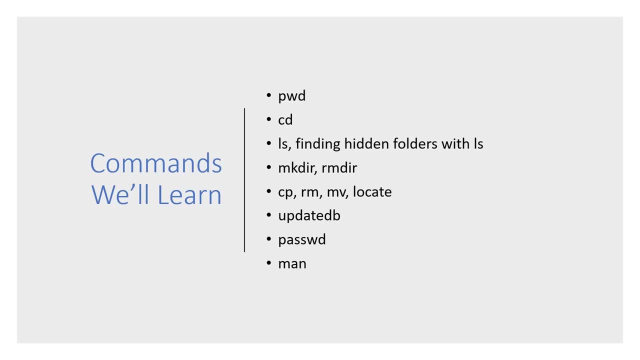 So first let's talk about some of the commands we're going to learn today. So we're going to learn about PWD, which is present, Which is present working directory. We're going to learn about CD, which is how we change directories. 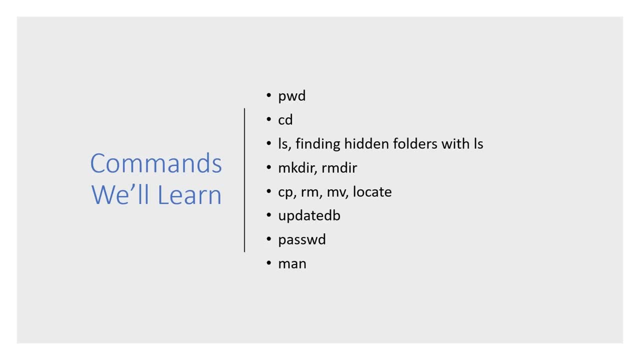 We're going to learn about LS, which is going to be listing the files in a folder or in a directory, And we're also going to talk about how to find some hidden folders with LS. We'll talk about how to make a directory and to remove a directory. 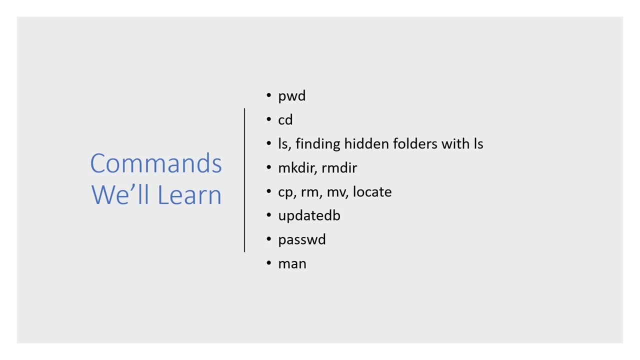 We're going to talk about copying, removing, moving and locating files. We'll talk about something called updateDVD And how that pertains to locating files. We'll talk about the password and how to change our password, And we'll talk about an important command called man. 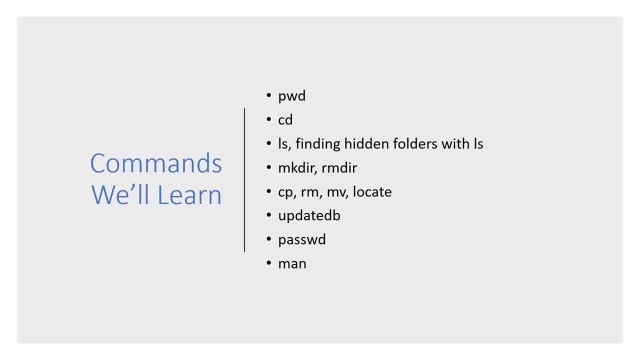 So by the end of this first lesson you should be pretty comfortable with all of these commands. It may seem a little daunting, but they all kind of play in with each other. Again, please make sure to take notes. You've got cherry tree built in. 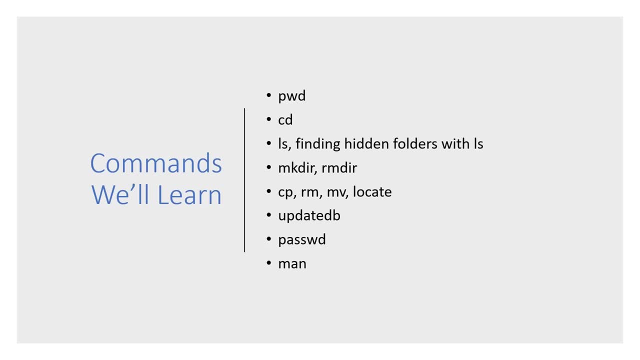 You can also use keep note or even just a notepad in front of you. That'll help with the experience, and also, maybe watching the video more than once will help with the experience as well. So let's go ahead and dive right into the command line. 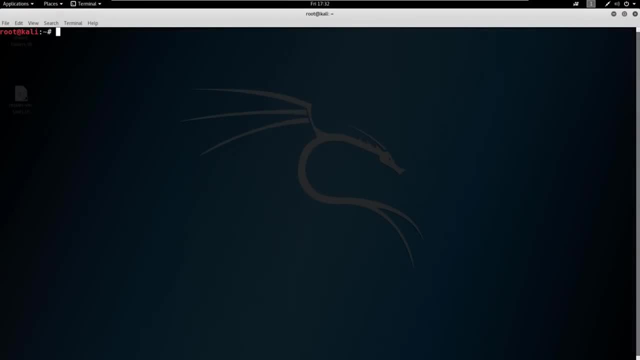 So now our first lesson in Linux terminology is going to be navigating the file system. So if you're a Windows user, you're used to navigating your file system probably through folders, through a GUI, So a graphical user interface. Well, in Linux we can do that. 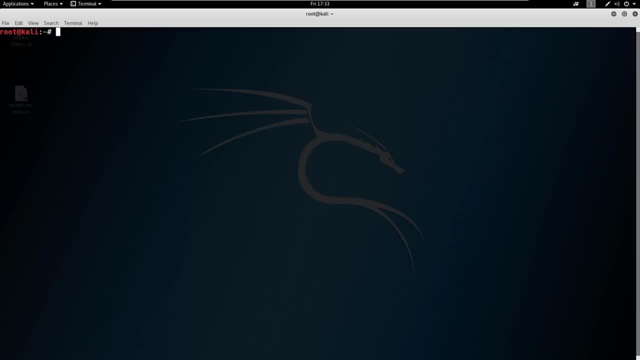 But the majority of time In this terminal here. So we really need to know how to get around. So the first thing we can do here is we can say: Hey, where are we at? And that's PWD. So that stands for present working directory. 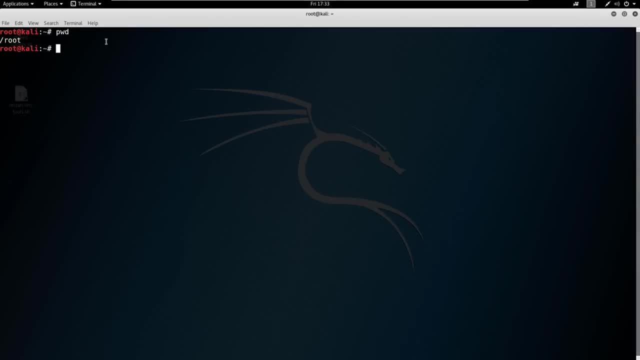 So you type that in, you hit enter and it says: okay, we're in the root folder. So we know that we're in the root folder, but how do we get out of the root folder? We can use a command called CD. 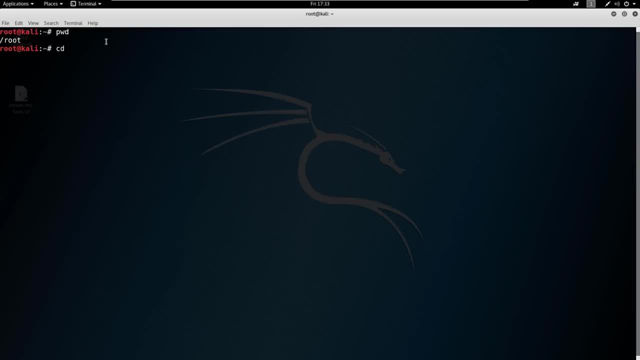 And that stands for change Directory. So if we want to change directory backwards, we just type in two dots here and now we can say, okay, where are we at? So we're in a slash, So we're just in a home folder here or just our generic slash folder, right? 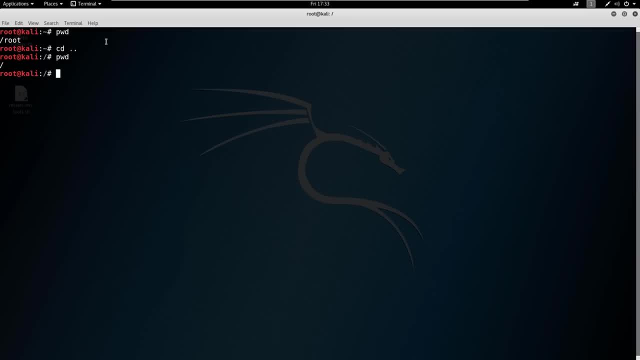 So what we can do is: well, how do we know? can we go backwards from here? Let's keep trying. So we do PWD again? No, we can't. This is our base folder, right? So you have to think of this as the lowest you can go. 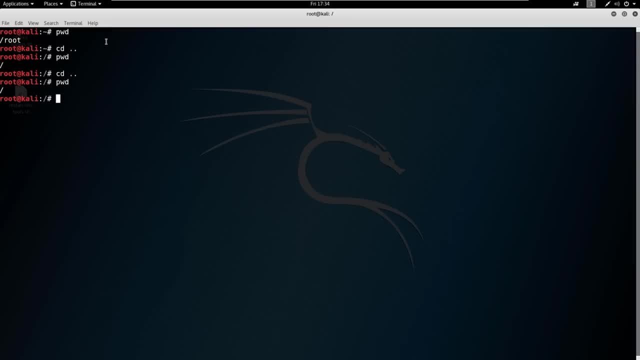 So now, how do we move around? How do we know how to go forwards again? Well, we don't know what's in our directories, right? So we're sitting in this, the slash folder, and how do we look around? So there's a command called LS that lists everything that's in the folder. 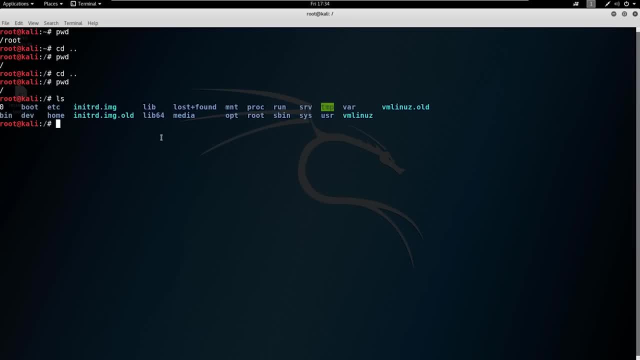 So if we say LS, Okay LS, we kind of see this color coordinated here and the color coordination it just depends on if it's a folder, if the folders read right. You know there's permission settings which we're going to get into later, but the majority 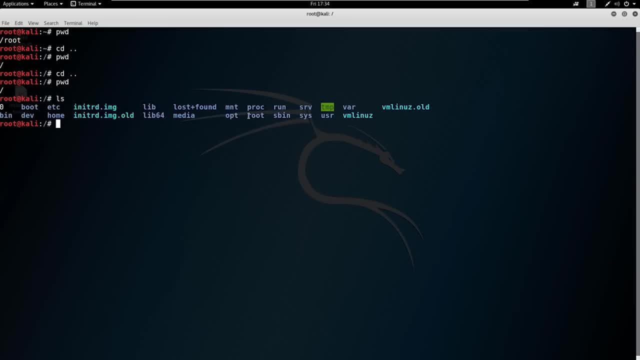 of these here are folders. Okay, Well, we know we just came out of route so we can go back into route. Now, how do we do that So we can say change directory route and we can actually hit tab to auto complete? 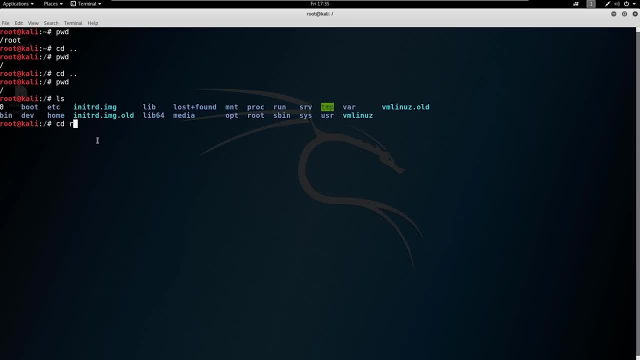 I don't know if you caught that, But there's no. There's not any folder besides route, So at all, I can just hit tab and it should type it out for me. Oh, I lied, There is a run in here somewhere, but it's hidden. 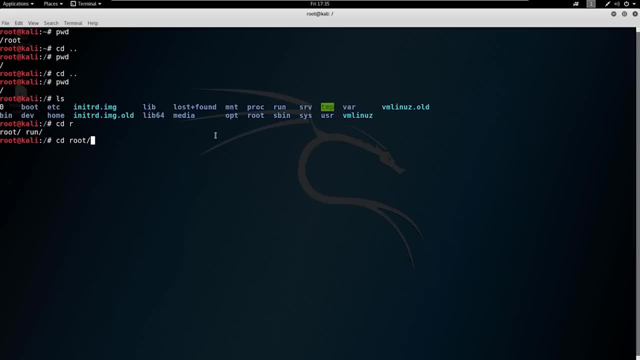 We're going to cover that soon as well. So our oh hit tab auto complete can change directory in the route. So it's LS and route and see what's in here. Okay, This is more like our home folder, right. 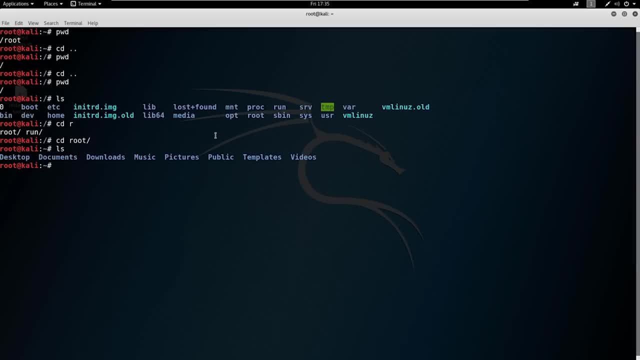 So we've got desktop documents downloads. This is kind of what applies to the root user. So what? What if we're sitting in this root folder here and we wanted to access instead this Etsy folder? Well, can we do the same Etsy command here, while I'm hitting tab and nothing's happening. 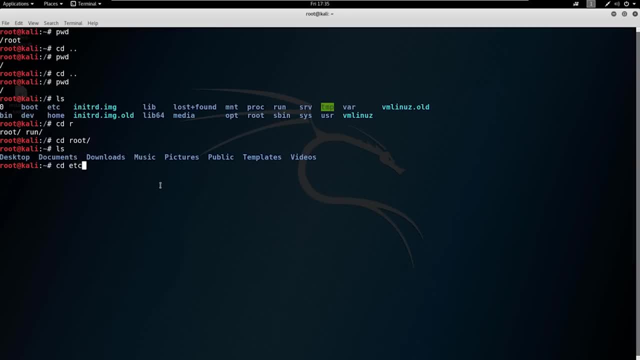 Well, because Etsy doesn't belong in this area, right? But if we put a forward slash in front of it, cause this is the base, and then we hit Etsy there, Now we can navigate to the Etsy folder and we can actually double tab and see what's. 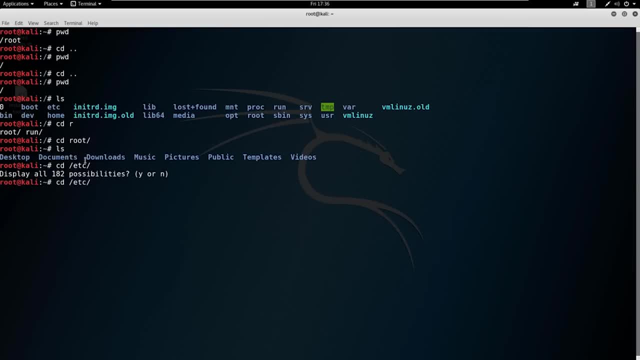 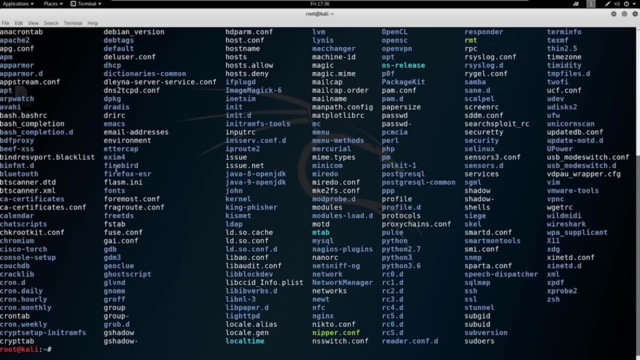 all in the Etsy folder, Like an LS say no. Another way to do that is, if we want it to LS what's in the Etsy folder without navigating to it, we get his type LS Etsy and you can see everything that's in here. 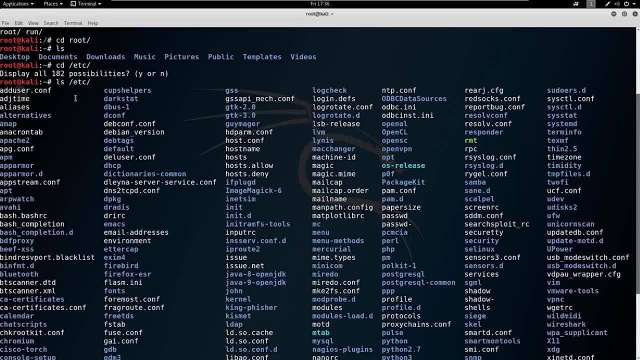 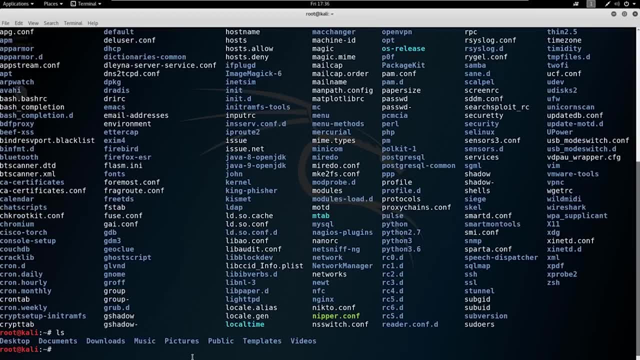 So there's some some tricks that we can do right, So we don't have to actually navigate to the folder to know what's in there. again, If we LS and we want to know what's sitting in videos, or even let's say what's sitting, 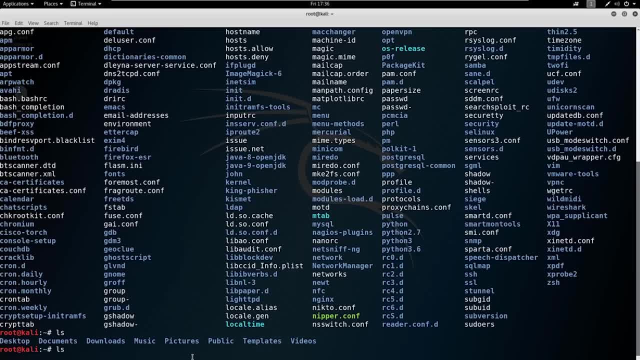 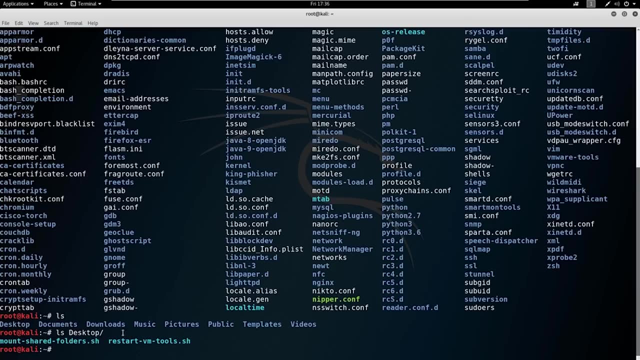 in videos. Okay, What's sitting in desktop for our folder? Well, if we start typing desktop and hit tab, we can't do that either, because everything in Linux is case sensitive. So if we start typing desktop and then hit tab, now we can LS and see what's in there. 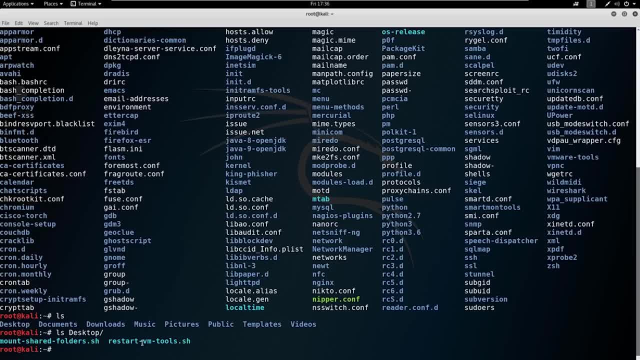 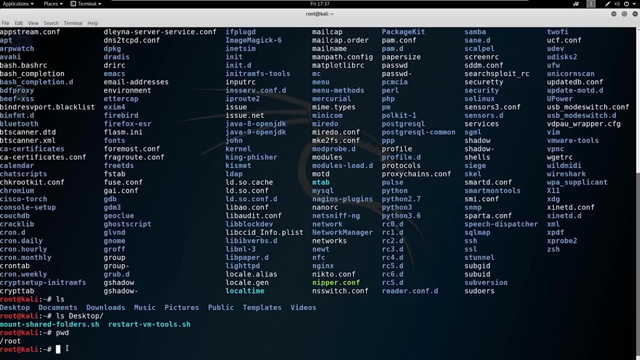 So our VMware came with a couple of shell scripts here that are automatically placed on our desktop. If we wanted to confirm that, you could see that they're both right here. So, as of right now, we are just sitting in our root Home folder and we know how to navigate around. 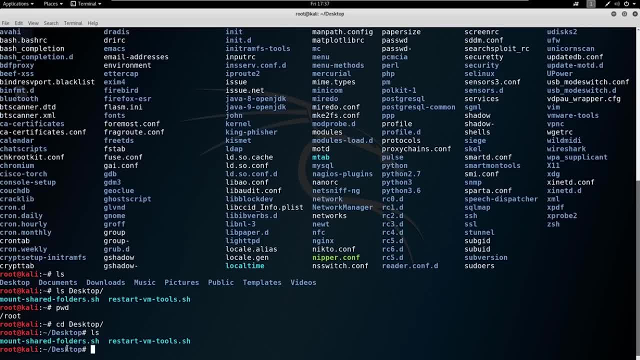 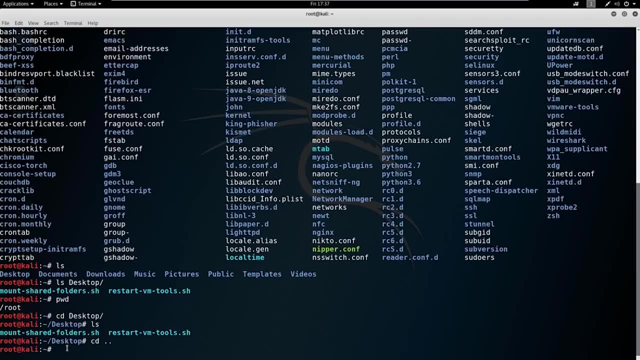 So if we wanted to go to desktop, we could. we could hit LS now and see what's in there. If we wanted to go backwards, we could. okay, now we're back in our, our root folder and you can also tell where you're at. 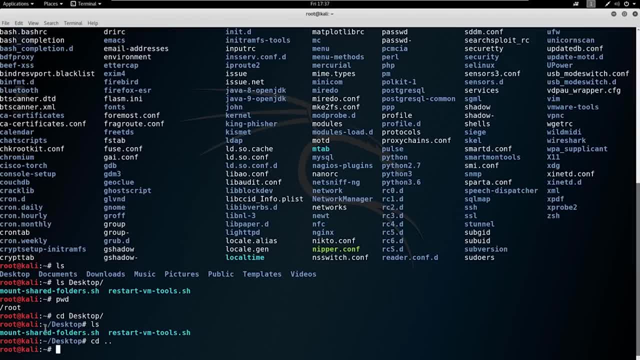 Your present working directory sits right here, right? So this little a tilde is actually your home folder and you can see that we're in desktop. So if we wanted to go back into our desktop Instead of typing- say you wanted to go to music from your desktop instead of going- 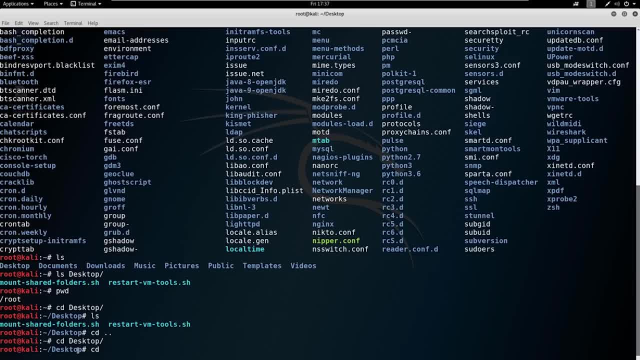 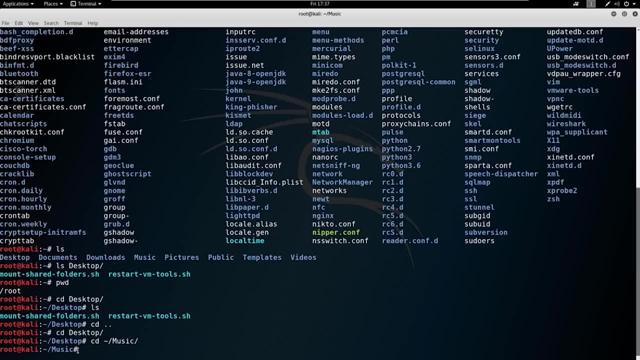 root music, which will work. you could also just say I want to go music, and that'll put you there as well. And notice, you don't need the leading forward slash when you use the tilde. So just some couple interesting tricks that you'll kind of pick up along the way. 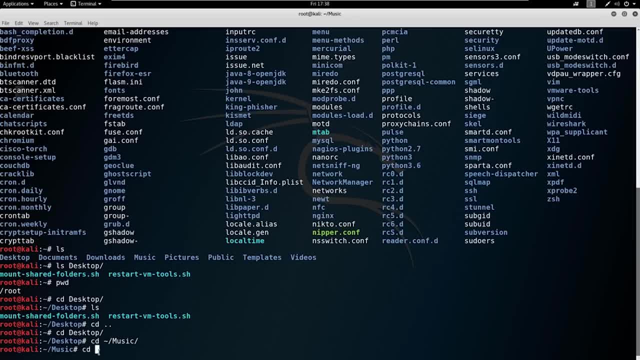 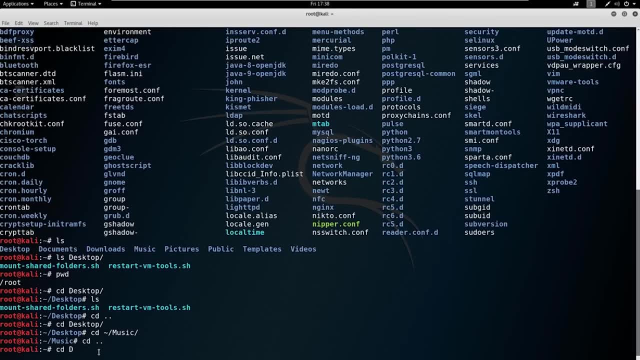 Tab is definitely going to be your best friend. If you run into something with multiple options- Say you're trying to CD and you say I want to go to my desktop and you're tabbing, it's not working- You can hit double tab and then it'll show you: okay, well, there's desktop documents. 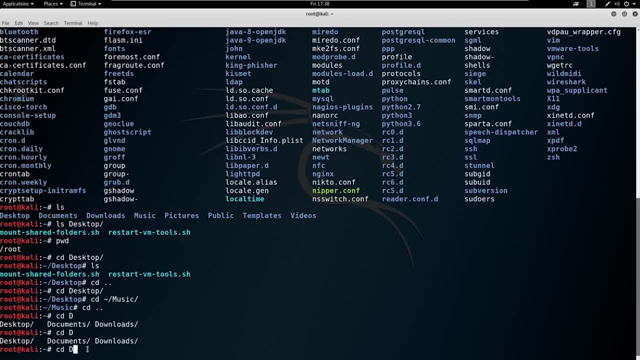 downloads. Those are your three options that start with a, D. So now you kind of have an idea as to how to kind of move around, but let's do a little bit more. So what if we want to make our own folder? Well, there's something called make directory, MKDIR. 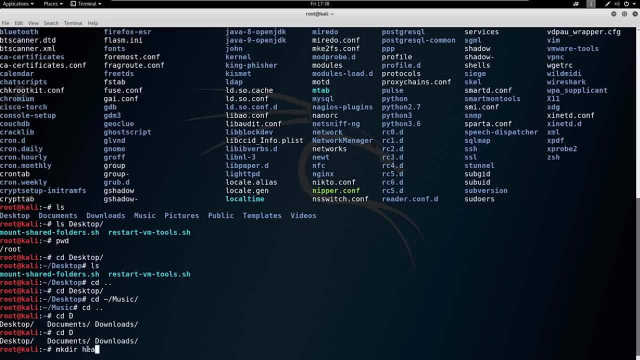 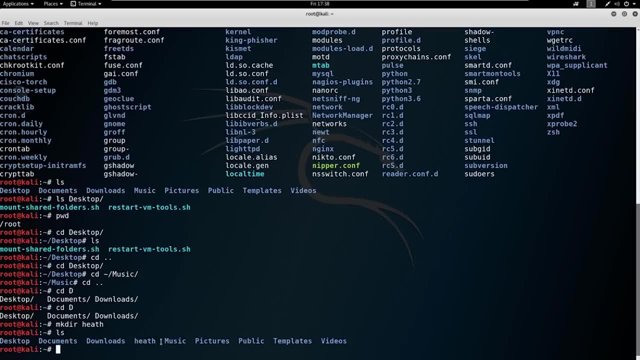 So if we say make directory and we'll say I'm just going to use my name Heath, So now if we LS, we can see that this Heath folder is now here, We can go into the Heath folder and there should be nothing in it, right? 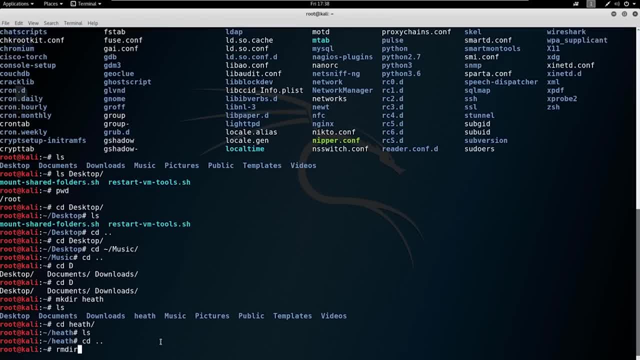 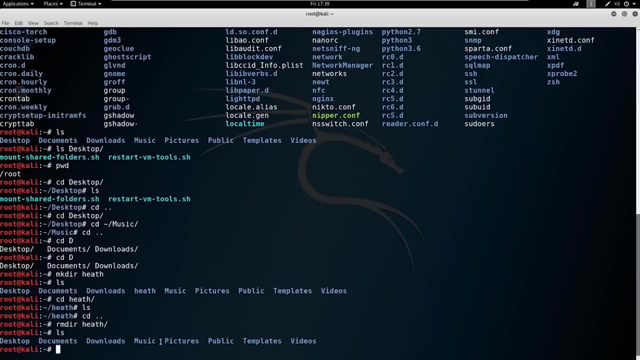 So we can go back and we can also get rid of the Heath folder. remove directory Heath. If we LS again, it's gone. So now, what else can we do? Well, we can also look for hidden folders. So we can say: LS, dash LA, and we can look for hidden files and folders here. 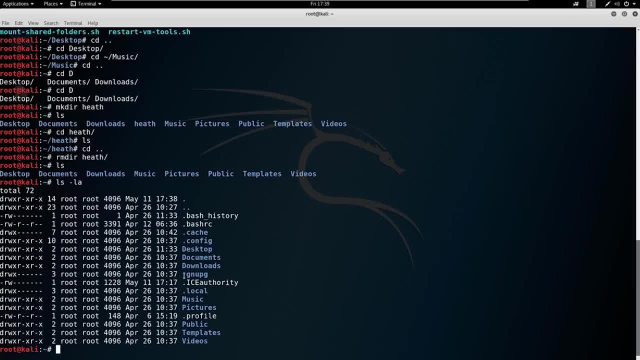 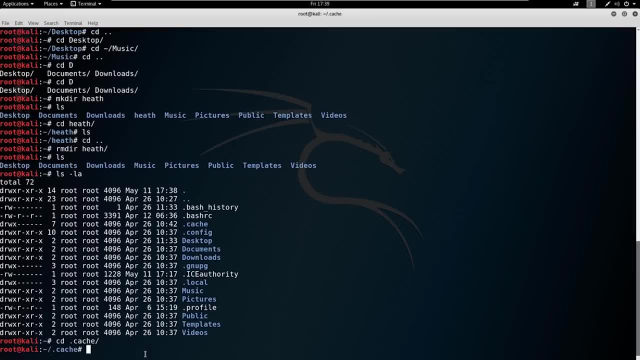 Remember the color coordination. So this dot cache right, That in theory is a hidden folder. So if we say CD dot cache, we can go into there, We LS, and there's actually some some information in there. but when you saw it originally, 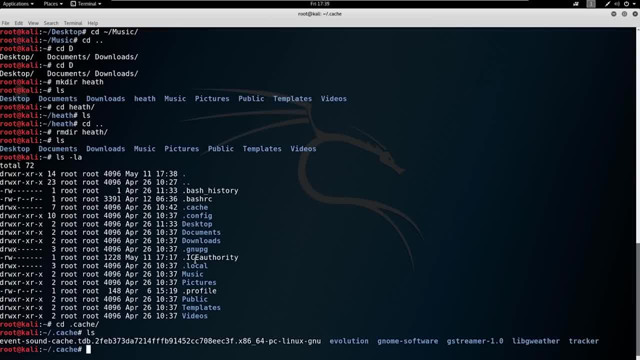 you didn't see that We're going to cover more on this. I just kind of wanted to show you that trick. As you see, over on the left side there's file permissions and properties. So be aware that just because it looks like something's not there doesn't mean it's not. 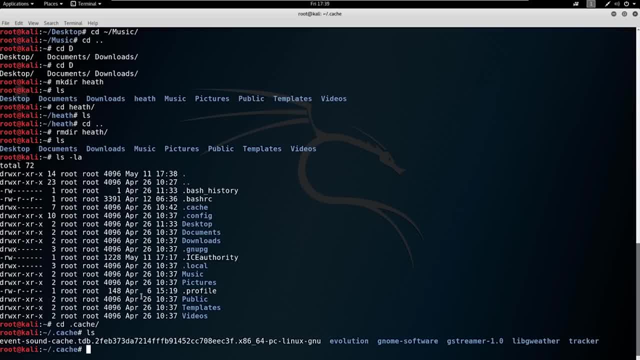 there. It might just actually be hidden, similar to windows, where you have hidden files and folders. So just a quick trick to show you that. So another thing we can do. so let's go back and don't worry about what I'm doing here. 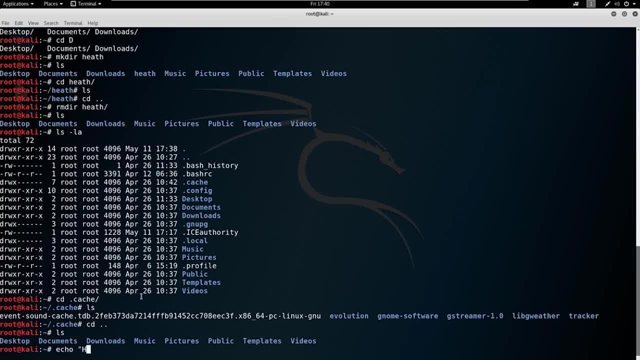 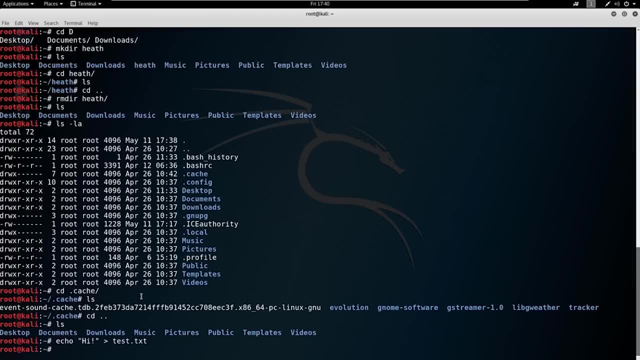 You're going to cover these commands in a little bit. Uh, I'm just gonna. Okay, I'm going to say echo Hi, And we're going to put that in a test dot text folder. So now, if we LS, you could see that test dot text is here. 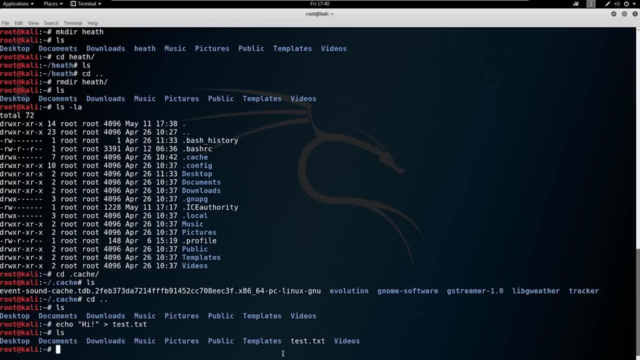 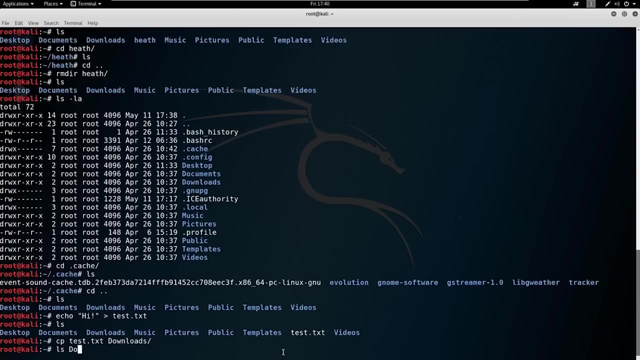 So if we want to actually copy this file, we can copy this file to another location. So we can say: Hey, I've got this test dot text, but I actually want to move it to downloads. Okay, LS to downloads. You could see that test dot text is actually sitting in there. 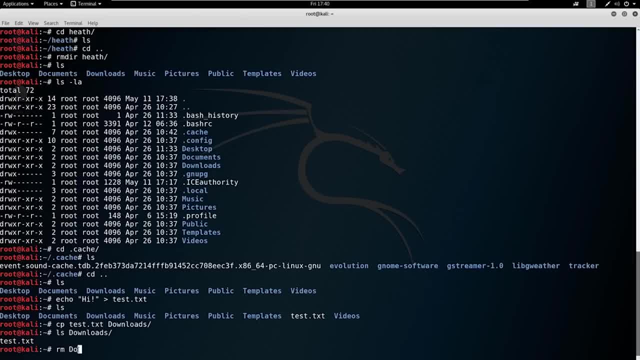 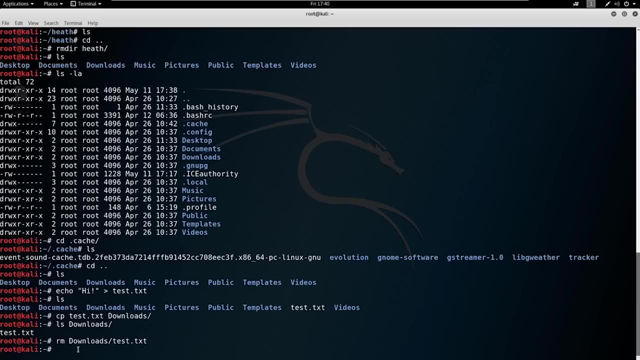 And if we wanted to remove it, we can just say remove from downloads or test dot text. Actually, sorry, remove downloads, test dot text. We don't even have to transition into that directory if we don't want to. So another trick: say we want to see now that it's gone and we want to LS, but we don't. 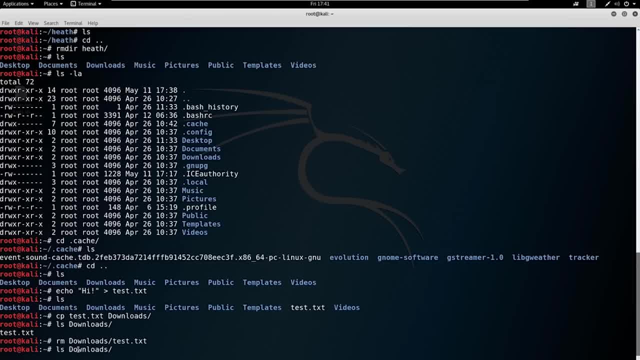 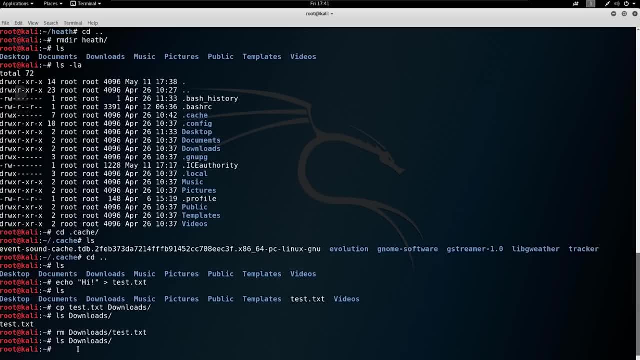 want to keep typing this out. Okay, Now you can just see your old commands. So if you keep typing a command over and over, you could see what's going on. So LS shows that there's nothing in downloads. Now we're able to successfully remove that file. 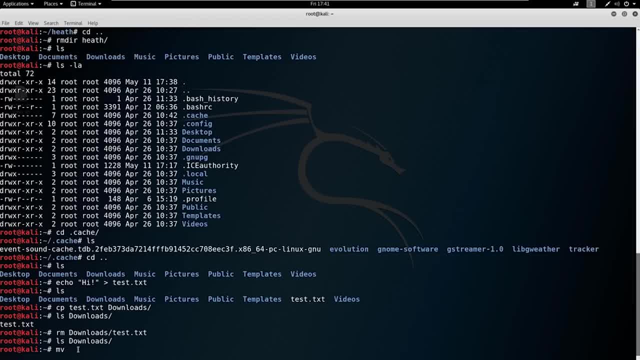 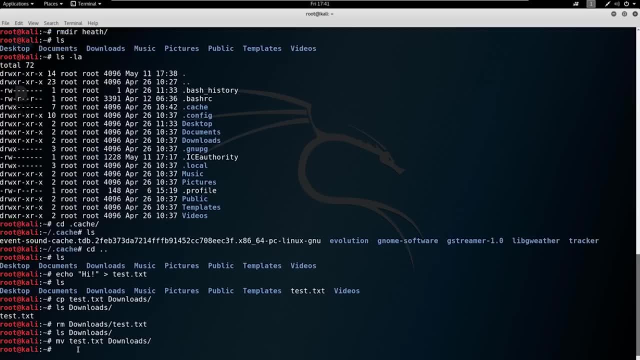 So another thing that we can do is we can actually move. So, say, we wanted to move test dot text and we wanted to put that into downloads. Okay, Now if we LS, test dot text is now gone from this folder because we've moved it. 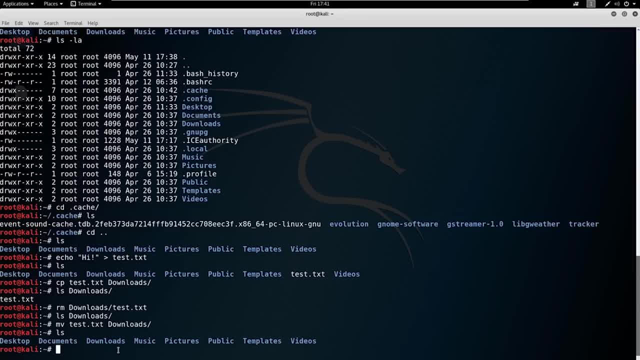 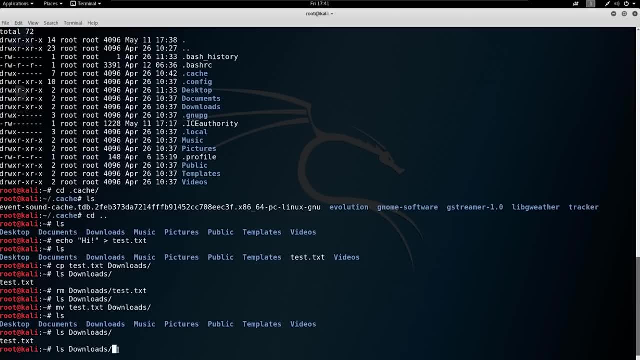 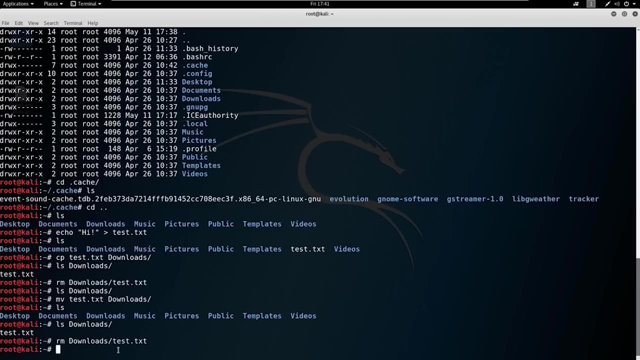 We haven't made a copy, We've actually physically moved it away. So now, if we LS actually, let's just tab up. You can see that test dot text is now in there and I'm going to remove that here. Okay, And now the last thing I want to show you is the locate feature. 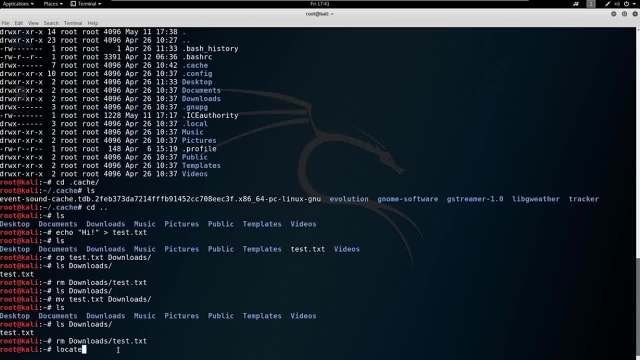 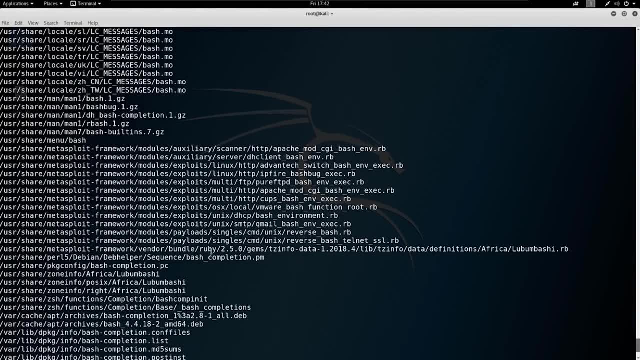 So if we wanted to locate a file- say I wanted to locate bash, let's see. So we're looking for a file and we're going to get more Specific along the way. but if you type in locate, you can kind of look through a system. 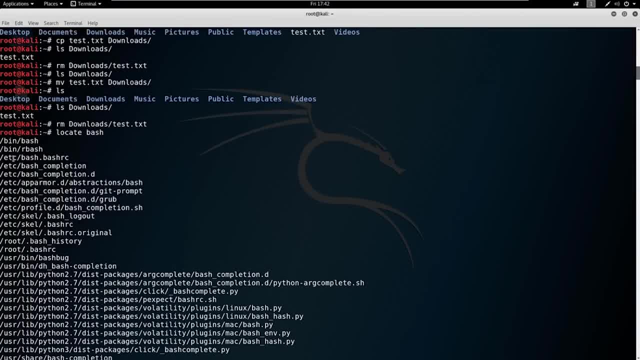 to see if you can find it Now. I'm looking for, say, any type of bin bash or bin R bash. That's fine, That's really what I wanted, but it shows you everything with bash in it. Now this might not work right away. 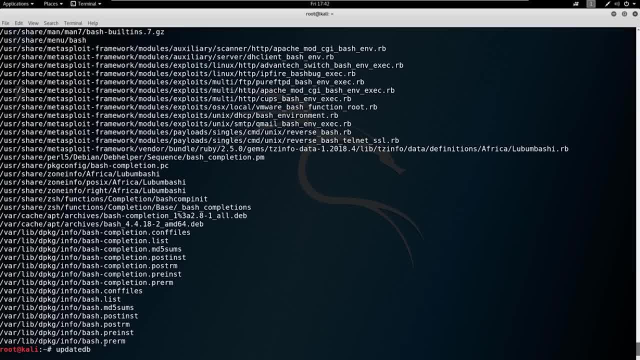 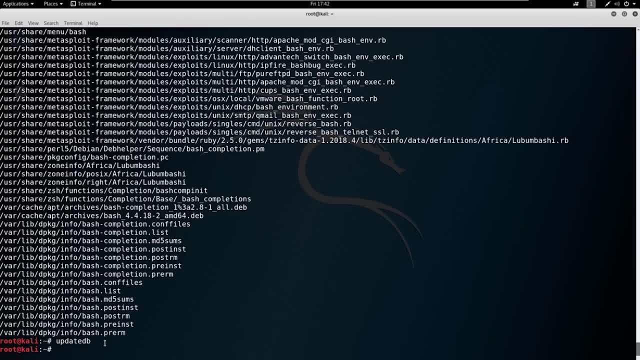 What you might need to do is update the database. So you type in update DB, it updates everything for you and then you can use locate again. Okay, So you want to build that database of the information that it's finding in order to locate what you're searching for? 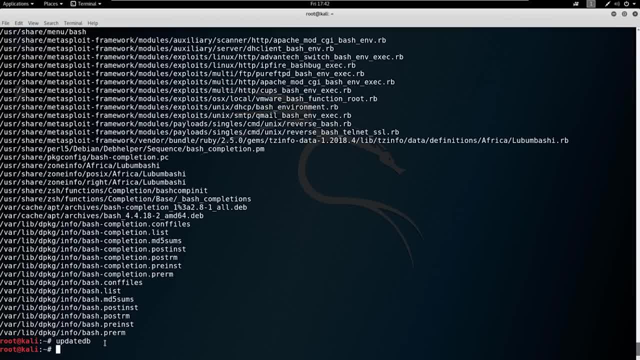 So make sure that you use update DB sort of frequently. Okay, So two more things I want to show you, and then we'll close out this video and move on to the next one. So an important thing you want to do with your new account is we're using a default. 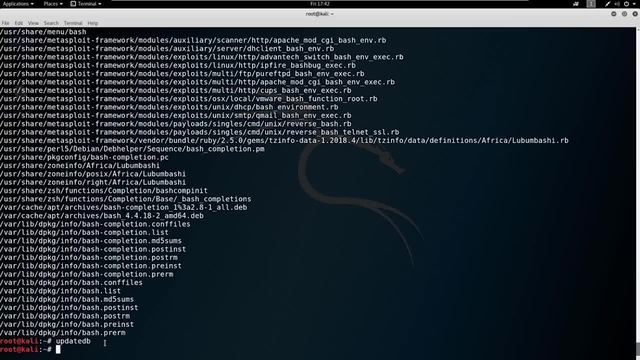 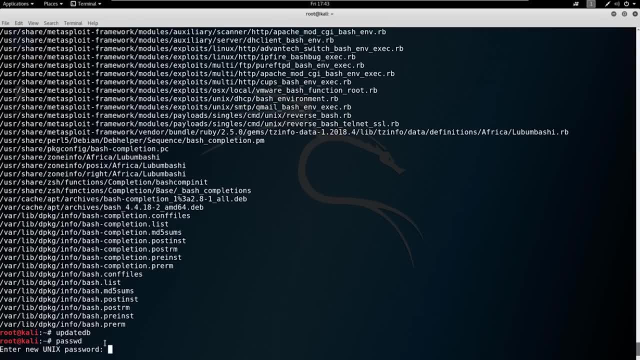 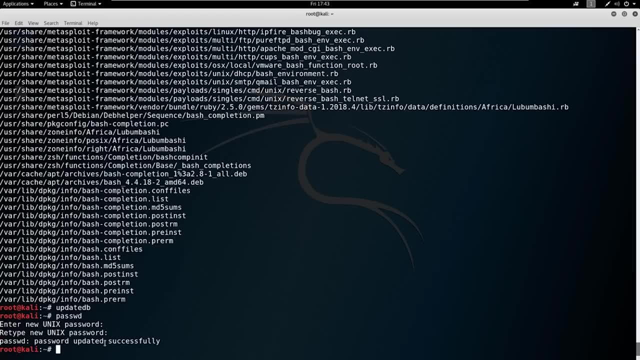 password and that's not very secure. So to change a password for our user, we can just type in P, a, S, S, W, D, And now it's going to ask us for a new password. So instead of using tour, we can use something else. 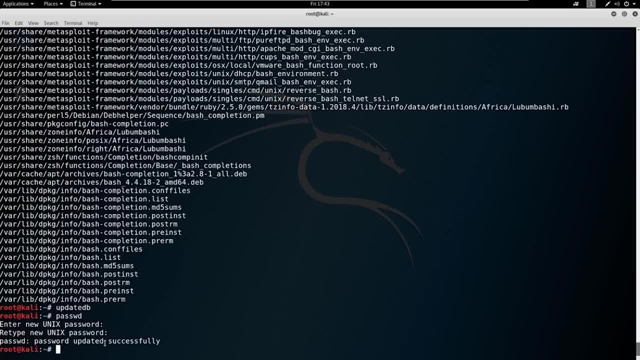 I'm going to type in the very secure password as my password for an example here. But if you plan on using this machine for future reference, you can type in a secure password and kind of keep it. So, lastly, I wanted to show you is something called man. 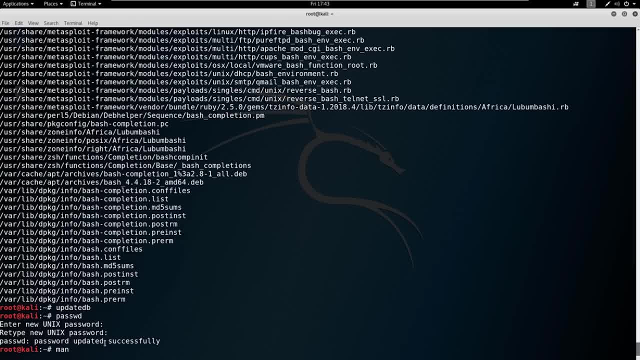 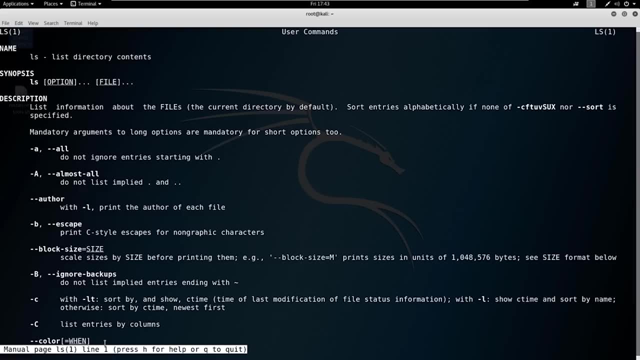 So man pages- man pages- are your instructions for any command that you're running. Most commands come with a man page. So let's say we want to look at LS. we can say man LS and then it's going to give us all this information here about LS. 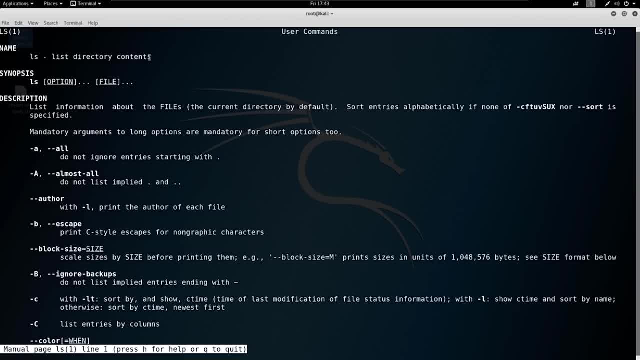 So if you see it says LS is list directory contents- awesome, And then it gives you what options we can do. Well, we can do a dash a for all what you saw earlier and you can kind of scroll through here and just see exactly what it has to offer. 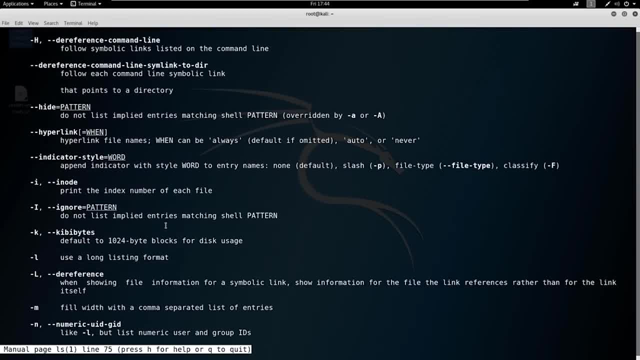 Okay, And that's kind of it. So when you go through here, um, you can kind of you know if you're struggling to like you know there's a command in there, but you're not sure exactly what the command is. 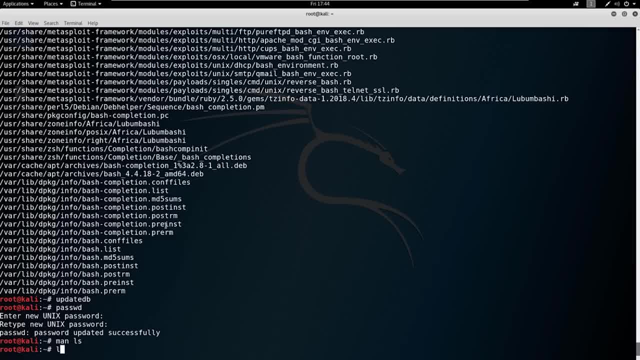 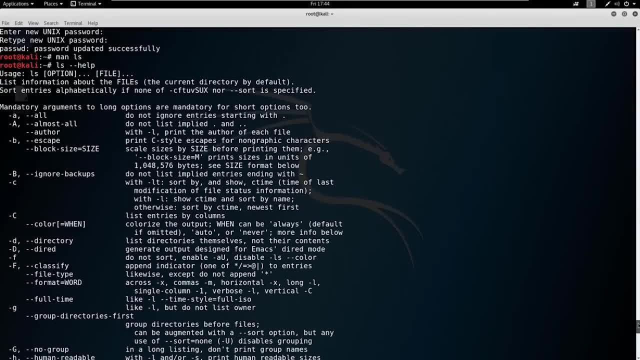 You can type in man and search it, and sometimes you can do LS. I don't know if this is going to work, but dash, dash, help and you get some information as well. It doesn't provide you the full man pages, but it provides you something pretty close. 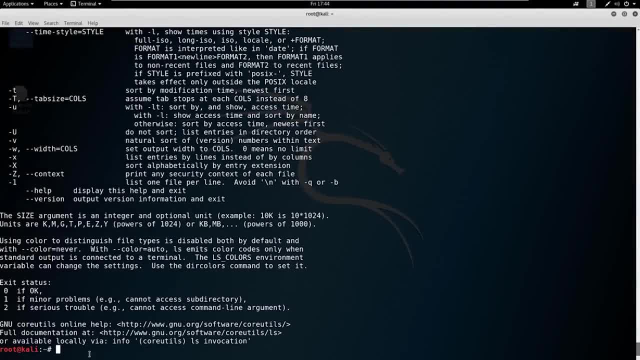 So that's kind of just your way around If you ever get stuck something to look for. Okay, So that's it for this lesson. Next we're going to move on to users and privileges: how to add users and how to- uh, how to change. 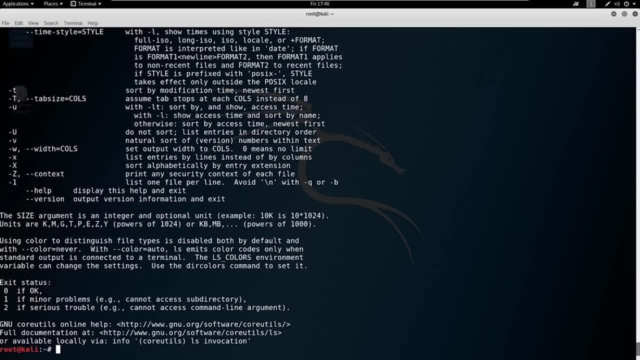 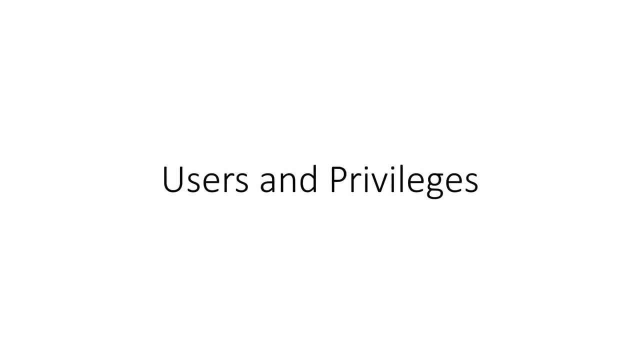 some pseudos and some modifications to our file permissions. So until next time, my name is Heath Adams and I thank you for joining me. All right, now let's talk about users and their privileges. So what are we going to learn in this lesson? 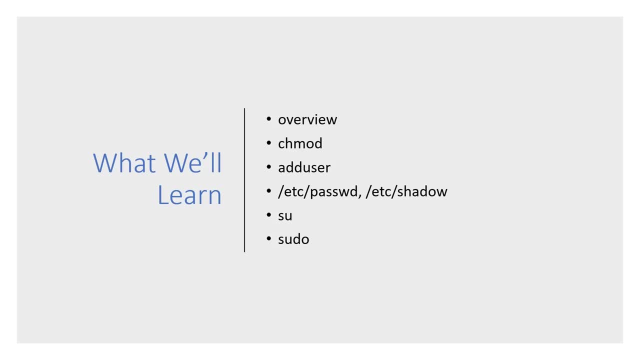 We'll do a quick user privilege overview from there. We're going to talk about the CH mod, The CH mod command, which is the change mode command that's going to let us change the permissions on a file or directory. We're also going to talk about how we're going to add a user with the add user command. 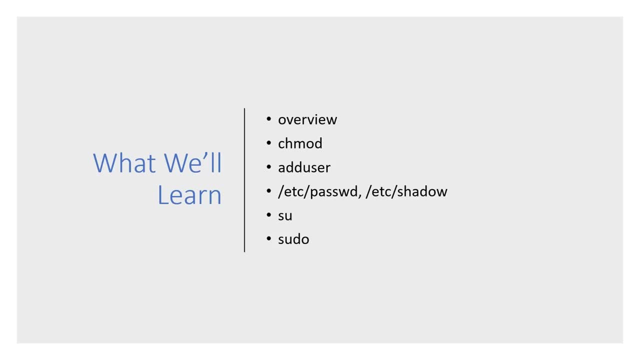 From there. we're going to take a look at a couple of important files. One is the Etsy password file and the other is the Etsy shadow file. So the Etsy password file is not actually where the passwords are stored on a machine. That is the Etsy shadow file which stores the hashes, but the Etsy password file does. 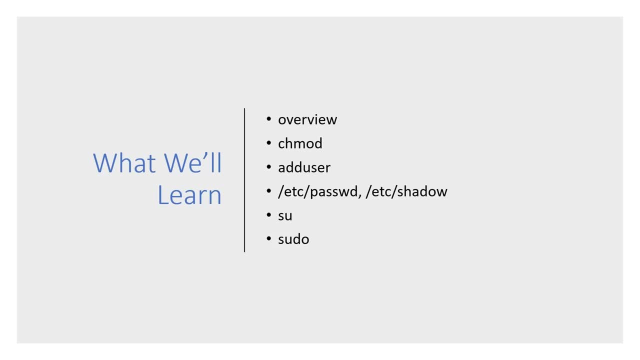 store it where the users, what users are on the machine, and you can correlate that to the shadow file. So we'll talk about those in more detail and their importance to pen testing- Very, very important. And then we're going to talk about SU, which is the switch user command. 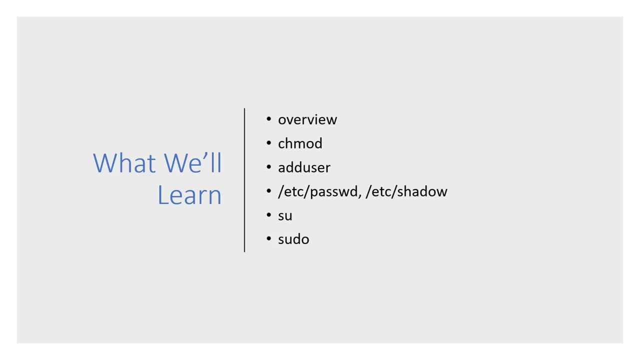 And finally, we'll talk about pseudo, which is a command that allows you to elevate your privileges on a Linux machine. Okay, So let's go ahead and dive right into our lesson. Okay, So now we're going to cover users and privileges. 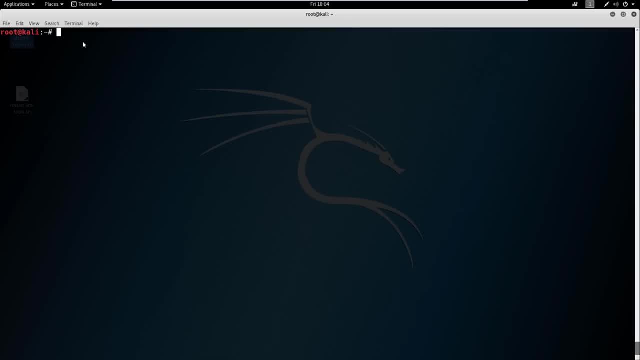 So in the last video we touched a little bit on privileges with our LS dash LA and we touched a little bit on users by changing the password of our root account. So now we'll cover a few more commands regarding those. So if we look again at LS dash LA, you could see all this crazy. 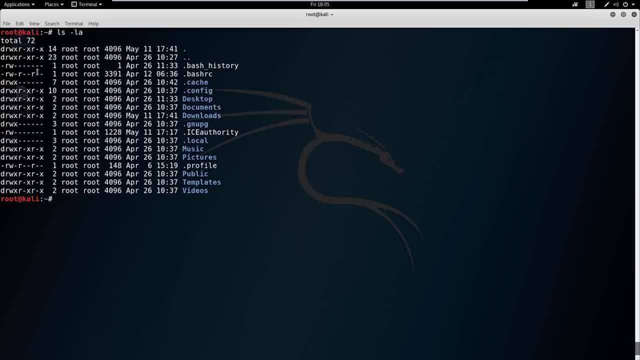 Jumbled wordage over here, right, So it actually means something. So we look at the first line here. If we see a dash like this, a hyphen, that means it's a file. If we see a D, that means it's actually a directory. 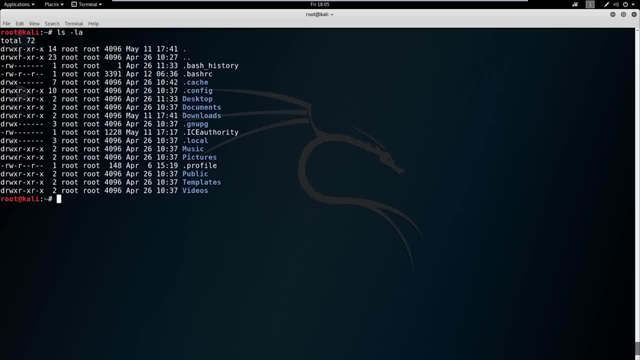 And then you see our W and X. So our W and X actually means read, write, execute. It's the permission settings that this particular group has. Now there are Three groups here: There's the first, second and then your third right here, right. 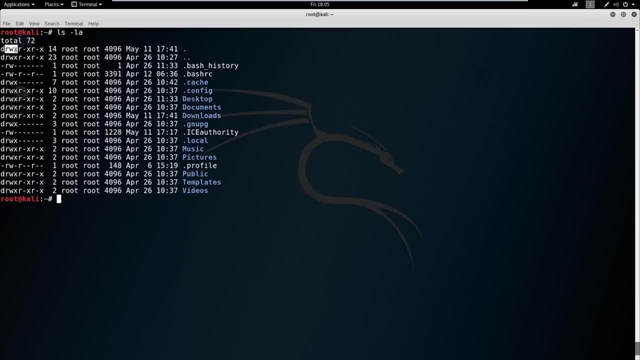 So your first group right here is the owner of the file. So it looks like the owner of the file has full read, write execution right. And then the next set of three here is actually the permissions for the members of the group that own the file. 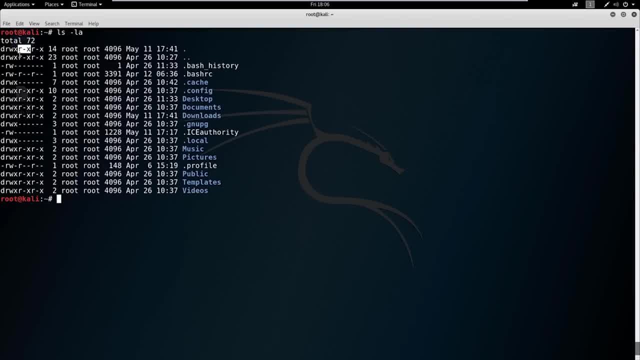 So this is a group ownership as opposed to actual ownership here. So for the people that are in the group that has access to this file, they can only read and execute. They can't write to it. Now for the last one. this is just all of their users. 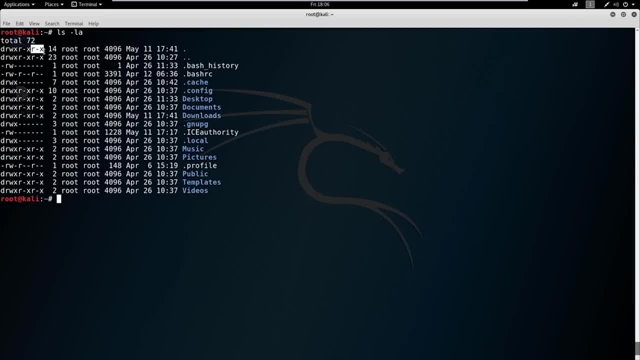 So any common user here can actually just read and execute. They can't write the document. So that comes into play, especially when we get into penetration testing, because with penetration testing we're looking to have full access right. So we're always going to be looking for that folder that has full read, write and execute. 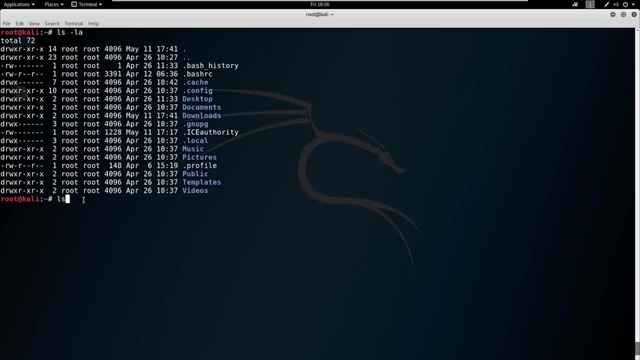 So we're looking to have full access right. So we're always going to be looking for that folder that has full read, write and execute. So we're looking for that folder that has full read, write and execute. Typically, if we look at temp, that's our temp folder a lot of times. 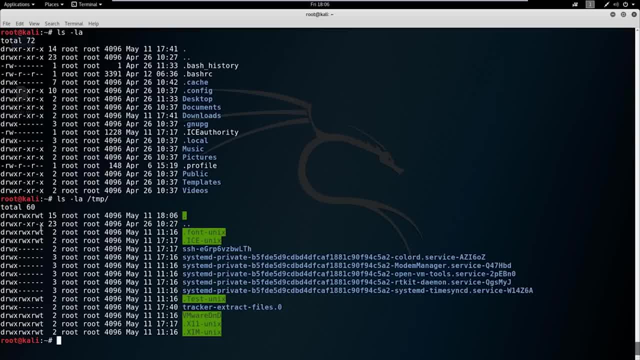 You see, the temp folder has full read write execute. So when we're doing penetration testing, we're trying to upload some sort of exploit, We might actually upload it into the temp folder because that's where we can execute those files. However, we could also be looking for other full read write execute files where we 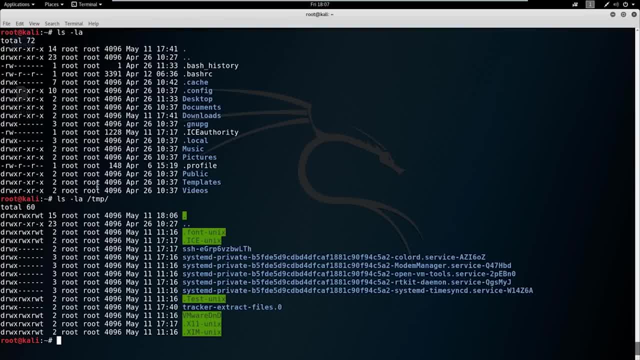 need to modify them and give us root access to a system. So it's all about insecure configurations and we're going to cover that more once we get into the actual penetration testing part of the course. So for the Linux essentials part of the course, all we need to worry about is these file permissions. 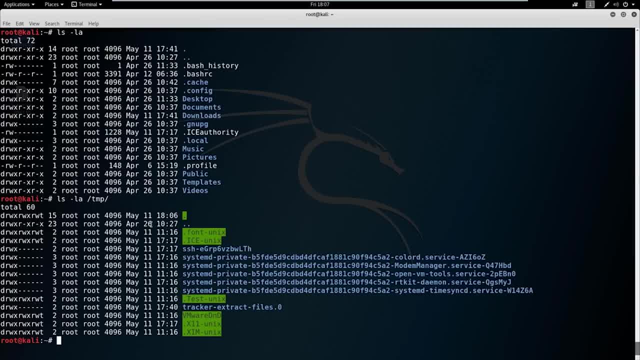 Another important feature of that is, if we were to create a script, our script's not going to be able to run until it has full access. So how do we change access here? So let's make a file. I'm just going to make. 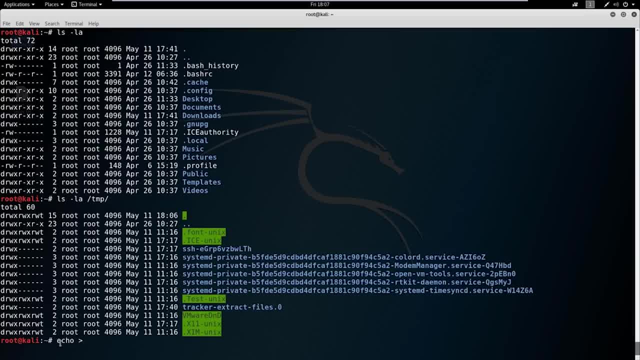 We'll just execute it, Okay, Okay, Okay, Okay, Okay, Okay, Let's echo another text document, right? So we'll just say hello, and Actually I typed that in backwards, So hello, and we'll call it hellotxt. 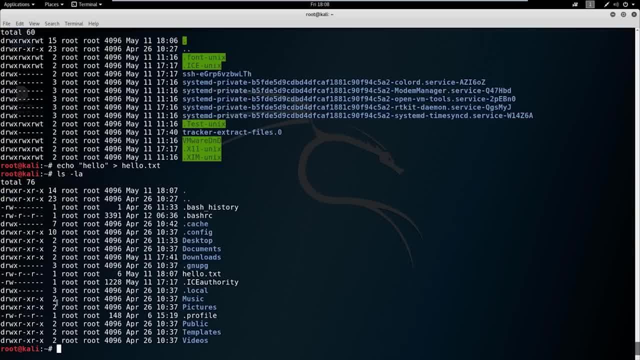 So if we LS here, by default we only have read, write and then read access for everybody else, Meaning if we wanted to read it, we could say cat, which we're going to get into later, Cat hellotxt. Now just say read. 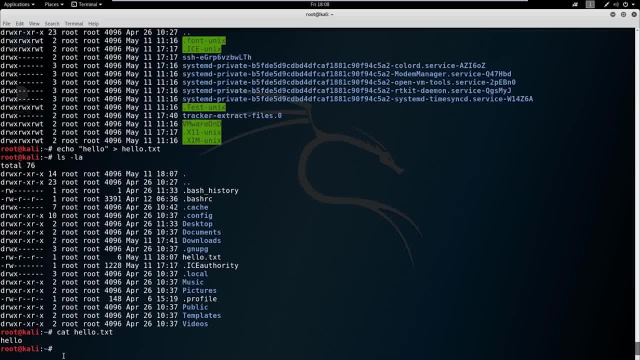 just says hello. So what can we do here? Well, we can use something called change mode, And changing mode is ch mod, And we have a couple options here. So we can do a plus right And we could say: well, we want read, write, execute, or we just want execute, But another way I like doing it. 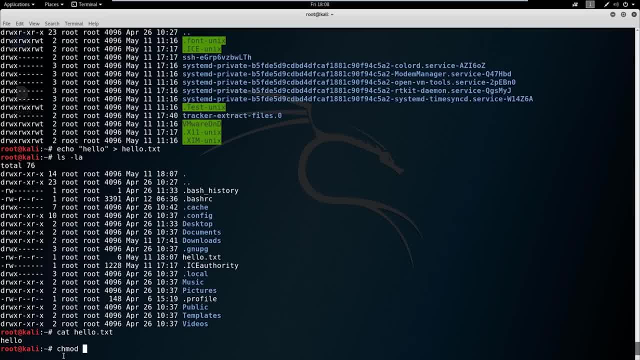 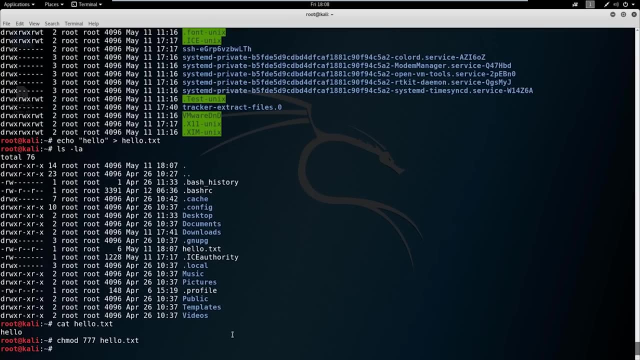 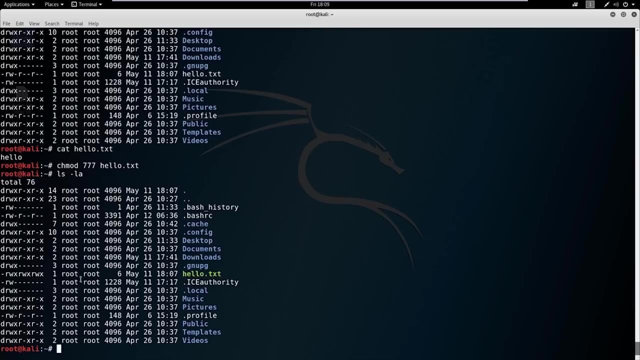 is you have a number feature, So the one you really need to know is all sevens. sevens gives you full rewrite access across the board. So if we say ch, mod 777, hellotxt, Now we LS la and you notice that hellotxt turns green, that means it is full rewrite. And here you go, we've got the. 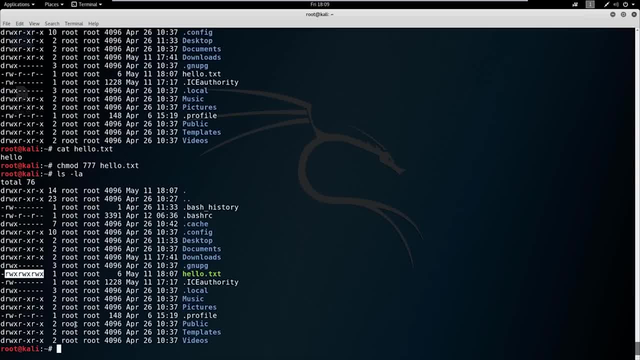 dash here saying it's a file And we've got read, write, execute or read, write, execute across the board. So this is how we change file permissions. you don't need to necessarily know about the other numbers in terms of penetration testing. it becomes more in terms of configuration. 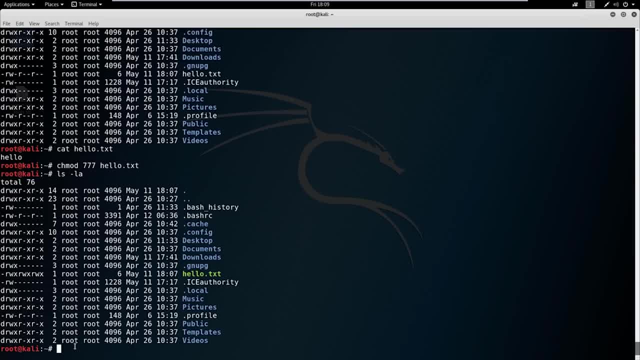 and security management of files if you were to get down that path. So to stay on the easiest path, just remember 777 or plus x will work as well. So changing the mode is is critical, And we're going to cover it time and time again throughout the course once we get a little bit deeper. So 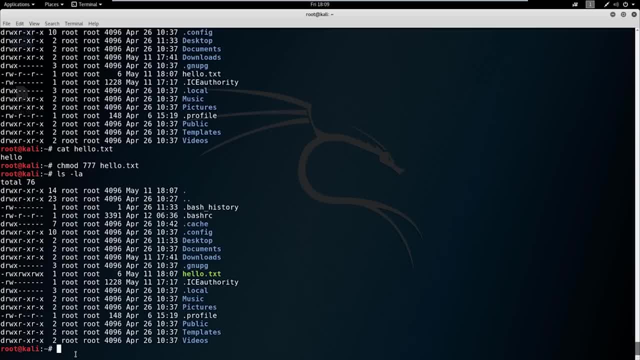 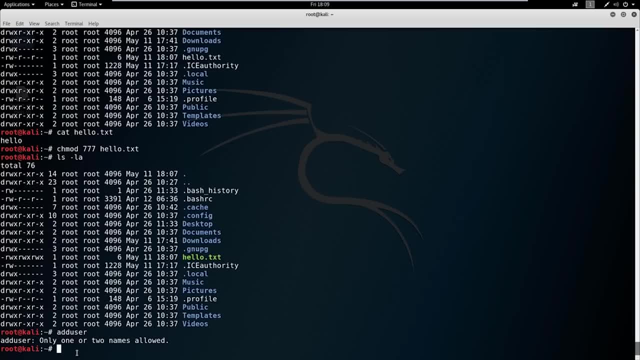 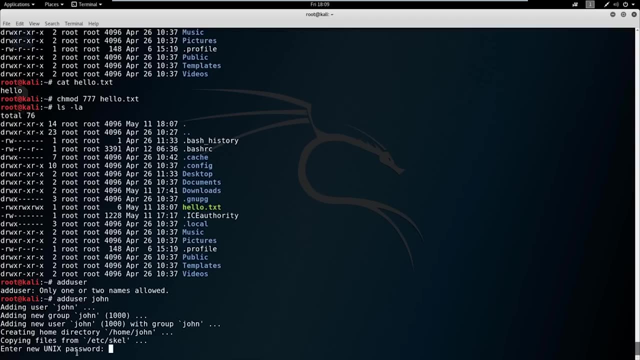 a couple more things we need to talk about. Say, we wanted to add a new user. Well, there's a feature called add user. So we say add user And one or two names is allowed. So we need to add user. say john, Okay, so it made something for john, let's give him a password. Give him. 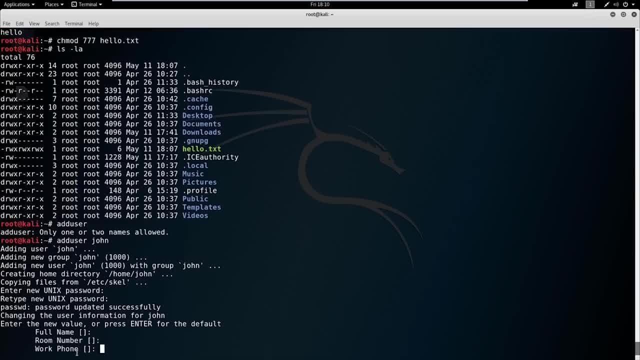 a password again And we'll just hit enter for the defaults. It's all correct. Okay, so we now have a new user And we're going to say add user And we're going to say add user And we're going. 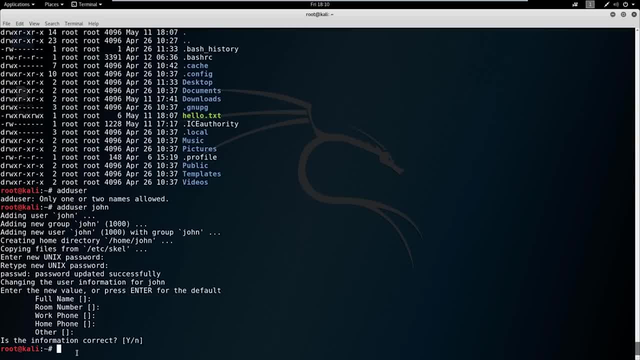 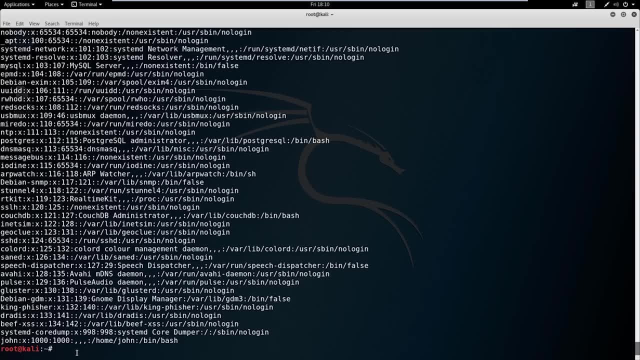 to have a user named john And we can confirm that. we can actually cat the Etsy password file here And you see, down at the very bottom we have this user, john. So this Etsy password file you're going to become very familiar with because it shows you all the users. Now this will there's. 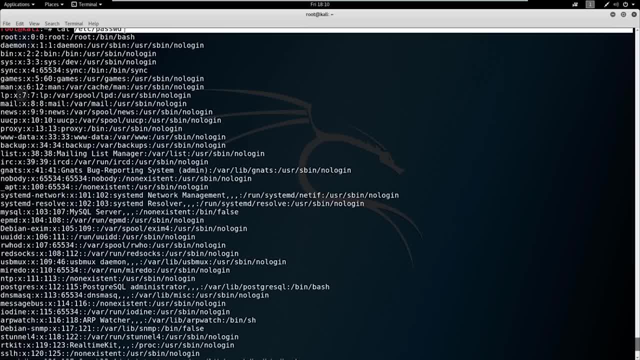 a lot of times where you're doing penetration testing. you're going to have access to this Etsy password file because it doesn't provide the password anymore It used to a long time ago. passwords are now in the shadow file, So you actually have a little bit of access and 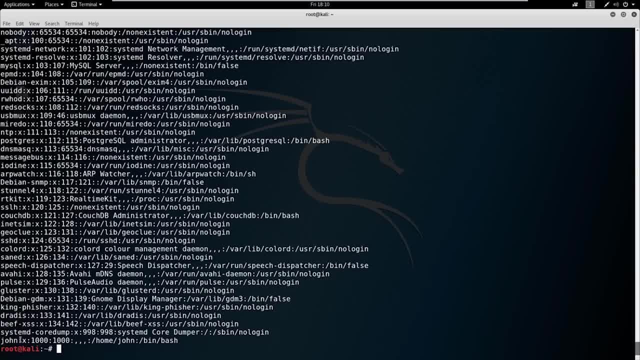 information disclosure here at the hands of poor configuration. So you see that I've created a user, john. well, that gives us a little bit of information. say, there's SSH on a machine or something else, we can use that username of john to try to break into the machine. So 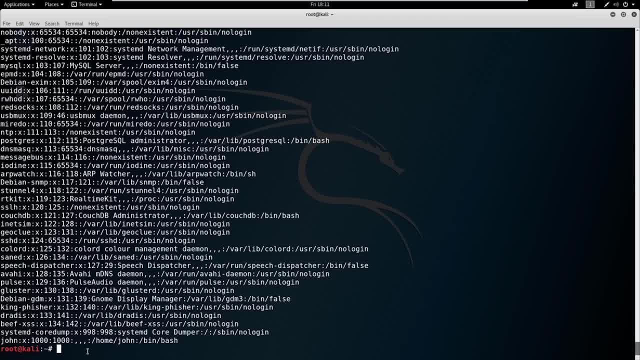 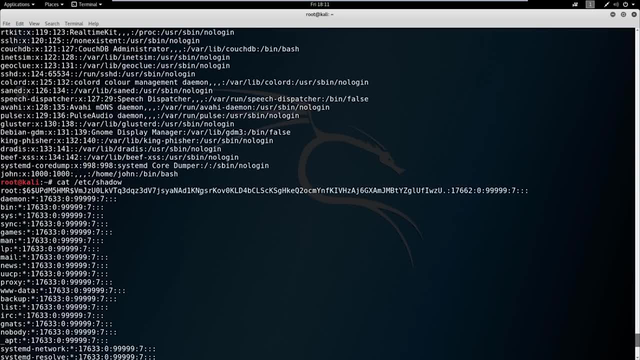 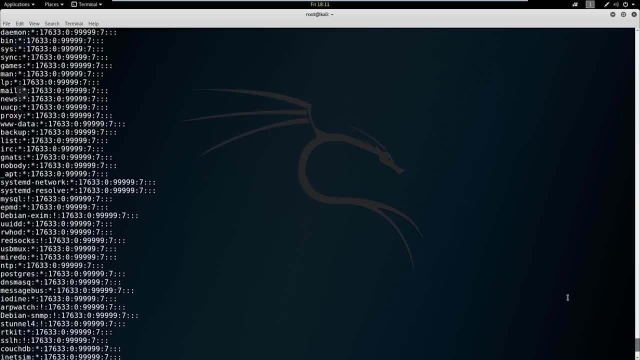 we'll cover that again later, But if we wanted to see what the Etsy shadow file looks like, now we come in here and you've got these, these jumbled stuff here, right? so it's just a hashing format. So what we're doing is we can actually use a tool like hashcat to break this. 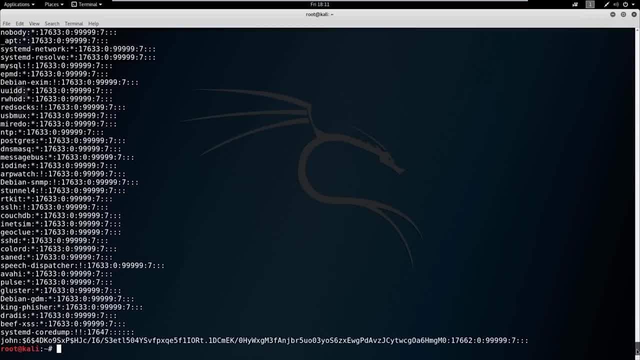 down and crack these passwords Now. a password, a password, will be very easy, But just know that if you have access to the Etsy shadow file, you have a good chance of cracking a password, depending on your capabilities And depending on the structure. 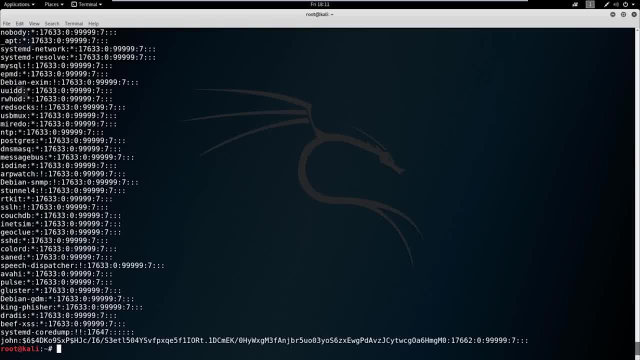 strength of the password that allow you access to a machine. So something to think about there. Okay, so now we have our user john. let's go ahead and switch to him So we can use something called su, which stands for switch user, And we'll say: switch user john. 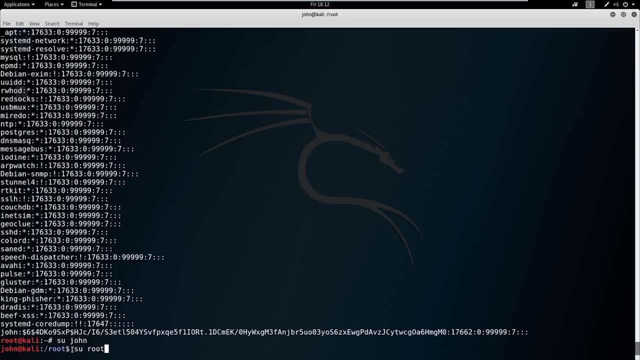 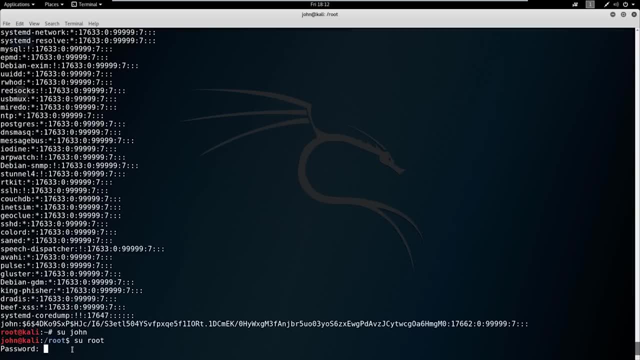 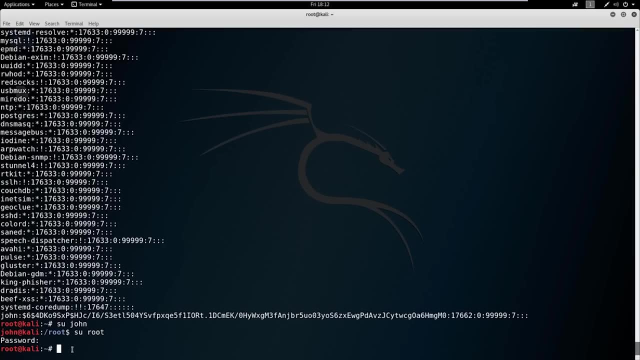 Okay, so automatically gave us john here. let's see if we could switch back to root. Okay, we can't just switch back to root because we need roots password, right, So we can type in password and that works. But if we didn't know the password then we'd be stuck on john. we are able to access john. 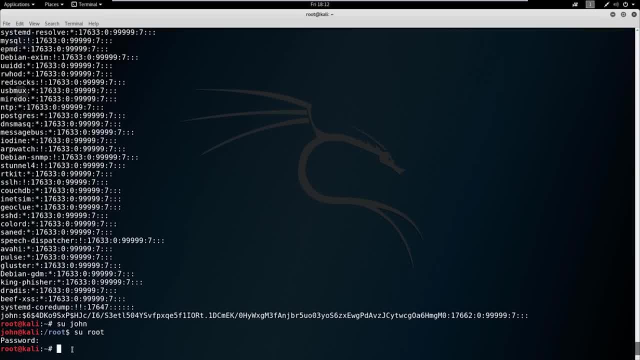 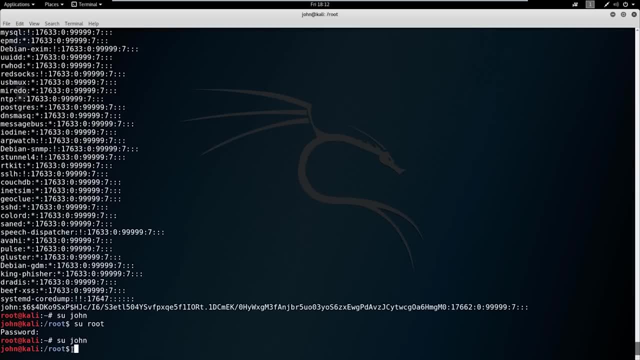 because we were already root. So this comes into play in terms of users. Let's go back to john here Now. if you're a user, you have to be able to do certain things. you need permission to do certain things. I should say right. So root has full access and permission to do everything. 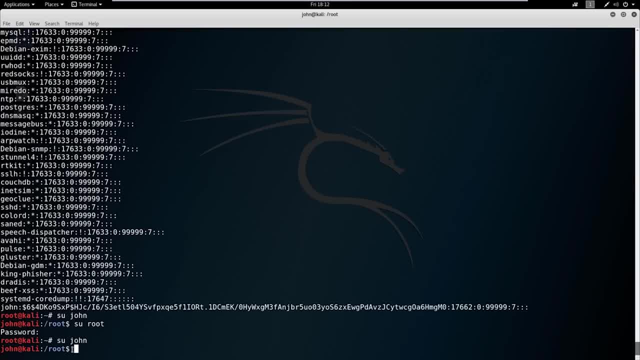 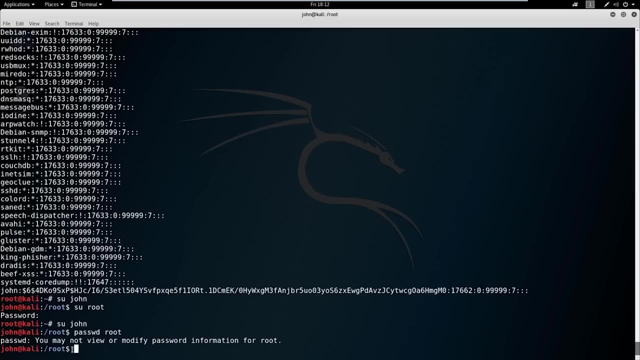 But john, we just created john. john doesn't have any sort of access. So if we wanted to, you know to, if we wanted to change the password, say we want to change the password for for root, I can't modify the password information because I don't have that kind of access. Now, 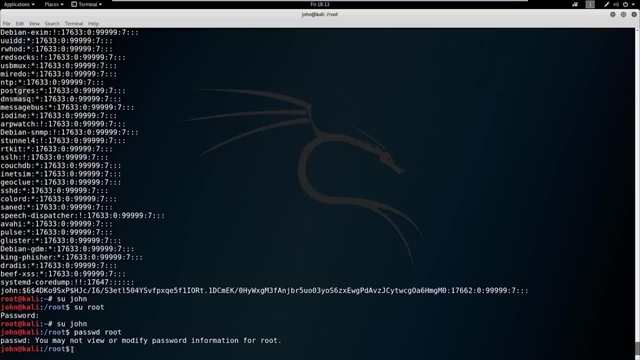 there is something called a sudo which would provide john that access if we gave it to him. So it's called a sudoers file And basically anybody in that sudoers file can change permissions given if they are a sudo user, right? So we would type in: 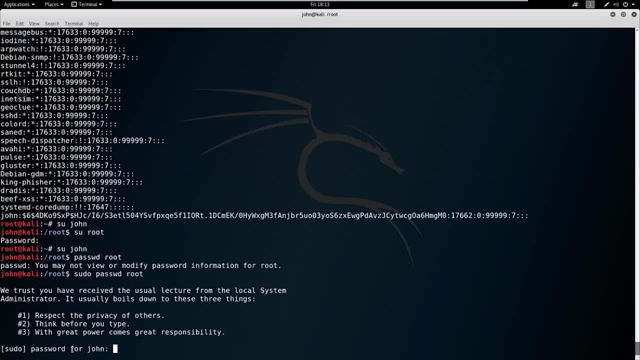 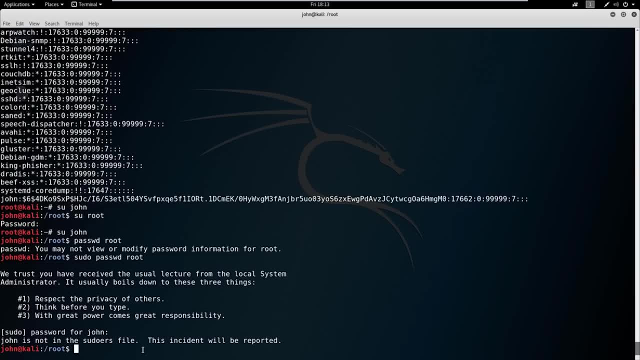 in sudo, password root And it's going to ask for the password for john. But you're going to notice hey, john's not in the sudoers file. john can't do this, So john has base permissions right. And we're going to encounter that a lot of times in penetration testing where, if we get in, 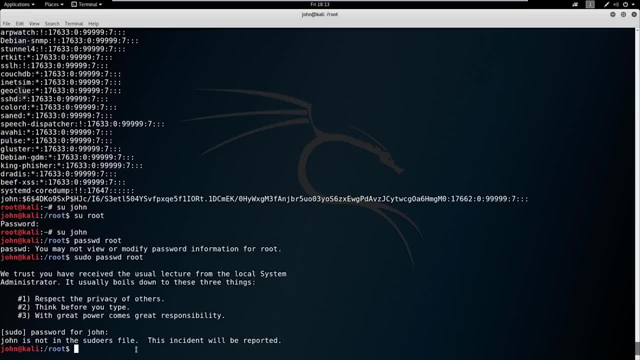 we'll get something called lower privilege And we'll get an account like john and we're going to try to escalate into root. but we just can't do it. you know, the chances of doing a doing that and and having a john in a pseudonymous file is just not high. It's possible but it's not likely. So 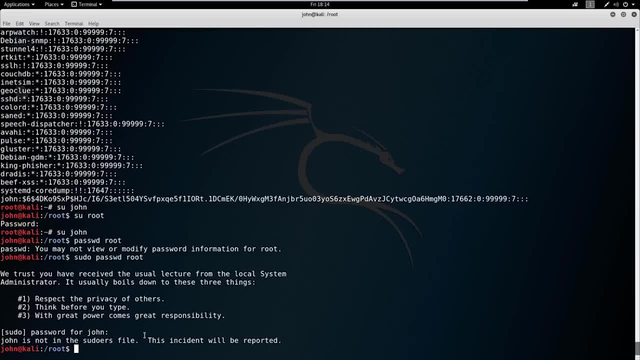 for now, just know that if you want a user other than route to have access to file permissions, you need to have them in the pseudonymous file. That becomes useful to in penetration testing because you can look at the sewers file if you have access to see what users have pseudo privileges. 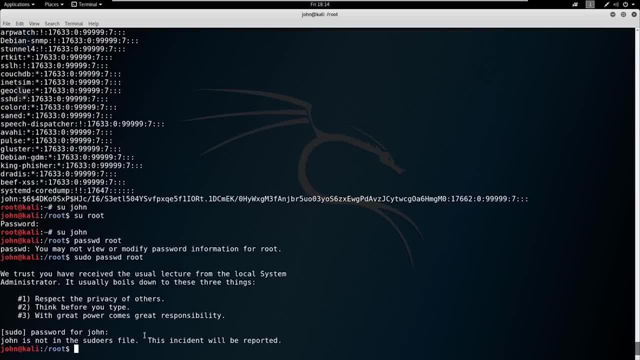 Okay, so that is it for this lesson, And the next lesson we're going to be covering network commands and moving on gradually towards scripting. So let's go ahead and get there And I will see you when we get over there. Alright, so now we're going to be covering common network. 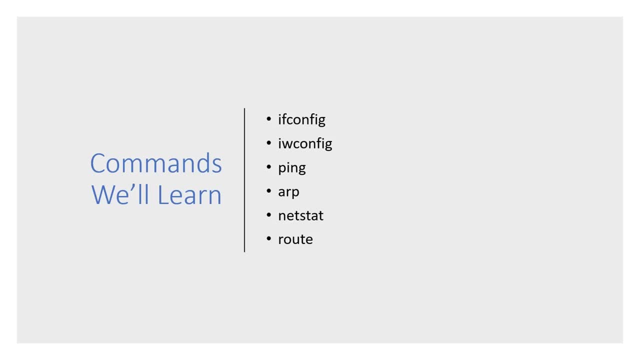 commands. So before we dive into the commands, we're going to learn. I'm going to go on a tiny bit of a rant here. So if you're not familiar with networking, now is the time to become familiar with networking. There are two things I think that a person needs before they really can dive. 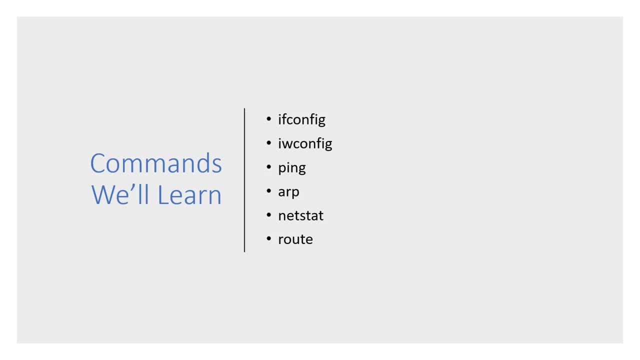 into programming, And that's the first one- is that they need to know what they're doing And pen testing, and that is Linux experience, which you are gaining some Linux experience now, because most pen testing is done in Linux, And the other thing is to have a good network. 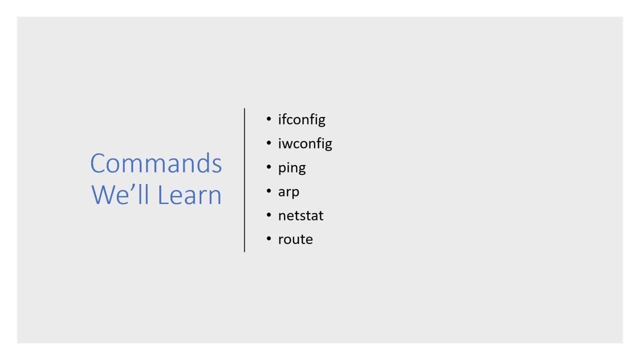 foundation. So if you're looking at these commands here and I say if config, which, if you're a Windows user and you hear IP config, you know what that is okay. that's basically the same thing. If you know what ping is, if you know what ARP is, netstat route, those should all be pretty. 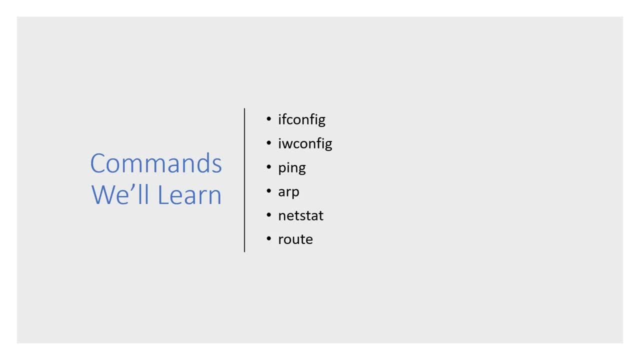 familiar where you can guess what those are. If you do not know what these commands are, you might want to brush up on your networking as well, Because the better you are at networking, the better you're going to be when it comes to pen testing, because you're going to have to navigate. 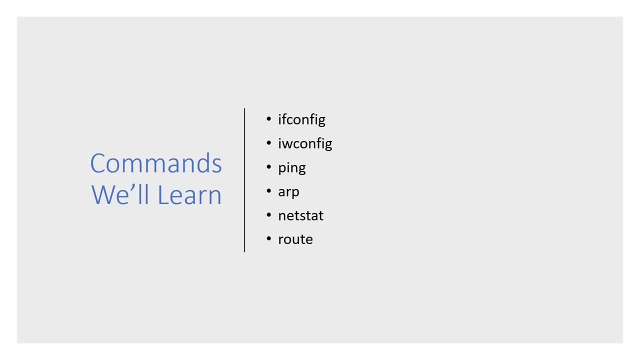 around networks. you're gonna have to understand where you are at in a network. you're going to need it for basic troubleshooting as well. So just to understand these commands are going to be very important, But what we're going to be doing here is we're going to be looking at some basic 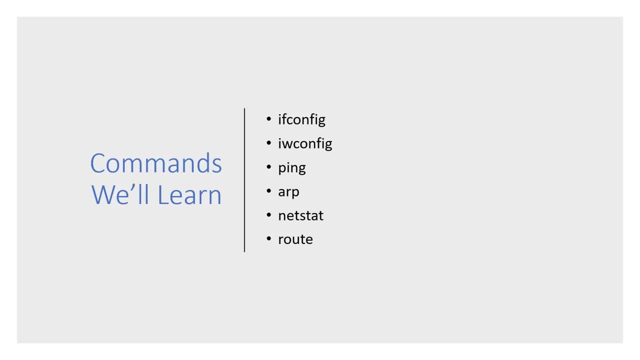 commands that we're going to be running as a pen tester And we're just going to apply those to their version in Linux. Some of these may be familiar to you, some may be new to you, But we're talking here if config, which is going to show us some information very similar to IP config in 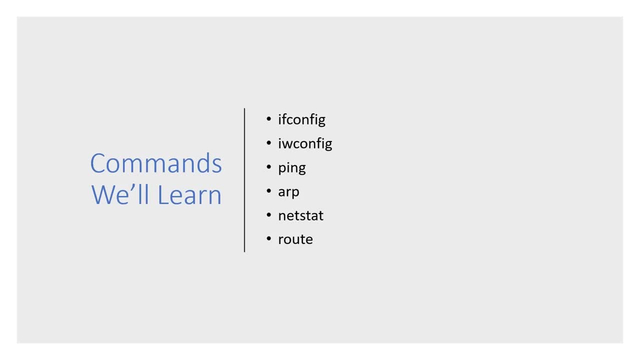 Windows where we'll see our IP v4,, IP v6,, if we have it information, our MAC address, things along those lines, our subnet mask, etc. The IW config is the wireless adapter version of that. ping is a ping command where we're talking. 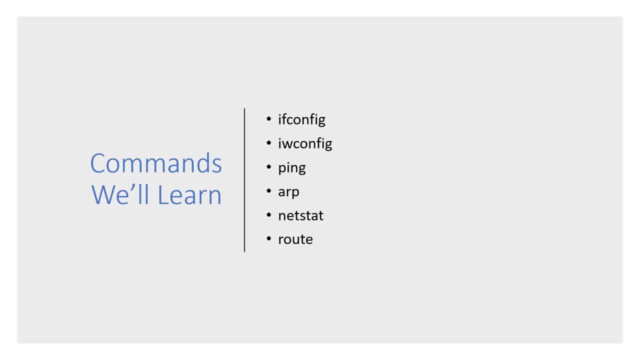 over ICMP And we try to communicate to another machine to see if it's alive and responding back to us. We've got the ARP command, which just maps IP addresses to MAC addresses, And we've got net stat, which is just a command line tool that's going to allow us to display all connections and 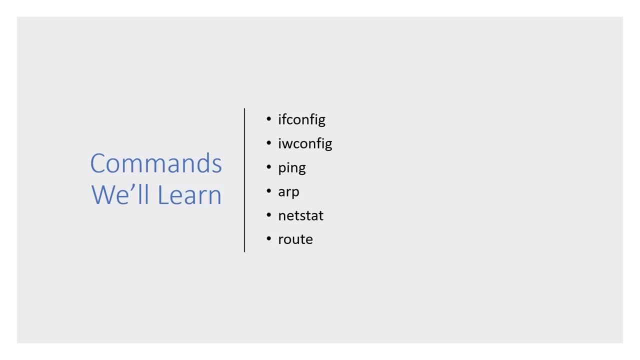 listening ports. And then, finally, we've got route which displays our routing table, So we'll go ahead and take a little bit of a deep dive into those in this next lesson, And hopefully this is a refresher for you. So again, if not, then you should be looking into some networking studies as well. Okay, so let's go. 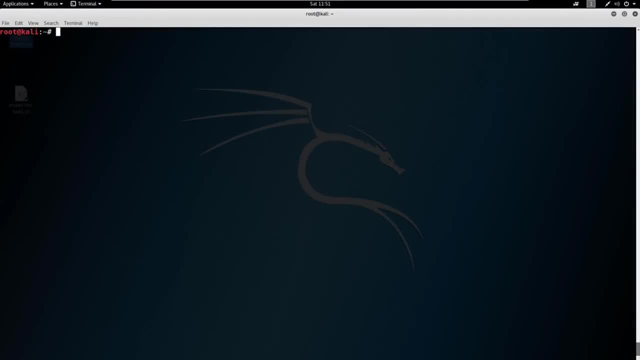 ahead and dive right in. Okay, so now let's cover network commands. So the first command I want to cover is if config. So you may be familiar with the Windows version of this, which is IP config, And they pretty much do the same. 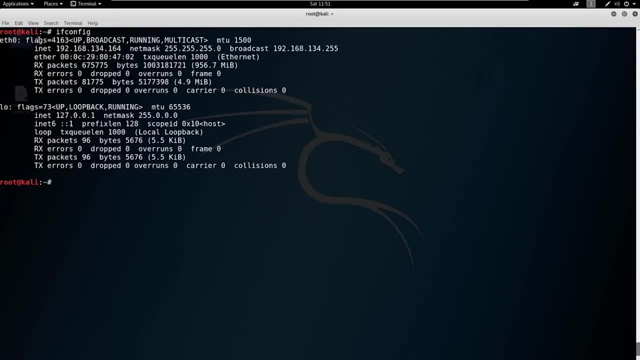 thing. So it shows you here your different interface types and the IP address associated with them. So each zero here, Ethernet zero, has an IP address of 192 dot 168, dot 132, dot 164.. You can see the net mask, the broadcast address, And you can see the MAC address as well. 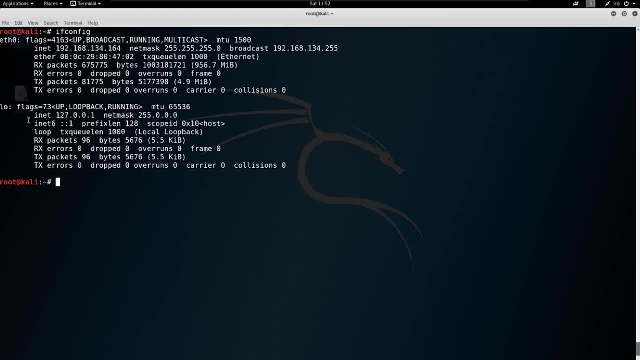 And we also have a loopback address here. Now, if your machine has a wireless adapter or at some point you want to do wireless penetration testing, you're going to need iw config And you should not expect to see anything on this at the moment. 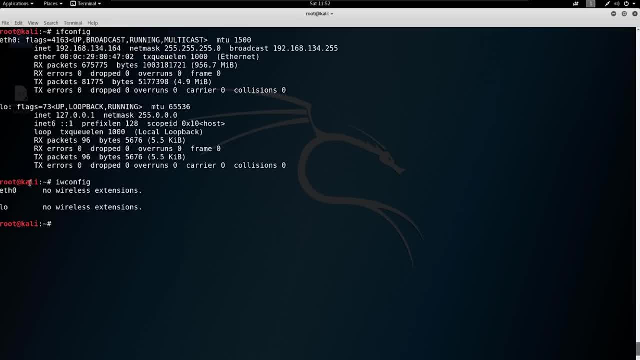 unless you're using a laptop, then you actually might see configuration down here for it. If you would see something under iw config, you would see like a WLAN one w LAN zero, something along those lines. Let's call this amp eaz. ramp in file p. noise ramp in file coli. We'll call this. uhm, we'll call this탔, Because, as we're using the IW config, we're actually seeing them give or 아버ate attempts in to tell us what's going to happen next. 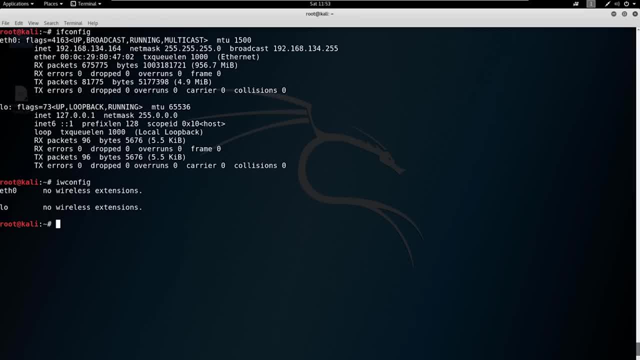 lower. So you're gonna want to Var accounted for coding something along those lines. okay, and another common command that we're going to see is going to be the ping command, so we can just type in ping and the address that we're trying to talk to. 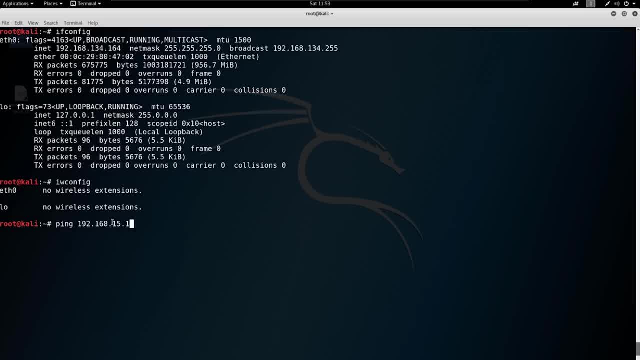 so, for example, i'm going to try to ping my home router and i get talking back. so if i tried to ping something that wasn't in my network, like a 16.1, you're going to see the results change. so with ping here, ping is going to be endless until we. 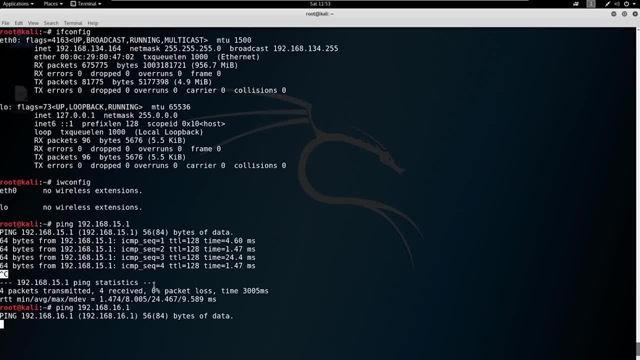 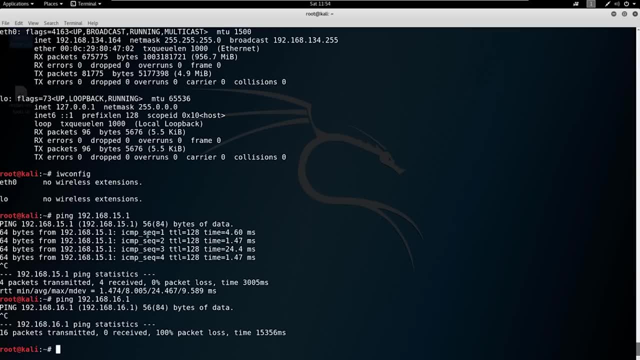 hit something like ctrl c to stop it, it'll ping forever. so i'm going to hit ctrl c again and kind of show you the difference. so you see that we attempted to ping here and we got replies, we got information back. well, that's good. but that means we're talking to the 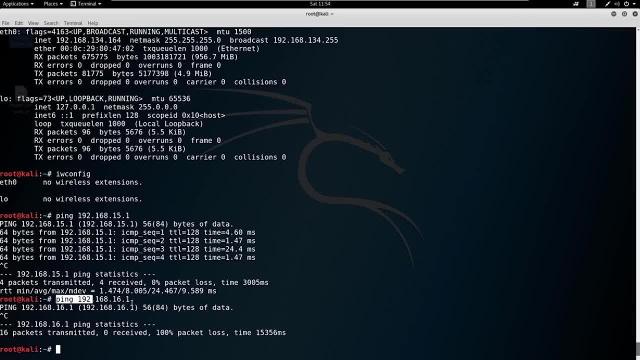 other machine. it says, hey, are you there? it says, yeah, i'm there and we try to ping this machine here, but this machine's not talking back. it could mean that the machine is on the network or that the machine is just blocking icmp traffic. icmp is a another. 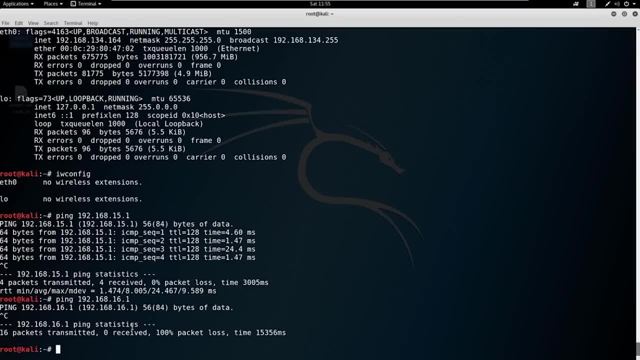 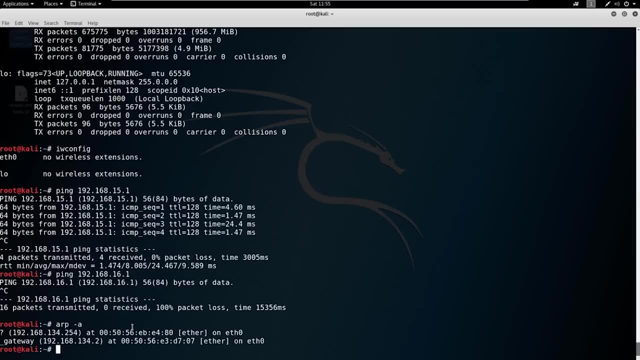 word for ping. so, moving on to the next command, i want to show you arp. so the best way i like to type in is arp, with the switch of a, and arp is just going to show you mac addresses that it talks to and the ip address. actually i said that backwards. it's going to show you the ip address. 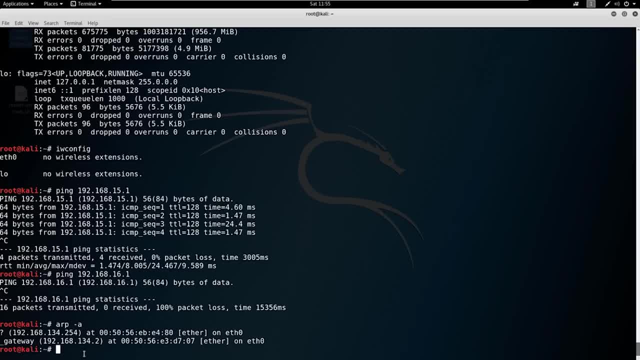 it talks to and the mac address associated with it. so if an ip address reaches out, say 192, 168, 15.1, talked out to this machine, it's going to say, okay, hey, who are you? it's going to send a broadcast message out and say who has this ip address? and then the ip address will respond and says hey, i do. 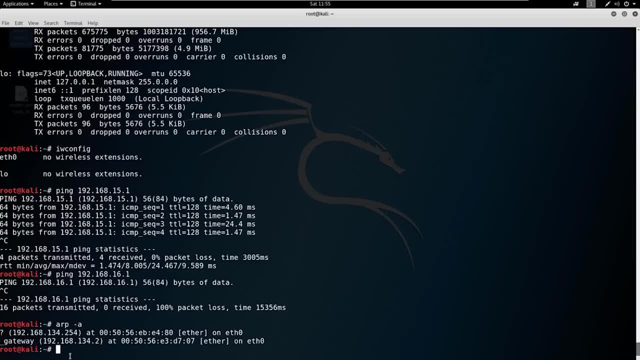 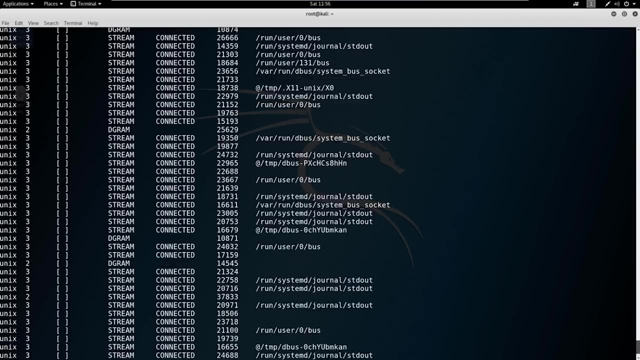 this, and then the ip address will respond and say: hey, i do this. and then the ip address will respond and once you know that, you can also look at netstat. so netstat-ano is another one of my favorite commands and this shows you just the active connections that are running on your machine. 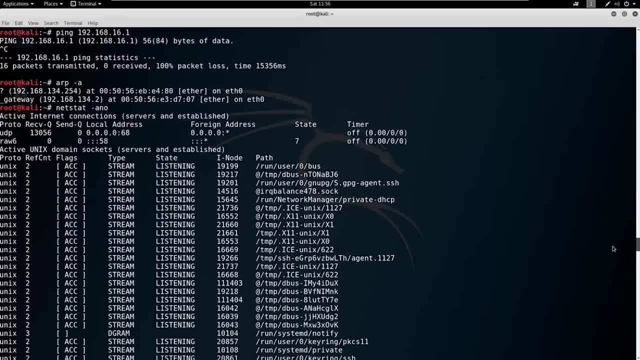 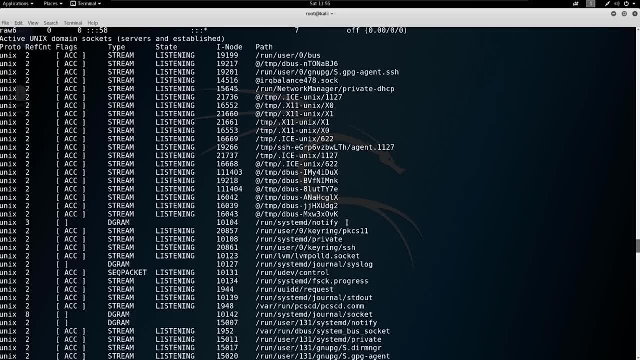 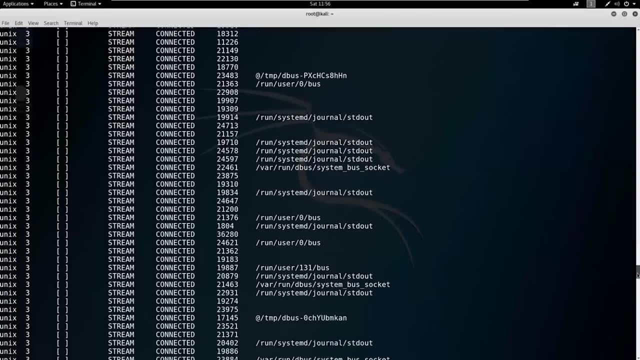 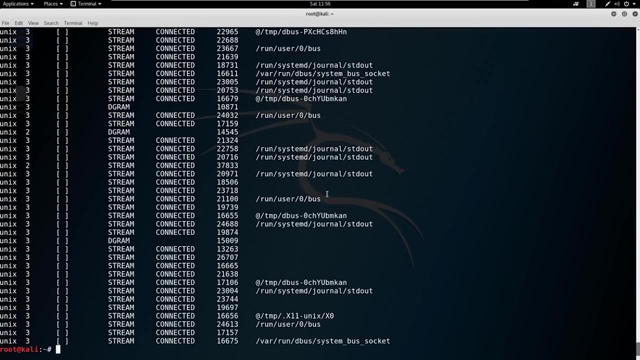 so if you scroll way up and you can just kind of see what's open and where what's talking here, where this really comes in handy on a penetration test is to see if a machine is talking to somebody else. same thing with arp. you want to know what that machine is associated with and is it talking? 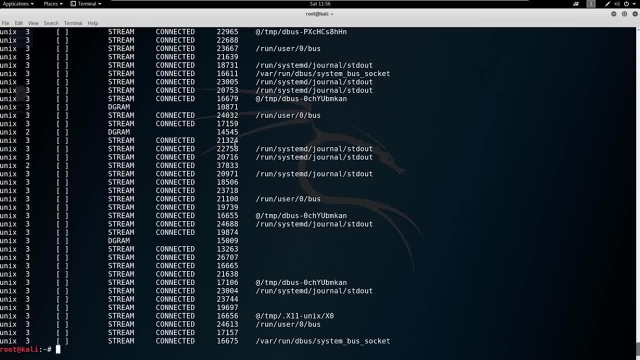 to something on a port. so this is more just internal right now, but it's still good to know. so, for example, if i were to open up a firefox page and connect out to the internet, then i went and i did a netstat again. i would see information about. 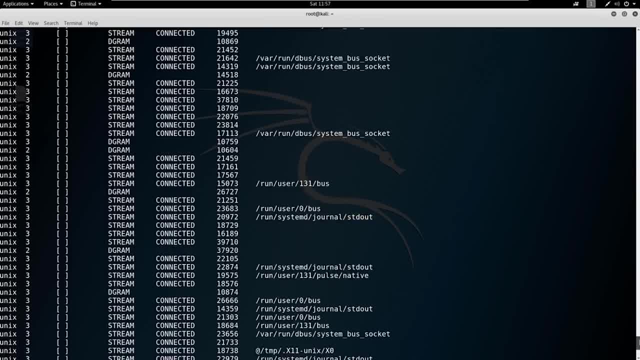 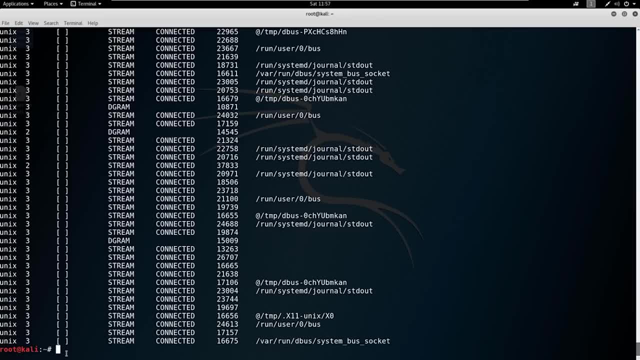 that port being open and and that i am going out with it. so just kind of keep that in mind. these are not commands that you really need to know in depth right now. um, network does come into play when you are doing penetration testing, but we're going to cover these commands time and time and. 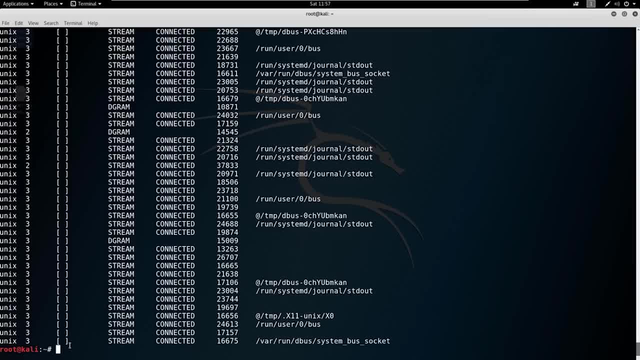 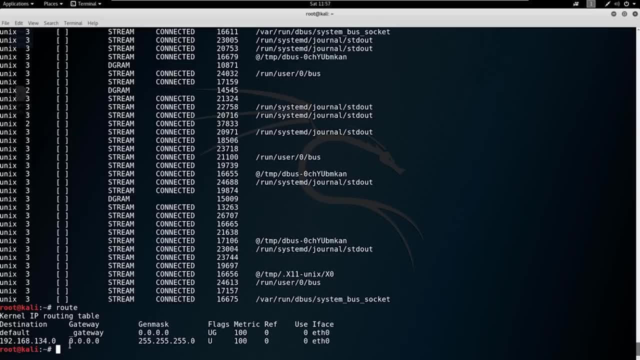 again. i just wanted to give you a very, uh brief introduction to them, okay, and the last command i have for you today is route. so if you type in route, that's going to print your routing table, and the routing table is important because it tells you where your traffic exits, essentially. 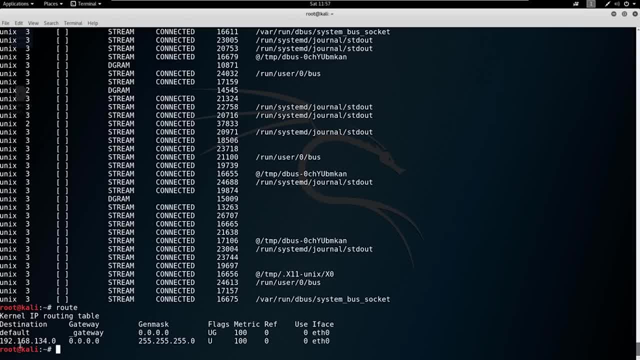 so for this vm my traffic is exiting on 192, 168, 134.0, so any traffic goes out of this 0.0.0.0 gateway in this range, right. so when it goes out this gateway it's doing nat, so network address translation and it's running off. 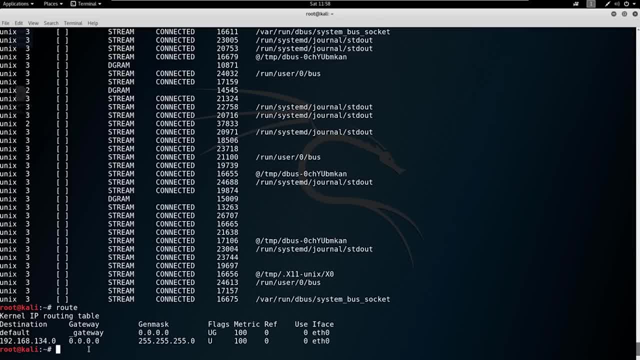 my computer so the best examples aren't here. but it's important to know route as well, because there could be a machine that you're attacking that has multiple routes. so you might see a 134 and a 135, because it has a dual home nick, the meaning it has two nicks inside of it. so it's actually talking to. 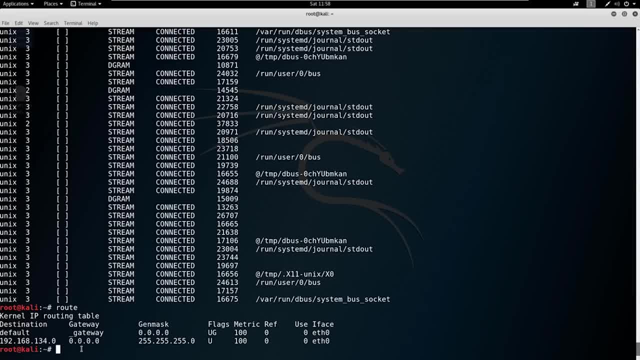 a completely different network that you didn't know existed. so you might have been attacking one network and the 134 range, and then 135 is just out there and this computer can talk to both. and until that point you had no idea. and that's the idea of called pivoting when you switch a network. 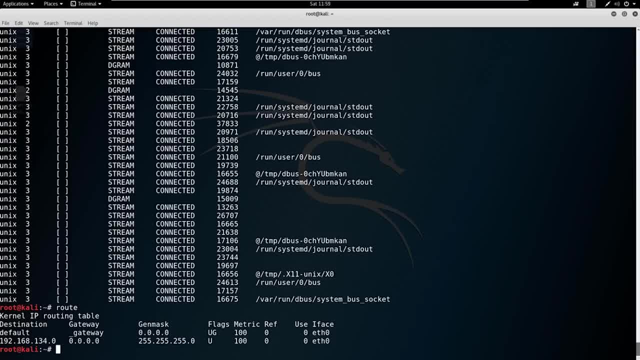 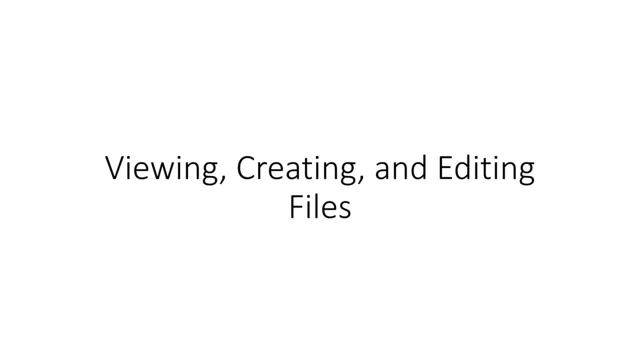 from one to the other, but you're using a machine, so that's it for this lesson. in the next lesson, we're going to talk about viewing, creating and editing files. okay, so viewing, creating and editing files. this section sounds exactly like what it is. we're going. 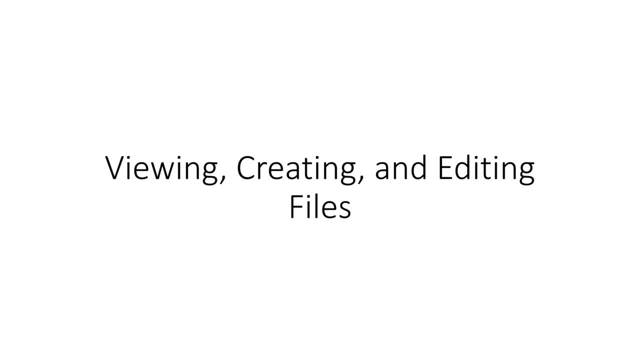 to talk about how to view, create and edit files. mainly, we're just going to be showing how to create quick text documents, but we'll teach you commands that will allow you to do further in the future, as you will see, as we get further in the course and get into scripting. so let's go ahead. 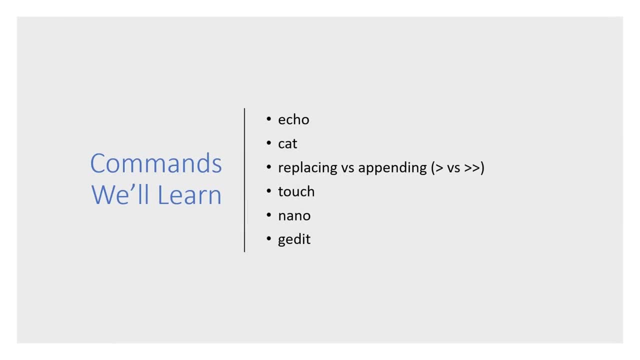 and take a look at some of the commands that we're going to be learning. so, some of the commands that we're going to learn. we're going to learn the echo command, which echoes what we write right back out to the terminal. we're going to command which is going to print out a document. for us it's similar to type in windows. we'll 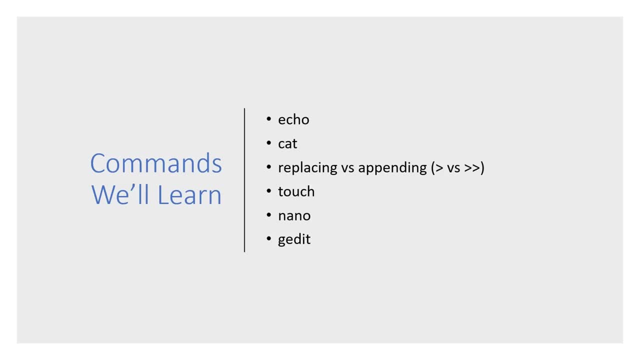 talk about replacing verse appending and which. which function does which and how to do it? we're going to talk about the touch command, which can be used to create a file on the fly. we'll talk about nano, which is a text editor that's built into the terminal, and then we're going to talk about g edit. 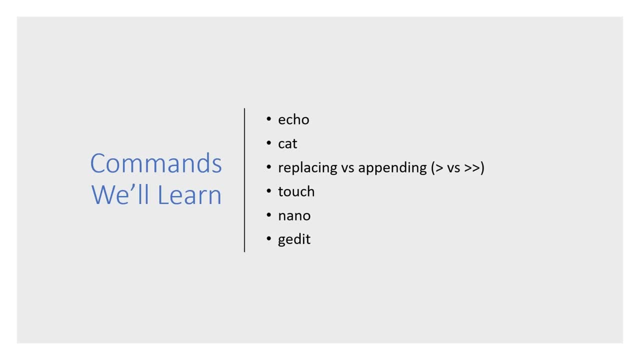 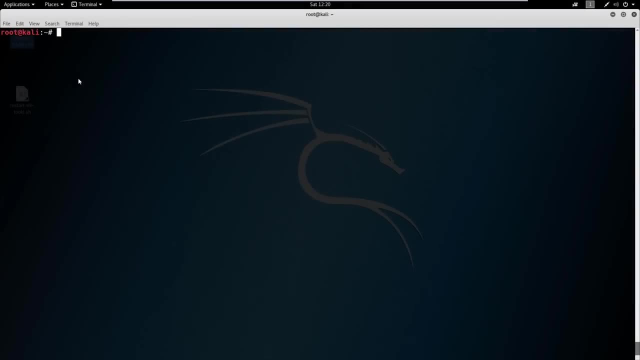 editor, but it is a gui text editor, so we do get a little bit of gui in this lesson, so let's go ahead and dive right in. okay, so this is my second time recording this video. the first time i forgot to turn my microphone on and performed for my cat, so she approved of it. let's see if you approve. 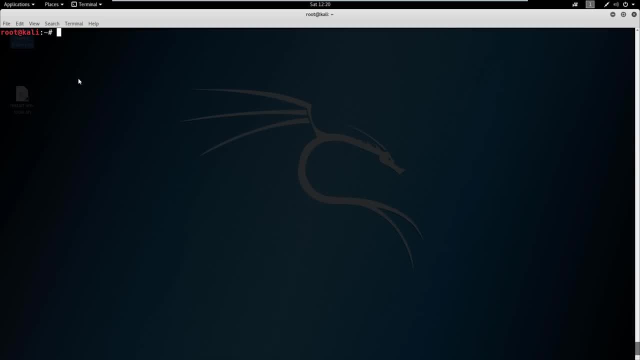 of it the second time around, now that i have a little bit of practice. so we're going to be talking today is we're going to be talking about viewing, creating and editing files, so let's first create a. it we've created, so let's go to the description. there's our 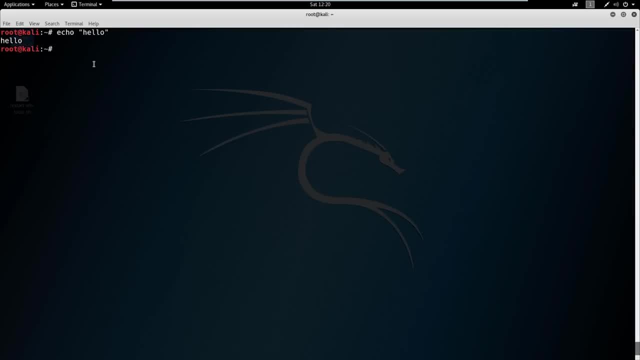 editor and we'll be writing it down. it's called all processes now. so here's how we're gonna do it: we're going to go right to program gear and we're going to type in. we're going to cd comic and we're going to type in preview. soul don't like this, so we're going to type in md comic. 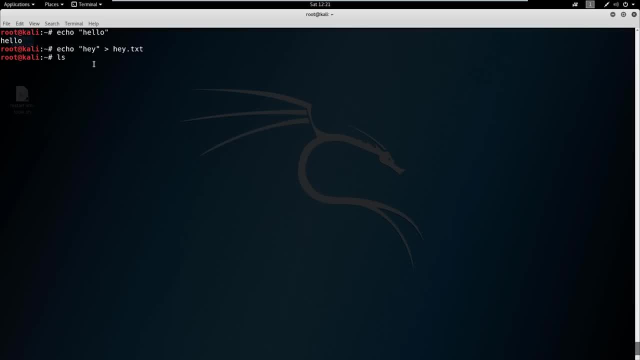 Well, we can look and see that heytxt is here and you can see my files from the previous ones. I'm trying to come up with more ways of saying hello, but we're going to use heytxt here. So if we cat heytxt, all cat does is print out to the screen what is in a file. 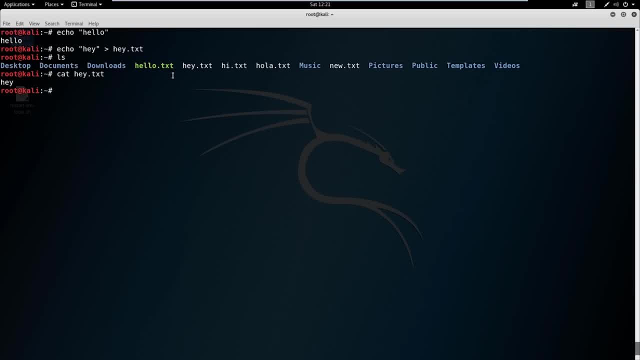 It says hey, Okay. so let's say we want to append heytxt, We can tab up here. What if we just say hey, again, We've got this greater than symbol here and we're just putting it into the heytxt file? 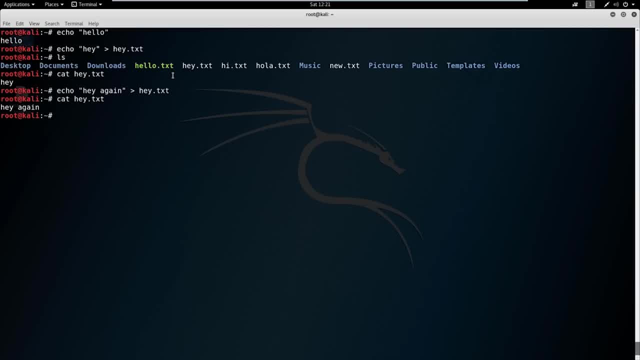 Well, that didn't work, We didn't append it, We actually overwrote it. So what can we use to actually append this here? What we can do is we can say hey, again, again, just to give us something different, and we 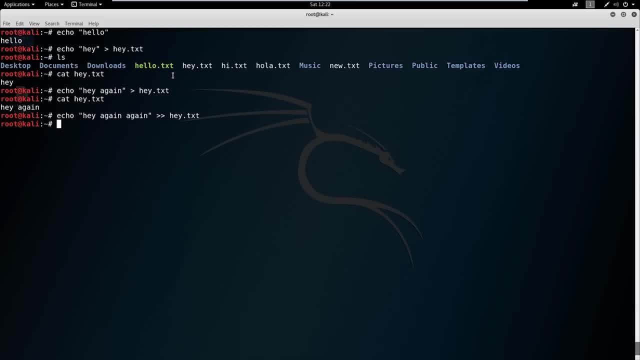 can add a second greater than symbol here. So now if we cat the file, you can see that we actually appended to the end of it. So this becomes incredibly useful when we are either adding stuff to a list- say, we're gathering IP addresses and we just want to combine our lists- or when we're creating. 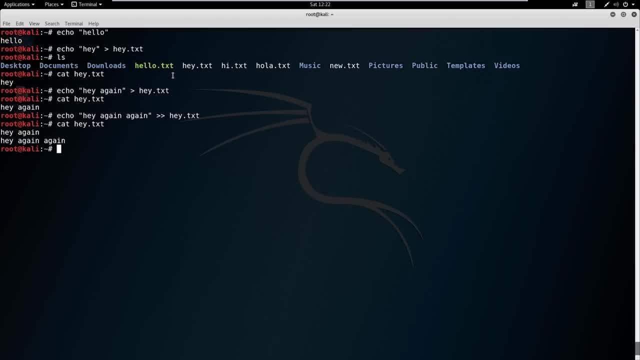 a series of commands Okay And we're going to use those commands to send all at once. We're going to cover that later when we're talking about file transfers in the penetration testing section, where we use a set of commands like this on a Windows machine to actually 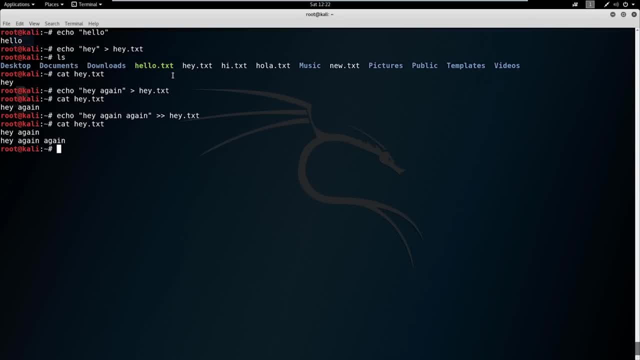 transfer files via FTP. It's just so much easier than typing them all in one by one. We can create a little document and run the document. So this becomes useful when we have a series of commands, and for other reasons as well, as you'll learn as you go on in your Linux career. 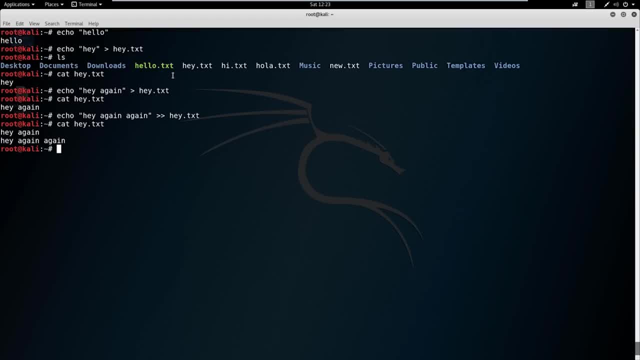 So we've talked about echo and we've talked about cat, so let's talk about some other ways to create a file. We can use something called touch and just say new filetxt, And if we ls, you could see that new filetxt is here. 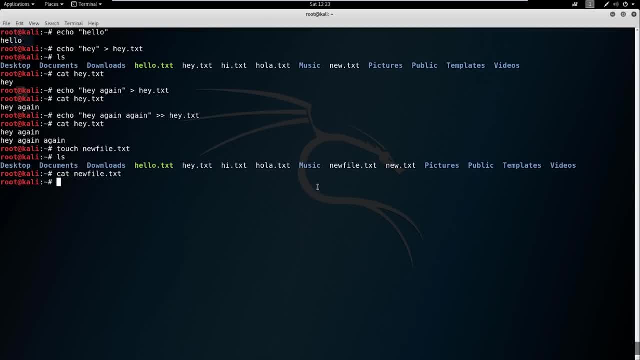 But if we cat new file, there's nothing in there because we haven't put anything in there yet. So there's a few things that we can do. We could use echo and append the file right. We could also use a tool called nano. 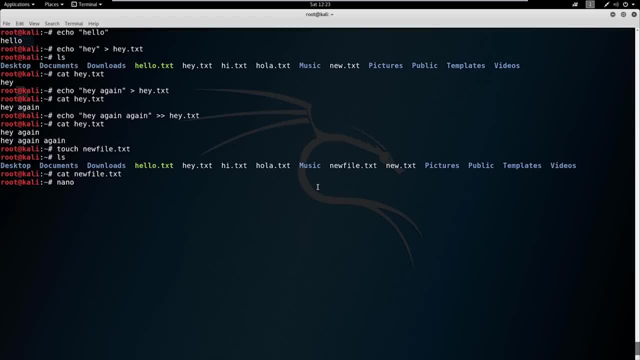 Now, nano is a terminal text editor. There are other terminal text editors like vi and vim. I don't prefer those. personally, I like nano the most. Some people have their preferences, So I encourage you to play around with any of them as you wish. 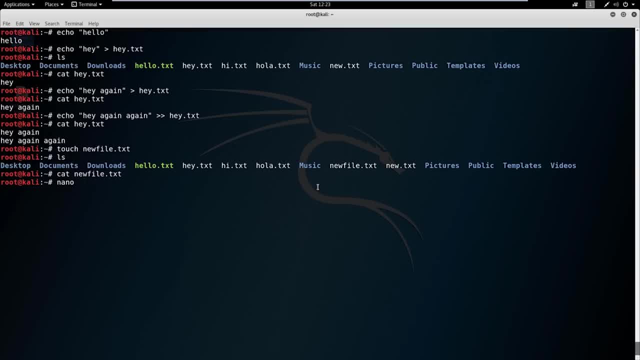 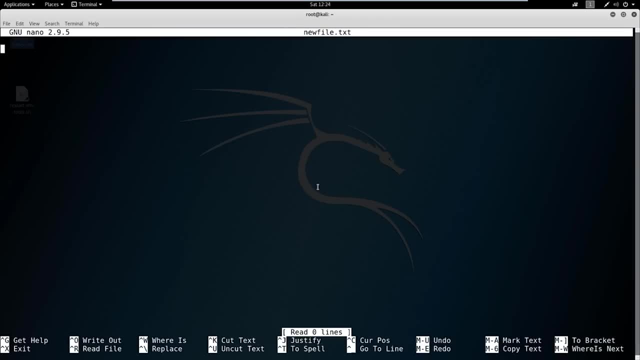 Vi and vim are the other two. But for this course we're going to be using nano. So if I say nano, new filetxt, I could type whatever I want in here, And we're going to be using nano a lot to create scripts, to create Python scripts. 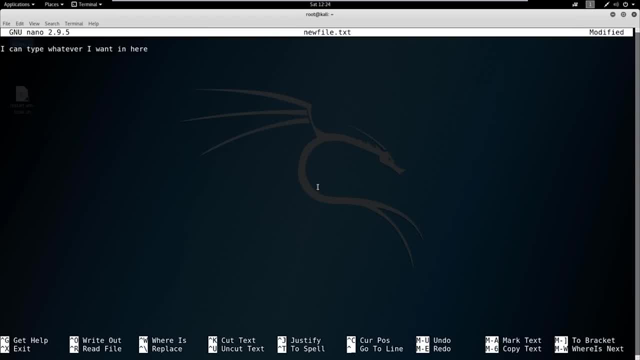 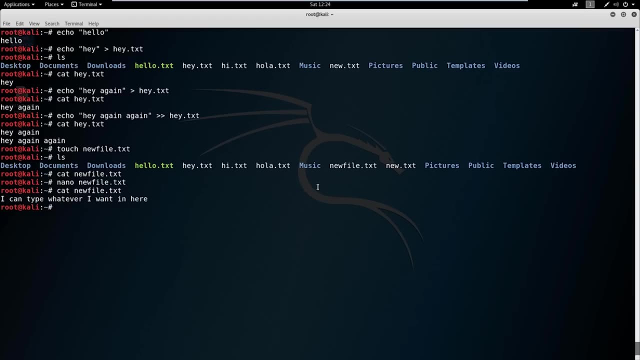 and to edit shell code as we get into a little bit of exploit development. So I'm going to hit control X, I'm going to hit Y for saving And then we'll save it to new filetxt. If we cat this now. it says: hey, I could type whatever I want in here. 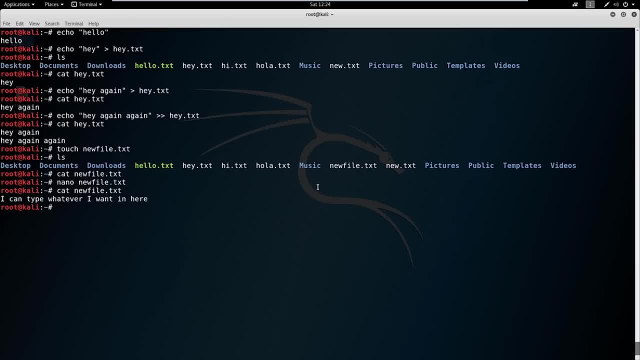 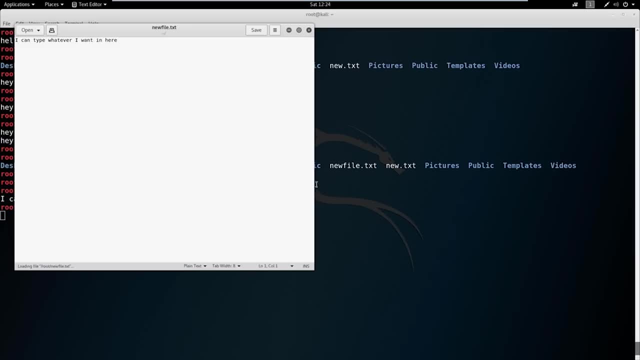 So that's one way of editing it. Another way of editing it: It's using a graphical interface, So we can use gedit and say new file. And if you don't like using a terminal, you're more than welcome to use gedit here. 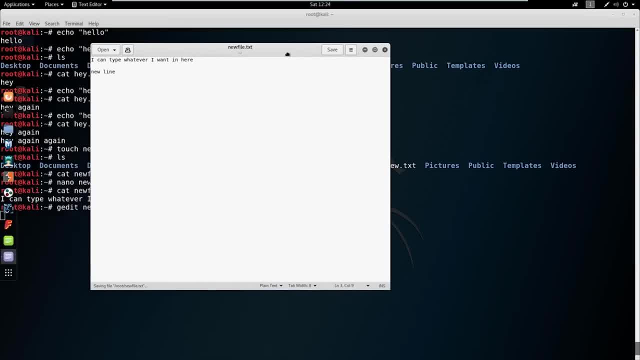 Just type in new line here and save it. And I like using gedit. It's a lot cleaner because I can highlight and delete. I don't have to use my keyboard to navigate around like I do in the terminal. So if you have the option to use gedit, for sure. 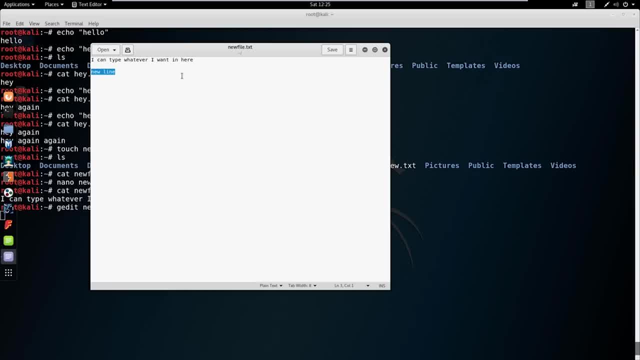 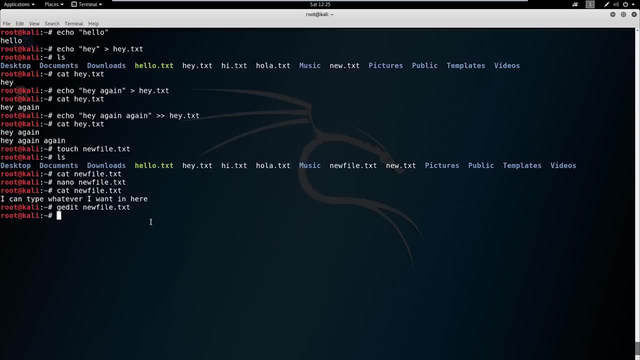 But sometimes you're going to be on another machine That's not your own or is headless and doesn't have a GUI, that you're going to have to use nano, So get comfortable using both So we save this. Let's go ahead and cat it out and see what happens. 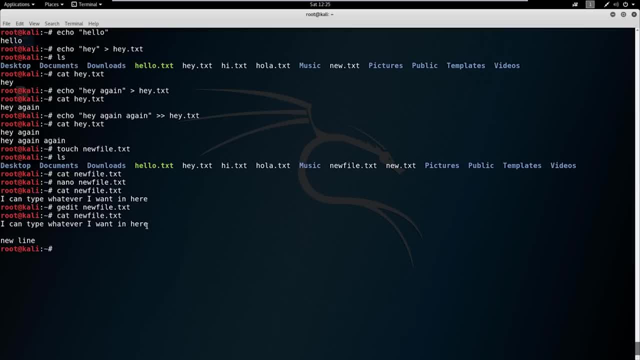 Okay, You can see that the new line is in there. So really that's the overview that I wanted to cover. So just know that you can create files pretty much using echo touch, and actually you can create files using nano as well. 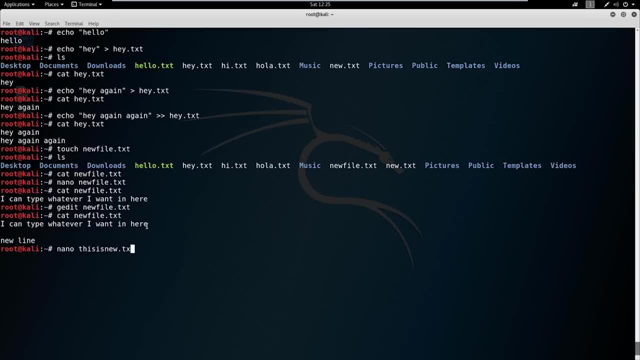 If you say nano, This is newtxt. I'll just say hello, control X, save it, do LS. You can see this is newtxt is right here. So you can use all of these tools in different ways to create files. 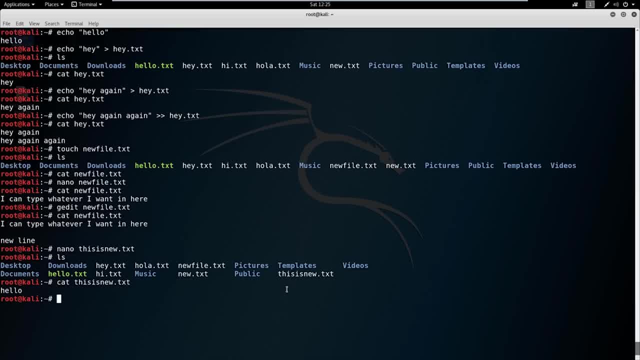 It's completely up to you how you want to do it. Personally, when I'm creating a file, I use nano and I just create a new shell script, Python script, text document- that way. Okay, You can also do it using G edit as well. 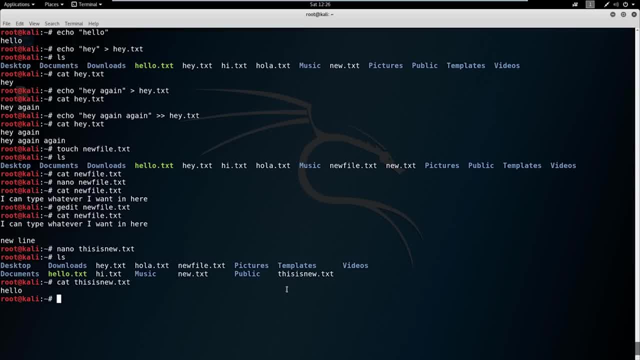 So just know that we're going to be using these a lot and try to get comfortable with these, And from here we're going to be moving into controlling Kali services. So we're just going to briefly talk about what services you need running on boot and 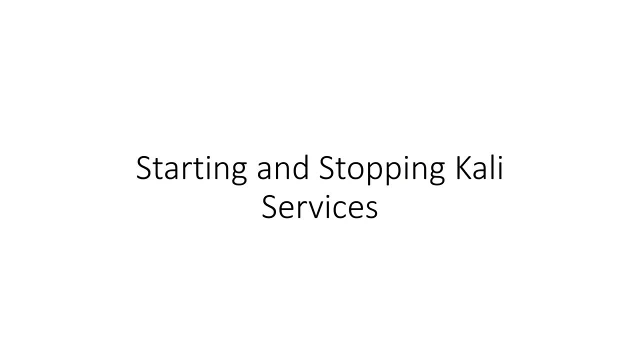 how to do that. All right, In this video we're going to be talking about starting and stopping Kali services. Let's go ahead and just take a quick look at the commands we're going to learn. So not a lot of commands in this video, only two. 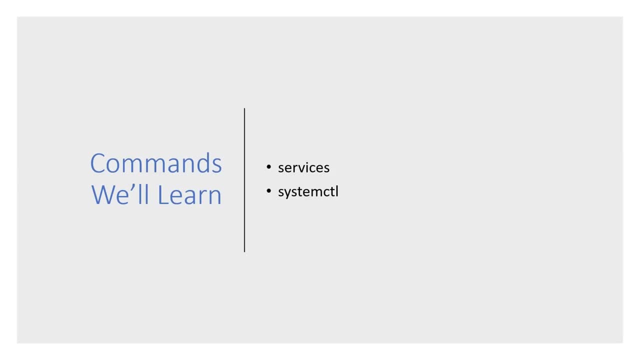 We're going to talk about the commands. We're going to talk about the service command and the system CTL command. So the service command deals with services. It's going to allow us to start and stop services on the fly, And the system CTL command is going to allow us to enable or disable services so that they 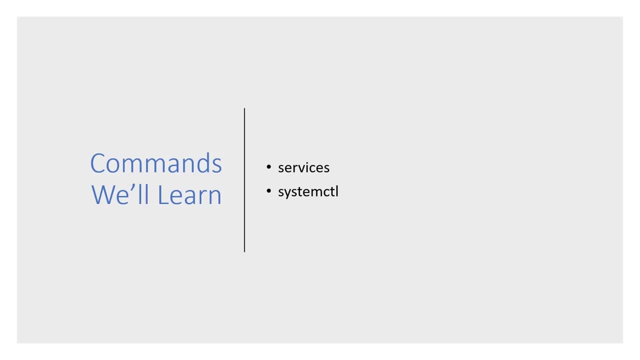 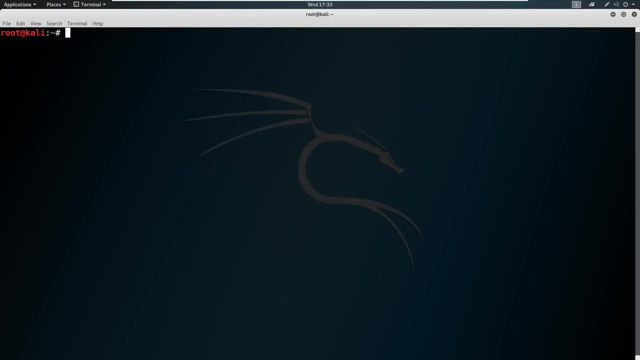 load up on boot or do not load up on boot. So let's talk a little bit more about services and look at how these commands can be useful for pen testing. All right, So let's talk about starting and stopping Services. So when we're in Kali, there are a couple of different ways that we can start and stop. 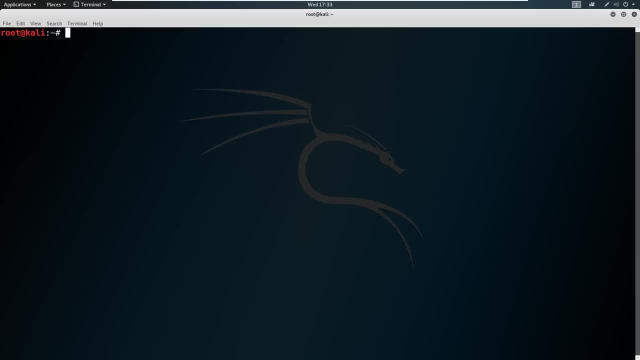 services, And when I talk about a service, I'm talking about something like a web server or SSH or maybe a SQL database. So when we cover this video today, I'm going to show you a few different services and how to start them and stop them. 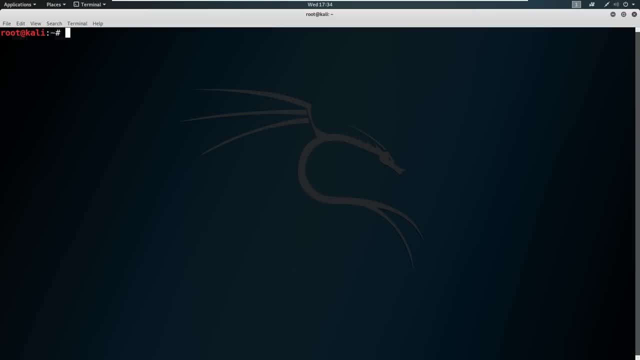 I'll show you how to start them permanently on boot and we'll talk about which services to keep on boot, which services are important to just start when you feel like that, just starting them, or when you need them, et cetera. 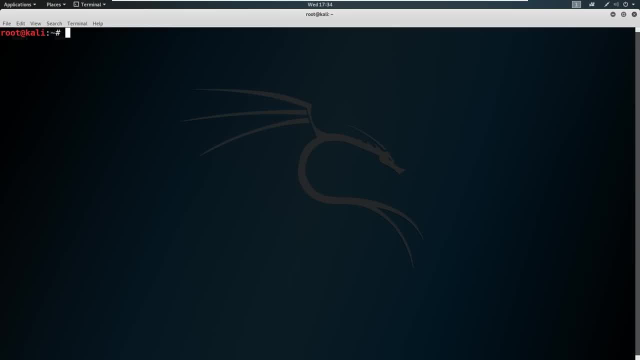 So let's start with our first service, which is going to be Apache two. Now, Apache two is a web server, So let's go ahead and do a proof of concept. first, Let's start with the command that we learned in an earlier video, which is: if config, I'm 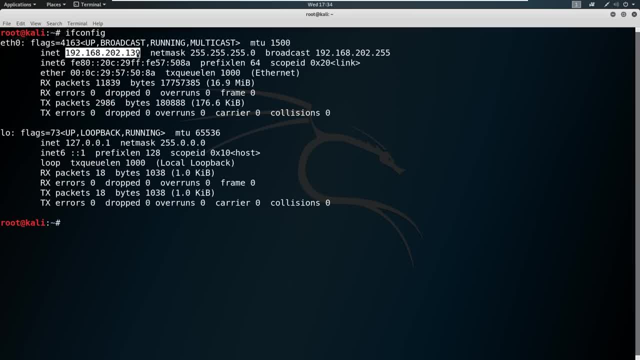 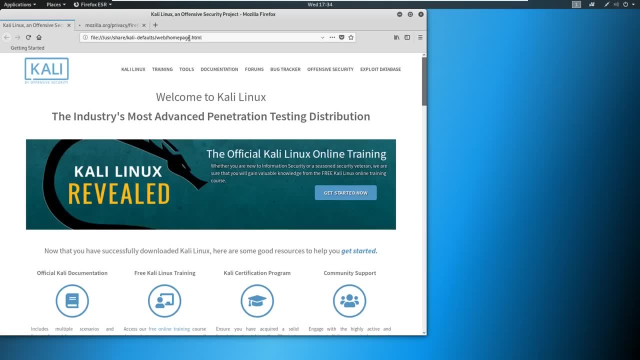 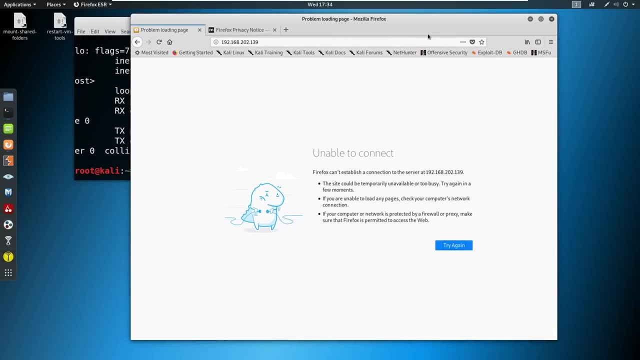 going to grab our IPV4 address right here And I just want to copy this. Okay, So I'm going to go out to a web browser over here and we're just going to paste this address. Now you'll notice that it says it's unable to connect. 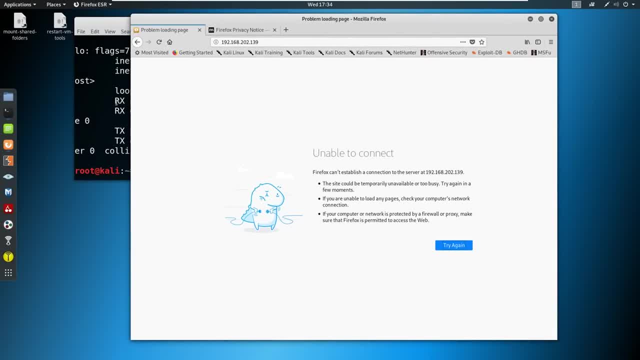 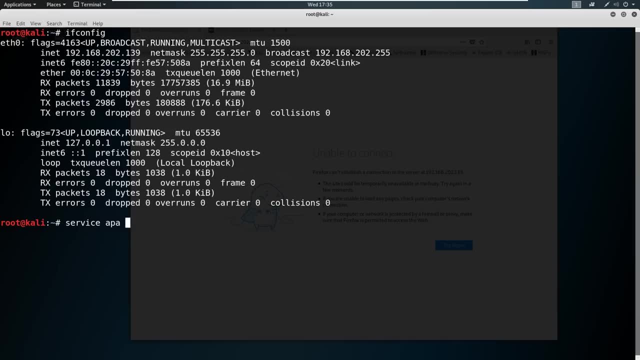 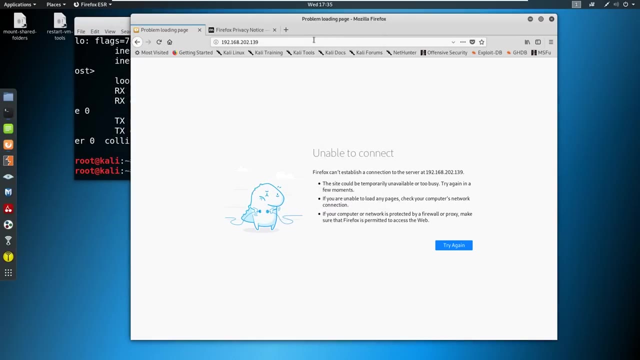 This is expected here. We're not running a web server. Now let's go back in here and let's just say: service Apache two- start. Okay, Looks like it went through. Let's go ahead and hit enter again, And now you can see that Apache two Debian default page has been loaded. 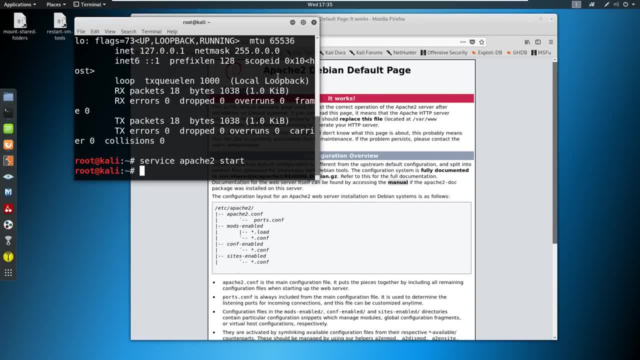 So what has changed? Well, when we boot our machine, this Apache two service is not running by default. So if we want to run a web page, then we actually have to start up the service for it to work, As you just saw here. 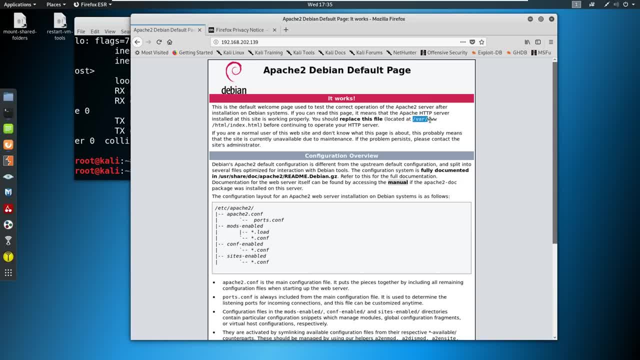 Now you could see that if we want to add files or replace files here, well, we're going to have to edit the VAR wwwhtmlcom. I'm going to go ahead and hit enter again, And now you can see that Apache two Debian default page has been loaded. 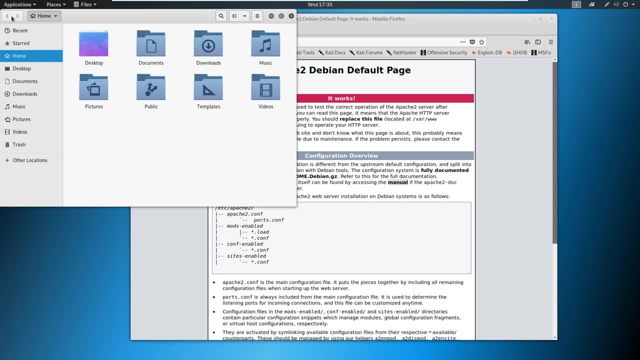 We've got a VAR wwwhtml folder. So if we come out here and we go into other locations computer and then we go into our VAR wwwhtml, you'll see that the indexhtml page is here. So if we actually wanted to maybe host a malicious web page and have it point back to us this: 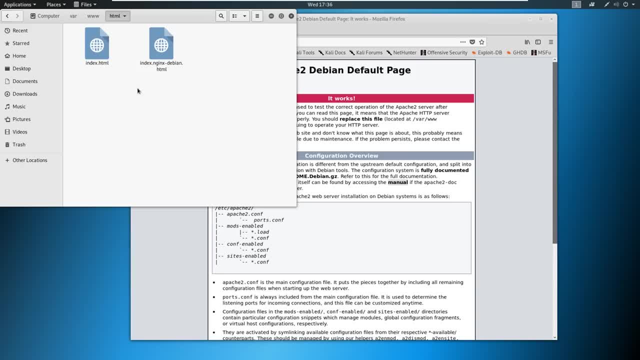 is one way we might do it right here. If we want to serve up some files, say we have something that we want to upload to a machine that might be malicious, or a file that we want to transfer to somebody else or download on another computer, It doesn't. 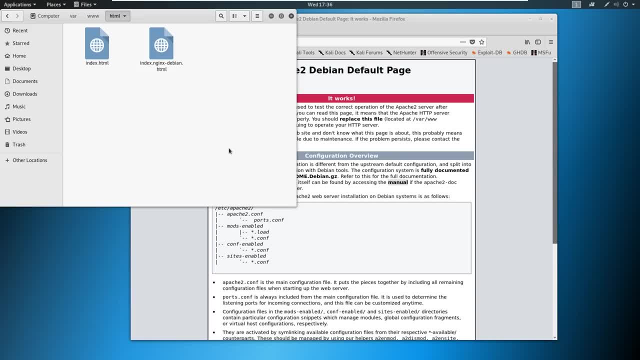 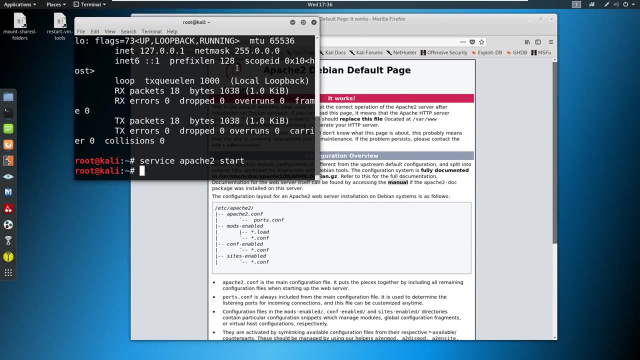 have to be malicious. We could host that file in this folder here. Now. that is fine. This is one way to do it right. You could put your files all in one location. But it's not my favorite way. It was my favorite way when I first got started. There is a much easier way now, and I will show. 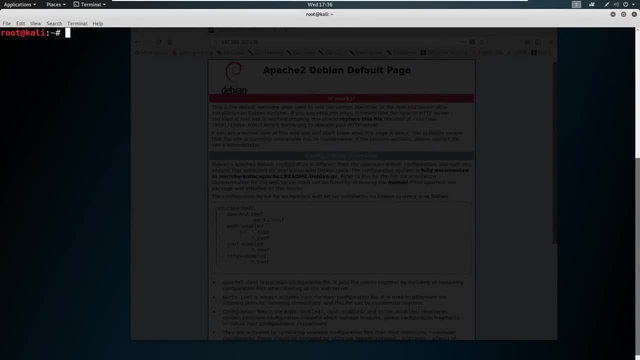 you how to do that. So let's go ahead and type LS. you'll see we have no documents here. So I'm just going to echo hello into hellotxt And then have that hellotxt here. Now what we can actually do is we can spin up a web server So we can just say Python dash M for module and say: 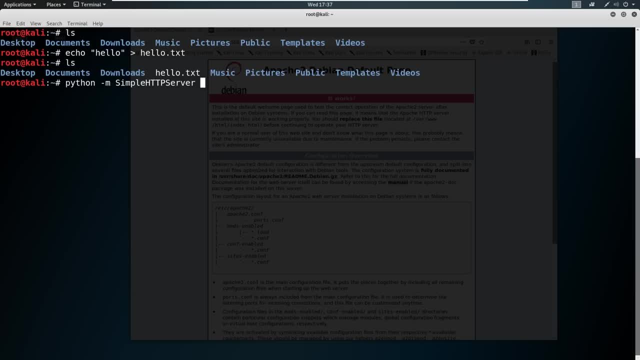 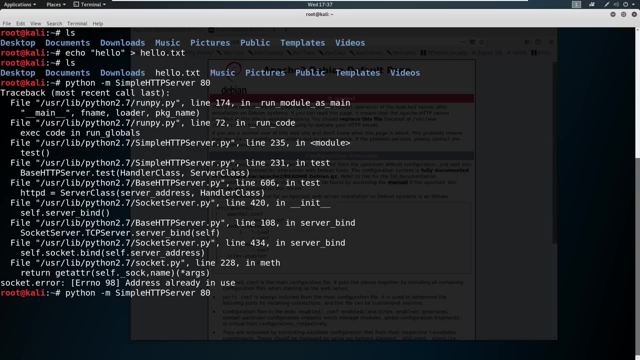 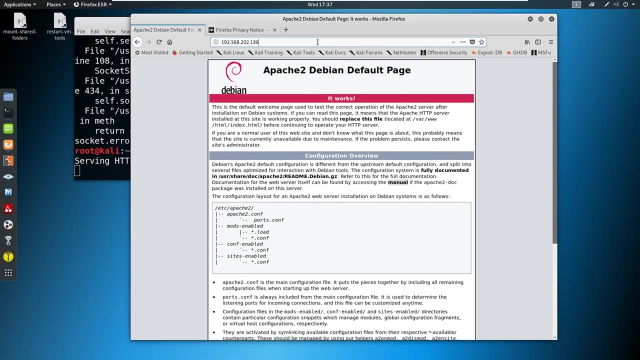 simple HTTP server. you can auto tab it And then say 80 for the port. Oh, 80 is already in use, So let's just give it 8080.. 80 is in use from the Apache server at the moment, So instead let's look at what happens, So let's just call it. 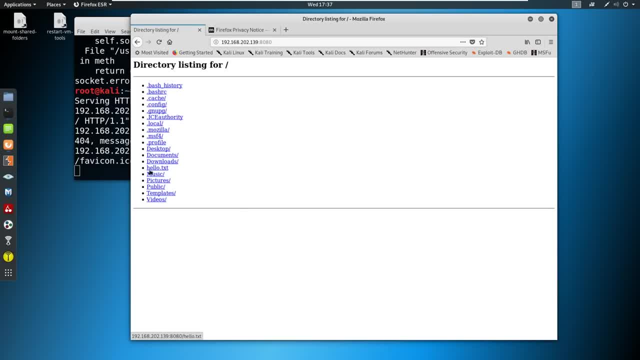 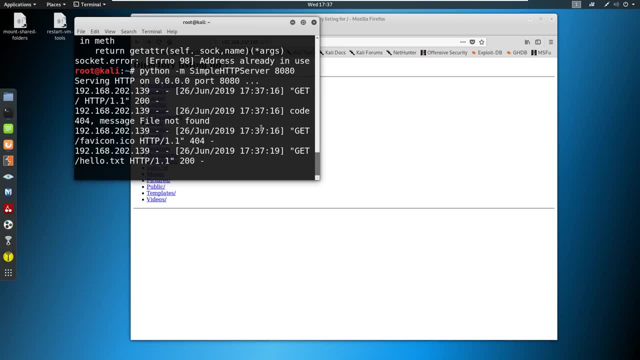 out at 8080.. And you can see here that I can go to this hellotxt and actually get the file. I have information in real time whether or not that file was captured And overall this is just a web server that's so easy to spin up. I can put it in the directory that I want it to. 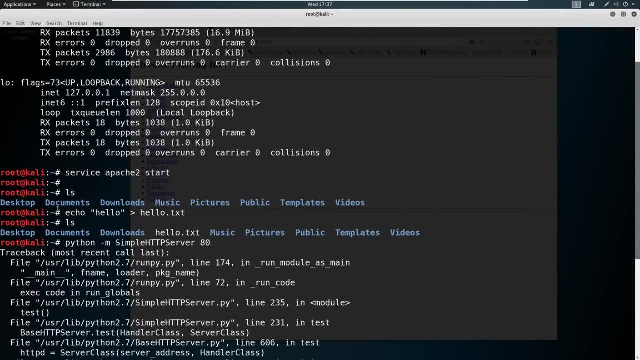 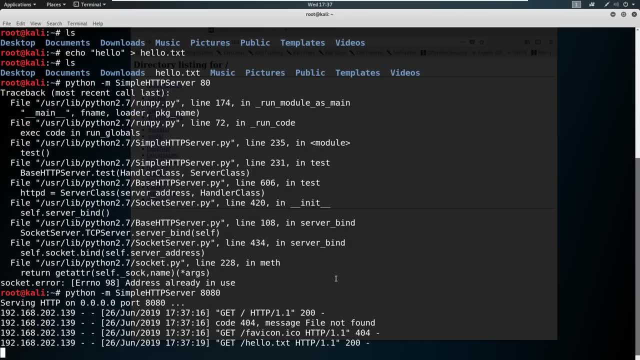 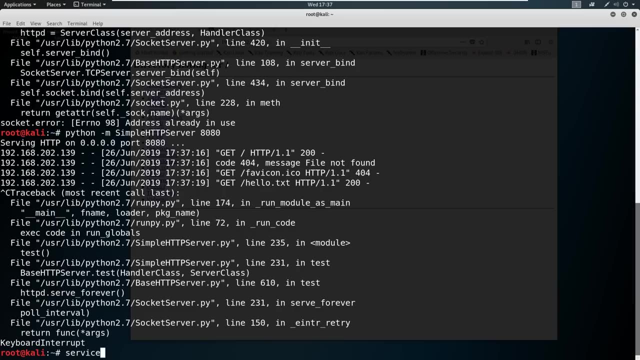 So if I wanted to serve my desktop folder, I would navigate to desktop and then spin this, this Python module, up. I don't have to put everything into a var www folder And it just makes life really, really simple. So just proof of concept: we can do a service Apache to stop, And we can. 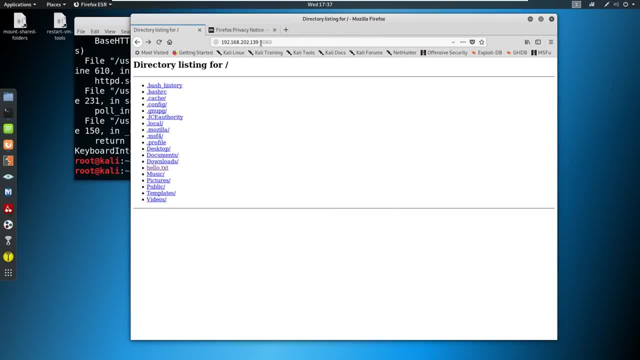 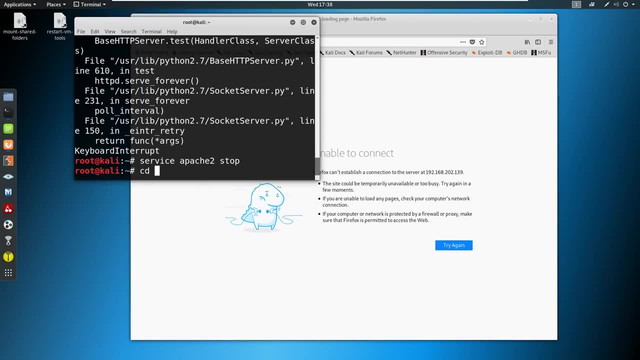 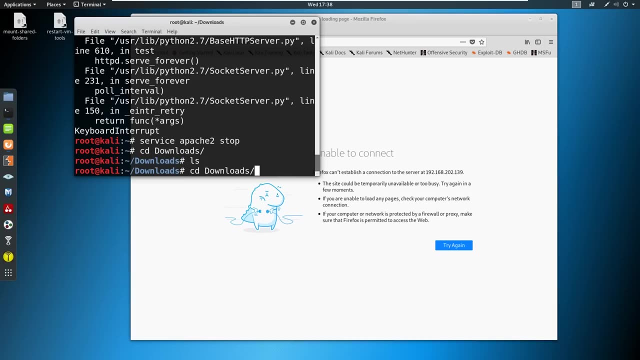 come back and make sure that that web server has been stopped. by going here And refreshing- and I could see that it's gone. We can CD into something like downloads. We say LS, there's nothing in here, So we can tab up a. 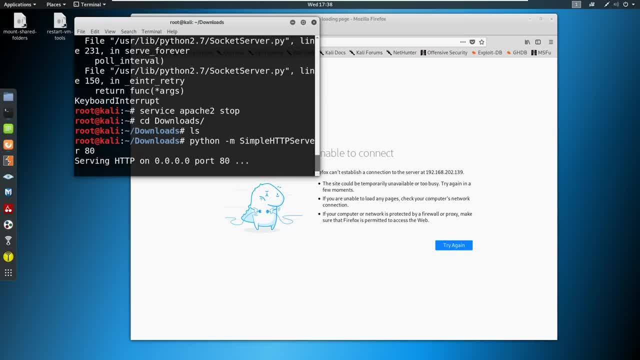 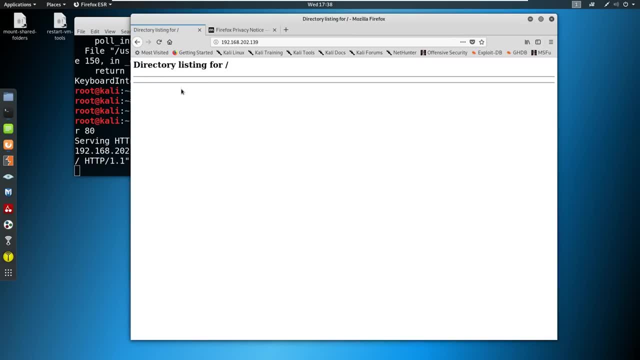 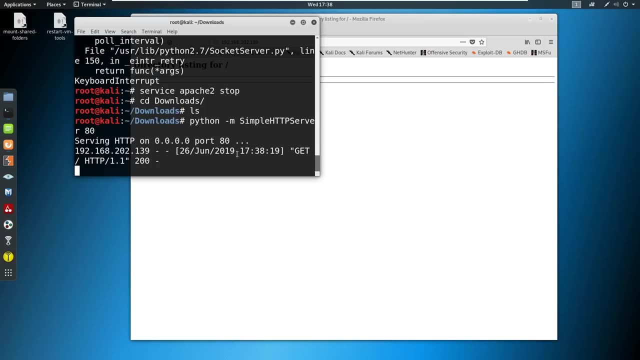 couple times And just serve up port 80. Now, because you can see it's not in use anymore And come back here, Refresh, you can see there's nothing in the directory listing because there's nothing in the folder. So this is just an easy way to spin up a web server. I think it's much easier. 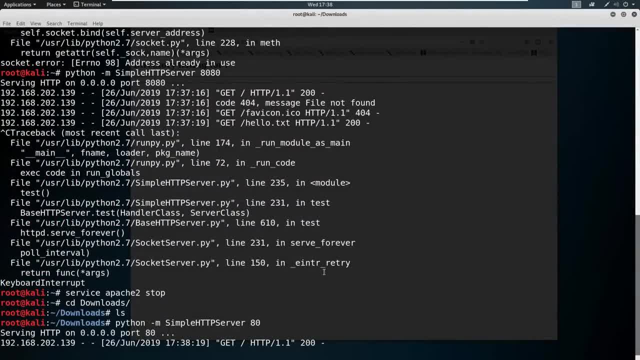 than Apache two. I'm showing you both because I like to give alternatives, But using Python, moving forward is a great, great feature. My challenge to you is to look up how to spin up a FTP server with Python. So I won't get redundant here. I do have future lessons and other courses that talk about this. 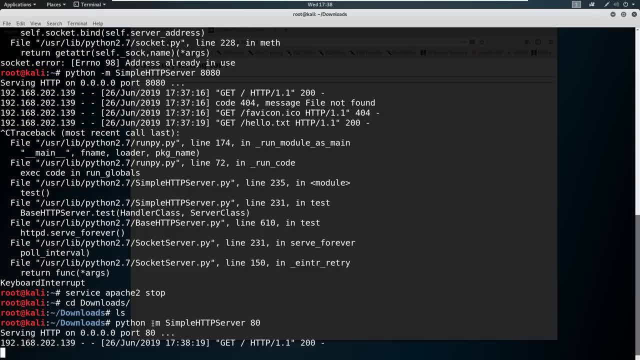 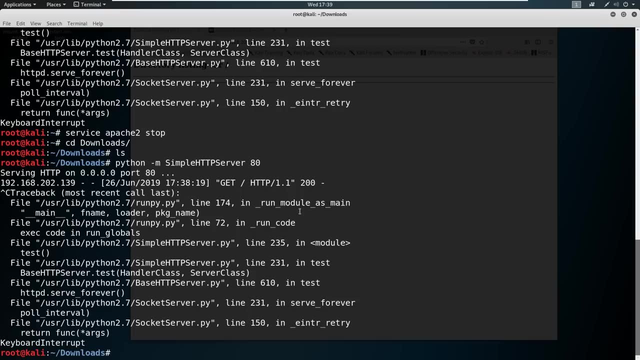 But if you want to challenge yourself to figure out how to spin up an FTP server, that's my challenge to you. There's a module out there that you can download quite easily and spin up your own FTP server. So let's go ahead and Ctrl C and we're going to close out of this. And now let's talk about spinning up a service permanently. So let's say that we just had the Apache two running and then we rebooted the machine. When we reboot our machine, Apache two is not going to be online because we're only doing a service start. it only holds during this session. Once we reboot, that session is gone, that service is gone. So if we want to keep something online the entire time, what we can do is use system C. 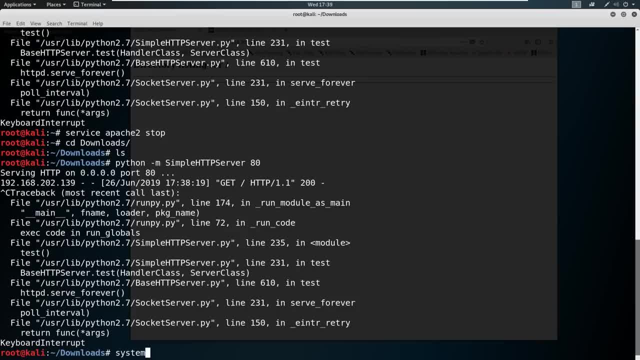 TL, So we can say system ctl enable or disable if you want to disable something. And, for example, we could say ssh. Now I'm not going to hit enter here, This is just an example. But let's say that we wanted to have an SSH available on our machine So we can SSH into it. we are opening up SSH for this feature here. Okay, let's say that we want to have a. 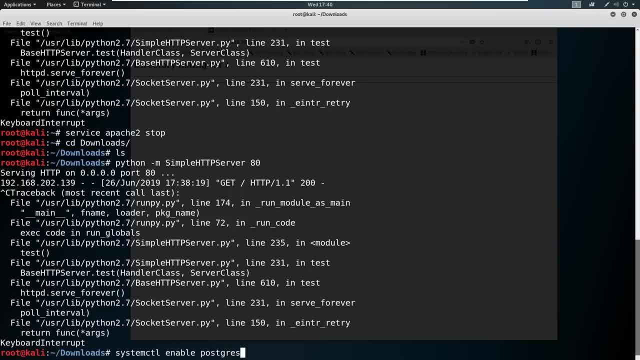 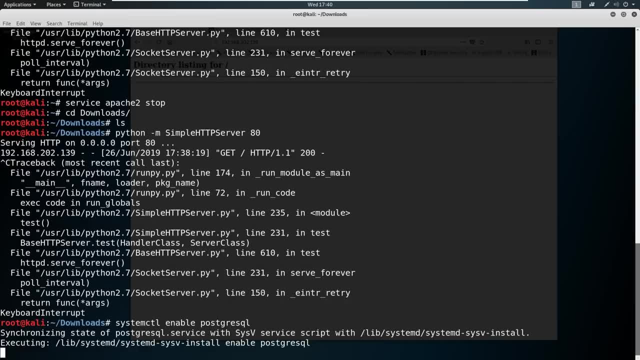 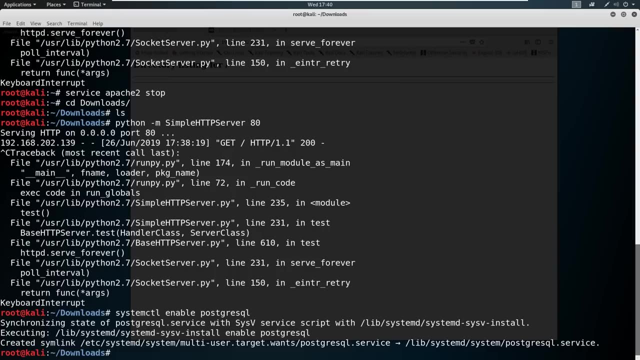 server and this is one I do you to hit enter in. this is going to be a database, right? This is a PostgreSQL. So we're going to say: systemctl, enable PostgreSQL. And we have enabled that. So now we reboot, this PostgreSQL will load every single time. Now why is this important? Well, this is important because 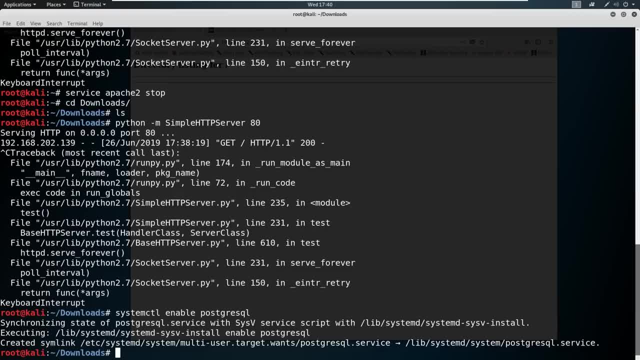 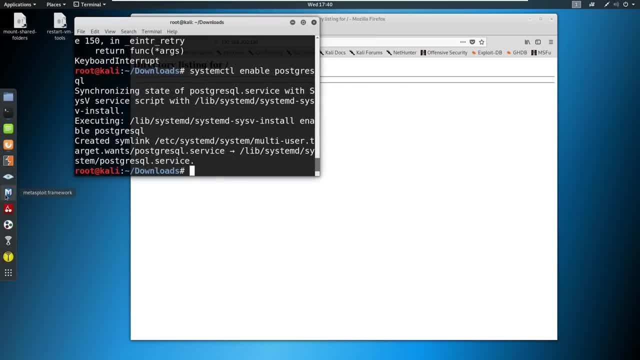 it's going to allow us to run Metasploit and have the PostgreSQL database running when we boot, So it doesn't have to take the extra time to load it. If we come over here, we just click on the Metasploit framework. Now PostgreSQL is working And it says database. 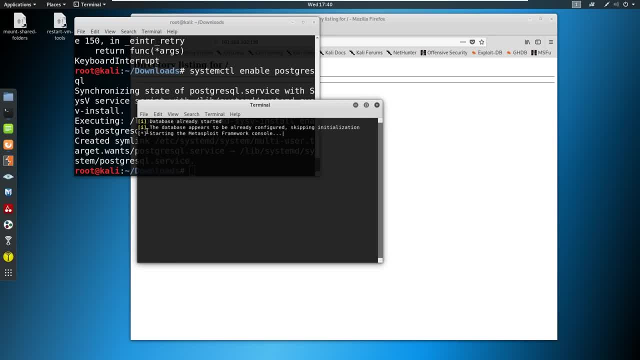 already started, So it's already configured. it's going to skip initialization, it's going to go ahead and get right into it, So it just saves us a little bit of time. Metasploit can take some time to to run And I think that if you continue on- I know if you continue on with being a pen tester. 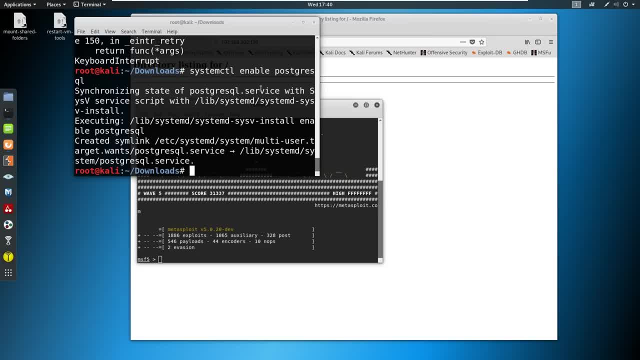 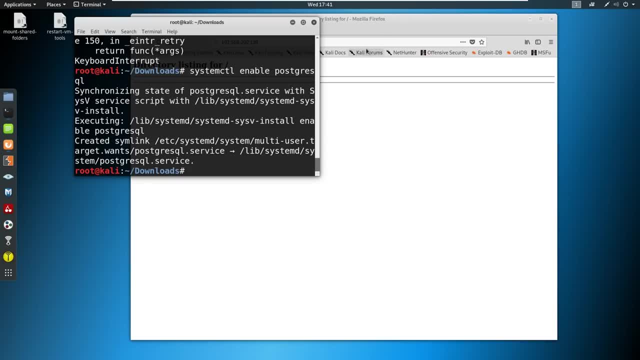 you're definitely going to be using Metasploit quite a bit, So this is just one feature that, if you're going to be using it, it doesn't hurt to have it enabled on your system boot. Now, if you feel that you want to have Apache two on boot, you can go ahead and do the same thing with. 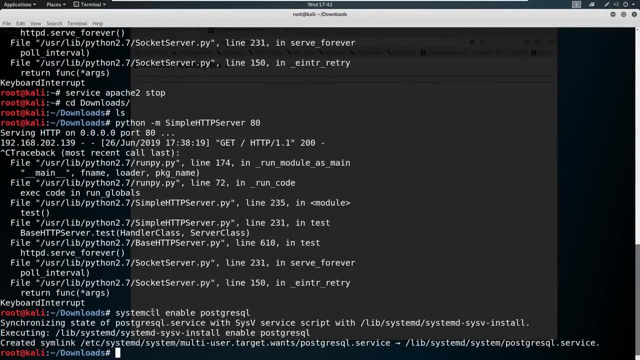 the system enable, systemctl enable, But the only one that I recommend putting on is this: systemctl- PostgreSQL. Okay, so that is it for this video. In the next video, we're going to be talking about installing, how to install things from GitHub and how to install the PostgreSQL database. So if you 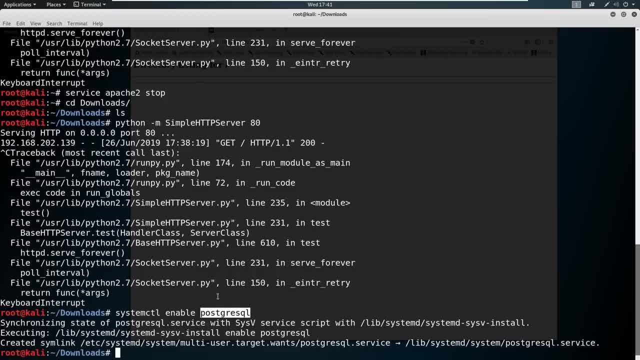 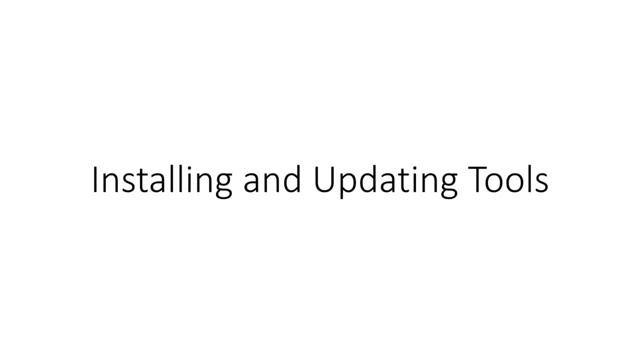 want to install using apt get. so let's go ahead and move right into that video. All right, welcome to the pen ultimate video. we are going to be focusing on installing and updating tools. So let's look at our agenda. So what are we going to learn? we're going to learn how to install updates. 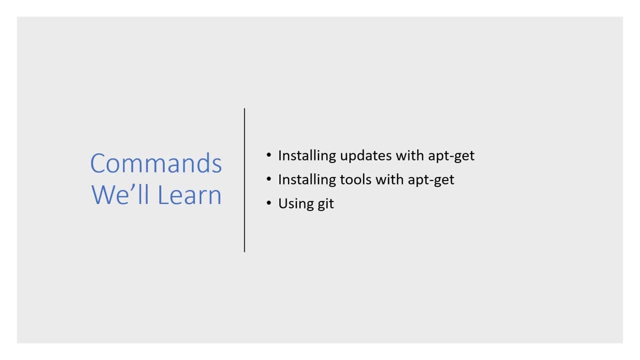 for Kali. So we're going to learn how to install updates using a tool called apt get, And we're also going to learn how to install tools using apt get. Specifically, we're going to be installing a tool today called get. we're going to be using get then. 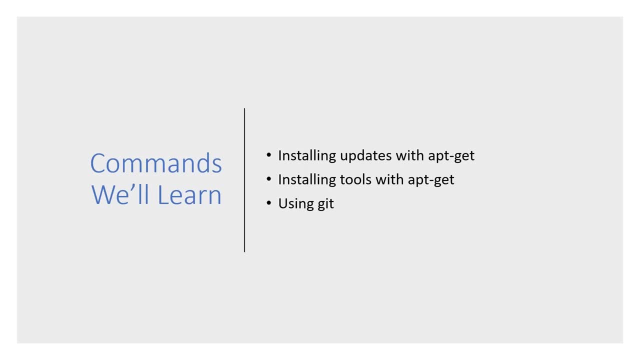 to clone from a website. So sometimes when we have a tool that we want, it's not always in apt get, it's not in the repository. So we're going to actually have to use GitHub and maybe use a tool called get to download tools or other items from GitHub. But this is just going to be one example. 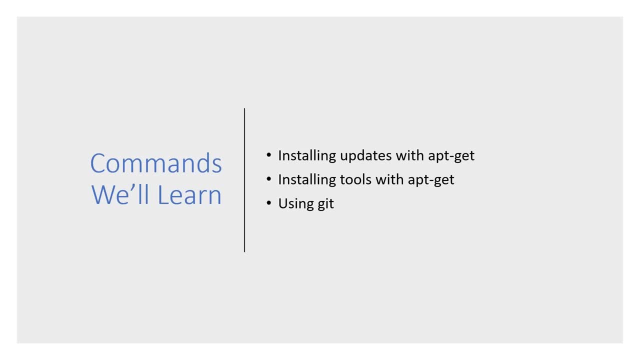 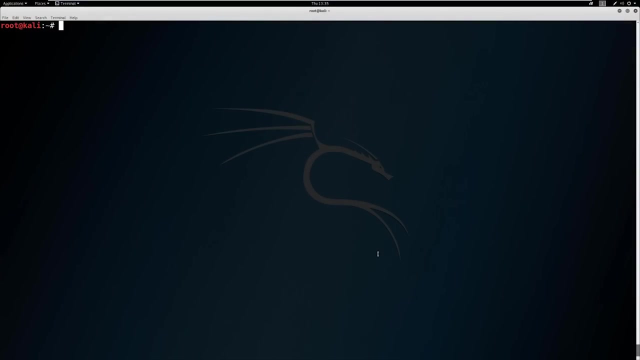 but it's a very, very common example that you may have to do as a pen tester, So let's dive in and take a look at how we can use these commands to install tools and update tools. Okay, so one of the important things you need to know is how to not only install files on 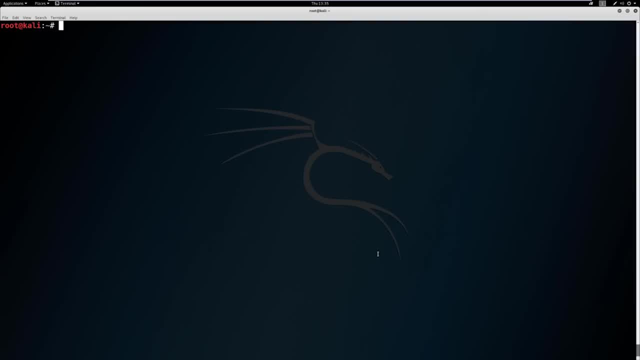 your computer, but also how to install updates on your computer. So for Kali, since it's a Debian base, we're going to use something called apt get, And the first thing I'm going to show you is how to install updates. 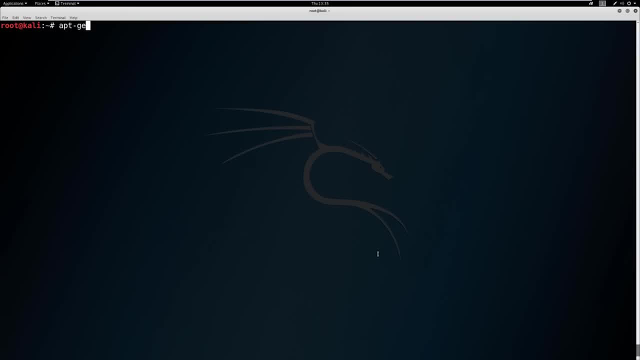 So if you don't use the GUI and you want to use terminal, is apt get update, And then we'll do, and apt get upgrade. Let's go ahead and just hit enter on this. Let's explain what it's doing. So the 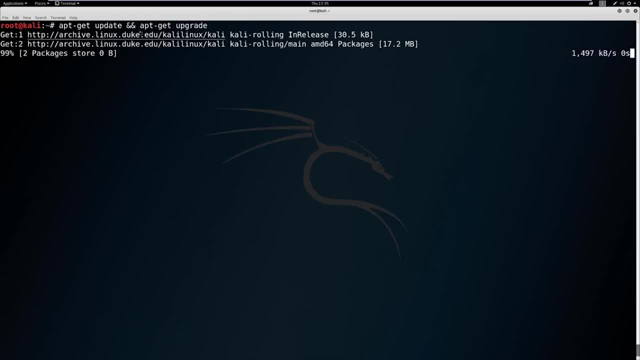 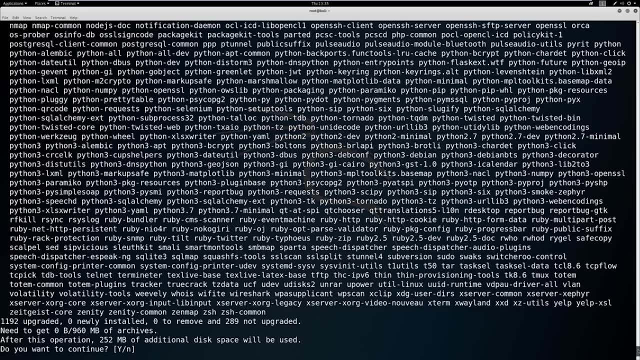 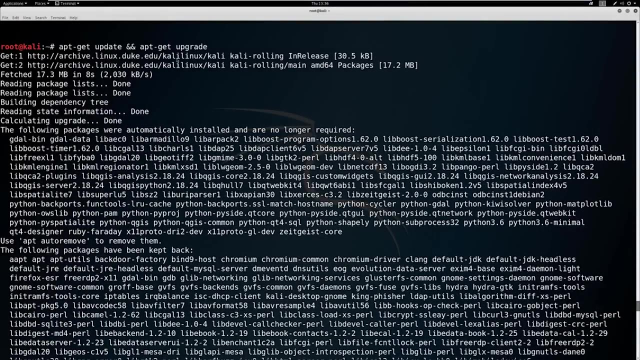 first command here is saying: apt, get update. So what we're doing is we're looking through packages. Now, these packages are predefined, they're repositories, And what it does is it says: okay, I'm going to check packages here For updates, And it went through. looks like they use archive Linux, Duke IDU. they check these packages. 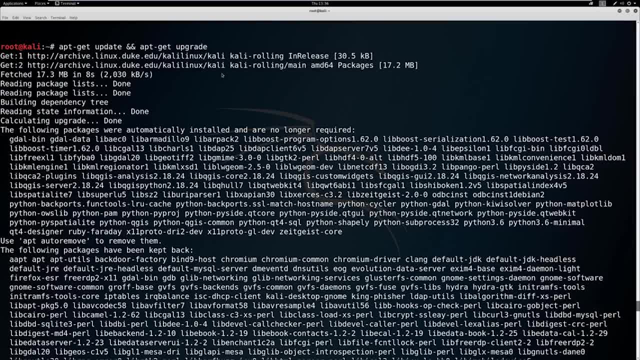 here And they update the packages And then, once they update the packages, they run this command. So, basically, the and command is: you're going to do something as well, right? So first we're going to update and then we're going to upgrade. So, based on what's in these packages, it's going to say: 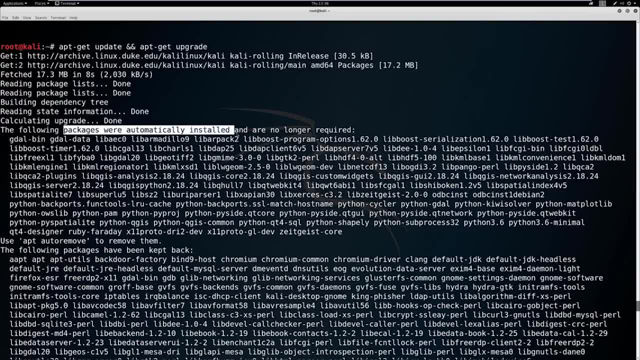 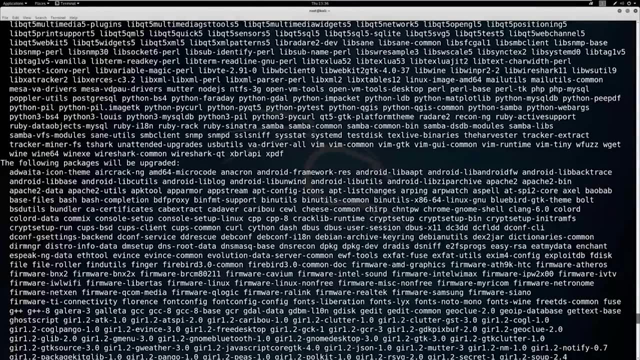 okay. well, we know the following packages were automatically installed in, no longer required, So all these things, right here, they're going to be removed. And then the following packages have been kept back: Okay, they're fine, They're not going to uninstall those. And then we have the following packages that are going: 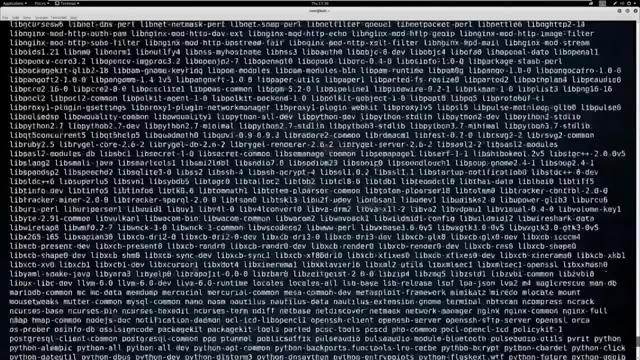 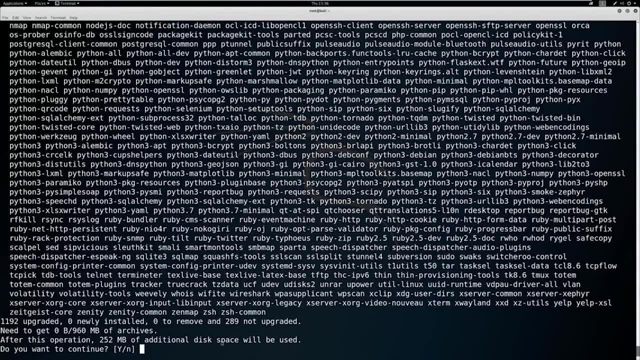 to be upgraded. Okay, so it's a long list that needs updating. And then you come in here and you say, okay, well, it needs 252 megabytes of additional disk space to continue. You could hit enter for yes and they'll automatically start upgrading. so if you want to update your machine to its 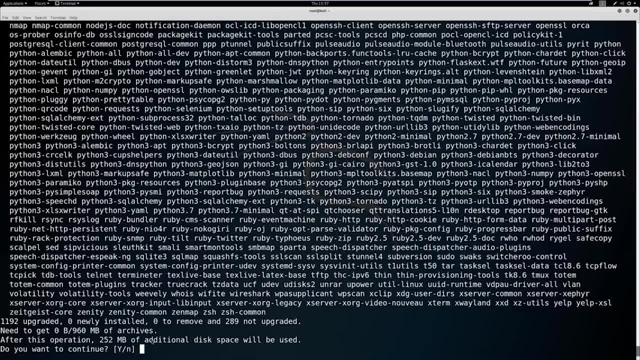 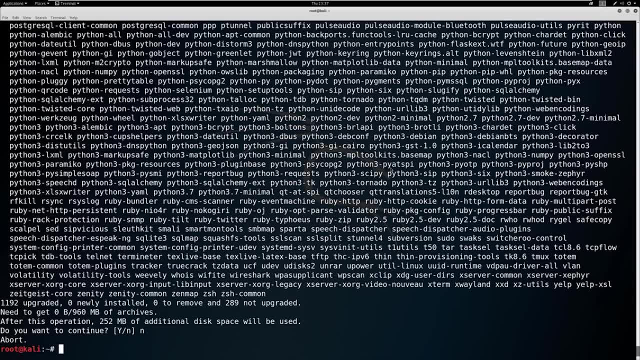 newest and best form. you can go ahead and do that. I'm gonna go ahead and just hit no on this guy, okay. and now it's also important to know how to install files, so I'm going to show you two different ways. one way is through apt-get, similar to what we just did, and the other way is going to: 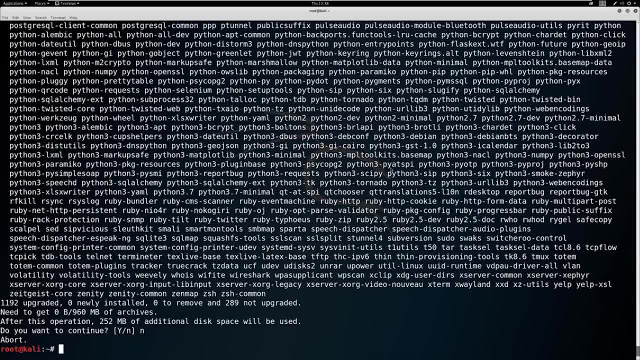 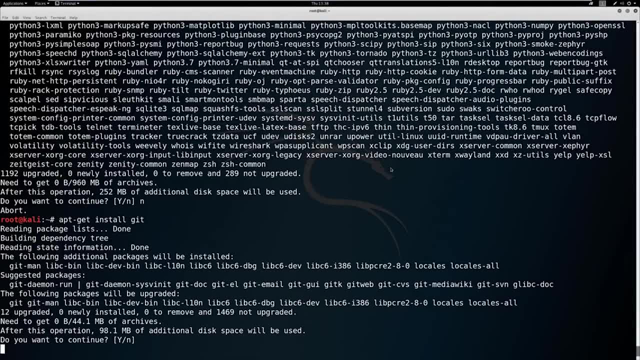 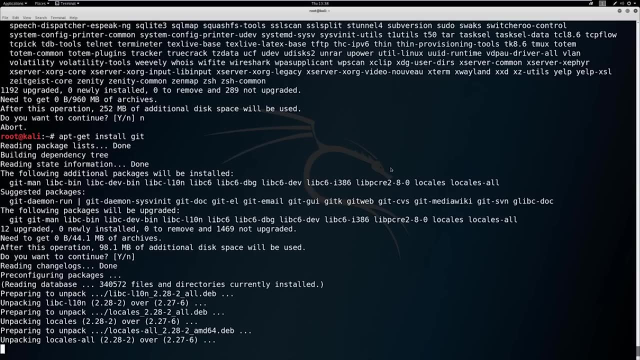 be through git itself, so let's go ahead and install git. we're gonna use apt-get to install git, so it'll look something like this: we'll just say apt-get- install git and we'll hit yes on this. and another way to do this is to add a dash Y at the end of this, so you'd say: apt-get- install git. 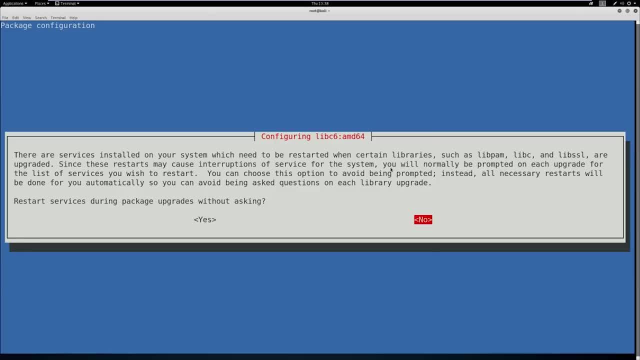 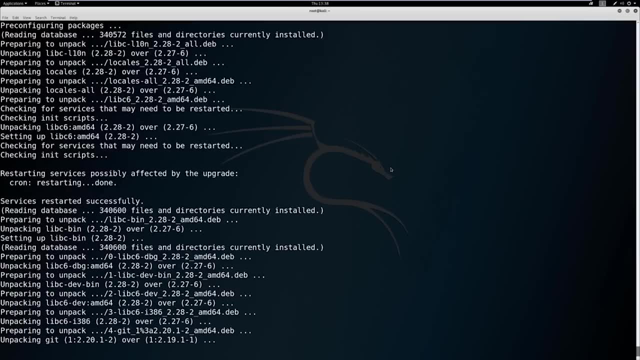 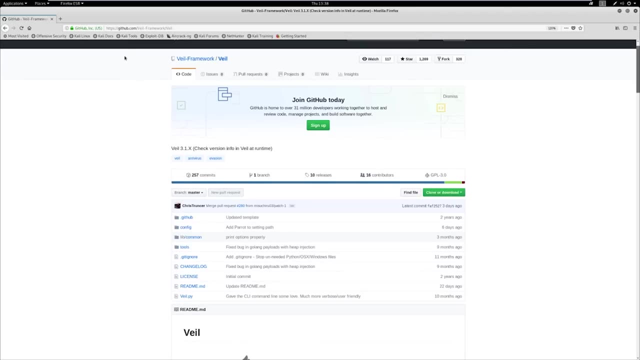 dash Y and that'll automatically say yes. if you just want to accept whatever is coming out for you, you go ahead and just hit yes on that, and it may take a minute for these to install. while this is installing, let's go ahead and talk about what git does. so git works with github. so when we talk, 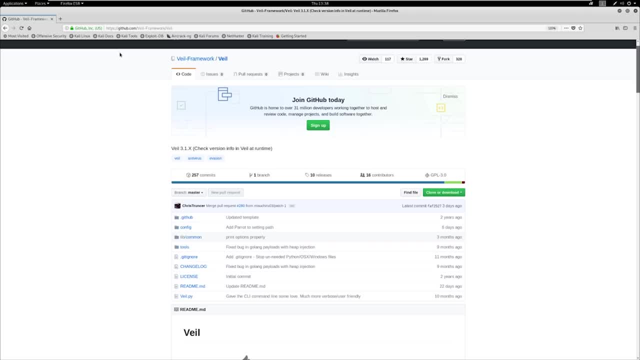 about github we're talking about. a lot of people update their projects, their code, their frameworks on to github, especially in the penetration testing slash hacking community. it's often that you're going to find them in the hacking community. it's often that you're going to find them in the 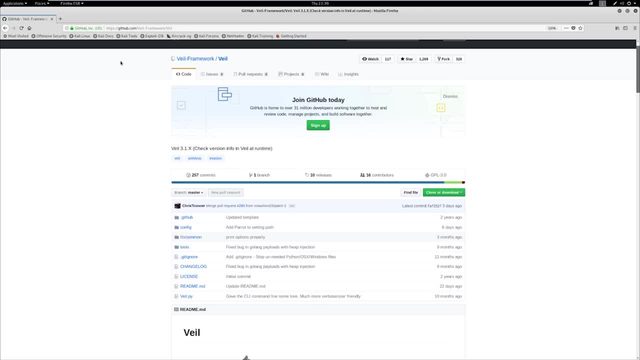 find some cool tools that are out there that are installed on Kali Linux can't be found through apt get, And you have to actually download them from GitHub. So it's very important to know how to use get, And it's very, very simple. So we're on a page like this: This is veil framework. It's 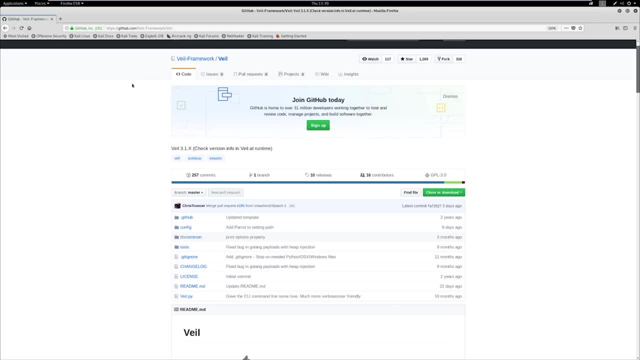 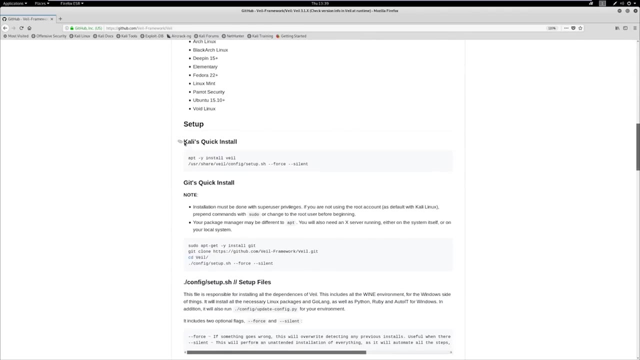 a very popular tool in penetration testing and malware analysis as well. So say, we wanted to install this. Well, there's a couple things we could do. The first thing we could do is always read the directions and see what they recommend. There is a quick install here And if you look, 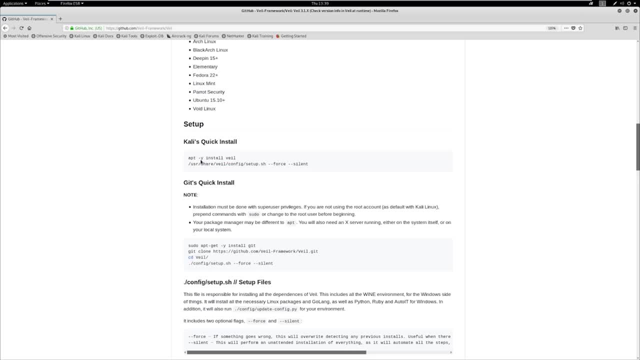 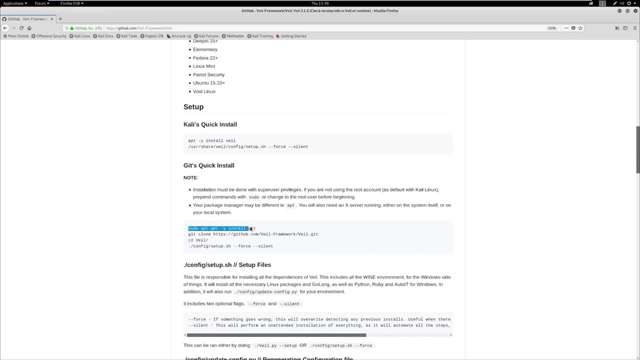 they have a apt install veil here with a dash y, So that will work. Or you can use gets install, where you have to install get first, Okay, and then we do a get clone And we run the configuration setup. So that's what we're going to do here: we're going to install a get clone And then we 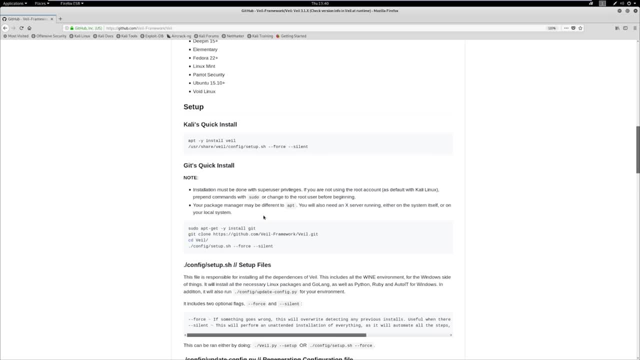 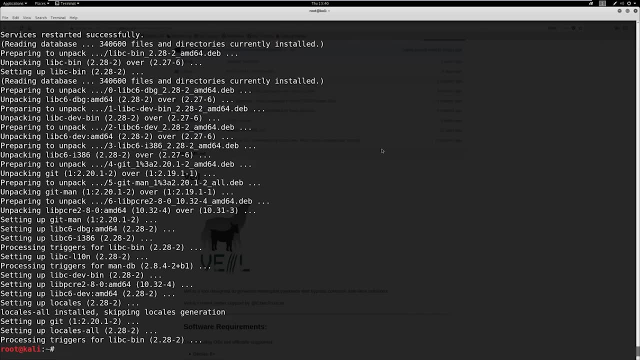 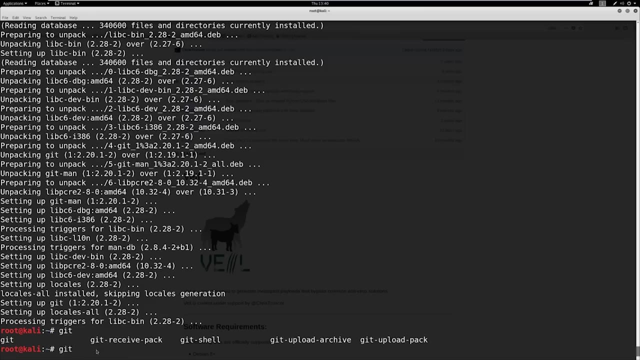 are going to install veil just for the fun of it, just so you can kind of get used to how to use GitHub, how to use get and go from there. So let's go ahead and just alt tab back over. looks like we have it. we can check it by typing get and hitting tab. Okay, so get is here And we're just going to. 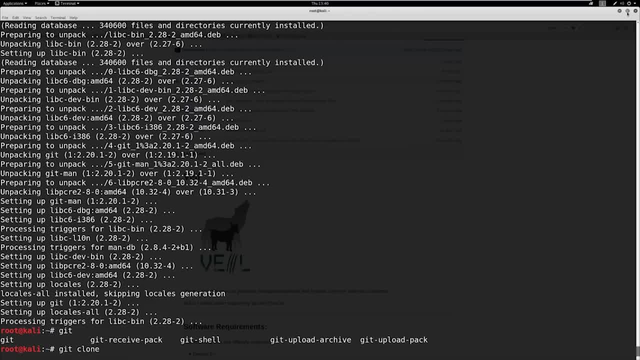 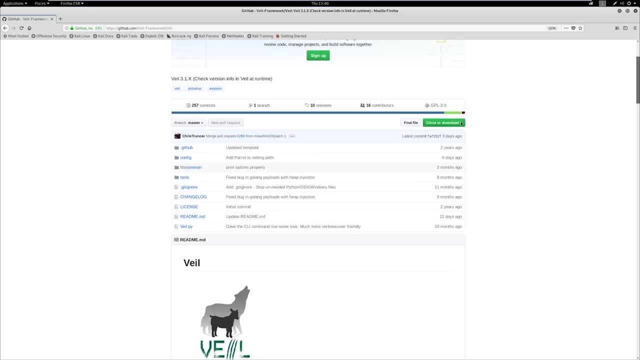 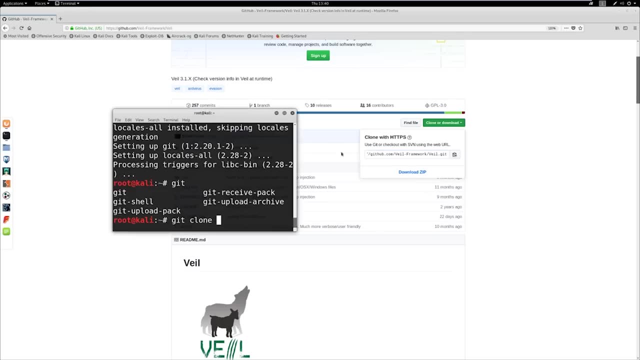 hit space. we know the command is clone And while it provides it for us, down here it says: Hey, get clone, copy this. The other place you can do it is right here, where it says clone or download. you just copy this bad boy right here, We'll all tab. 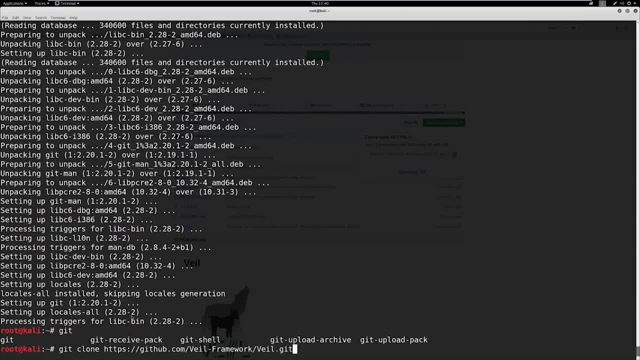 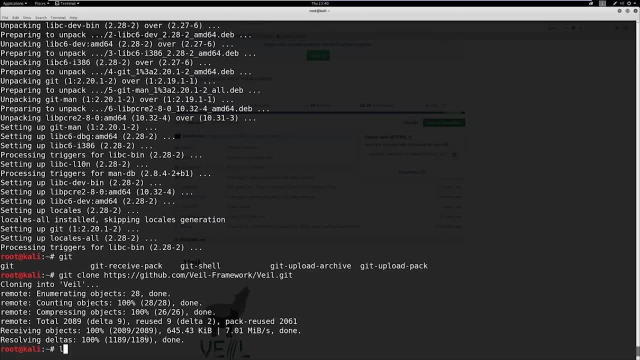 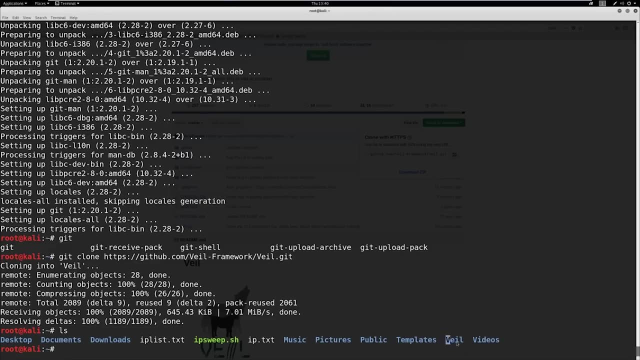 back over to our terminal and just hit paste Okay, and this is going to install in the directory that you choose. So I just put it in this root folder here- And actually our home folder, I should say- and it's installed right here. the folder is veil right here. Typically when I 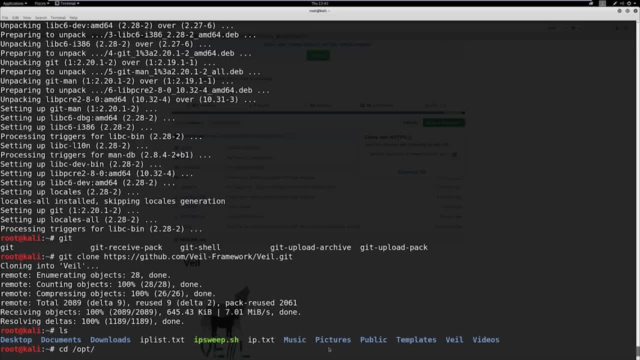 install things, I like to put them in the opt folder. So here, CD opt. But since I went ahead and downloaded here, let's just go ahead for an example purpose. If you do want to install to opt, you're more than welcome. You can. 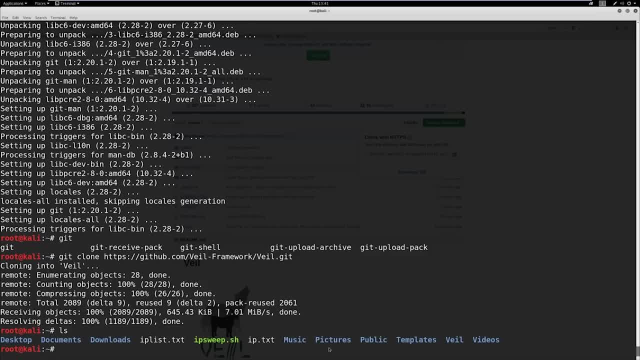 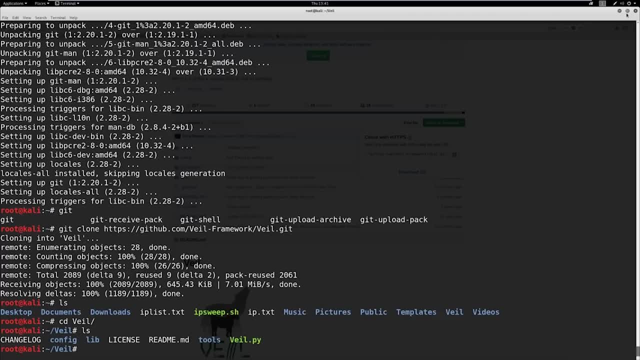 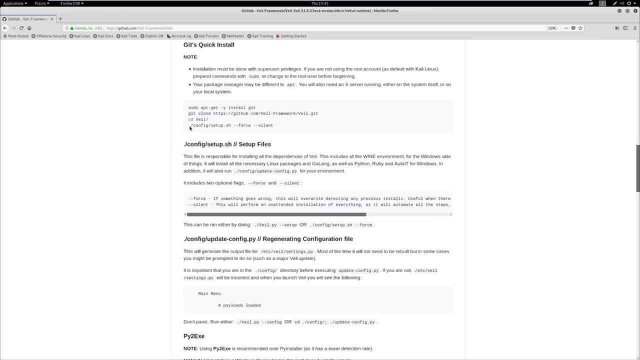 move the folder there as well. So what we're going to do is we're going to CD into veil And then we'll hit ls. Now remember there were instructions, So let's go ahead and look at what those instructions were. The instructions said: you're going to run dot forward slash config set. 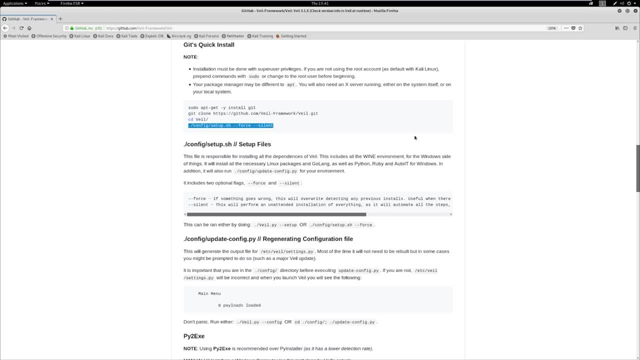 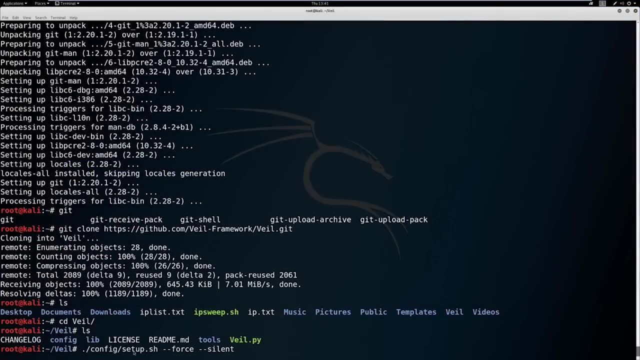 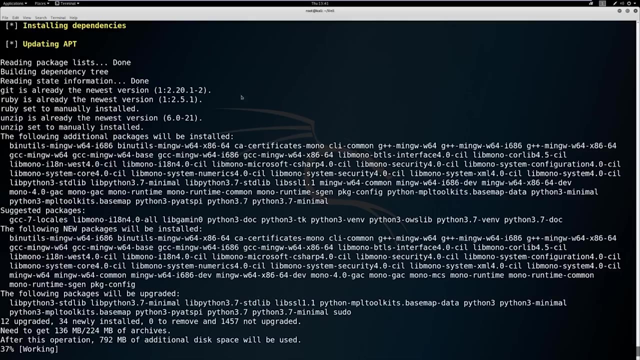 up the sh force silence. let's go ahead and just copy this guy. We'll come back in here And we'll hit paste And it's just going to run out of this config folder, setupsh, And now it's installing. So we could have easily installed this with app dash get, which, if you look, look what it's doing. 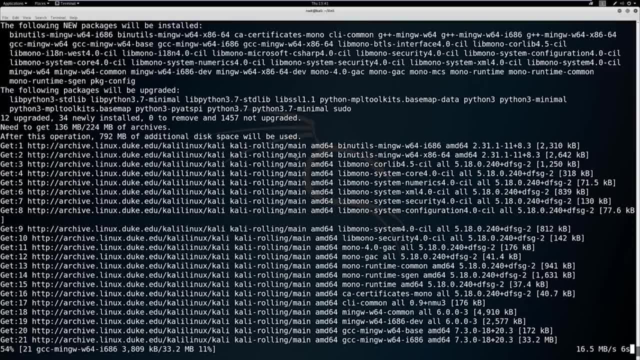 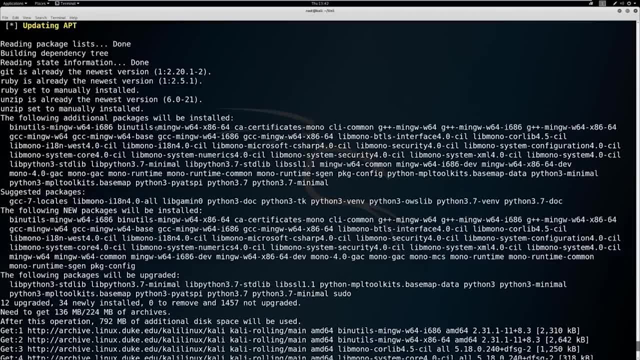 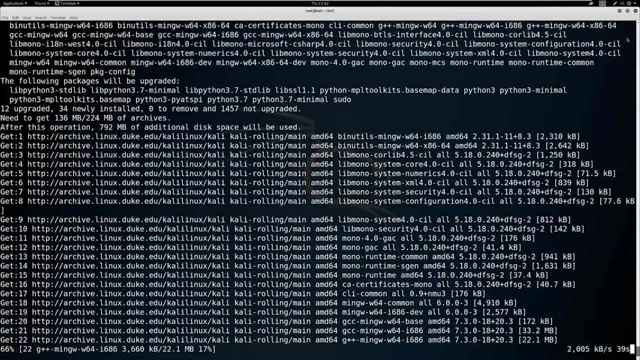 it's actually rolling through the packages here And it's updating the repositories, right, these packages, And then it's going to go ahead and download what it needs. So it's running apt get. Anyway, if you see, updating apt, it's installing the dependencies. So the easier way, the quick way, which is: 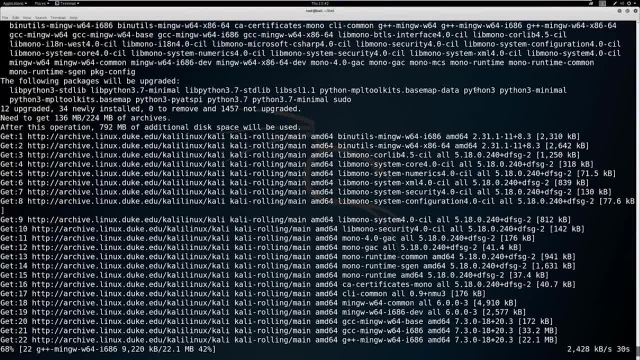 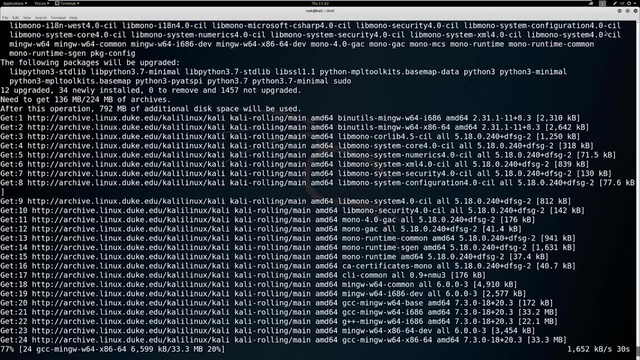 suggested was to do it through there, And it's right. they don't always have installed packages in apt get, So that's why I wanted to show you the GitHub version of it, So you can go ahead and let this install. Let's just go ahead and recap quickly what we just did. So we 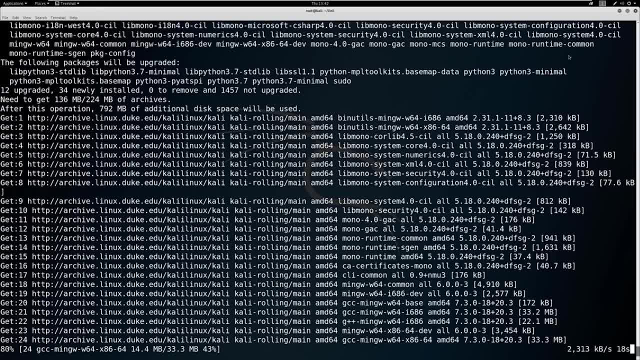 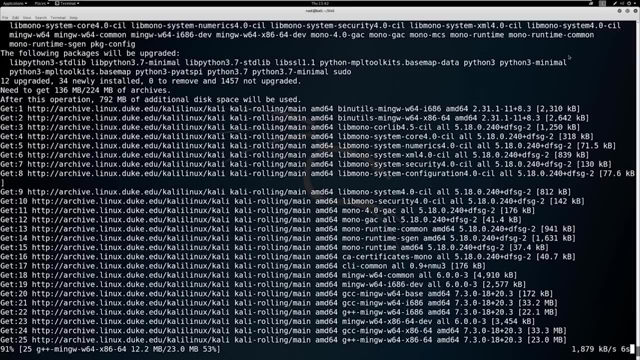 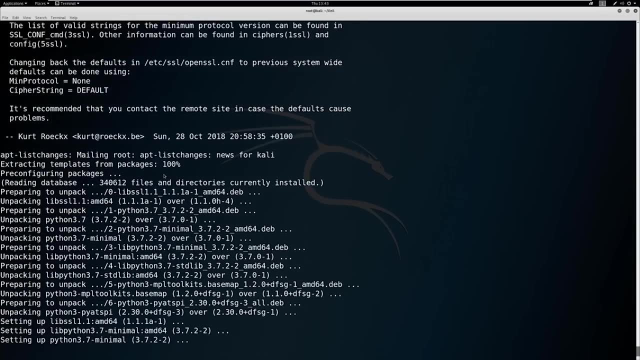 used. we used apt get, update and upgrade to install updates in our system. We used git clone to be able to download packages and clone packages off of GitHub, And we used apt get to be able to download git itself. So that's really it for this lesson. What I do encourage you to do is go through the man. 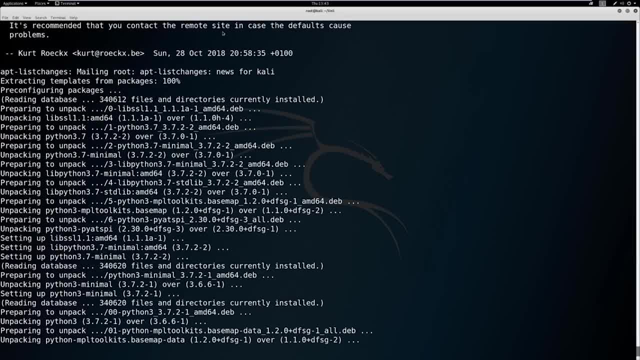 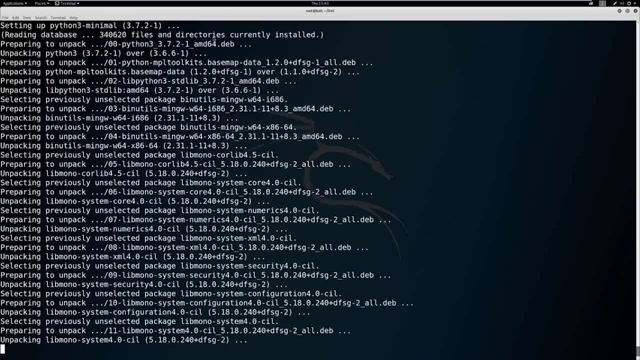 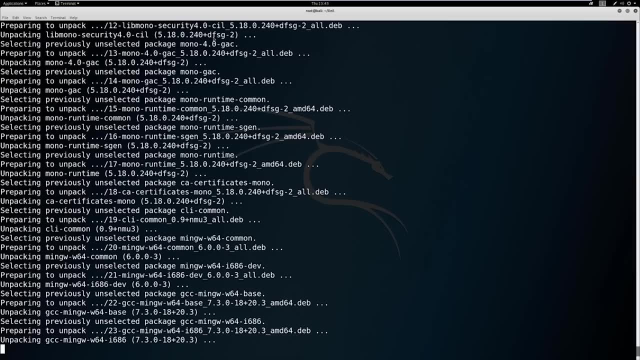 pages of git and go through the man pages of apt get And then you can go ahead and download the apt get, Because you're also able to remove programs, update specific programs etc. So this lesson really just wanted to introduce you to the basics of downloading and updating for your system. I 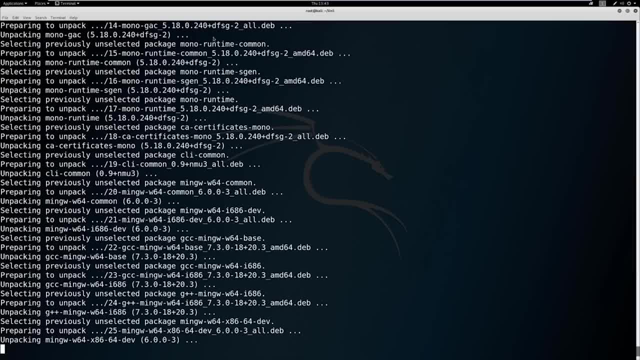 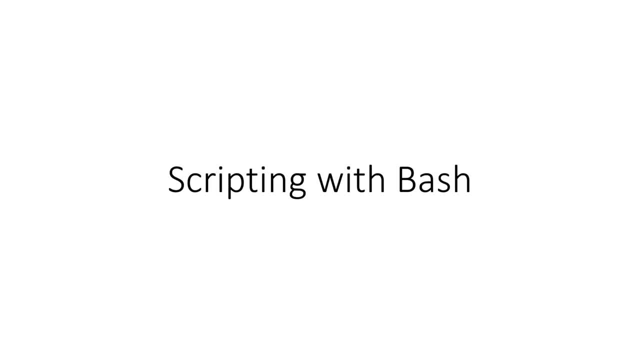 encourage you to learn how to remove files, as well as a little bit of homework for yourself. So thank you for joining me and I'll catch you over in the next lesson. All right, welcome to the last lesson video. So in this video we are going to be: 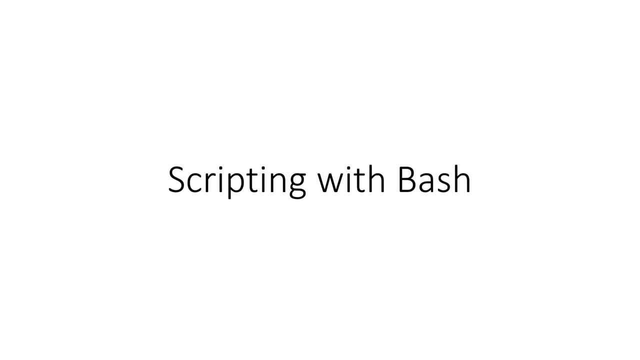 scripting with bash. Now, this may seem a little overwhelming at first. what we're going to be doing is building out a ping sweeper script. it's going to be pretty basic, And what I want you to do is maybe just watch this video once And then the second time through, really try to follow along. 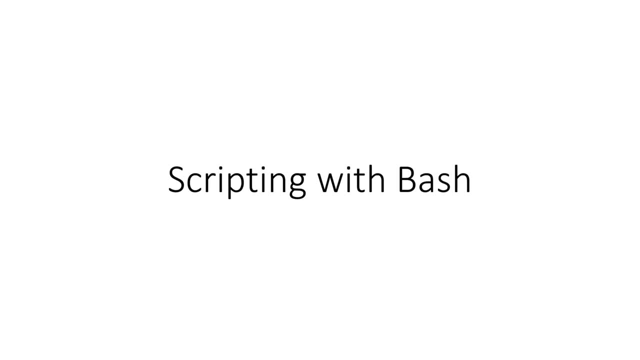 with it, take notes etc. I think first time watch through, you know, just to get the concepts understand what I'm doing, And then the second time, really, really get hands on with it, And I think that'll be probably the best way to learn. But if 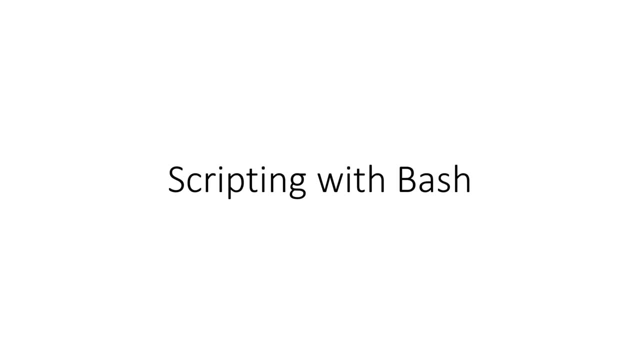 you have a different learning style, please do go ahead and try that as well. The only thing I can say is: don't let this intimidate you. Hopefully, by the time the video is over with, you will have a pretty good understanding on basic scripting and how scripting can really be beneficial, and 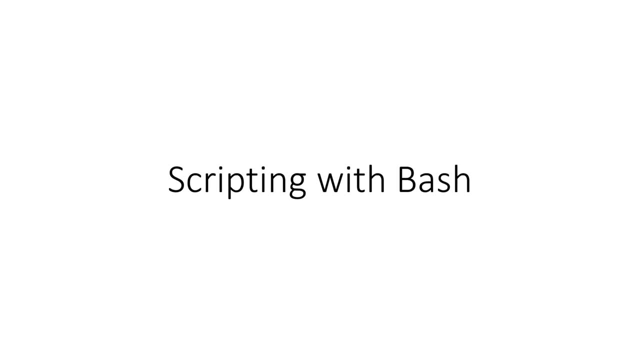 improve our timing, improve automation, etc. So let's go ahead and quickly talk about some of the things you're going to be learning in this video. Okay, so some of the commands and items we're going to learn. we're going to talk about grep, which is going to allow 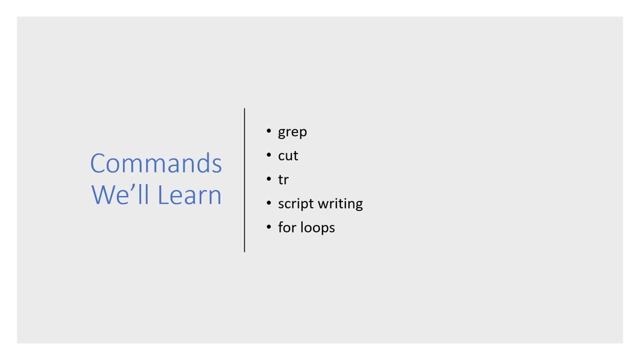 us to narrow down some results. We're also going to talk about cut and TR. Both of those are also going to help us narrow down some results. So, basically, we're going to start with a ping that we're going to send out and we're going to want to gather information back that says that ping was. 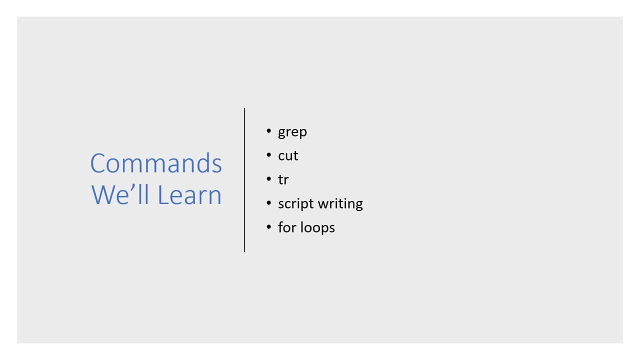 valid. So we want to know any computer that responded to us. Well, how are we going to do that? Well, we need to identify what a valid ping looks like. we're going to use grep to to kind of narrow down a string or 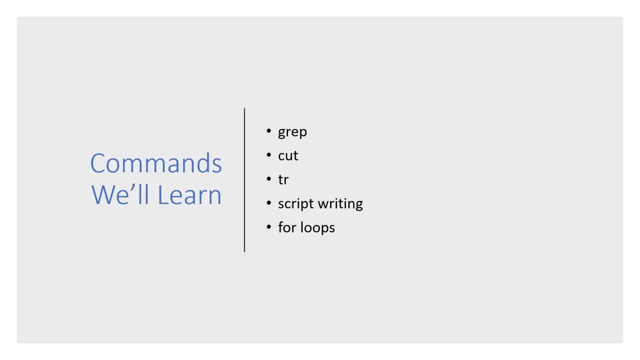 a sentence or something that identifies with a positive ping, And then we're going to cut out everything we don't want and use TR as well to cut some things out that we don't want. So we're going to put this into a script when it's all said and done, And we're also going to be talking about. 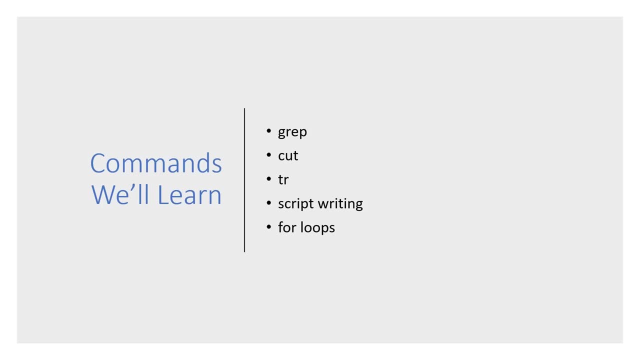 the usage of for loops and their importance, not only with using them in this script, but how we can use simple one liners to do everyday things for us. So I'll show you at the end of the video how we're going to use like an end map and use a for loop with n map to run through an n map. 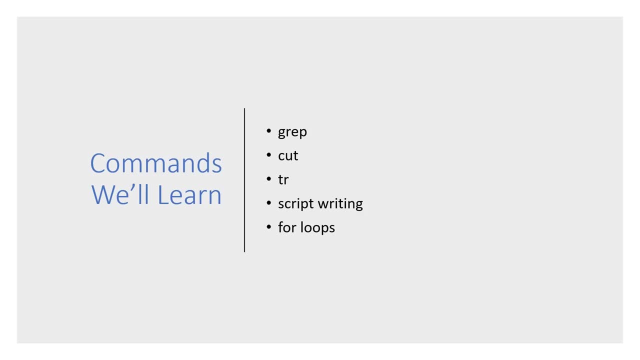 script. So stay tuned through the video. Again, if you are a hands on learner, maybe first time through you you try hands on, but my recommendation here is to just sit back, watch the video, understand what's going on Second time, really follow along with it, take notes and get the most that you can out of this lesson. So let's go. 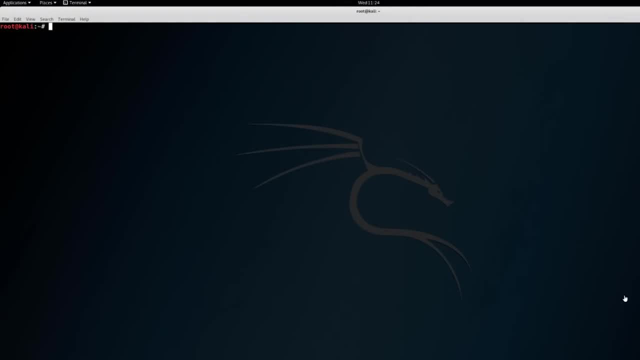 ahead and get started. All right. so now we're going to be covering bash scripting. So the first thing we're going to need to cover before we get into writing our scripts is how to narrow down results. And we say narrowing down results, what we're saying is for given a block of text and we 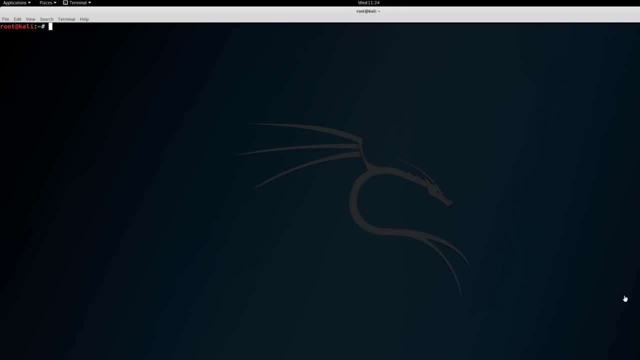 want to extract some information from that block of text. how are we going to do that? So that's what we're going to cover in this lesson. Okay, so let's go ahead and get started. What we're going to be doing today is narrowing down a ping. 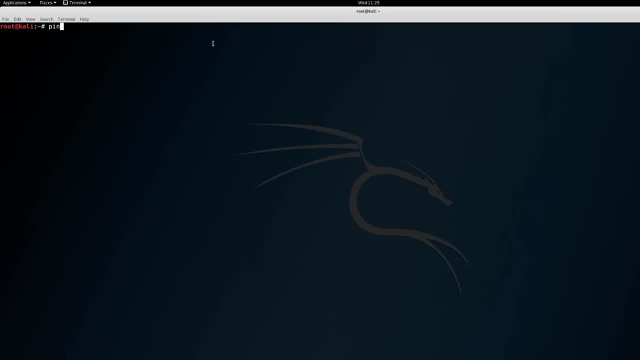 result. So if we come into here and we need to ping an IP address within our system, So I'm going to be pinging 192.168.1.90.. And you're going to see that it returns a 64 bytes from that address. So it looks. 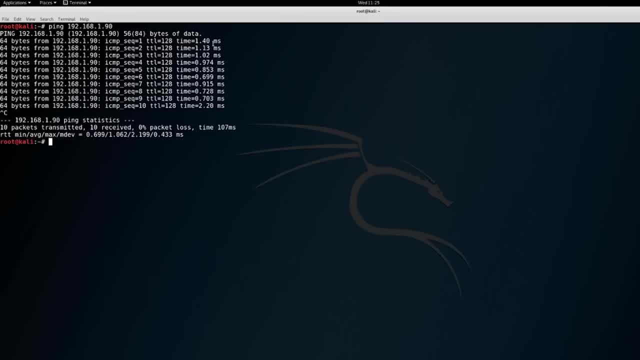 like we're getting a response. I'm going to hit Ctrl C here. So if you remember from the networking section we actually get a response unlimited until we cancel it, right, like we just controlled C here from ping. So there's another thing that we can do if we 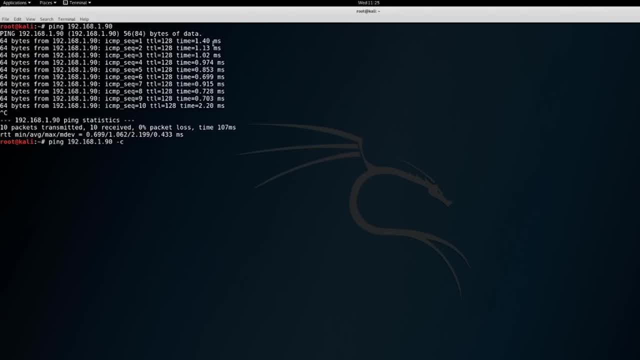 only want to send one packet and see if it's alive or not. we can do a dash C of one, So we're just going to do that. So that's a count of one. we're sending one packet over. if we set 10, it would send. 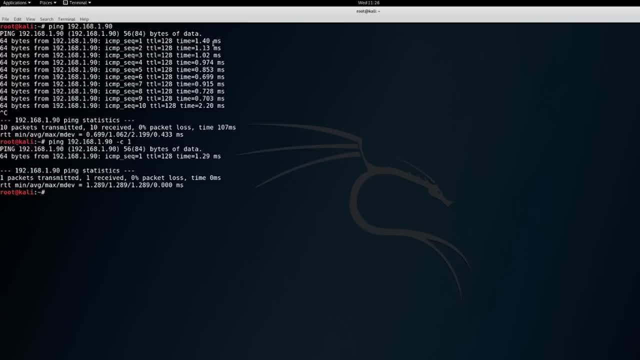 10 packets over, if that makes sense. So now what we're going to do is we're going to put this into a text file. So, if you remember from previous video, we just use this little carrot here and I'm going to call this IP dot. 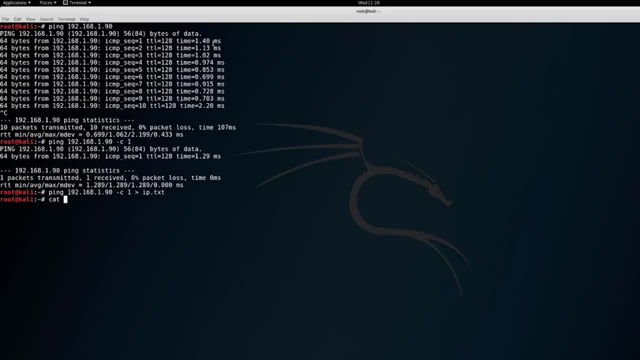 text, Okay, and if we cat IP dot text, you'll see the same results there. So now, what we're going to want to do is we're going to want to narrow this down. What do I want to extract from here? Well, I want to extract this IP. 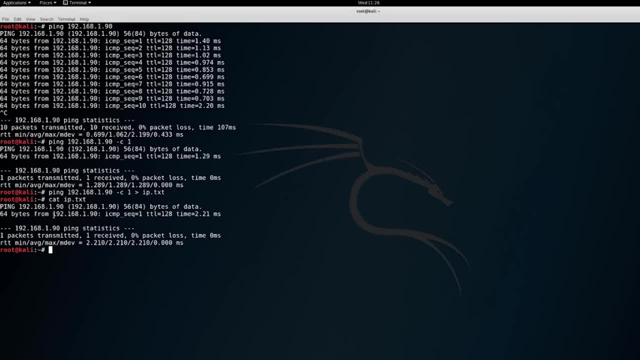 address, And it'll make more sense when we get into the scripting part. But what we're going to do is we're going to get out specifically of this, This IP address from this line. Now, what we're interested in actually is a returned IP address that has a valid 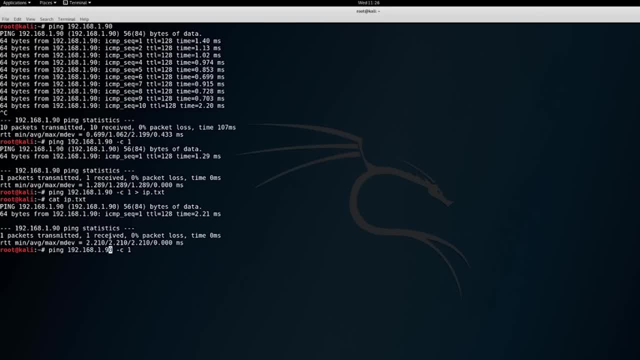 response right. So if I were to attack or if I were to enter in here, say 15.90.. Okay, there's no response there. So this is kind of what it looks like When it doesn't get a response back: it just kind of lingers, And then we hit. 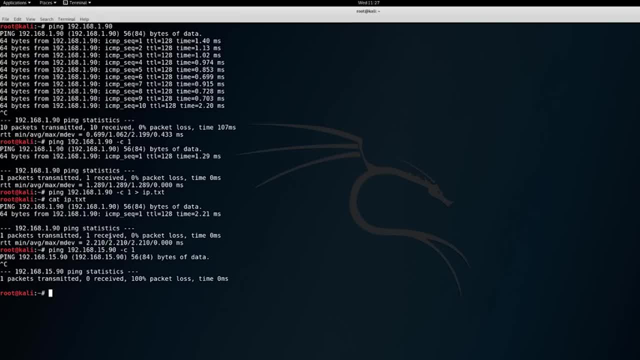 Control C and it says zero pings Right, nothing was was received back. So what we see when we get a response back, as we see 64 bytes, when there's no response back, we don't have any bytes. So if we're doing a sweep through a network, which we're going to be doing, 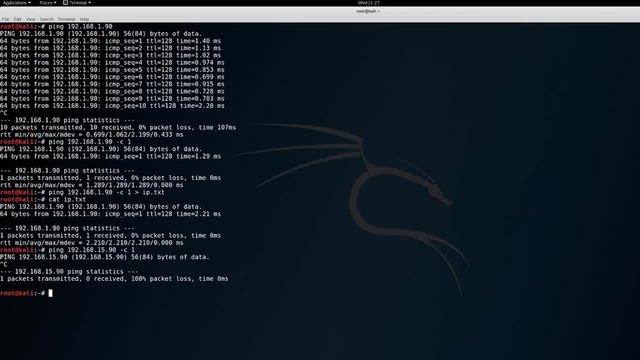 later we need to be able to narrow down these results. So if we're sending, say, 192 dot, 168, dot 1.1, all the way through to 55. And we want to see who responds back and then take that list and narrow it down. 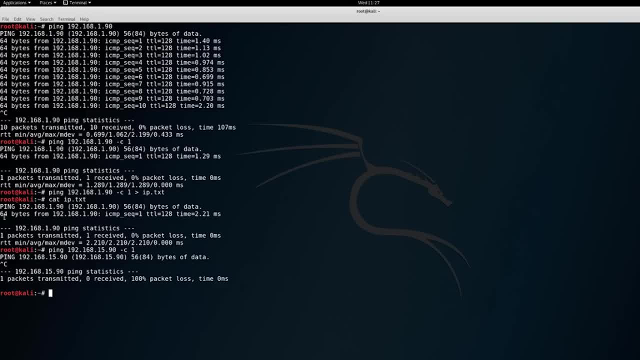 To the IP addresses, which is exactly what we're going to be doing. we need to know how to narrow that down. So what we're going to be narrowing down on specifically is the 64 bytes. So let's tab up a couple times to this cat IP address And we're 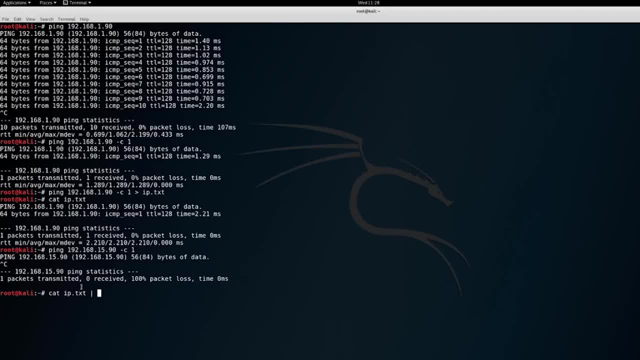 going to do a pipe, and the pipe just means we're going to add an additional command here. So the additional command we're going to do is called grep. grep is going to grab any line with what you specify. So let's specify 64 bytes and see what. 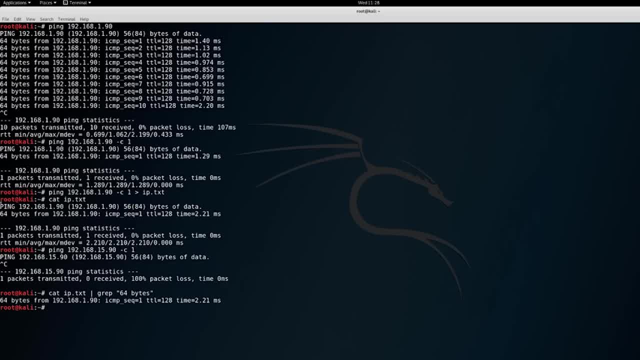 happens. See now, if you noticed, we had all of these lines before, And now what grep is doing is grep is taking only the lines that contain 64 bytes. So again, a valid response. So we have 64 bytes here and we have achieved a response. So what we're going to? 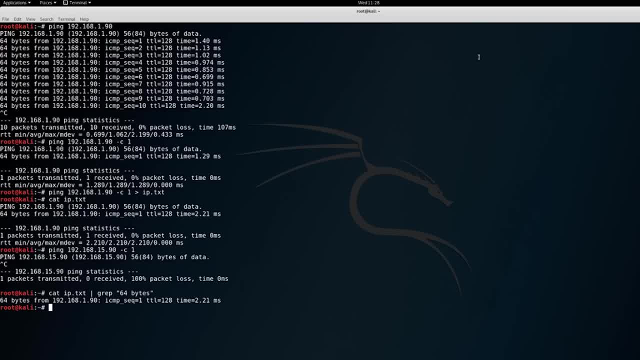 do now is we're going to narrow this down some more. Okay, we've got this line here, But again, we're still trying to extract this IP address. So how can we do that? Well, there is a tool called cut. So if we tap up again, we do another pipe because we're sending a new. 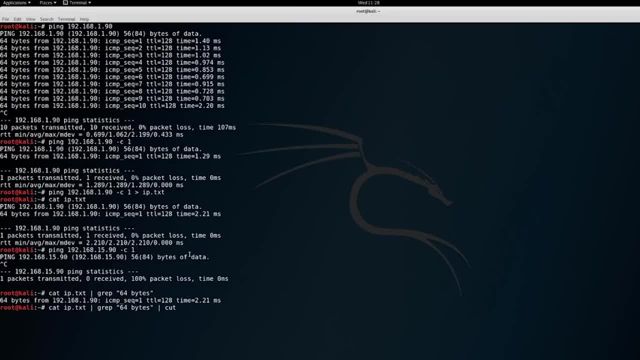 command. we're going to say cut and cut. syntax looks like this And I'll explain it once. I type it out here: Okay, so we have cut, and then this hyphen D, that's a delimiter. So the delimiter is what we're going to be cutting on. So we're giving a delimiter of a. 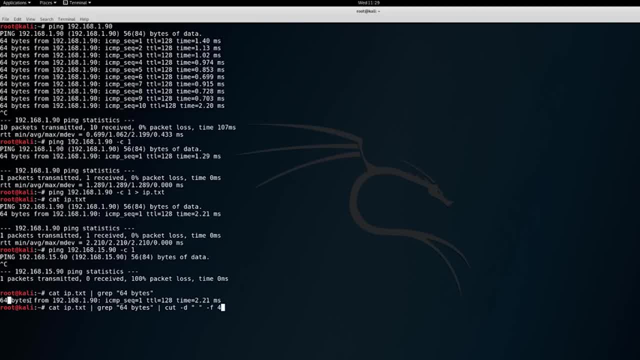 space. here's a space, here's a space, here's a space. So we're going to be cutting on these spaces. And then we give a field. we say, Okay, what field we want to retrieve back from this cut? Okay, we want field four, if you look, 1234.. And the fourth field is our IP address. So it's. 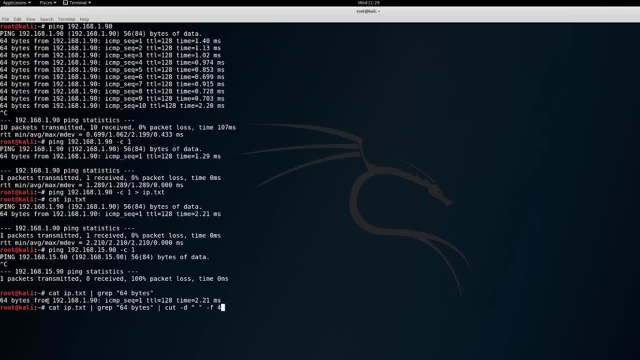 going to say, Okay, I'm going to cut on this space. I'm going to cut on this space, I'm going to cut on this space And then I'm gonna take it right here. Now, if we identified field five, we would be taking this. we identified field three, we'd be taking from. So let's go ahead and just hit Enter and see what that. 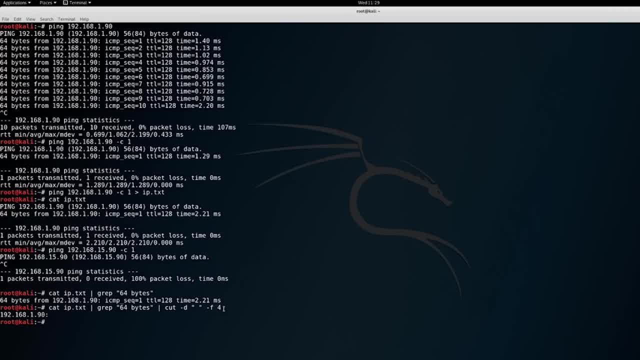 looks like Okay. so now we are narrowed down even more. But there's an issue here. If we were to try to send this IP address, we would have this little colon here attached on to it And you can't ping with that IP address. So we're going to be doing a sweep or narrowing down. 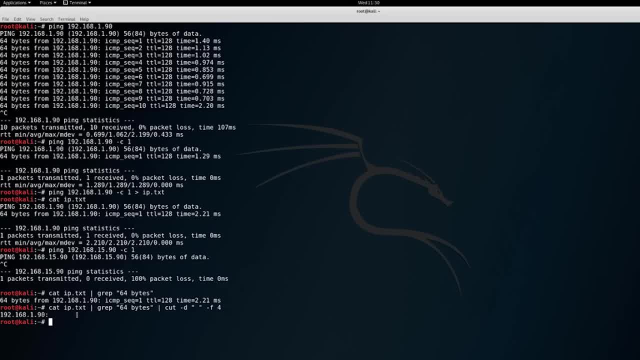 this list, then we're going to actually need to remove this guy here. So let's take a look at how we do that. So if we tap up again and again, we're going to add a pipe. Now we're going to use a command called 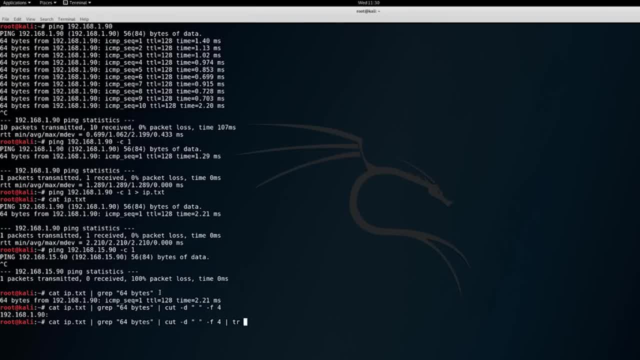 TR, And TR just means translate. What we're going to be doing is another delimiter, So dash D there And we're going to be taking out that colon. So it should look something like this: If we hit Enter now, you can see that that colon has been removed. Okay, now let's talk. 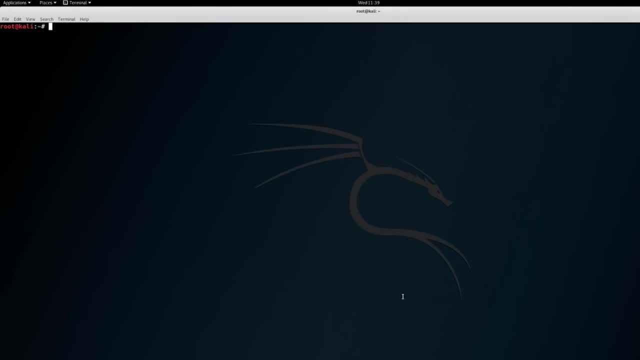 about how we can use this information to write out a script. We're gonna start with a basic script and we can add upon it as we go. So I've gone ahead and written out a script, But we're going to talk about it very slowly So you can actually look at it and copy it down. So what we're going. 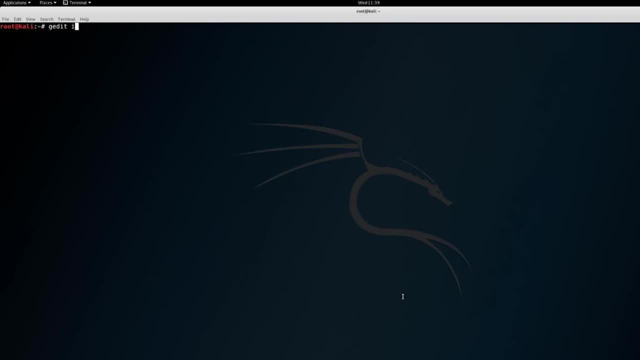 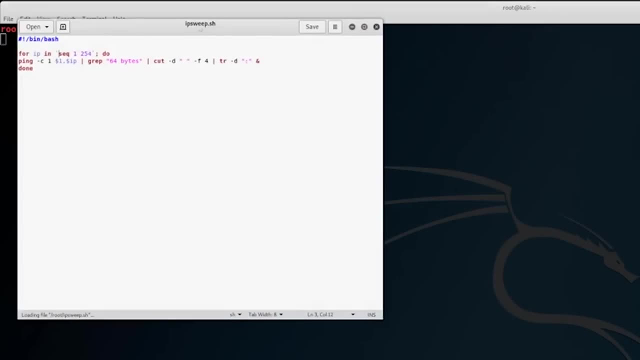 to do is go ahead and say g, edit, And I call this IP sweep dot sh. So go ahead and do the same or something similar, Enter. So let's take a look at this script. So at the very top here we have to. 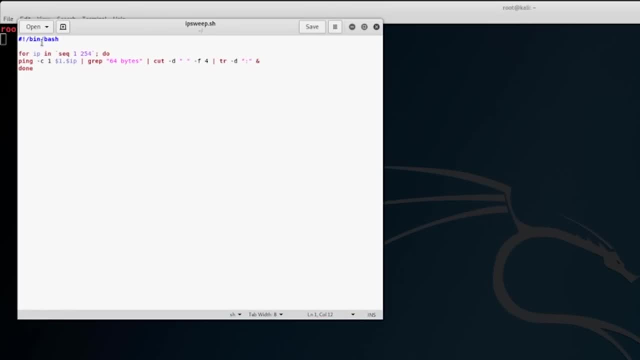 declare what we're doing. So we're going to give a hash bang, And we do this with any scripting language. So if it was a Python, we'd be entering Python here, but this is bash. So we're going to be doing a forward slash bin, forward slash bash that declares that we're running a bash script. 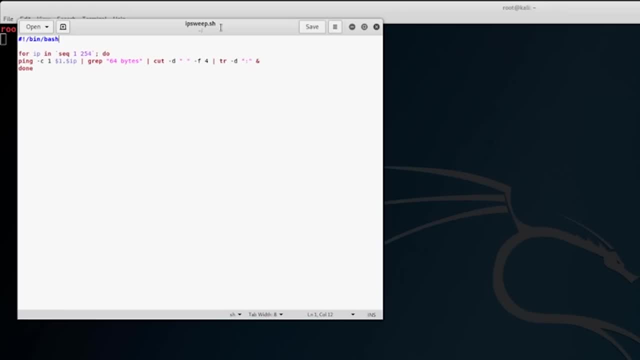 And the dot sh also indicates that we're running a bash script. So I want you to ignore this line here, in this line, here, For now, let's talk about this line. this should look very, very familiar. So we're doing in this line, we are saying we're going to. 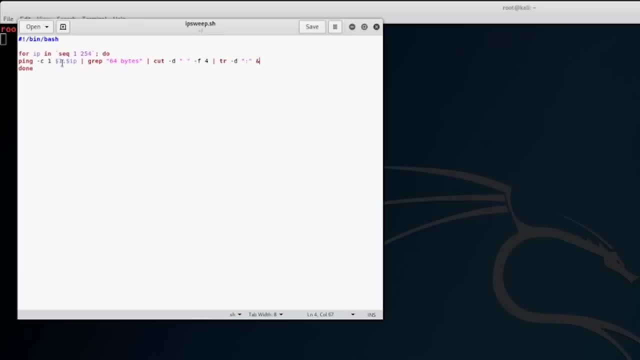 ping with a count of one, which we talked about, And then we're going to do something. here we've got $1 and $1. IP. let's just ignore that for now. Okay, so we're going to go ahead and do. 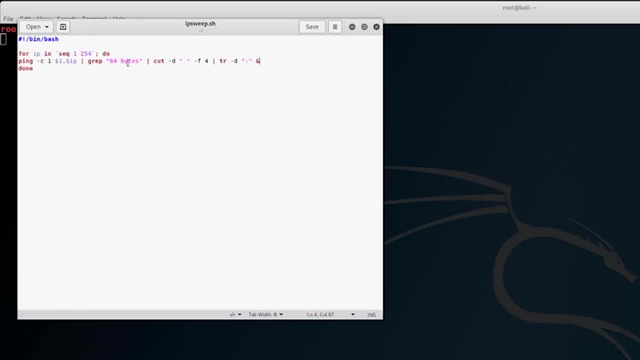 the rest, that should look familiar. we're going to say we're going to grab 64 bytes, we're going to cut the delimiter of a space field of four And then we're going to do a translate right and take off that little bit at the end. Okay, I added an ampersand here at the end, So an ampersand allows. 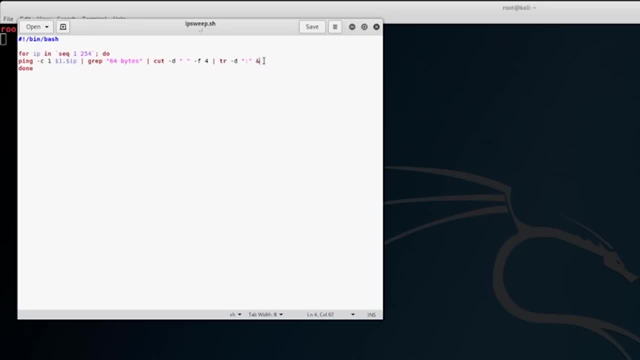 us to do threading, So that's exactly why it's in there. If we didn't, we'd have to let the process go one IP at a time, And we'll talk about that in a second as well. So let's talk about this for line. 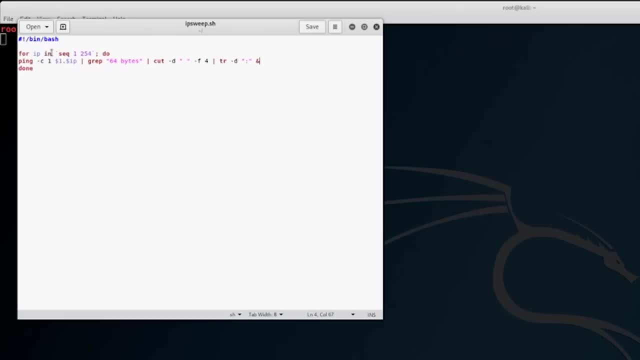 So a for loop is what we're actually running here, And the loop is saying: I want to do an IP address. we're just declaring a variable here, you can call it whatever you want. We're saying hey for this IP in a sequence of one through 254, we're going to do something, and that do is a ping. 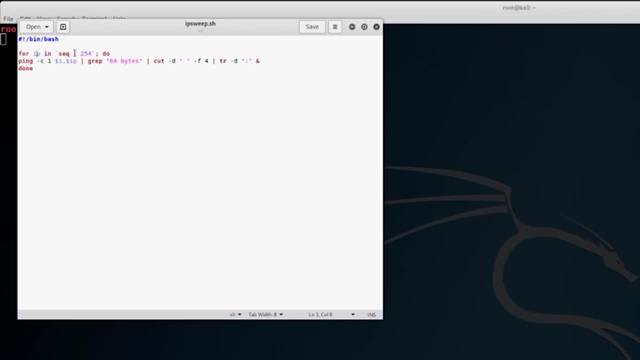 So what this means is for IP, and if we think about it in sequence, one through 254, what it's saying is 1234, all the way up to 254.. Okay, so think about it this way. if we say for one, 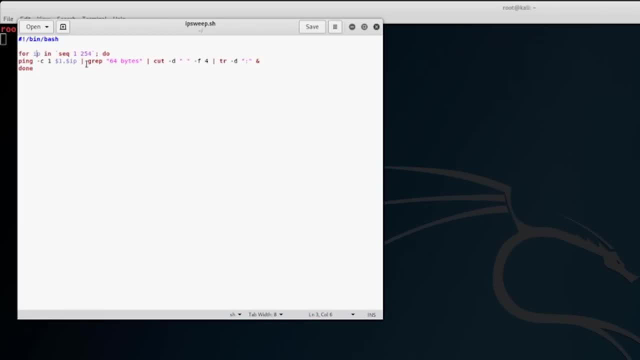 in this ping sweep. we're going to do that right. So we're going to say for one, for 243, all the way through 254.. That's what this loop is doing. So it's a very, very simple loop. Now, IP is. 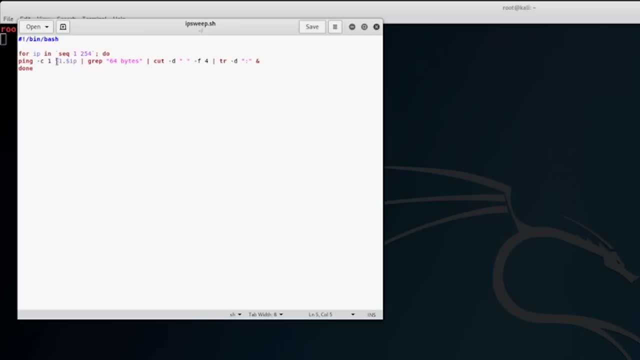 the same as a loop, right? We're also calling out this dollar sign one. Now, this dollar sign one is user input, So we're going to actually do something. this is called IP sweep, right? So we're going to have to call out this IP sweep, something like this: sh, and then we're going to have to give. 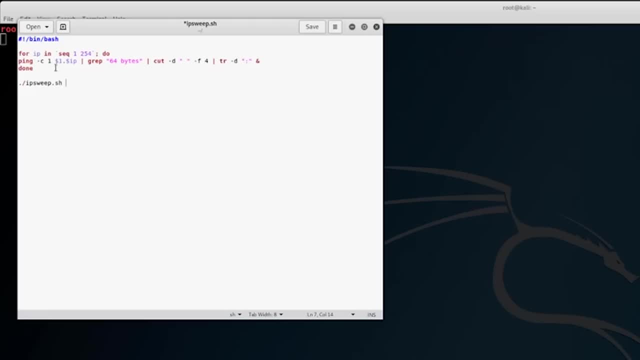 out some information. it's going to request information. if we don't provide it, it won't know how to ping. So what we're going to do is we're going to say the first three octets of our home network. So if yours is 192.168.1, like mine is- then you just enter 192.168.1.. 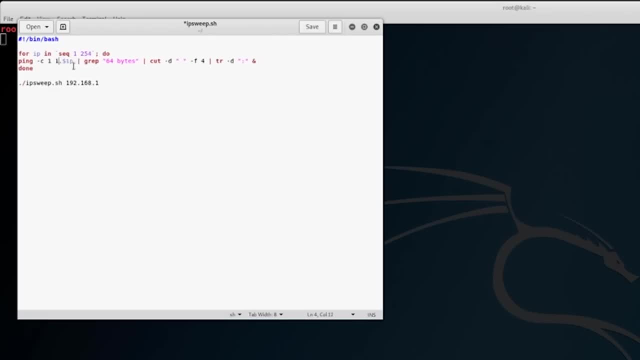 Now we could also, for simplicity, just hard code this, So we can say 192.168.1.ip address, And it would be fine. we don't have to build this in. The only reason we're not hard coding it is: 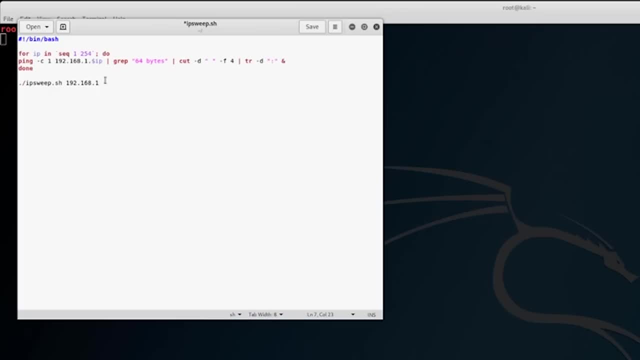 because you can do multiple ping sweeps. this can be a ping sweep script for you in the future if you're on a different network or you just want to write something out really quick. $1 works, perfect. But if you want to leave it hard coded like this, it'll also work. So let's. 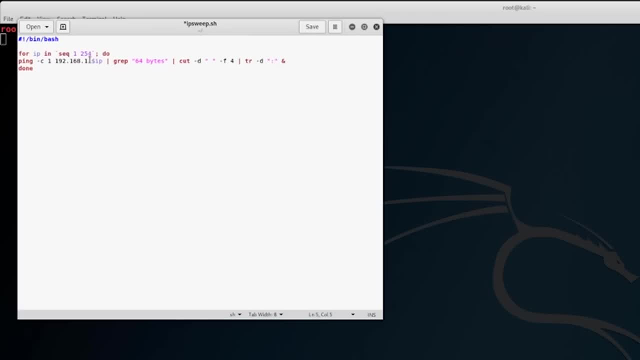 go ahead and just delete this out. I'm going to put this into $1 again to have a proof of concept, And then we are going to run this. So all we do here at the end is declare done. If we didn't run this with an ampersand here, we would have to add a semicolon similar to this: 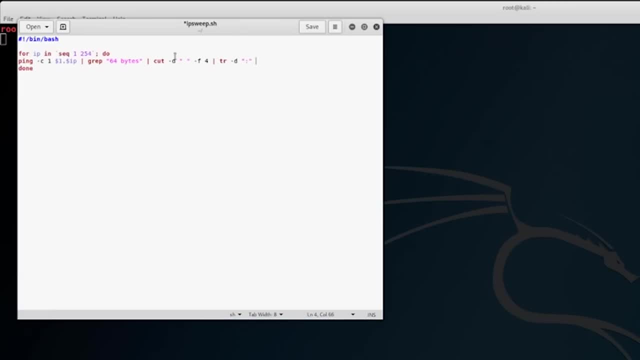 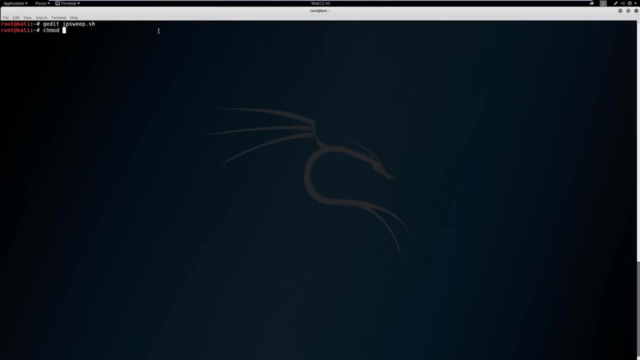 But because we are having an ampersand, we can actually get rid of that and just put that back, just for some syntax clarity here. Okay, so let's go ahead and save this And remember for my lesson: we're going to have to change the mode of our script because it's not. 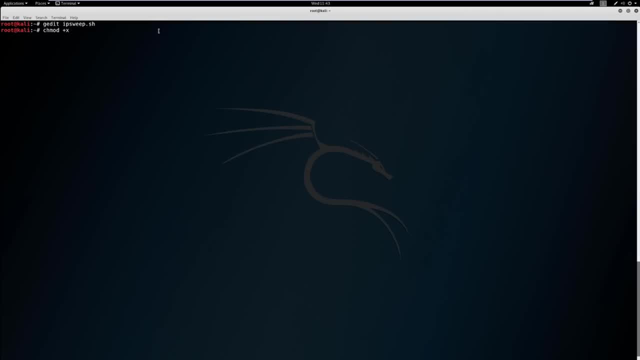 executable by default. So we're going to do a plus x here And then we're going to call our IP suite sh. we can LS and make sure it's green. Here's IP sweep sh. And then we'll do a dot forward slash. 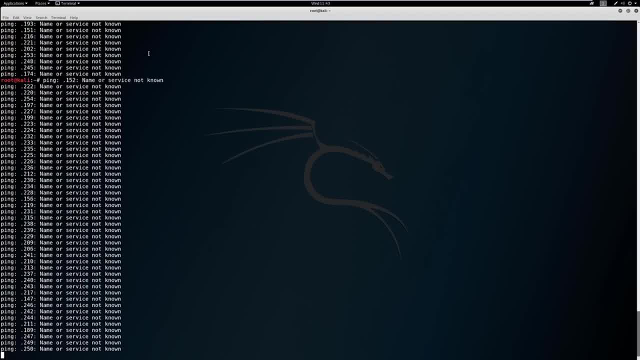 IP sweep sh, And I'm not going to enter anything in as want to show a proof of concept. So see, it ran through every single number here and threading and name or service not known because we didn't provide an IP address. So what we can do here is we need to provide that IP address: 168.1.. 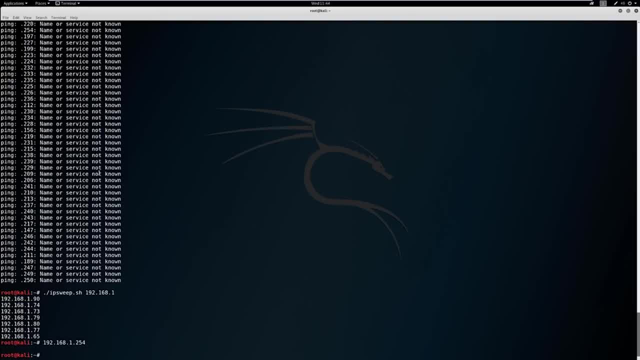 Hit Enter, Okay, and it pulls back some information. So what we can do with this information? let's write this out to a file. So let's just call this IP list dot txt, something like this. Okay, it's done. 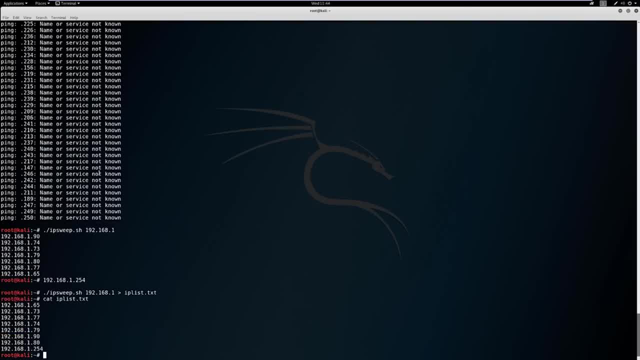 Now let's just cut out the IP list dot txt. Okay, now we have an IP list of the IPs in our network that we just swept right And we can use this information later on. But before we go into that, I do want to go back and just improve our 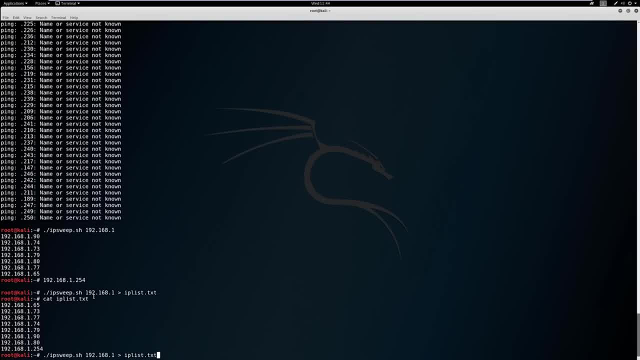 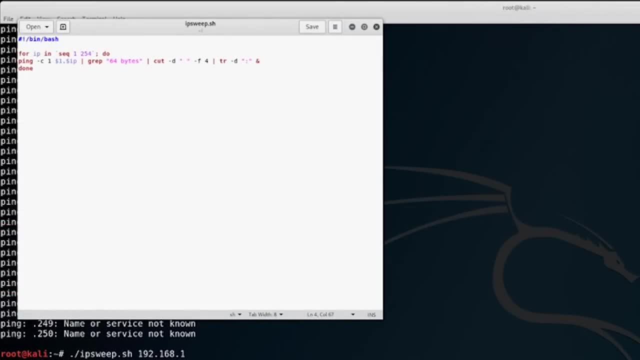 script a very, very tiny bit. So let's go ahead and just tab up a couple times till we get to our g edit And let me show you how we can improve this script. It doesn't have to be overly complicated. What we can do is we can say something like this: 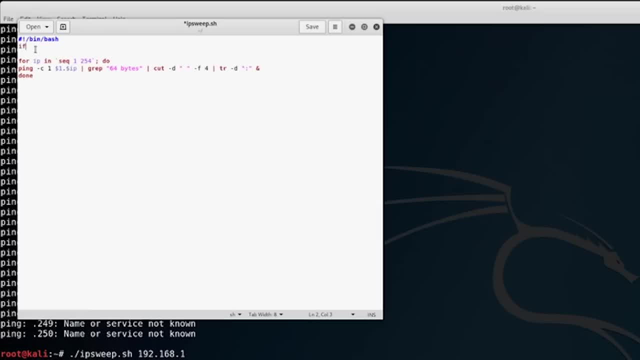 We can come in here and give an if statement. So if is conditional, right. we're going to say: if this exists, then do something, and if it doesn't exist, do something else. So we're going to say: if dollar, sign one. 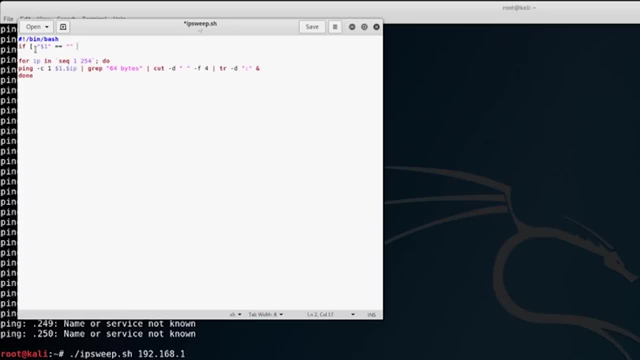 is equal to nothing. we're just going to give blank space here And then we're going to say: then we want to do something, So what are we going to do? we can echo out something similar to you forgot an IP address And then echo out what you need to do like syntax. 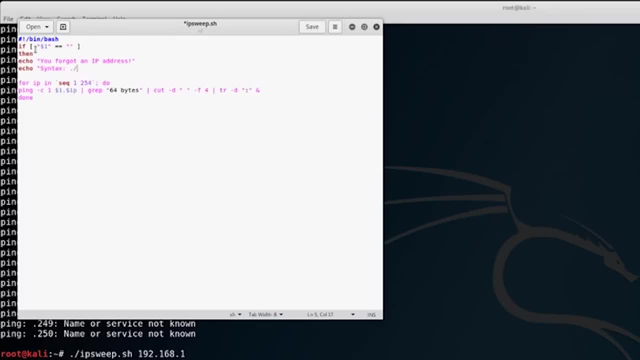 dot, slash, ping sweep or IP sweep is what we call this: IP sweep, sh and then IP, Or we can even write it out an example, right, Something like that. So that way our user, if they're using it- we wrote this for somebody else- they know what we're talking about. 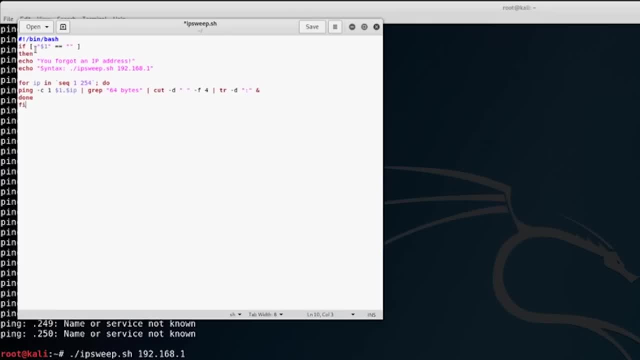 And at the very end we just need to write: if backwards, we'll put a fi. So what this is saying is: if this is not, then echo here. right, we're going to echo these. And then we need to add one other thing here, which is an else. Let's go ahead and hit enter, just to space this out a little bit. 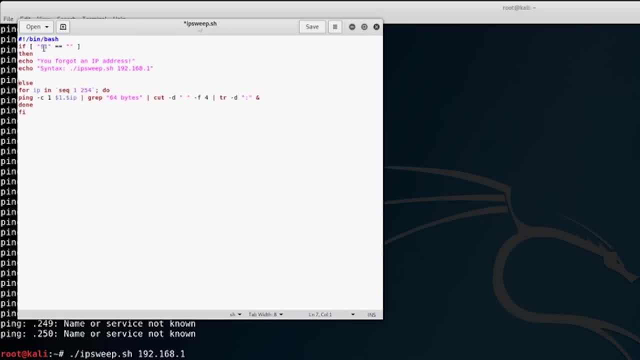 So if we have no dollar sign one declared right, if we have nothing entered in, we're going to say: echo, you forgot an IP address and syntax here. If we do have something in dollar sign one, okay, we're going to do something else. we're going to do our ping sweep And that's it. 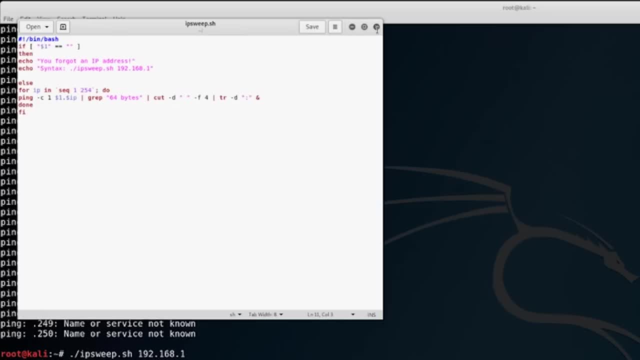 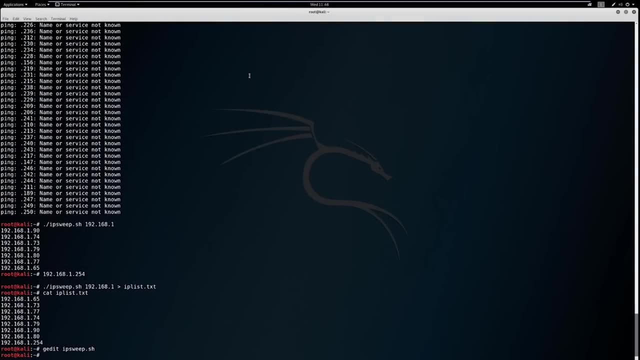 So this is very similar and modified from Georgia Weidman's that I've got a long time ago, So full credit goes to her for this little script. It was very, very easy to learn And it's also very easy to teach, So let's go ahead and just run this one more time. we're going to say IP sweep. 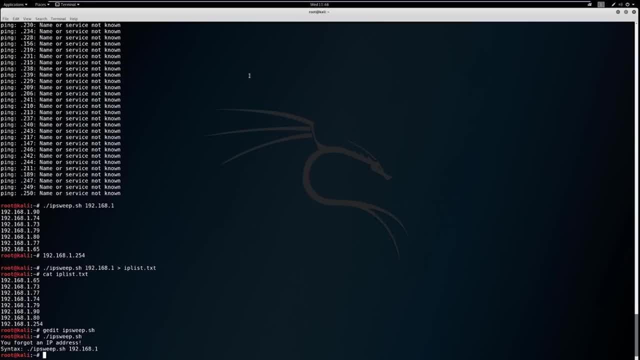 the SH And look what happens. Now it says you forgot an IP address. Now we can declare a number in there or anything. And the scripts not perfect, right? We're expecting three octets And we could give it a one, And it's still going to do something like that. 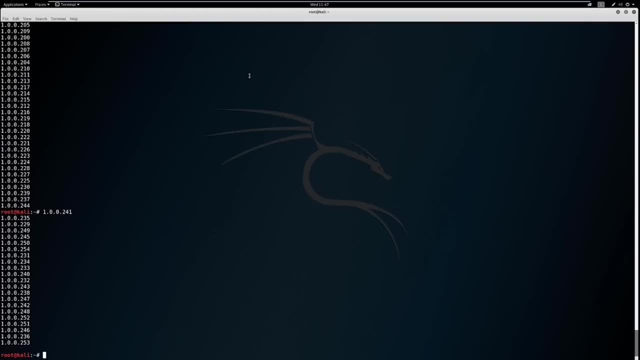 which isn't correct, right. So we need to be able to, to modify this down more. but that gets really advanced scripting into declaring that needs to be three octets And if you don't provide those, then what? and that just gets more advanced. So we really 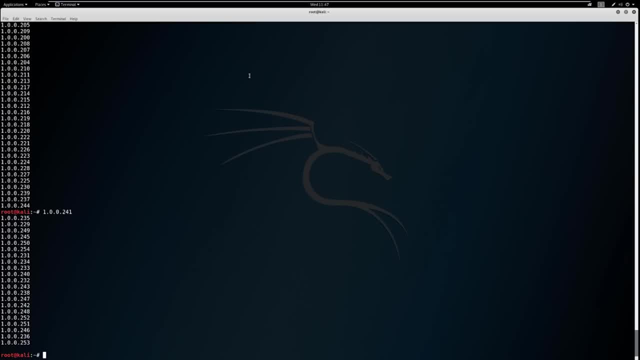 just need to know, hey, what we're doing here- very basic script for ourselves and something that we're not going to be able to do, So let's go ahead and hit enter And we're going to say to remember: Okay, so let's clear our screen. Last thing I want to show you: So we've been able. 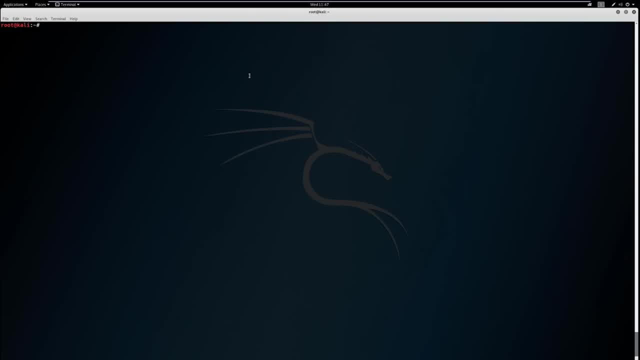 to write a script out, But we can also do looping in one line, And this is where it becomes kind of fun. So we have this IP list. right, We did cat IP list dot txt. Now let's say we've got this IP. 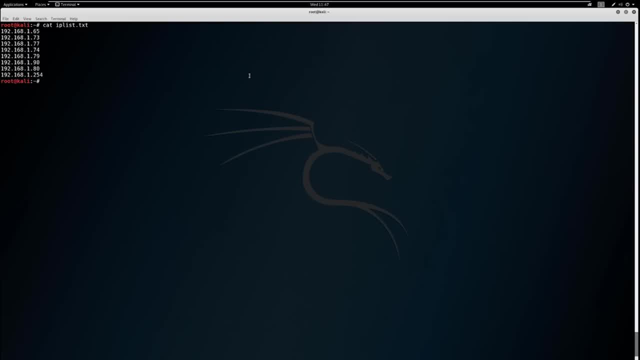 list together And we want to do an N map scan on all of these IPS. Now we could just say: and map and type in the syntax you want and the IP address of it For every single one of these, start a new tab and let that happen, Or you could do something in a for loop So we can write the 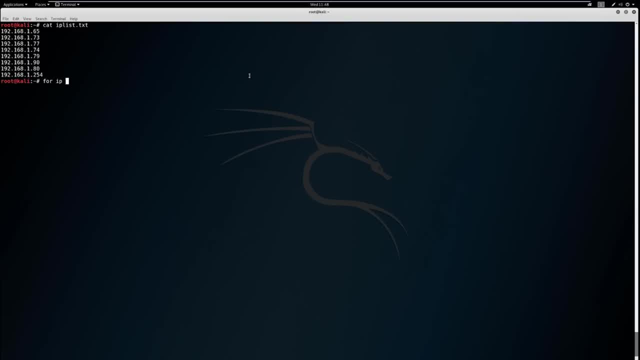 same for loop that we did before. we're going to say for IP, And then what we're going to do is we're going to write a dollar sign and we're going to cat the IP list dot txt. So all it does is it's bringing out this list that we have here And it's saying: okay, for this IP. 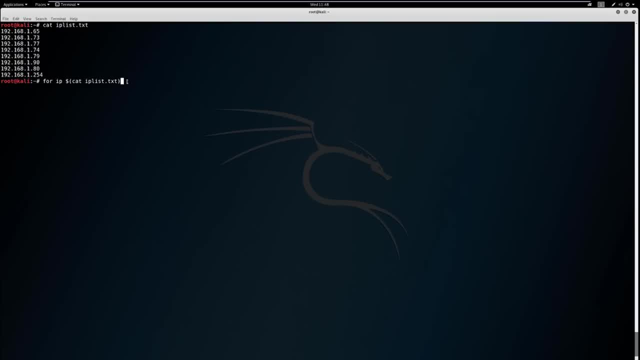 this IP, this IP, etc. we're going to run through all of these. That's what the loop does, right? Okay, we're going to do our semi colon And then we're going to tell it to do something right. 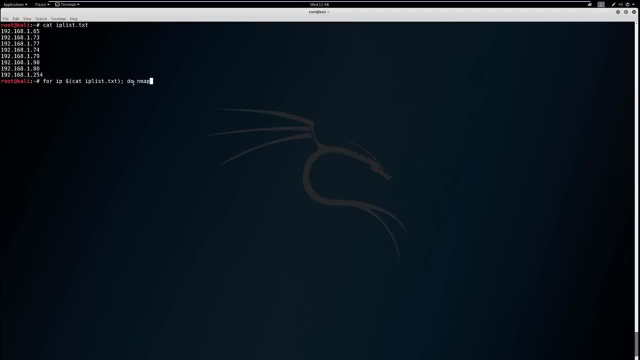 So what do we want to do? Okay, let's run an N map script. So we're going to say do and map And we'll ping or we'll do a port port 80 on all these and we'll say: stealth scan that on port 80.. 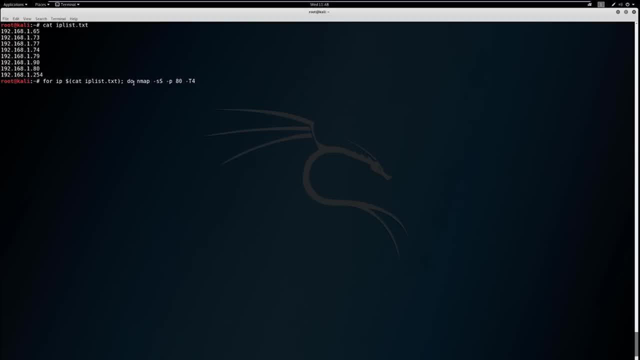 And we'll do t four for a speed, And that should be it. So then we can do done like this and let it run through one at a time. we can also do the ampersand and let it run multiples like this: we can hit enter and. 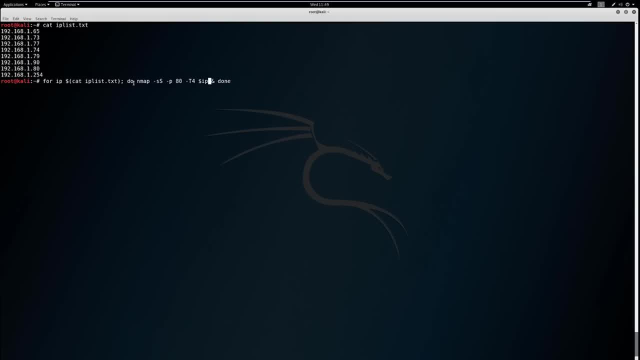 see what that does. But I also forgot one thing here: got to declare the IP address, So let's talk about it real quick. So we've got a very, very simple one liner- And you're going to see one liners a lot if you get into ethical hacking- and just allows us to do things quickly. 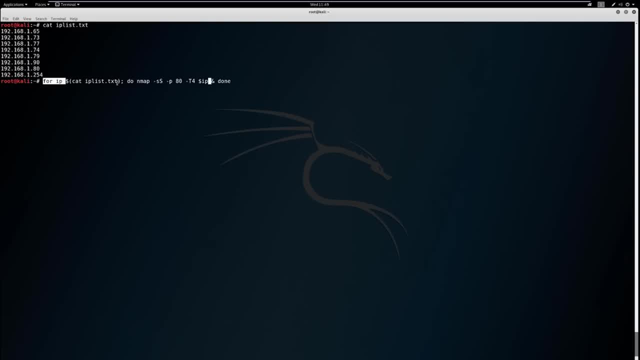 and scripted. So we got four IP address in this list. So every IP in this list we're going to loop through. When we do that loop, we're going to do and map, we're gonna do a quick stealth scan a port 80. 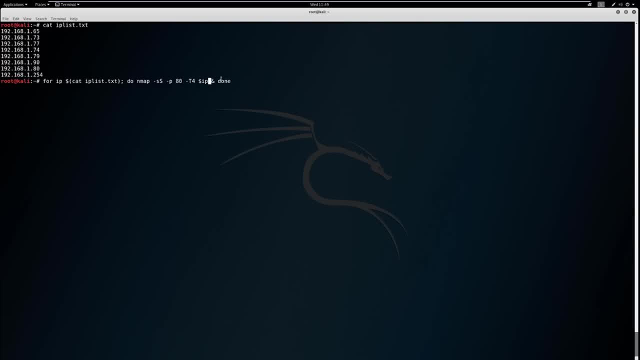 t four And we're going to say: declare the IP address. If you're not comfortable with an map, that's okay. This is purely an example and something you will see in your career. I will make a scripting video at some point for an map and we'll cover an map more in detail. 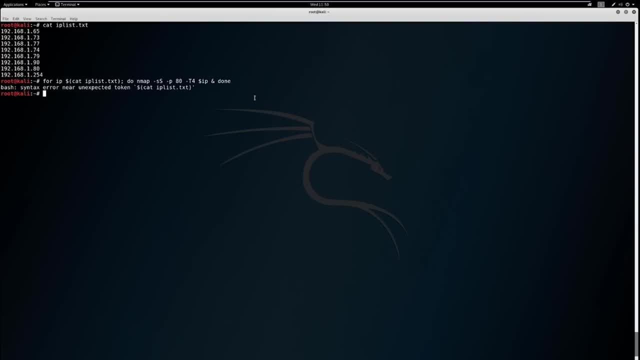 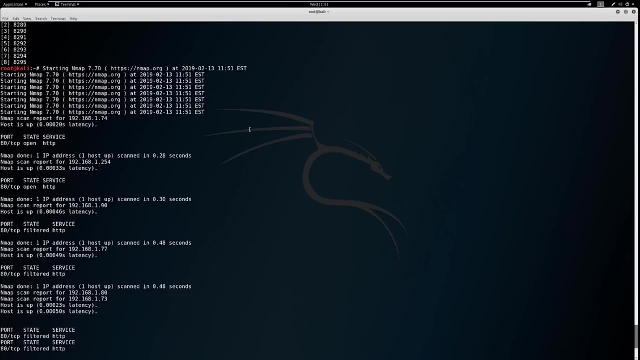 So let's go ahead and just hit enter. Okay, I messed up my syntax, So what's going on? Okay, So for IP in: this got deleted. for IP and cat IP list: Let's try this one more time. Okay, So we just did all these scans, seven scans at once, And what we did is: 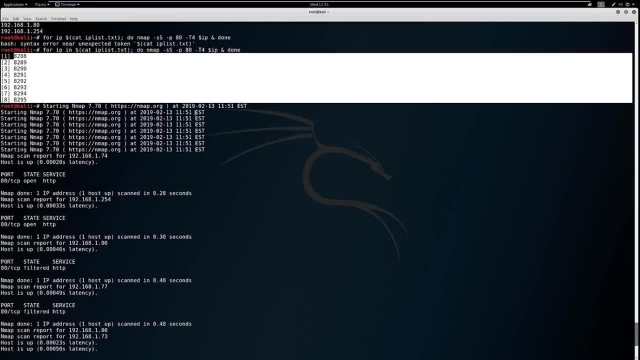 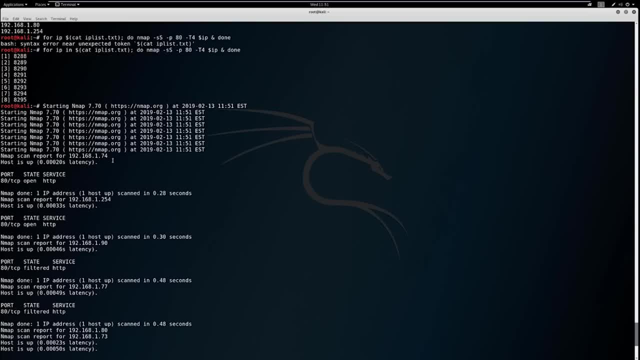 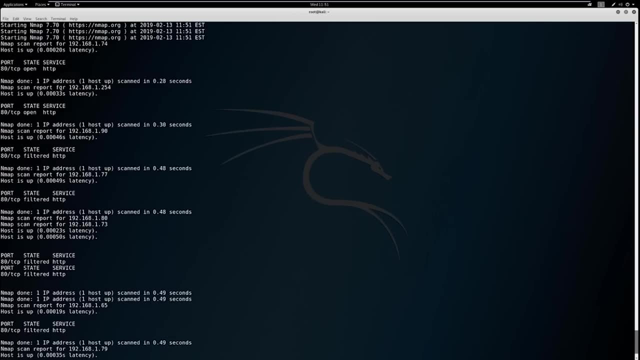 see, these are the processes that are starting. So it started up eight processes, actually, not seven, And it's just running through this list doing the scans And we're going to go ahead and just kind of look at it. So it says, okay, on 1.74 is at open, it's open, Okay. And then on 254 is at open. 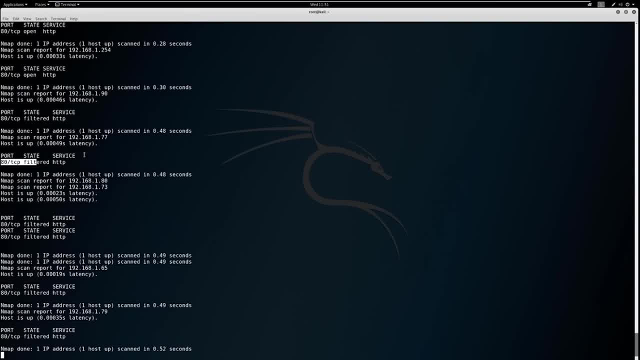 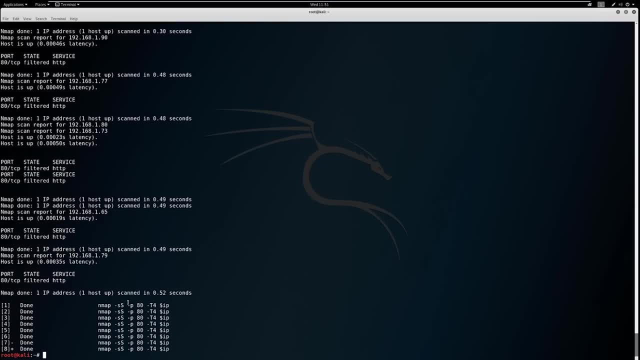 it's open And then you see filter down here where it's not running filtered, filtered, same thing. So we can hit Ctrl C or hit enter for done, And that's pretty much it. So what we just did is we ran a map scans at one time instead of having to copy and paste these. So it's just a little bit. 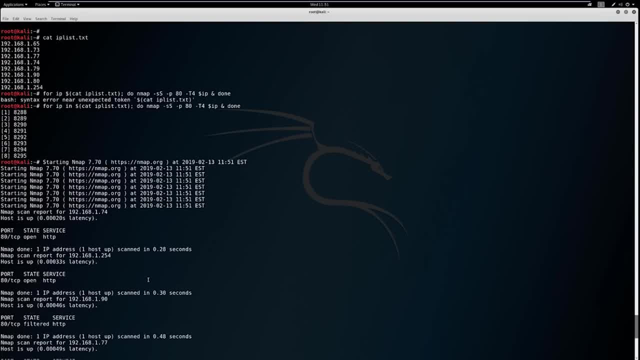 more advanced, but be able to know a one line for loop is a really, really important if you go into penetration testing, And it's just important in basic bash scripting as well. So that's really it for this lesson And that's really it for this course. 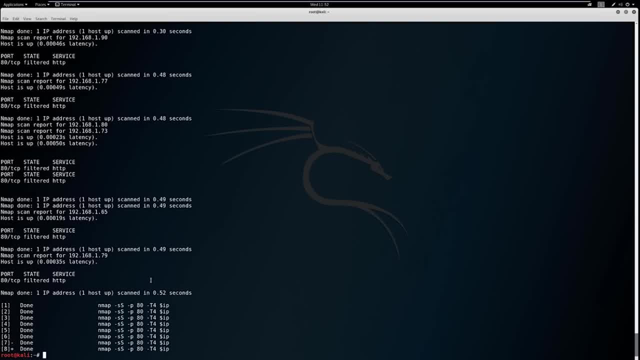 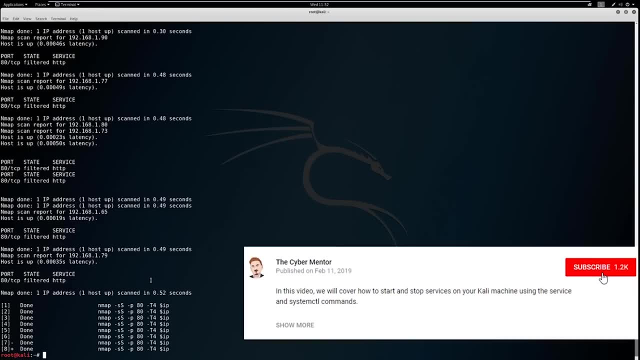 So I hope you really learned something from this course. If you did find it valuable, please do share it with others. Please subscribe. If you haven't, please do like the video. word of mouth is the best thing for me. It helps me grow my channel and helps me give. 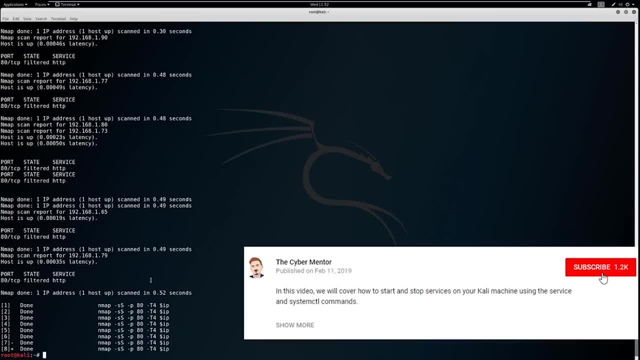 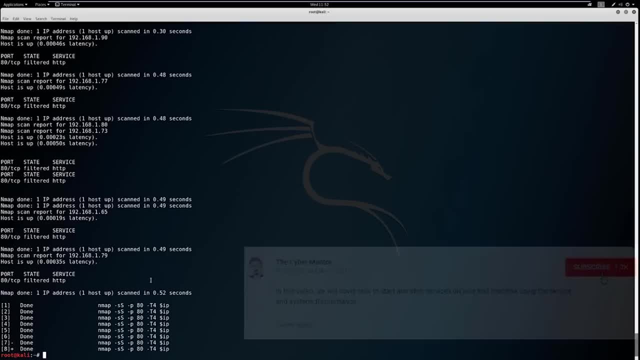 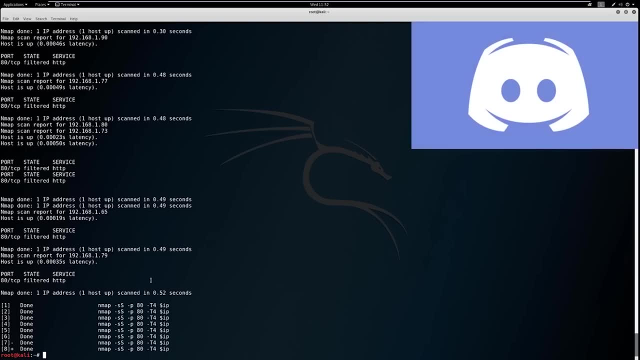 content back to you as I get more feedback and I grow as a channel. So I'm looking to do more courses in the future and appreciate you taking time with me. If you like this course and you want to chat with me, check the descriptions down below. I've got a discord channel. we've got quite 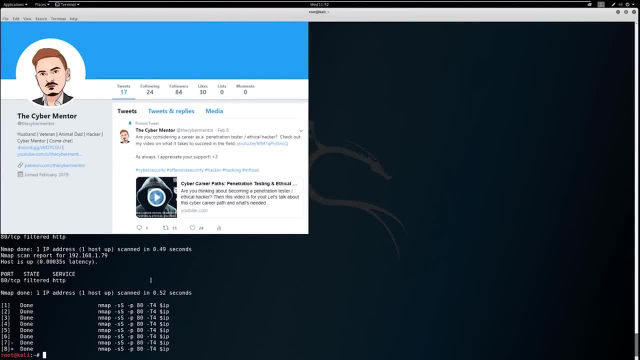 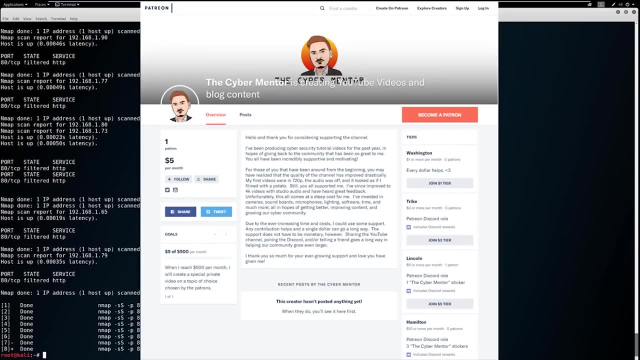 a few people in there And I've also got a Twitter if you want to hit me up there. Lastly, I do have a Patreon if you felt like this course is valuable and you'd like to support me. Any dollar goes a long way for me. recording equipment, recording software- all that's very expensive. 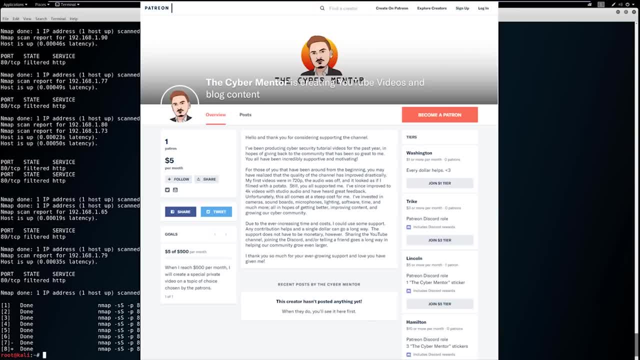 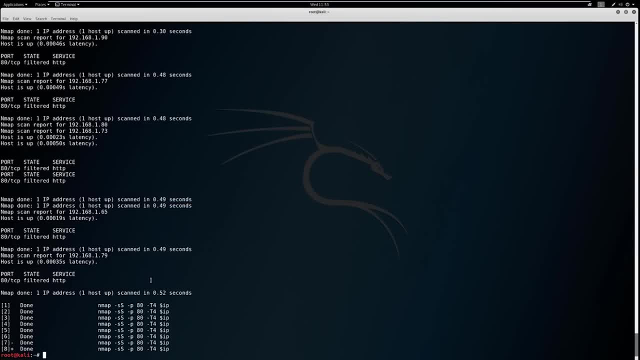 And the time spent on this is also very detailed, long hours. So if you want to support me or or anything, a like, subscribe etc. goes a long way. I appreciate you taking the time to watch this course, And until the next one. thank you so much for joining me. 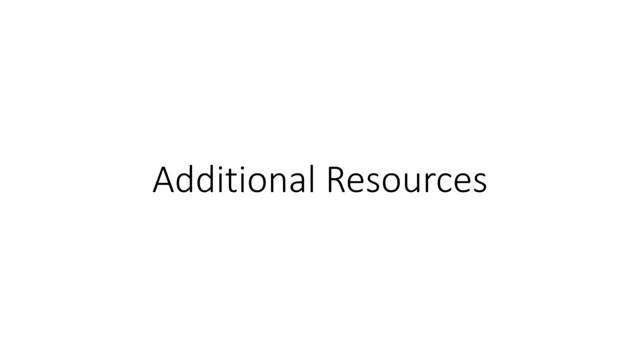 Alright, and now some bonus material. So I'm adding in some additional resources. These are for those of you that want to continue on. You've learned the Linux now and you're like, hey, I really want to be a pen tester. I think this is for me. I'm going to provide you a whole 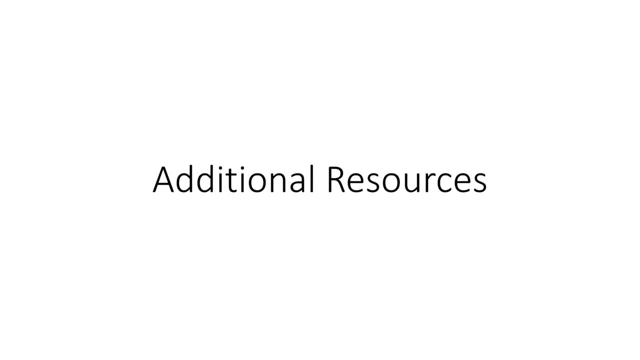 lot of different resources here, So take notes. These are some of the best resources I could think of for those wanting to get into the field. I'll briefly cover each of them and then leave you at it to do your own research and hopefully see you in the field someday as a pen tester. So let's take 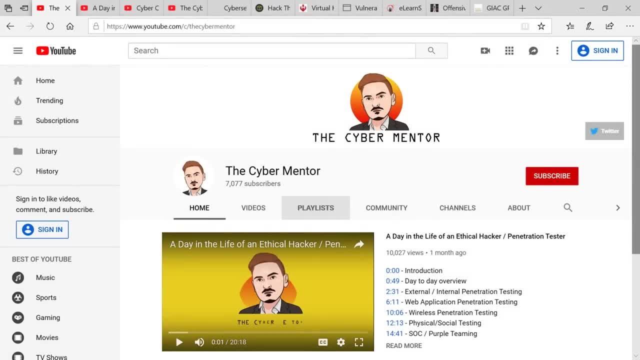 a look at some of these resources. Okay, so first resource is a shameless self promotion, And I only do this because I do think that I'm a valuable resource. I'm trying not to be biased here, But I've got some good. 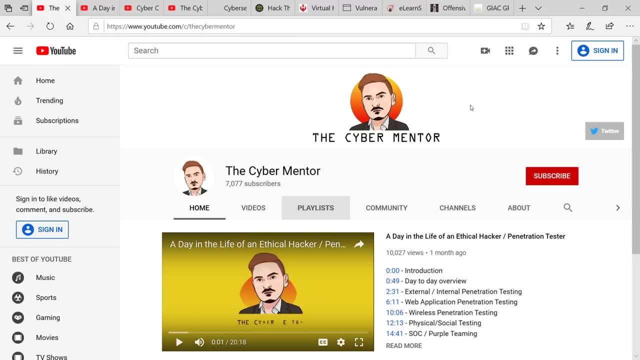 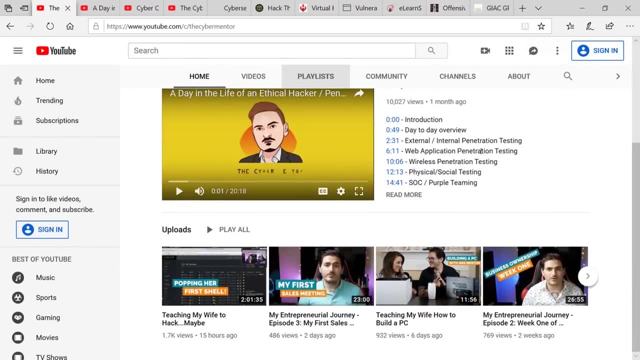 good stuff that's completely free if you are interested in it. So if you come to youtubecom, slash C slash, the cyber mentor, you can come to my page here And you can check out all the videos I have. One video is a day in the life of an ethical hacker. 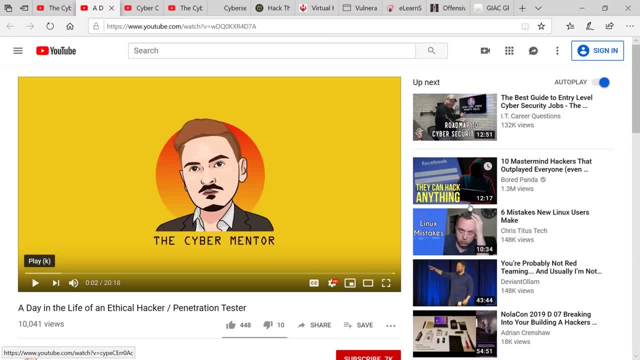 So if you want to know what it's like to be an ethical hacker, if you're still not in the sure, if this is the field for you, this might be a video for you to view. talks about the day in and day out stuff that you might do, what kind of assessment work you might be asked to do, and 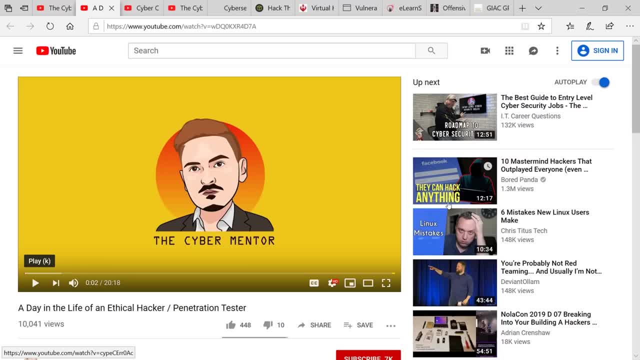 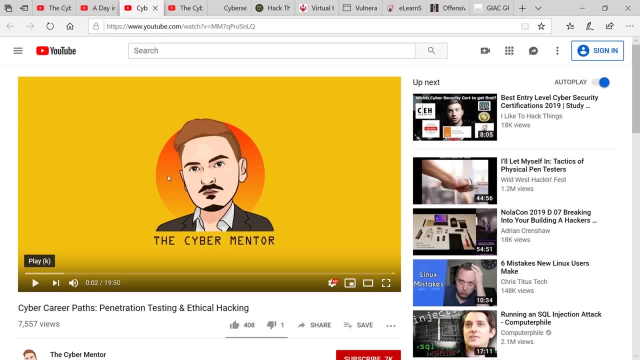 what it's really like to be a an ethical hacker. On top of that, I've got another video on cyber career paths about penetration testing and ethical hacking. So if you're looking to get into the field and you want to become a pen tester or ethical hacker and you're not quite sure where to go, 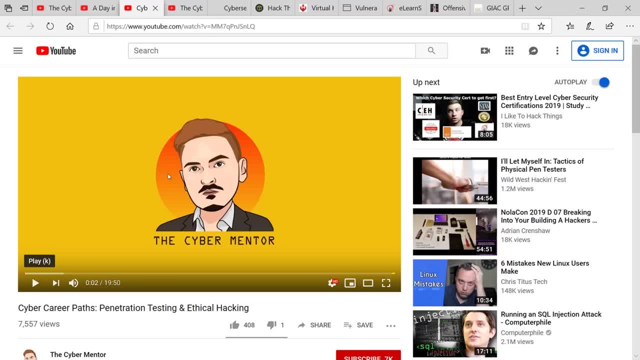 this is probably the better video For you. it kind of talks about all the knowledge that you'll need for a junior perspective and really the knowledge that you'll need to be successful in the field, including certifications, etc. So if you're watching this video as an additional resource, 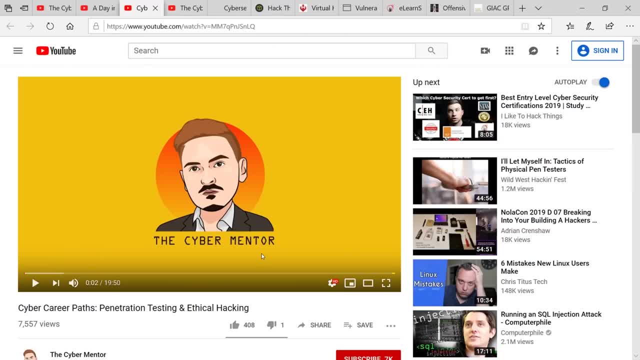 this would probably be additional resource. Part two is a good way to call it. this is the one like really detailed on penetration testing and ethical hacking. On top of that, over here I've got playlists, So if you come into the playlist I've got a few courses. 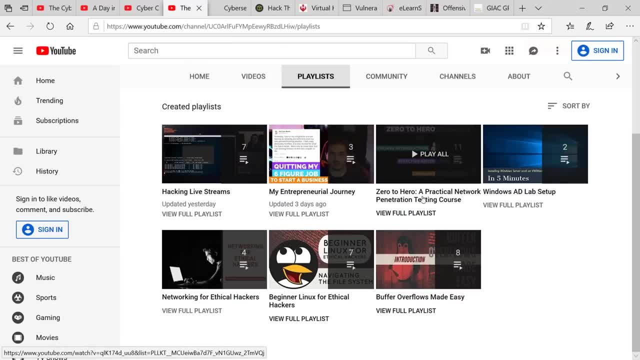 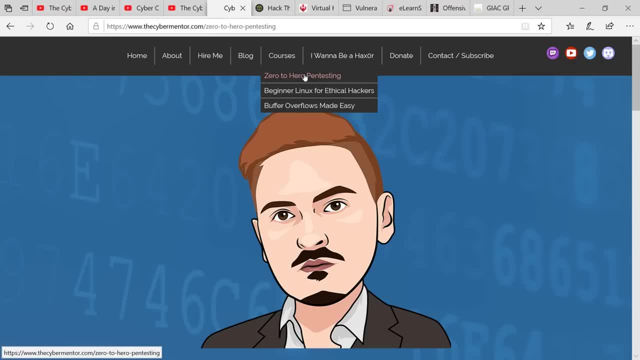 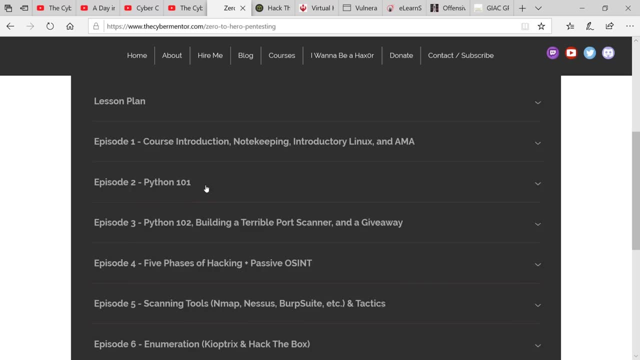 most importantly is our zero to hero course. So if we come to the cyber mentorcom and you go to courses over here and you go to zero to hero pen testing, you can find more information on the syllabus. So I put it into lesson plan as well here. 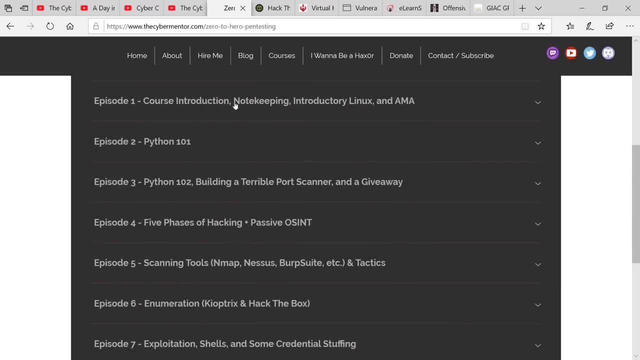 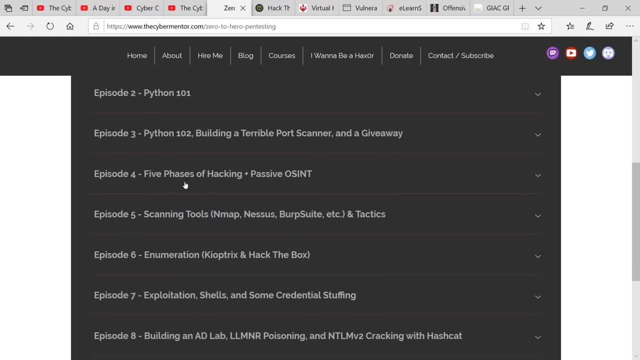 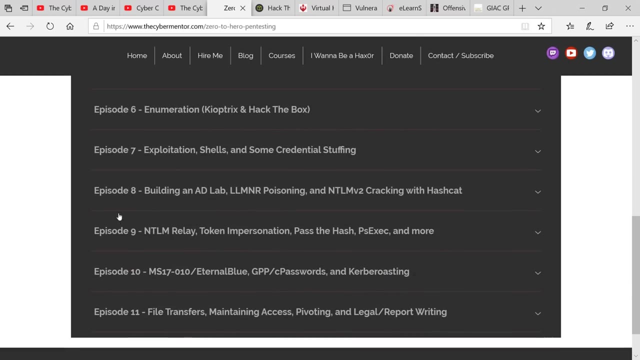 But there are, let's see, 11 episodes. we start with Linux, kind of like. you've already learned note keeping, some introduction. we do Python for two weeks. we do information gathering, OSINT, recon, scanning, enumeration, exploitation. we do internal attacks as well. So we'll build out an Active Directory lab And we'll learn how to do. 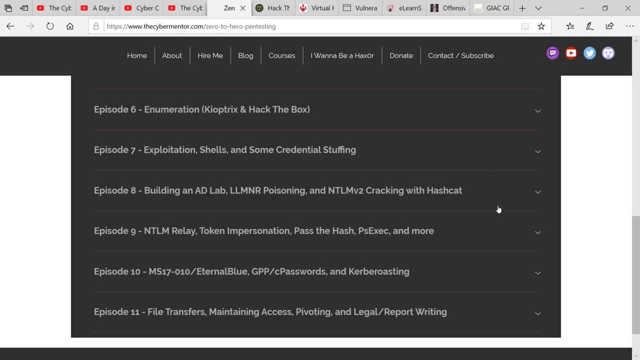 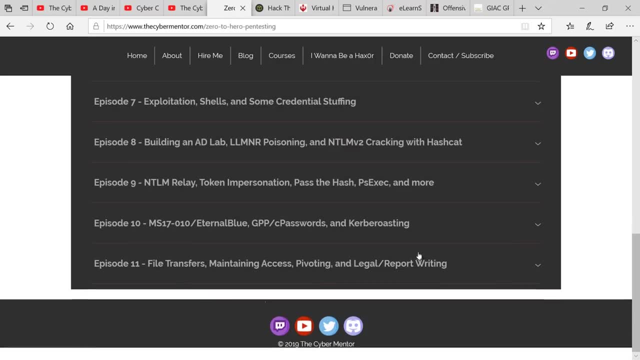 these internal attacks that aren't really taught in a lot of courses, And then we'll end it with some file transfers, maintaining access, etc. report writing as well and career advice. So this is like my complete course. it's called zero to hero, to take somebody from from a complete 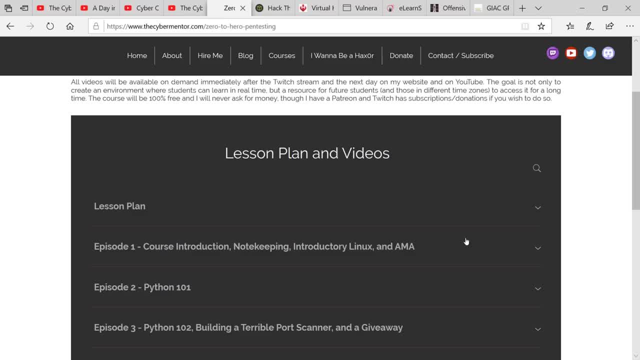 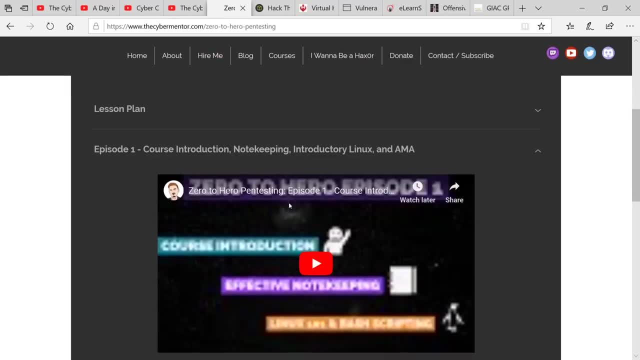 zero and bring them into a hero where they can start doing some pen testing on their own. so again, if you're interested in that course, you can come to my website and check it out. with the lessons plan you can just click in the tab and play the video, or on my youtube channel you can click right. 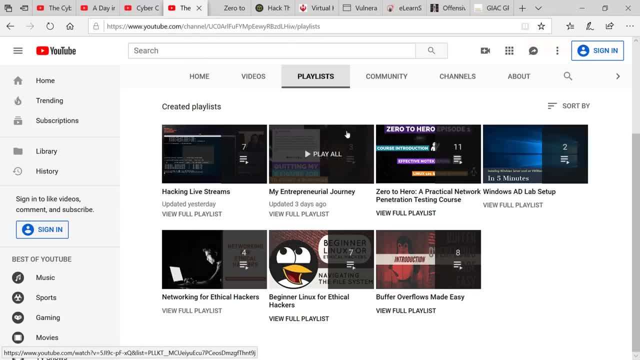 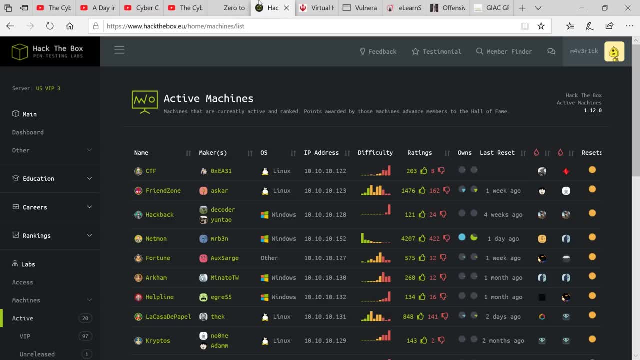 on the playlist and play it from there as well. so, leaving the shameless self-promotion, let me talk about some more cheap alternatives. hack the box is a great, great alternative, if you're just getting started. so for hack the box, what it is is: it's a series of vulnerable machines, so you could think. 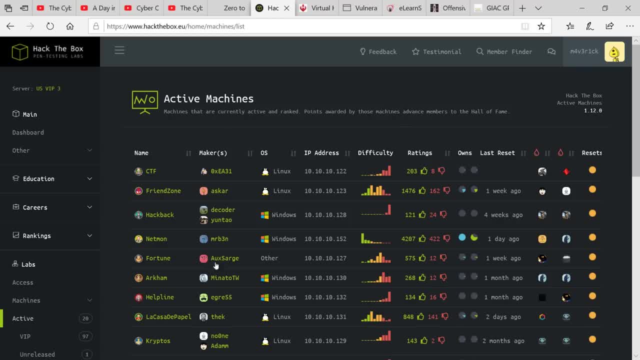 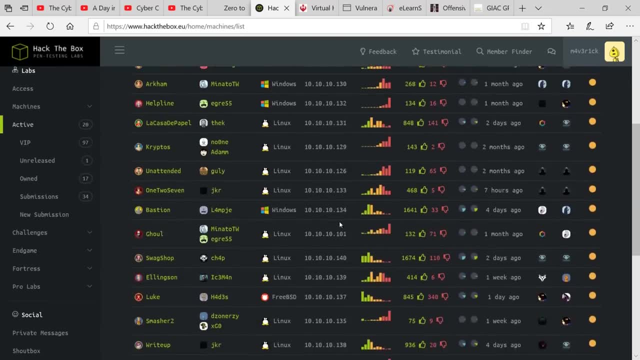 of it almost like a game. so if you want to do some hacking, this is a great place to just start practicing and learning the ropes. what we can do is like say we could pick something on the easy side. you want to look for something like that's more green right on the left, because that shows. 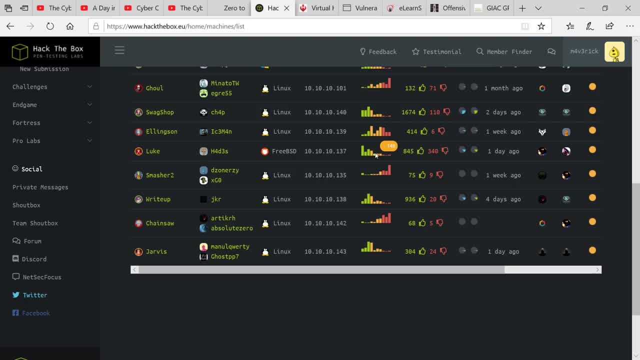 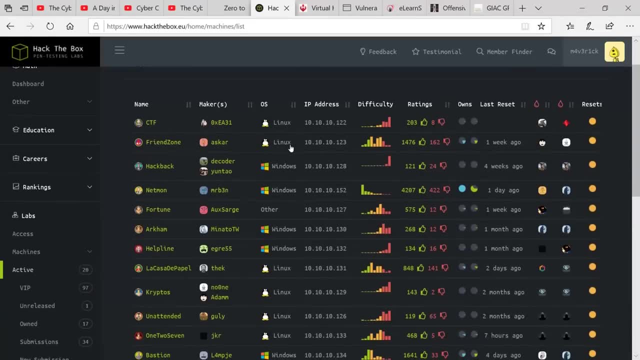 easy. you would pick a box like this, you would scan against it and you know. if you don't know what i'm talking about, that's fine, but you would scan against it and try to find vulnerabilities and hack it. So, really, really great website If you have the 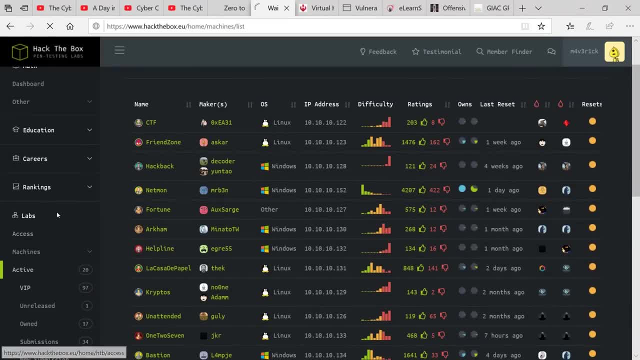 VIP. they're starting to move it. It's in beta right now, but they have 20 boxes that you can attack on active side and 20 in the VIP. But the nice thing about the VIP is they're about to open up all 97 that have been retired. So they retire one every week and they bring a new one in, So 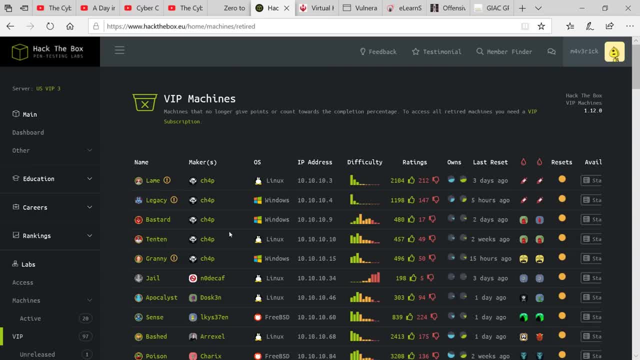 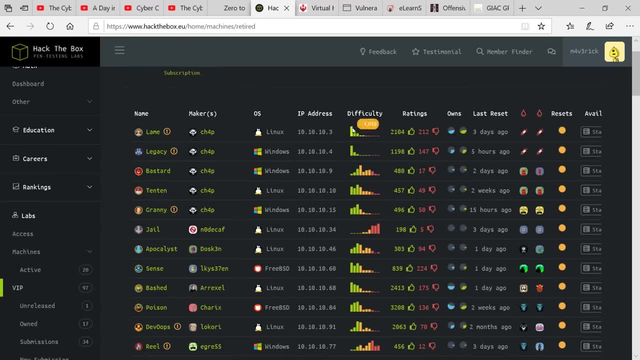 you gain access. It's like $13 a month. This is free, completely free platform if you don't want it, But this is $13 a month for the VIP access And you can come in here and do some of these machines that are super, duper easy And if you click into them, they'll have write ups for them. 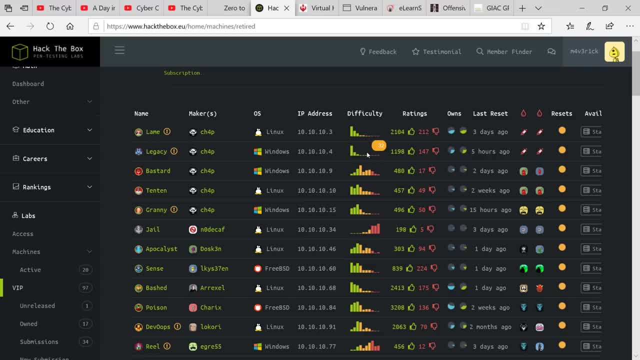 and they'll also have video walkthroughs for a lot of these machines. So that's a really, really great stuff, right? If you have no idea what you're doing, this is a great place to start, because these retired boxes are boxes that have already been done. You can watch how somebody 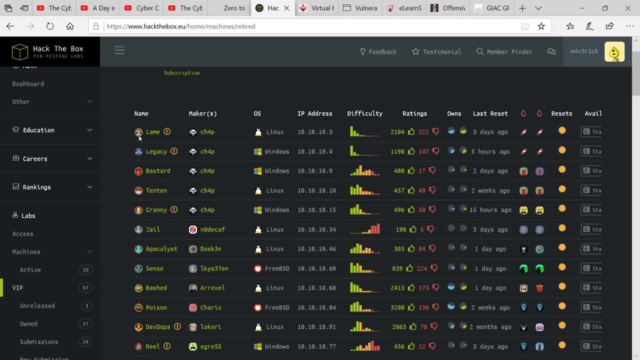 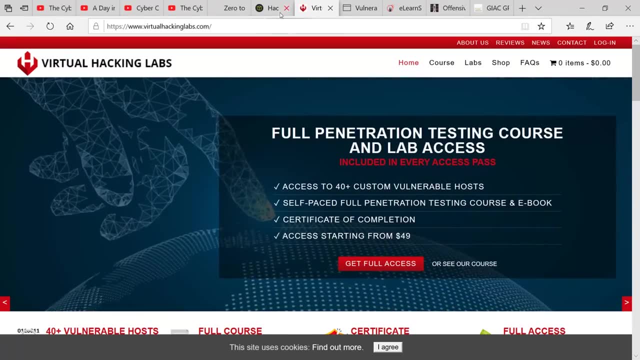 else did them. You can learn their methodology And this is really good for just getting the basics down Understanding. you know some basic hacking. Same thing here with the virtual hacking labs. It's very similar. They've got a labs, they've got a course and they've got different pricing. So you 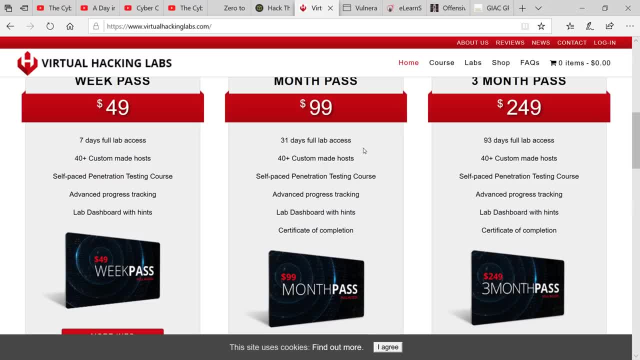 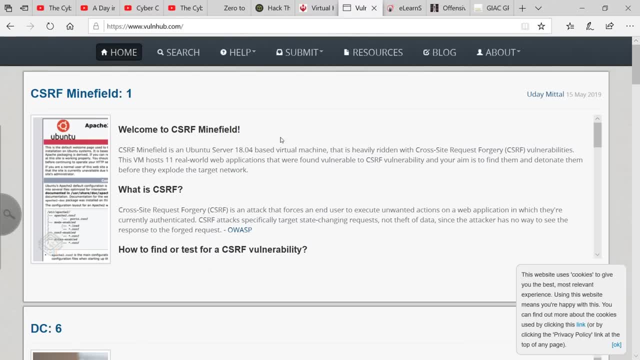 can try these out if you're interested in them. So they are, you know, just alternatives to just practice online. Then you've got VolnHub as well. You'll have to search through this and try to find something that's like beginner level or Google online, which, which are realistic boxes or what. 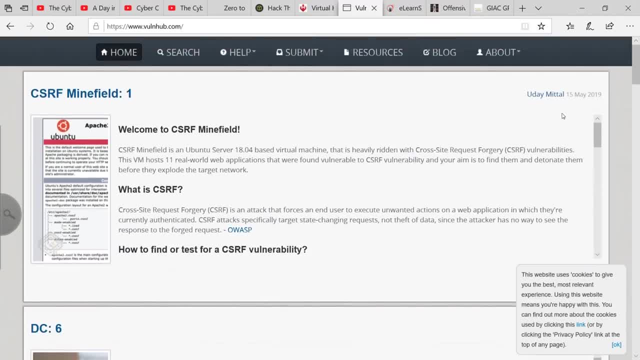 are good boxes on VolnHub. Basically, you just download the VMware file and you play it on VMware and you try to attack the machine. So you download a machine, you try to attack it And these are intentionally vulnerable machines. All these right here on these top three. 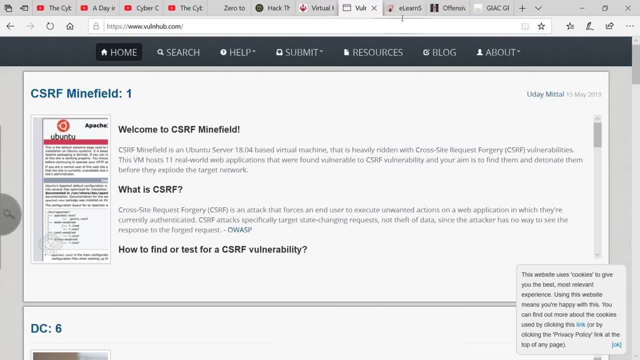 So let's say that that's not really where you want to start. You think maybe you could use a little bit more handholding and you like a certification to come behind it. I'm going to show you the top three in my order that I think for pen testing, at least at a beginner to me- are going to be kind of. 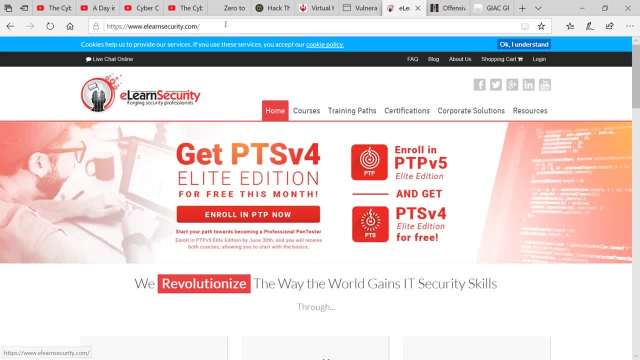 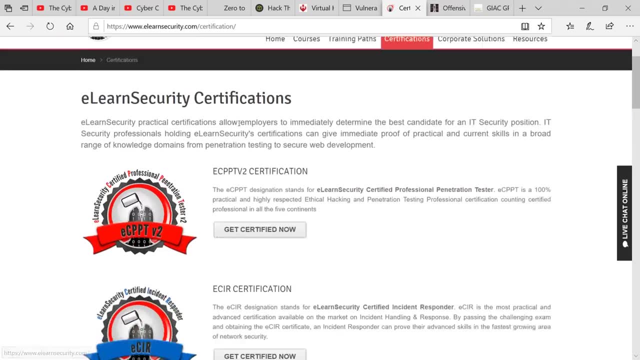 large boxes So you can basically download the VMware and you try to attack the machine and you download a machine tier level what the top three are. so eLearn security gets number one slot in my mind if you come into here and you go on to certifications. so they've got a couple different ones: the eCPPT. 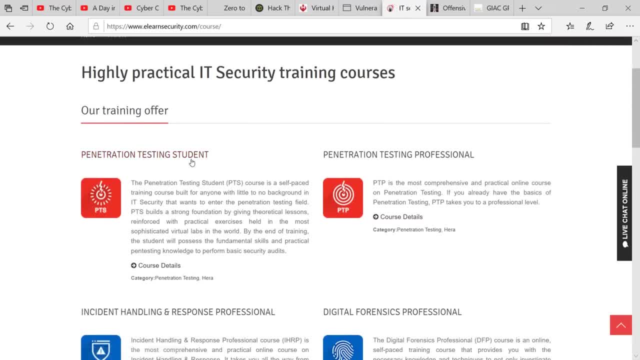 or actually let's go to courses. so the penetration testing student and the penetration testing professional. the student is for the beginner, the professionals a little bit more advanced. it leaves off where the beginner ends. so if we come in the student, you can see some of the things that you'll. 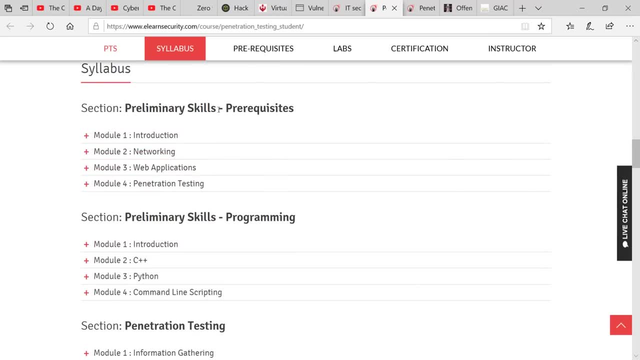 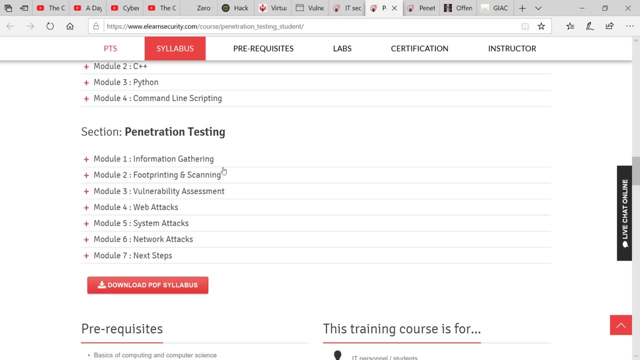 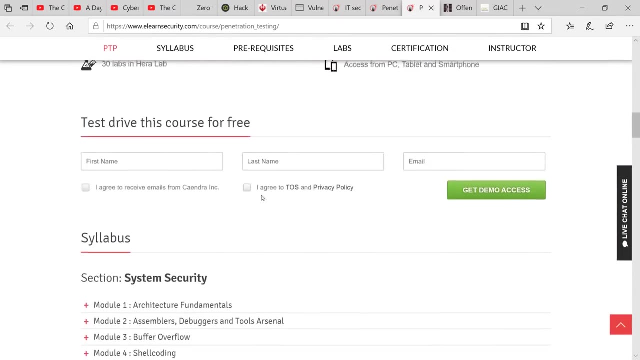 learn. so they've got you know. it talks about the preliminary skills that you might need and teaches you those. it's got some programming and then just the basics of penetration testing, but it gives you an idea what it's like. on top of that, this ptp course they have is like 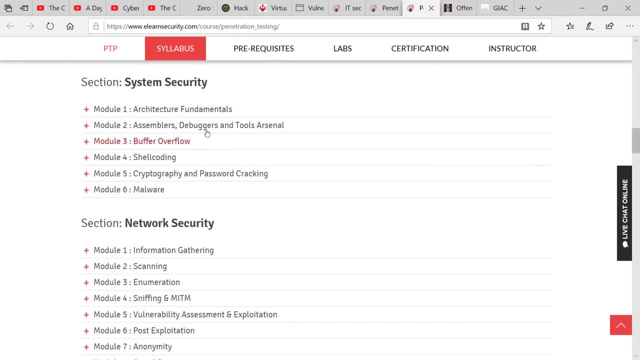 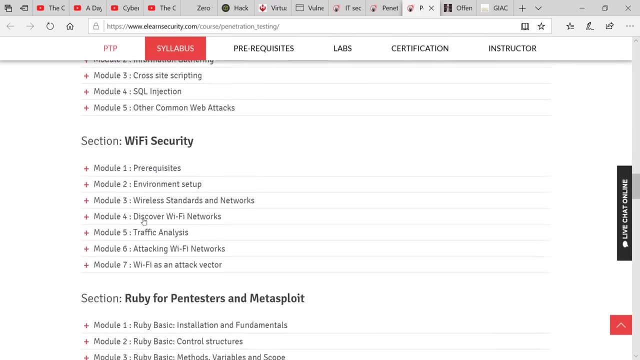 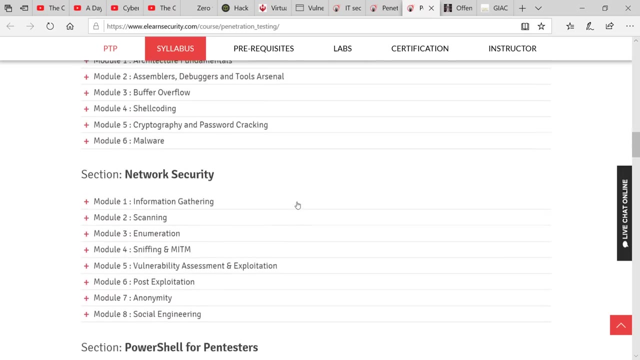 more in-depth, more advanced. you start getting into assembly language and buffer overflows. you get into network pen testing, some powershell linux web app, wi-fi, some ruby for metasploit. so i think this is really well-rounded, really up to date. the downside of this course is that it's not um, it's not really well known on the hr side of things. 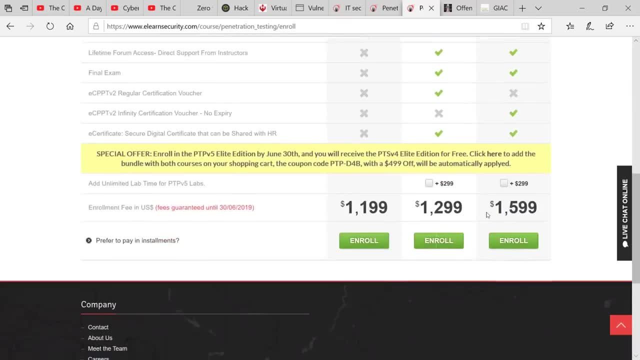 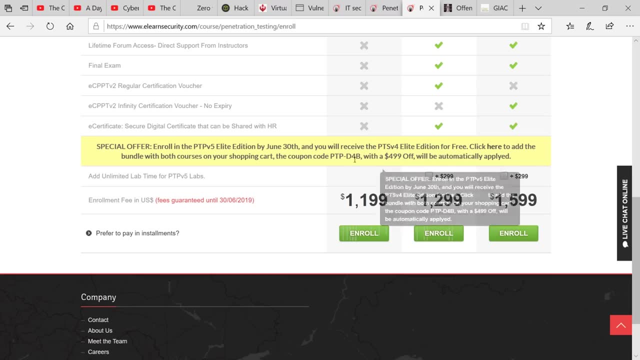 so and then the pricing can get a little expensive on the elite side. right now it's sixteen hundred dollars, uh, the cheapest is the 1200. i would at least get the middle tier, uh, but as of right now they're offering that pts and the uh ptp. if you buy the ptp they give you the pts for free. 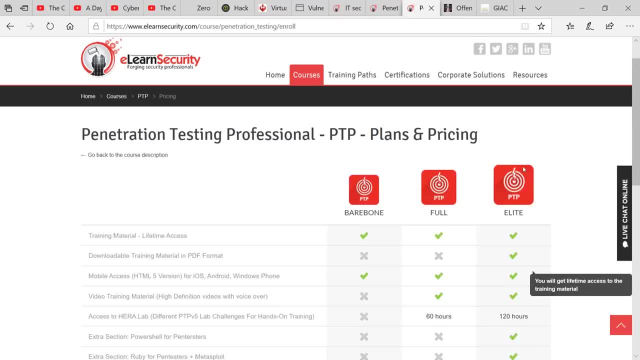 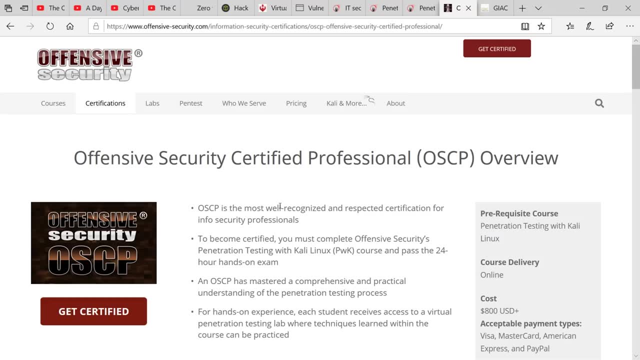 but, um, that won't be going on much longer, but you can always hold out for deals like this as well. another resource in a very, very well-known resource, probably the best certification in terms of being known is the oscp. so it starts out at 800 bucks, as you can see here. 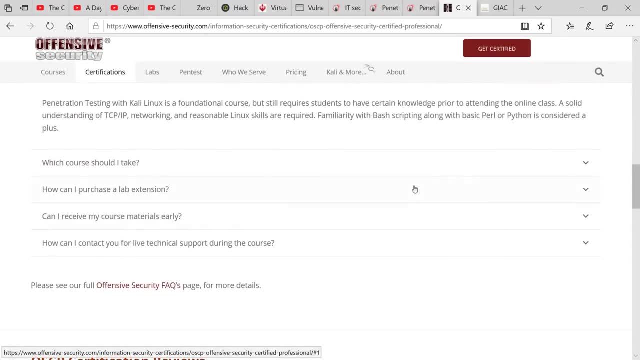 you're probably going to spend more money than that, because that's just 30 days. so the nice thing about this is it comes with labs. there's a certain amount of machines in there that you can try to hack against, sort of like a hack the box, but it's an environment. 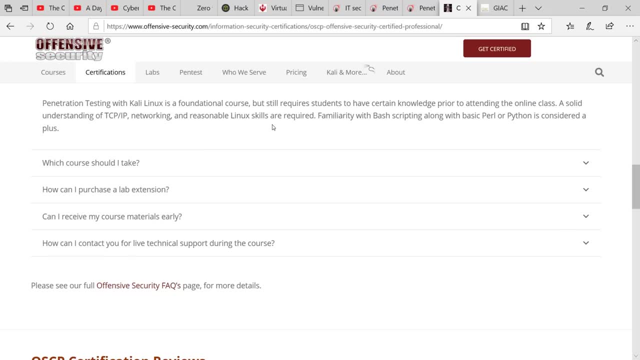 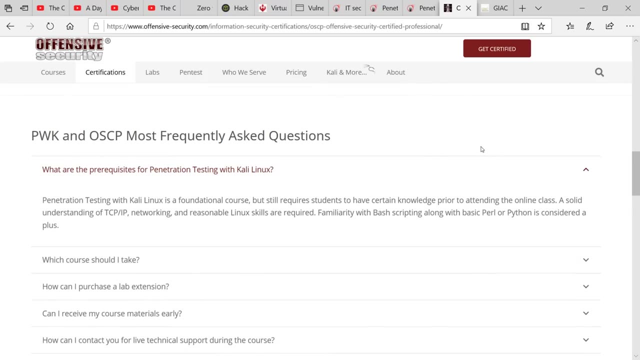 so you can, you know, just attack whatever you feel like and try to uh navigate your way through the network and then, when you are done and you want to test for the certification, you have to actually hack in an environment of a set number of machines you have to hack against and you have to be. 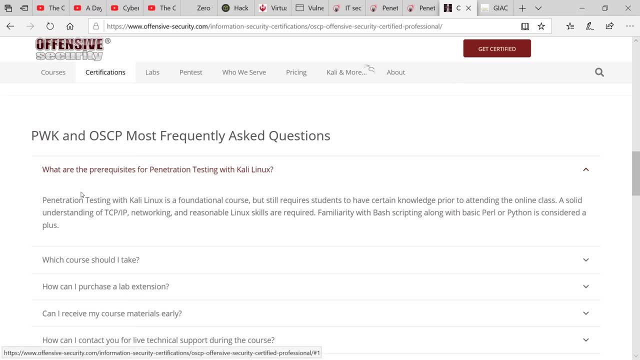 successful in hacking those machines to get your certification, so it's considered one of the more difficult certifications out there to achieve and you'll see it come up a lot of times in hr or java and you'll see it come up a lot of times in other applications that they want this oscp. 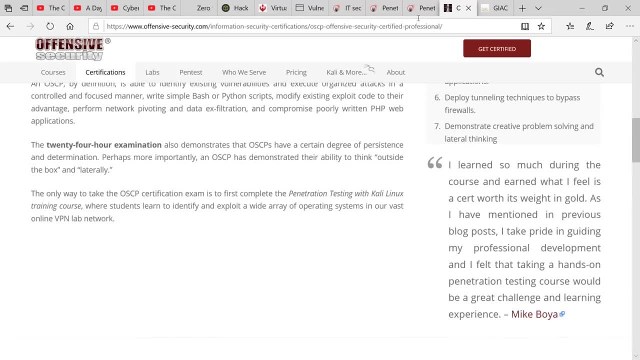 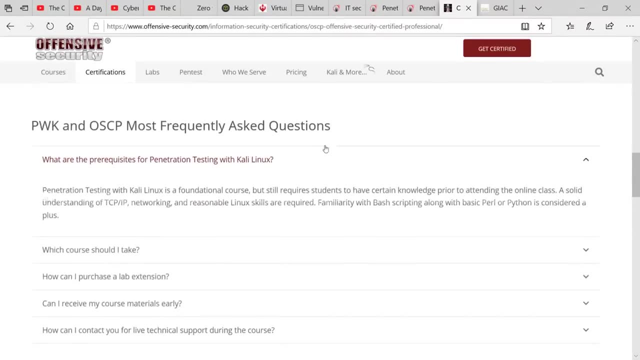 so this is something to look into and consider as well. the cost isn't as bad as the e-learn, but the con here is that office of security courses haven't been updated in five or so years, so you really need to. um, you know, it's kind of the the best of both worlds if you were able to do both. 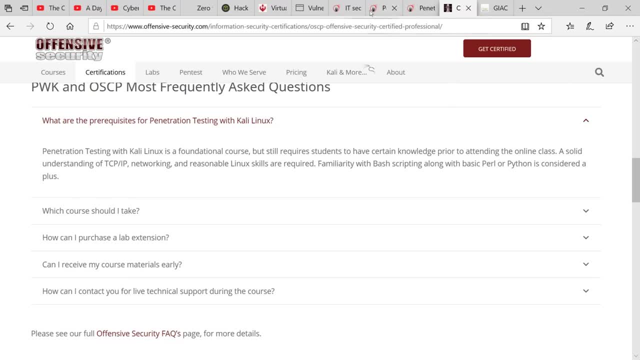 but this one will get you into more doors, this one will get you a little bit more current, but there are plenty of resources out there. all these tabs. i've shown you that you don't have to spend a money to get this stuff. these are more things that, if you want that certification, you want that. 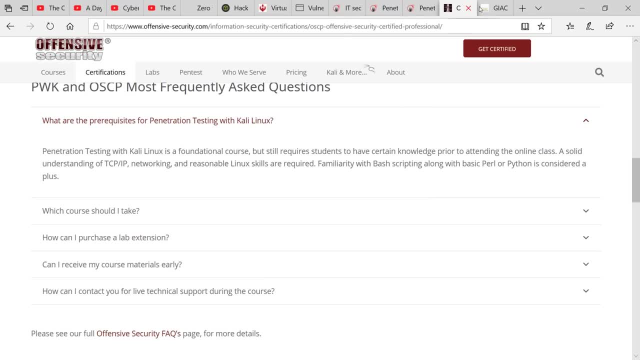 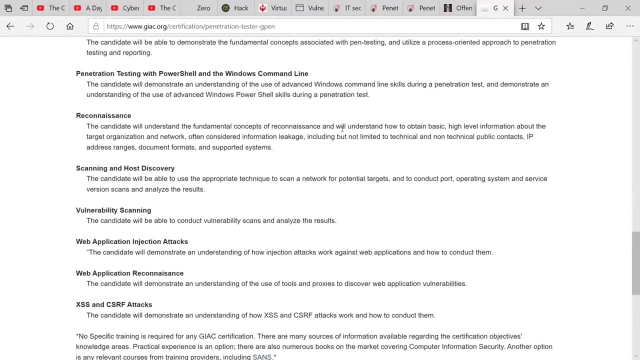 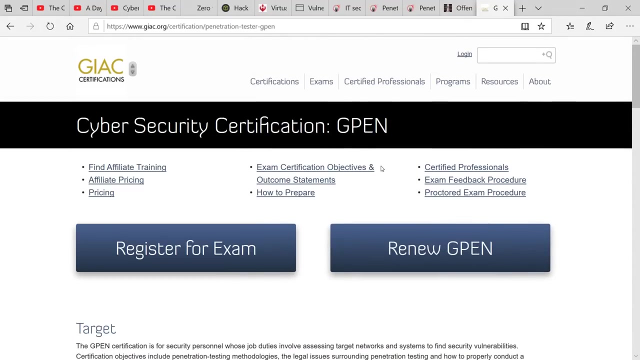 that coursework, that knowledge, these are great resources, all three of these. so last is the gpen. now, the gpen is just an exam. um, by itself it's seventeen hundred dollars. it is by sans right. so this is showing geiac. you actually have to take the corresponding. 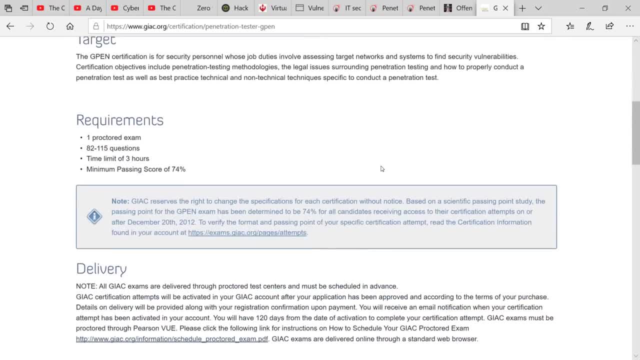 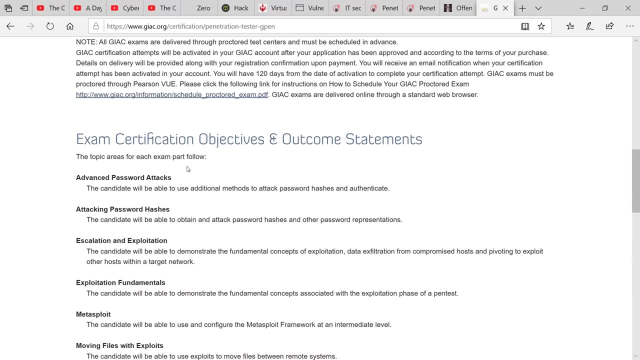 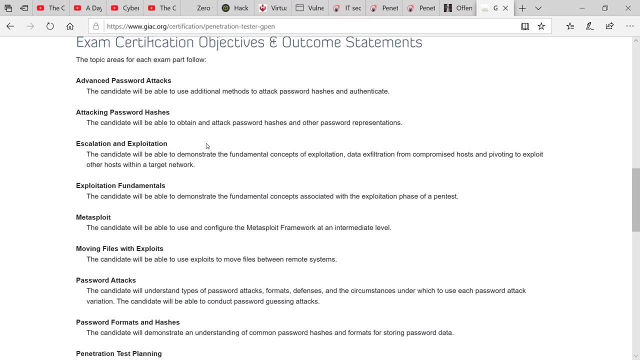 sans course that goes with it, um, and that course is upwards of six thousand dollars, unless you can get a employer to pay for this sans certification. probably not the best, but the thing that i like about sans is that, uh, it stays up to date. they are constantly updating their 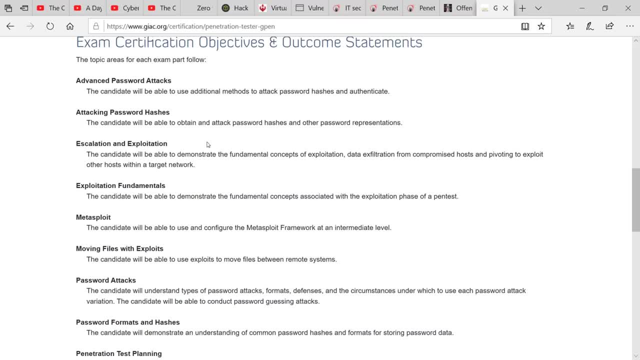 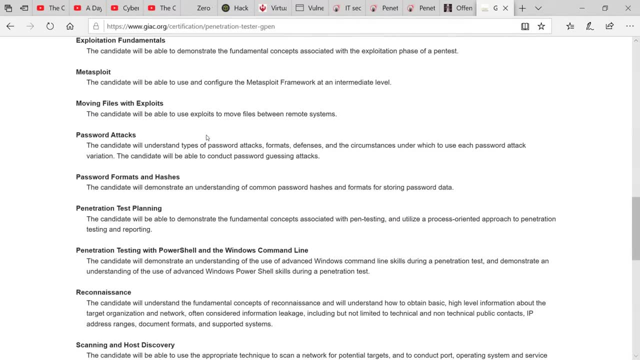 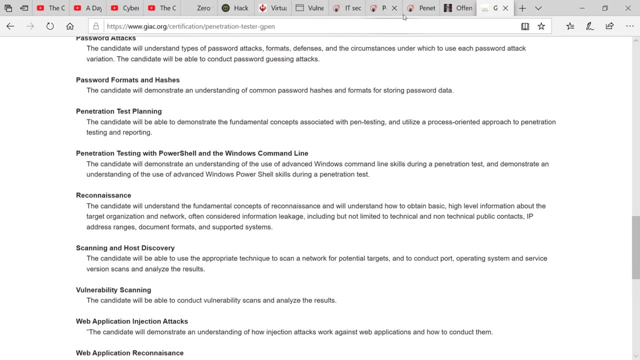 courses and that they look good on a resume. it's one of those really high tier, high level certifications, um, and the exam, from what i hear, is actually pretty good. it's not a practical exam, but it's a fairly good exam and the nice thing i didn't mention- e-learning security is also practical. 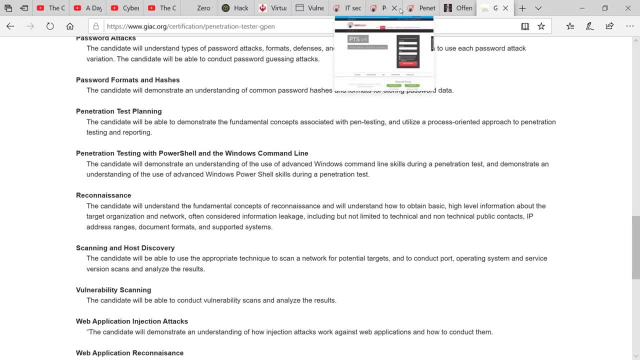 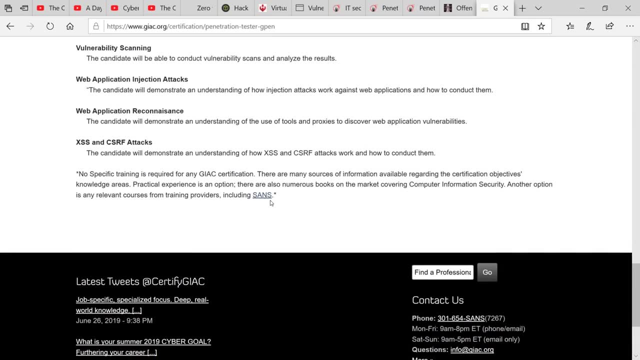 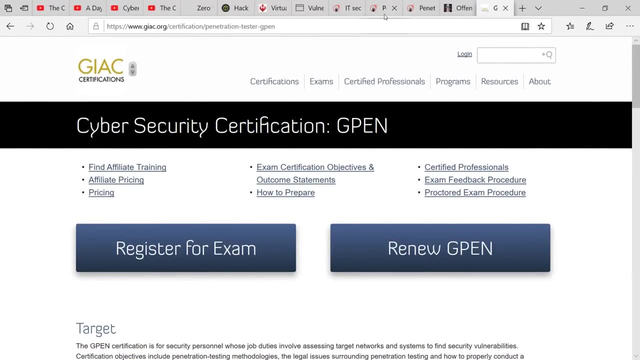 this oscp is practical. the e-learning security exam is practical. you have to hack your way through to uh to pass and write a report as well. this one is a multiple choice exam, i do believe, so these are three certifications that you can look into if you're wanting to go down that route. i would start. 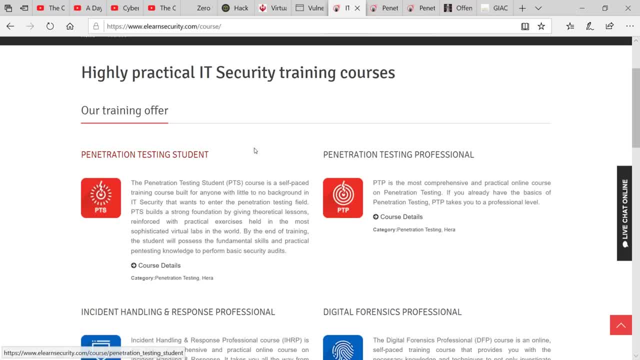 with the pts, if you can. it's dirt cheap. um, you know, if i have to make a recommendation just to make sure that you're you're really interested in this. if you know for sure and you want to do that, pts, ptp, you can go on the e-learning security exam and you can make a choice if you want to go down. 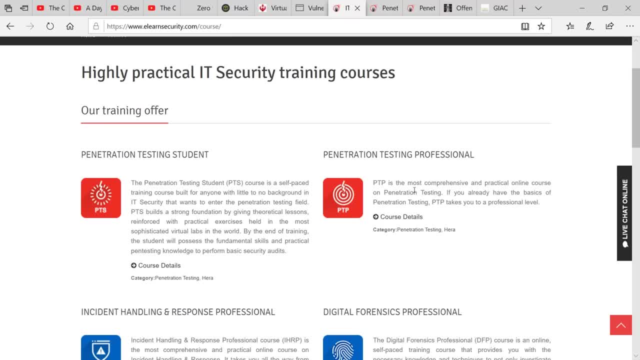 combo. this might be a good choice here, but other than that, i mean the free resources. like i've got my channel. there's a ton of videos. the zero to hero course is like at least 20 to 30 hours of material. uh, hack the box you'll spend a lot of time on. there's plenty of write-ups if you just 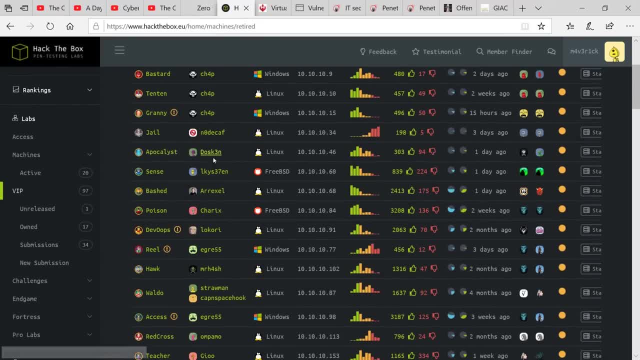 google like honestly, if we go into here and we say, uh like apocalypse here, if you say that and you google that with write-up, you're gonna find the write-up for this or you'll find a video for this or some kind of walkthrough, right? so you just want to look through these and try to try it on. 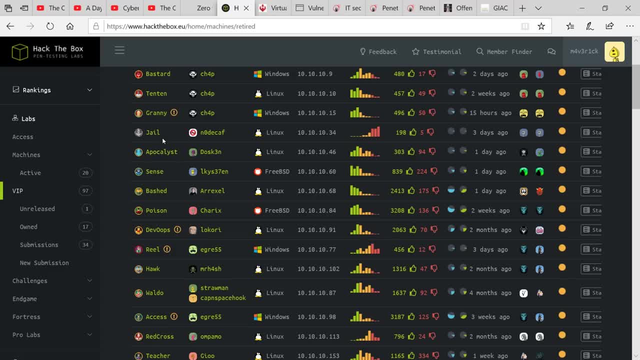 your own and then go back and then watch the write-up and see how you could have improved if you got through it, or where you can improve an enumeration or whatever is you need to, uh, to get better to actually succeed the next time you try attacking these machines. so that is it, uh, you have. 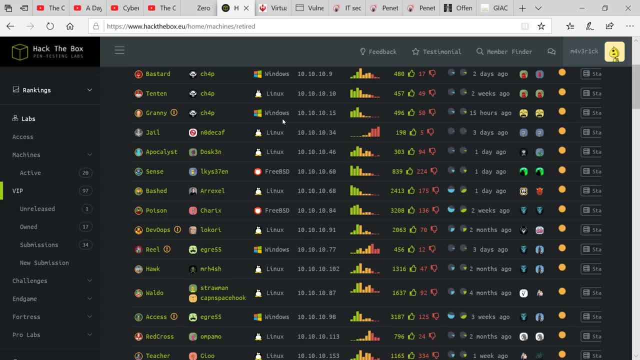 reached the end of this course and the end of the bonus material. if you need anything, i provided my contact info again in the beginning. you can find it on my website at you know, i'm at the cyber mentor on twitter. you can reach me on youtube as well, and i really do. 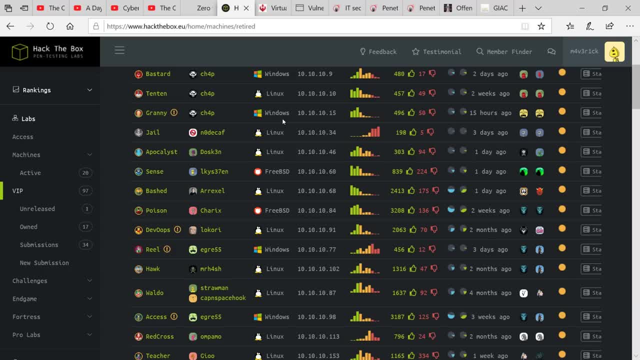 thank you for joining me. i look forward to seeing many of you take the next step from this linux. if you made it this far, you've already gotten through the beginner linux and that's awesome. i hope you take this next step and that you are intrigued by penetration testing, because we need more people. 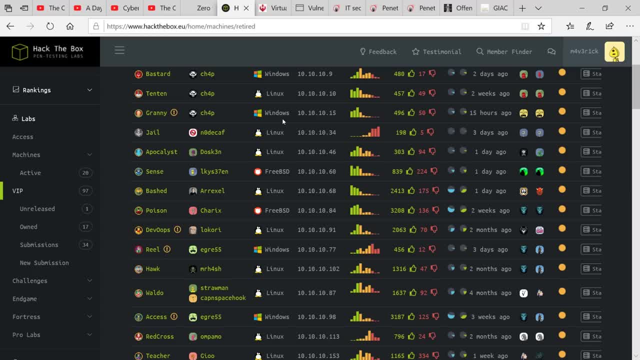 in the field, so i look forward to seeing you guys and girls. uh, come through and and hopefully i'll work with some of you soon and i'll see you in the next video someday. so until next time, my name is heath adams and i thank you for joining me. 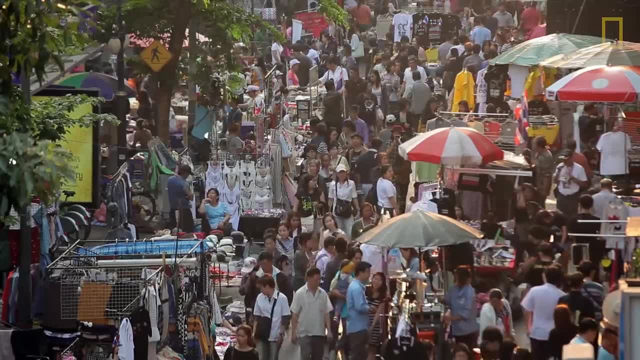 Human activities, from pollution to overpopulation, are driving up the Earth's temperature and fundamentally changing the world around us.